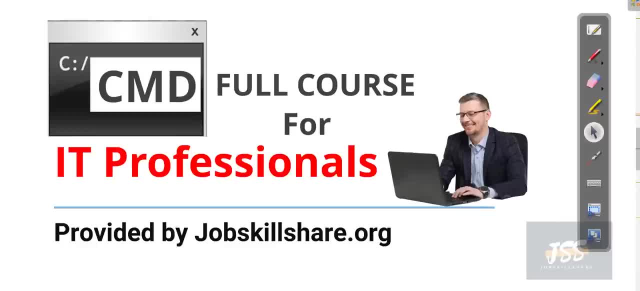 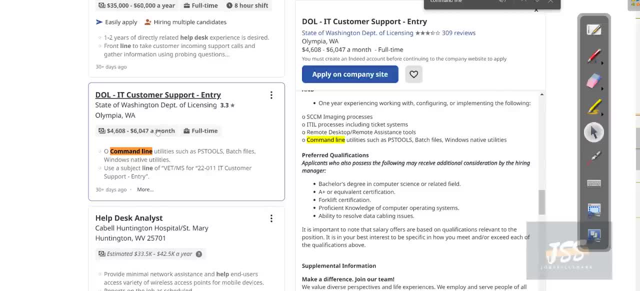 Before you get into the learning zone from JSS instructors, you should be asking yourself a question: why do you need to learn about CMD First? you're going to come across this type of writings and descriptions. So, number one, we're trying to teach you the skills. 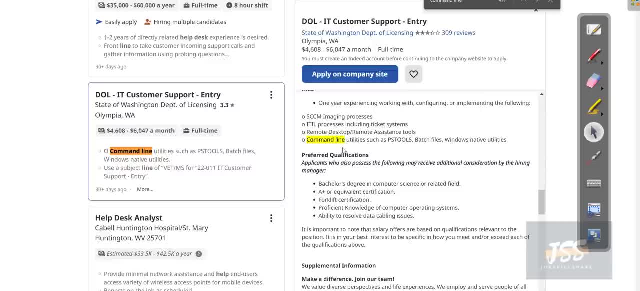 so you can get confident with these descriptions. So one is simply: you're countering the descriptions, you're getting more confident. The second reason is that it doesn't matter what level you are on in IT, whether you're a help desk, whether you are that extreme master level. 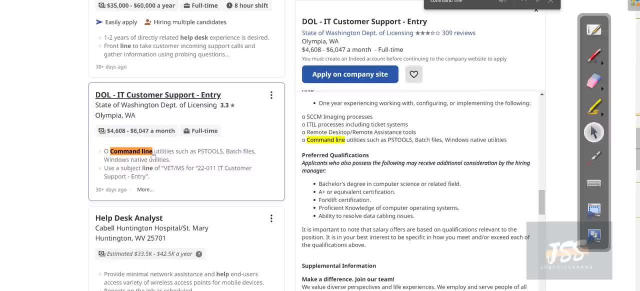 engineer, you still need to know about CMD. Ping is something that you're going to do almost on a daily basis. if you're working at the engineer level, working with Cisco routers or switches, working with servers, working with whatever you can name it in front. 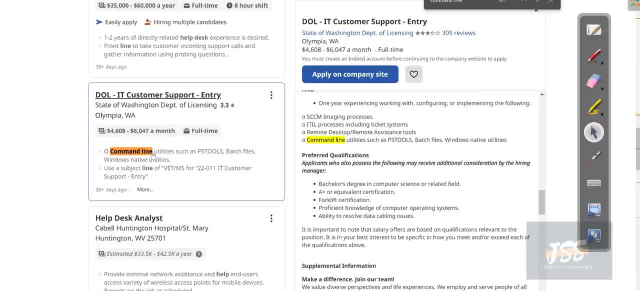 of me, Even at cloud level, you're going to come across. So let's start with the first thing that you are going to do. You are going to use the command line. You are going to use the command line to get you through this. Now, 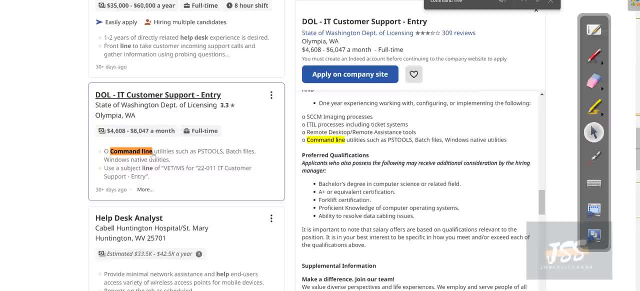 there are different types of command lines. We know that. we understand that There are more advanced things going on in the market right now, Like, for example, a lot of people will suggest to you: well, if you're learning about CMD, then just go straight to Power. 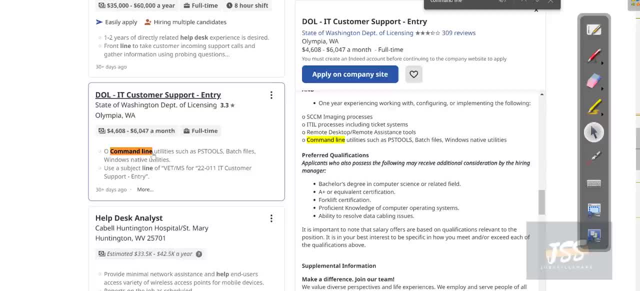 Show. We don't do that in these types of trainings, because our goal is start from something that you you're going to learn about cmd. first, it's going to give you the idea it's going to. it's going to show you how easy it is to use a command line, and then you move on to more, something more. 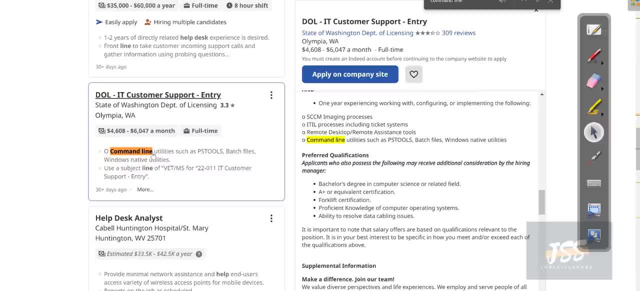 advanced because that's that's how it's designed. things are designed from little basics to more advanced later on. so it's important for you to learn cmd, because you're going to use it if you want to make your job easy. you're going to use it if you want to become a little more experienced. 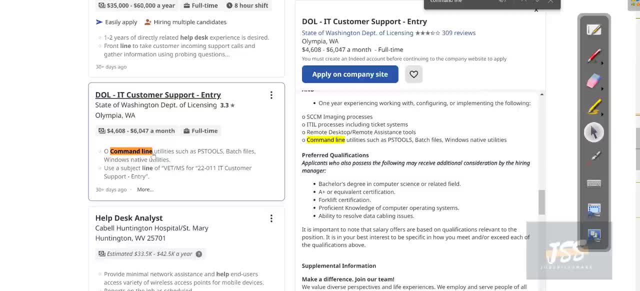 doing things because later on you may want to get into more command line scripting. uh, you know tools like that, where you are working with cloud type of technologies and you don't want to be relying on just a web browser anymore. you want to do things from a command line. so that's later on. 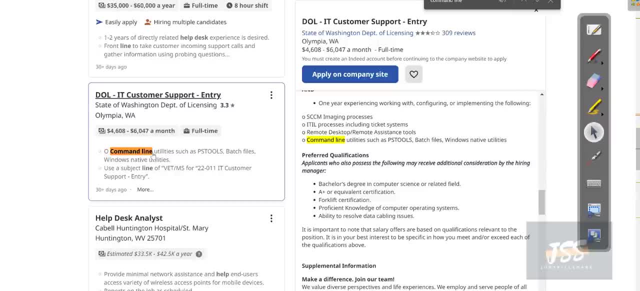 stuff, but for now you need to know the basics of ipconfig ping. you know all that stuff you're going to learn from this whole course and once you finish this course, i feel like you're going to have a very good idea: practical knowledge on how to do it. 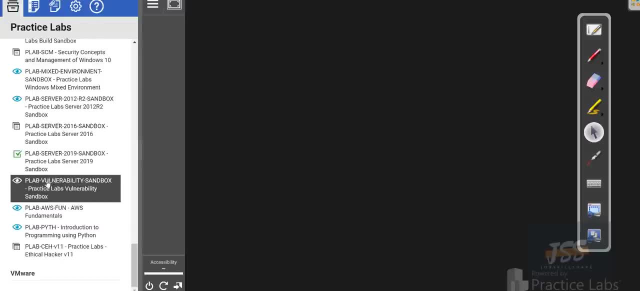 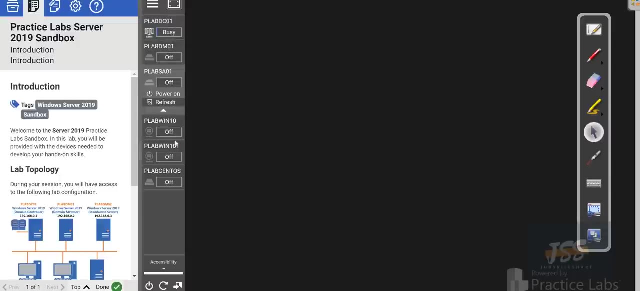 this now, if you have a lab access, sandbox, lab, lab access, if you, let's say, bought the light membership, plus membership, even premium, it doesn't matter. you have machines here and every machine will come with a command line so you can open a server, to open a cmd, you can open a computer. but 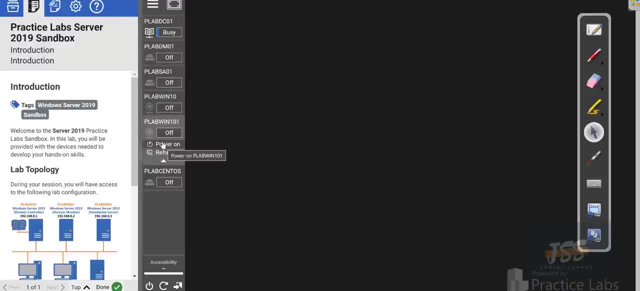 since these are domain joined machines and some are not. you can actually utilize what you learn from this course to find out about actual directory users, informations and and expand your knowledge. this means that you have the tools and that that already comes with active directory and everything is in there. so then go ahead online and then try to come up with more skills and build. 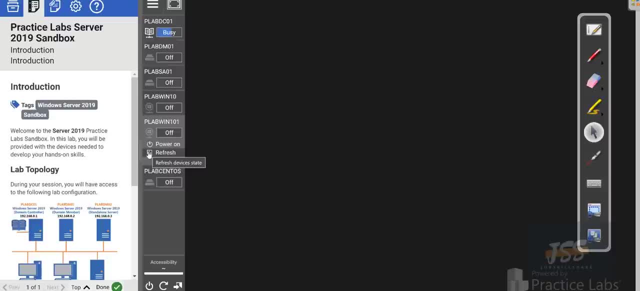 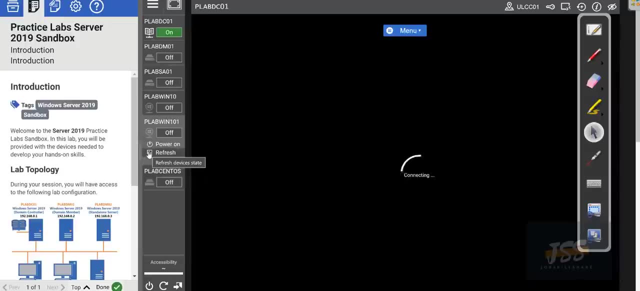 your skills, on top of uh, your what you learn from these videos. so this way, you, you will, you will have a very extensive knowledge on cmd, and this course will be used in multiple courses: network engineer course, sysadmin course, it doesn't matter. every course that we teach it, that's going to be. 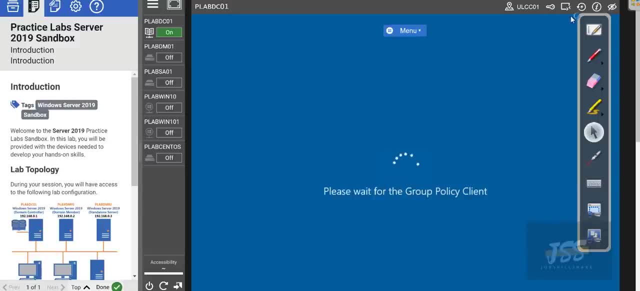 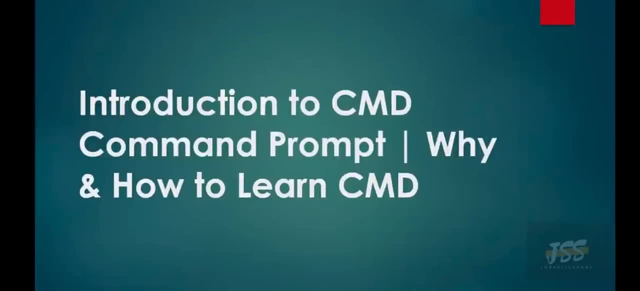 technical this. you will find that it's going to be very useful. so i hope you enjoyed this video. the same video in there. so now uh instructor will take over and good luck. hello, all viewers, and we are going to start this new course named cmd, and the course name is introduction to the cmd command. 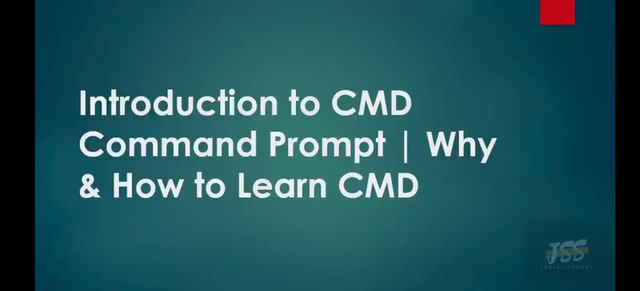 prompt: why and how to learn cmd. so throughout this course you will find that we will show you the importance of command line and we will also address all the answers that you raise the question about that: why we use cmd and what sort of uses we have to use cmd in our daily tasks, daily operation. so let's start. 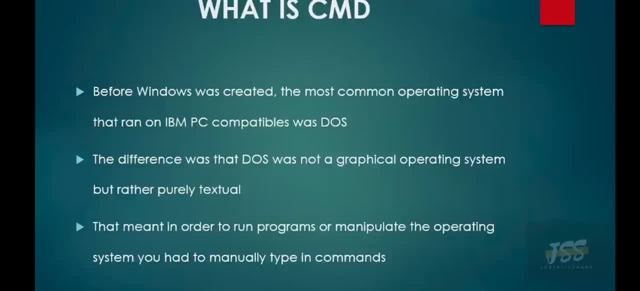 with the basic detail about the cmd, what it is. so, as you know that before operating system, the windows operating system, we have the dos disk operating system and it behaves as an operating system, but what it contains? it's look like a black screen where you could type text in. 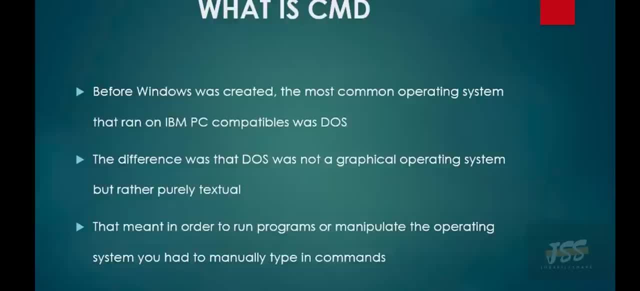 form of instruction. so you must know the command to run that operating system. if anybody, let's say for example, doesn't have idea or don't know about the command, so that kind of person unable to use that computer machine. so this is the basic difference between the command line and the 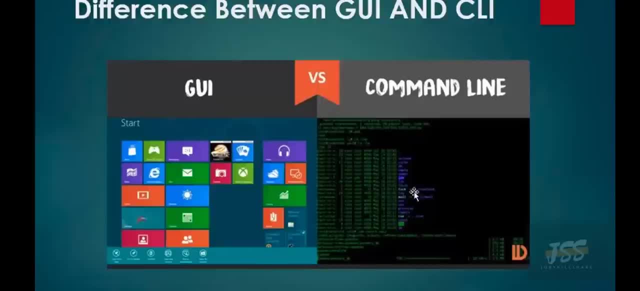 windows operating system is what that? in the command line you only have this black screen and where you could go with the commands, with the text and in the graphical user interface, as i'm going to show you here. you can see that this is the graphical user interface you have. 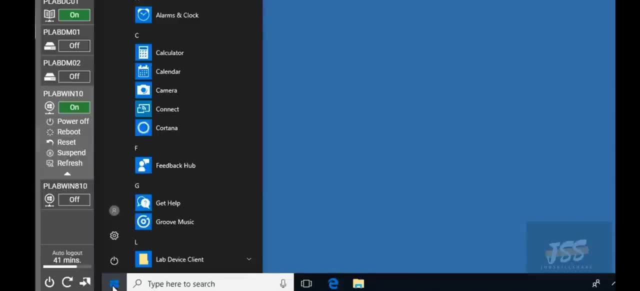 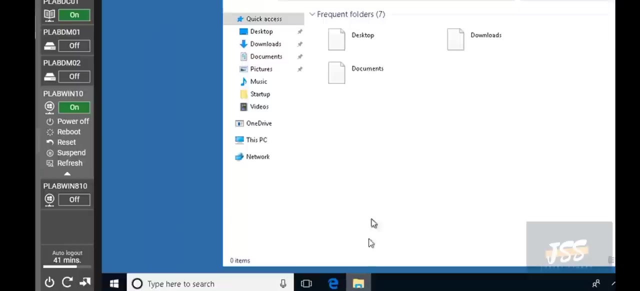 windows 10 offering system right now and there. you can see: if i click on the start window, it will display multiple applications at once, and only i have to use mouse pointer to open any application or even if i want to delete or add any files. so what i need to do is just open the file explorer. and in a. in a glance it just opens it, and or opening it more much. Alright, once opened. now it's going to want to install windows 10. it only needs to get the control with Esc and Enter to do something else. So I press next in. 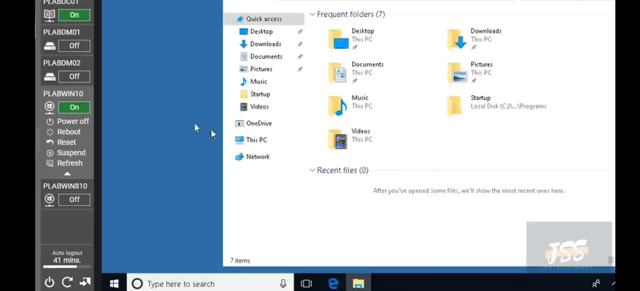 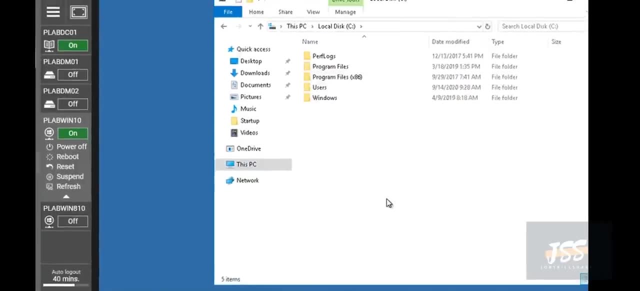 in an instant. it just opened the whole directory in front of me and that here you can see. if I click to this PC and go to the C Drive, so it will start showing me all the content, all the other directories. that is the part of your C Drive and easily you can right click on any of the folder. 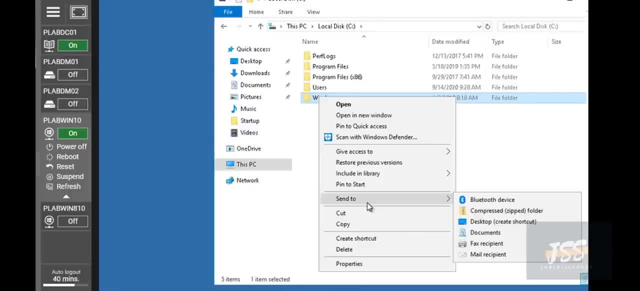 any directory and decide what you want to do with that directory. like you can cut, copy, delete, or if you want to check the properties of that directory, you can go simply in the graphical user interface, unlike in the command line. you need to know the command of each operation. let's say, if I open the 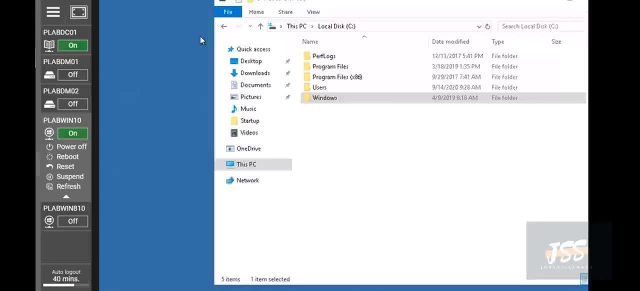 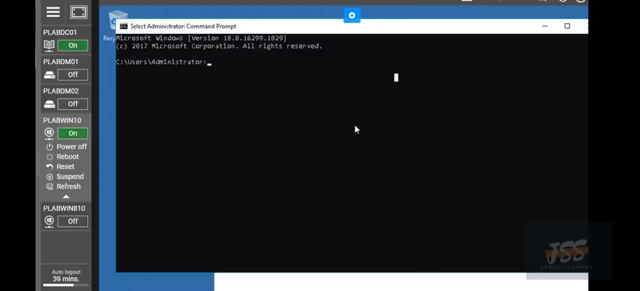 command prompt here and just check things here. so as you can see on the command prompt that I have the administrator prompt here now, here you, only you can use this application by tapping the command. let's say, if I want to clear the screen, so I must know the CLS command, clear screen command, so you. 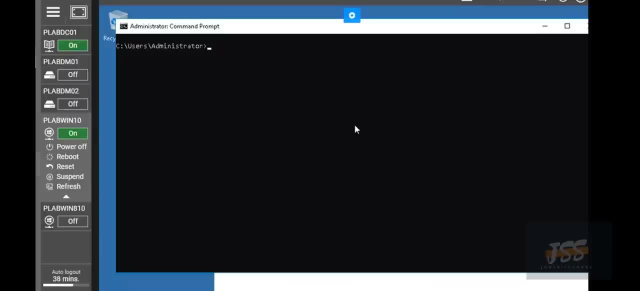 will see that. it will show you that you can use this application by tapping the command. let's say here: you will find that the command line is not user-friendly, but you can do a lot more things. you can even use this command line as your basic operating system. because why I'm teaching this? 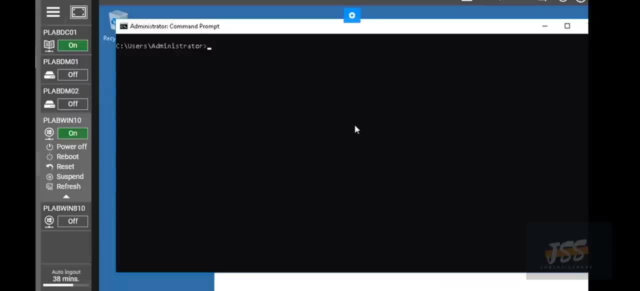 course. why I'm designing this course for you? because in many organization they are moving toward the server core product. and what is the server core product? it is different with the Windows Server operating system. here you will find the command prompt and the PowerShell. now the question is raised: what is the PowerShell and what is the difference between the command line and? 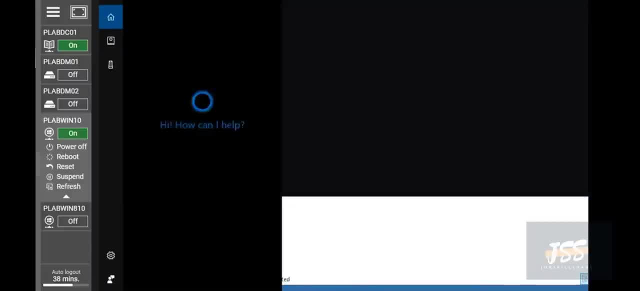 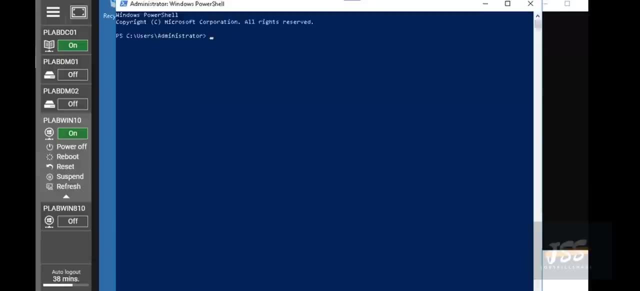 the PowerShell. let me show you how the PowerShell looks like. if I type here Windows, so it gonna suggest me in the second option, Windows PowerShell. so the major difference you can see here is in the color. now the color of the PowerShell is like blue and you will find the black color in the command. 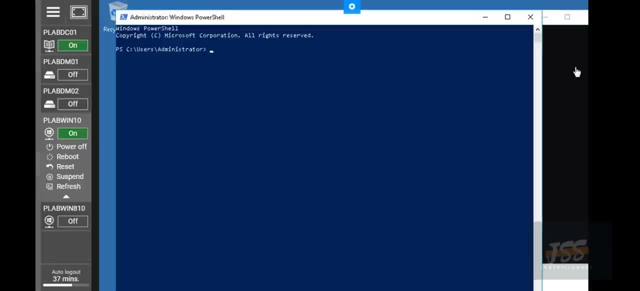 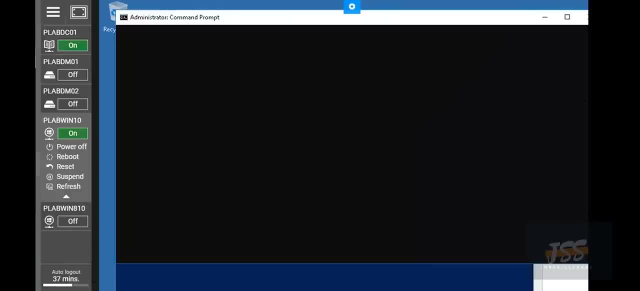 line, but that's. that's not the main difference. this is the difference of color. here you can see there's a mentioning of PS. so you can even open the PowerShell on the command line and the way to judge that whether this is a command prompt. this is the PowerShell. you can judge with the prompt you will. 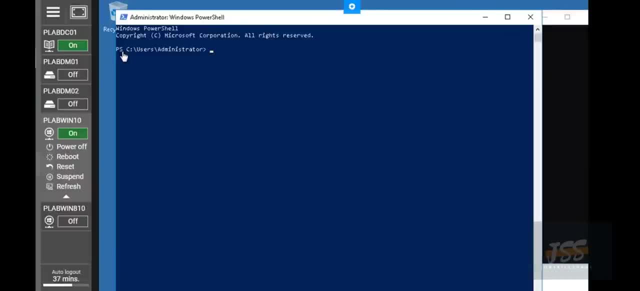 find PS in the beginning. that tells that this is a PowerShell mode. so if you go with the name, as the name suggests, the PowerShell, what it tells, that here on the PowerShell you can do wonders, you can manage things, you can run objects and it is more friendly when you are running a script. 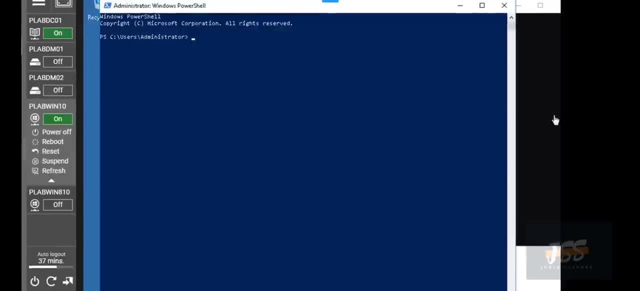 on your for operating system. this is not being easily done on the command line. so this is the major difference, and there are so many differences between the command line and the PowerShell. but as for this introductory video, and our focus is on the command line, the cmd, so that's why we're 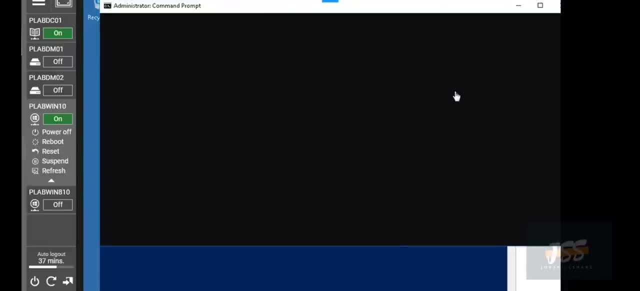 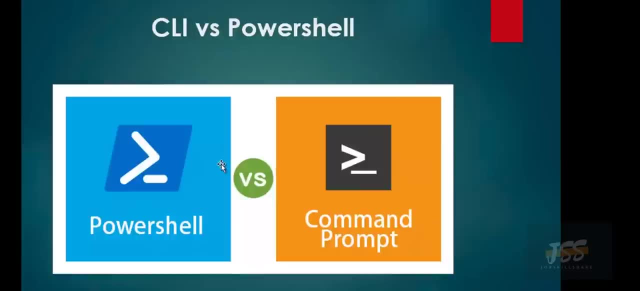 going to explore this later. what is the major difference between the PowerShell and the command line? but as for this introductory video, you only need to know that the PowerShell allows you to run a script and it can run different batches file by the command line, because it is originated with the microsoft company. it is designed and 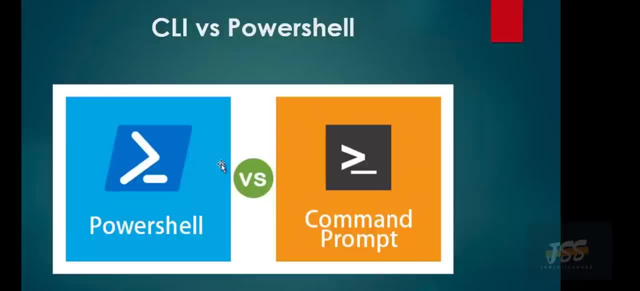 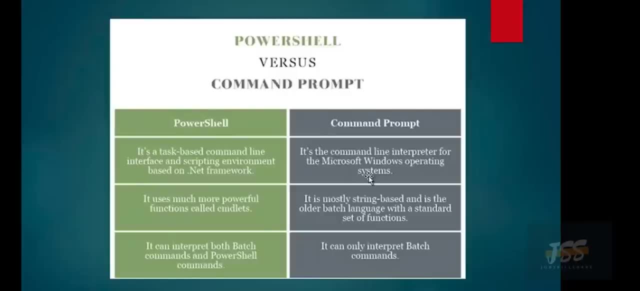 provided by the microsoft. that's why it run only basic instruction and if you further explore the differences between the powershell and air, so you will find that it is a task based command line interface and use also used for scripting environment and it is based on dot net framework. 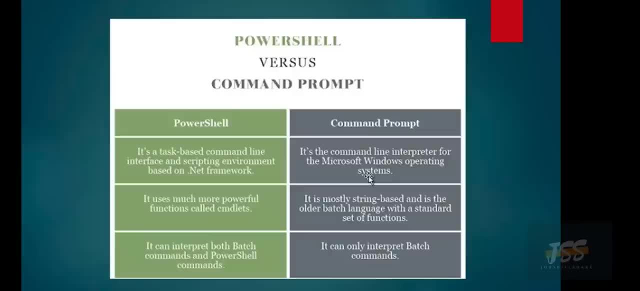 but unlike command prompt, it is just a line interpreter for the microsoft windows operating system. so there are so much difference and you can also call the commands of the powershell as a command list, but in the command line, in this command prompt, the commands are just called. 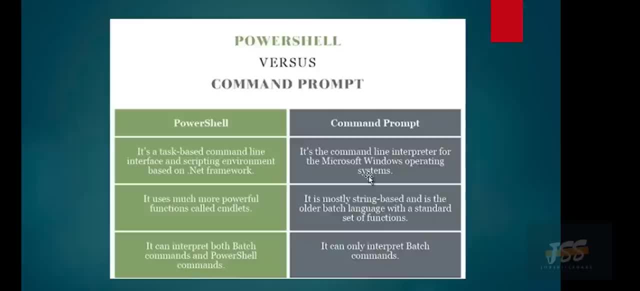 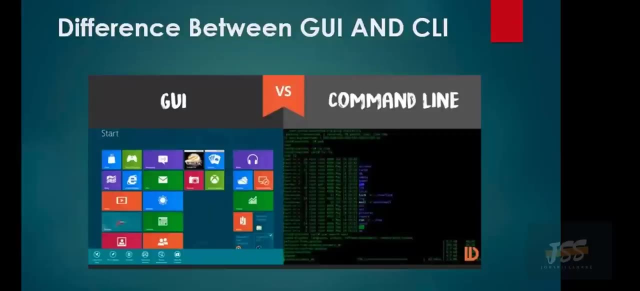 commands. so this is the major and basic difference, but there are a lot more differences that are just beyond this moment, beyond this video. we will discuss later. but during this course you will find that how we are showing things to you and how we are making this thing. 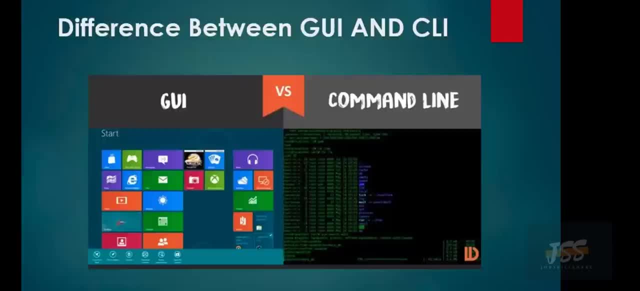 important for you because command line will help you in doing networking. you can do so much work, so much tasks related to the networking. even you can fix issues. you can use the command line in hacking and mostly you will find the command line interface in the routers in the networking sector. 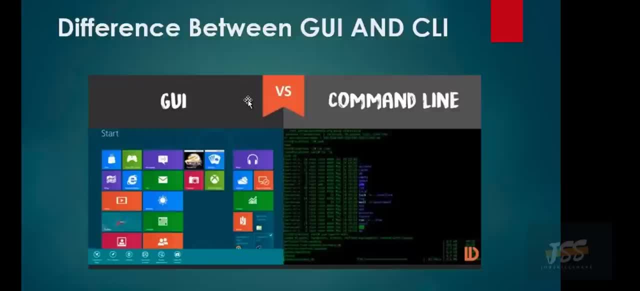 here they provide the command line where you need to know such basic command line commands to see the router properties. and similarly, we will talk about all those commands that are used in the windows environment in the command line to do further things like delete directory at directory and format partition, and there are a lot more things that we are going to cover to. 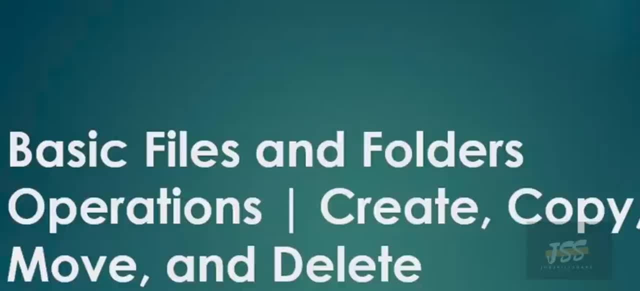 deal with the basic file commands: how to make folder operations, how to create sided and how to copy files, how to move files and how to delete files and other things. so in the next part of this share files and the folder in the command prompt. so let's go back to the desktop environment and 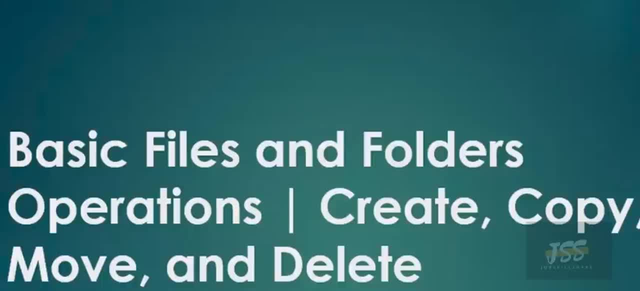 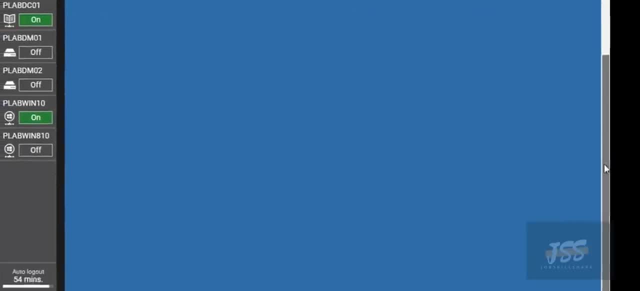 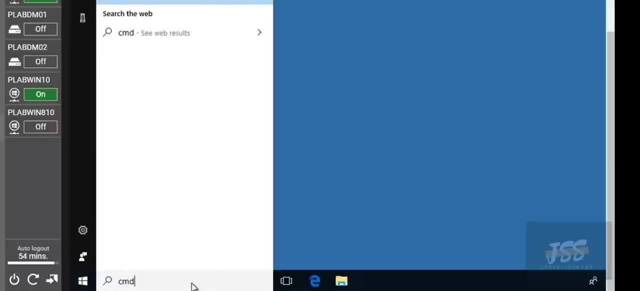 let's open the command prompt to further show you the operations and the steps. now, here I have this Windows 10 desktop machine and here in type, here to search, I'm gonna type CMD to show you these commands and their functions. so here, once you open the command prompt in your Windows 10, you 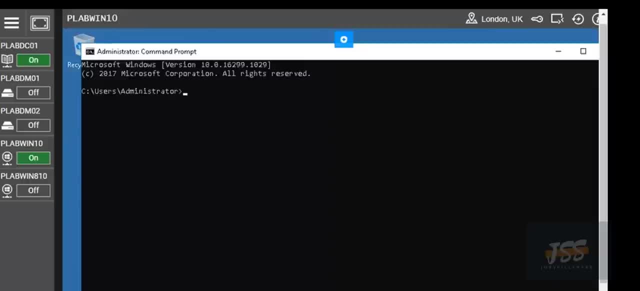 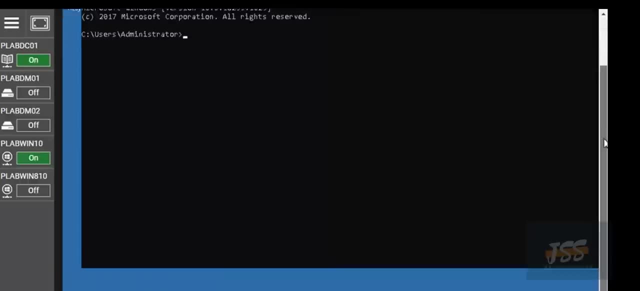 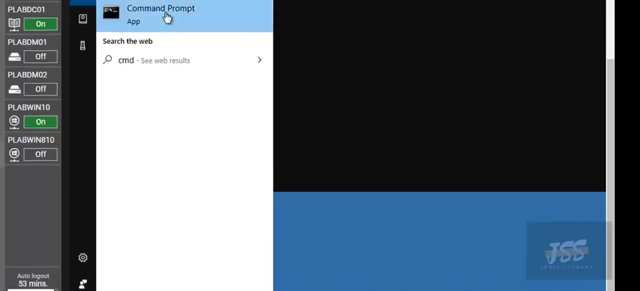 will find that it shows the administrator prompt. sometimes it came with the system 32. that depend. if you open your command prompt as the administrator privilege. let me show you. it is a little advanced thing but you need to know at this level if you right click on the command prompt. so 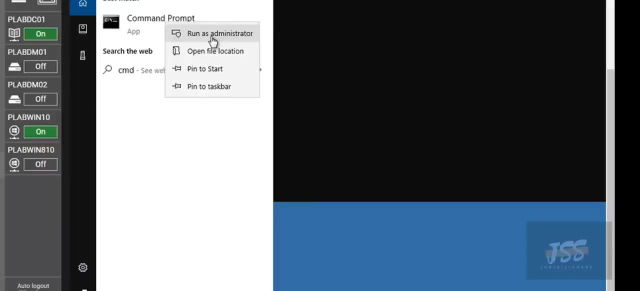 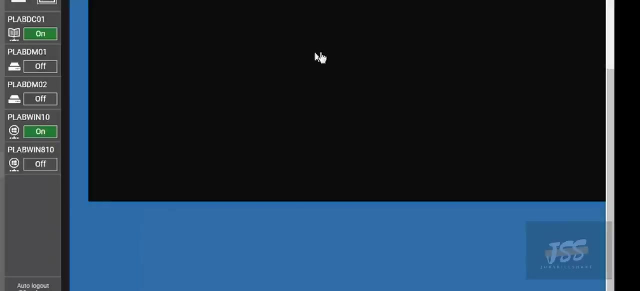 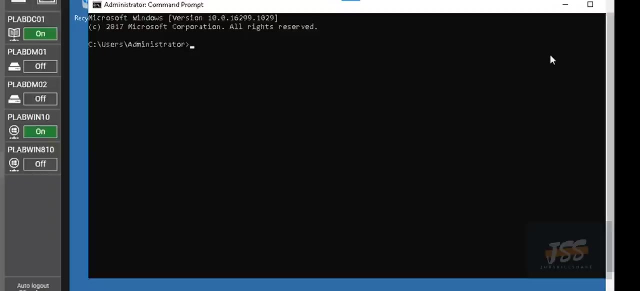 you will find this run as administrator. so this command prompt that you opens on the administrator privilege have some other powers. you could say have some other privileges to run things, to execute files, but here, as for this lab, we're going to just focus on the copy, delete, CD, those basic command that can easily be executable on 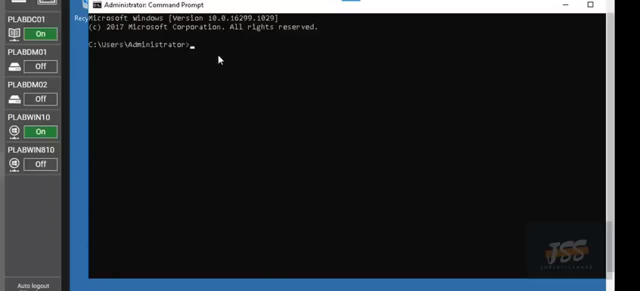 any level, any privilege of the command prompt. so, as you can see, that the whole tree of the directory is the originated directory, the C where you have your operating system, then you have user folder and in the user folder you have administrator folder. so this is the tree of directory. let's say: 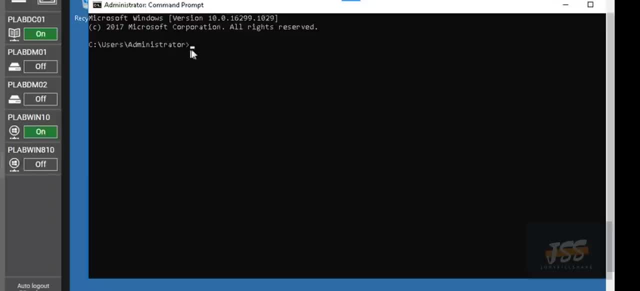 if you want to go to the user directory, right. if you want to change your current directory and you want to go to directly to the user, not to the parent directory, so the command you're going to use is CD double-dot, and if you press Enter so you can see that you just directly jump to your user directory. let's say, if 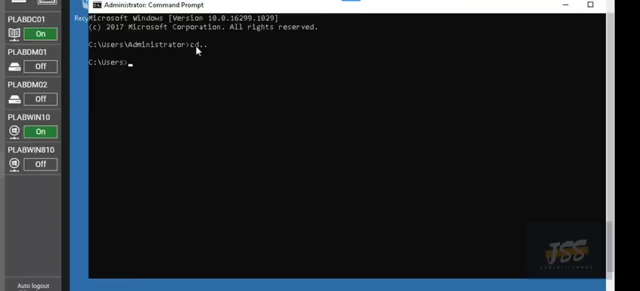 you are in the user directory and you want to see the content that both sort of file and folder are there in the user. so type dir and you will see the contents, the folders, the files you have in your user directory. so here you can see you have admin. definitely, this is the admin account. the administrator. this is another admin account. 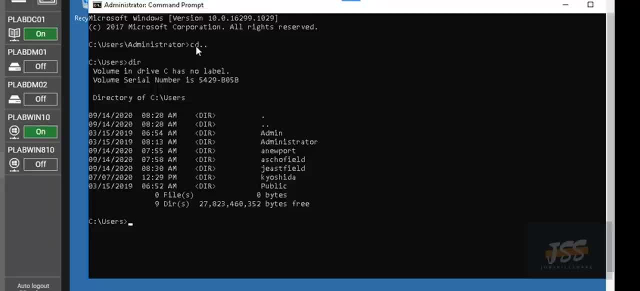 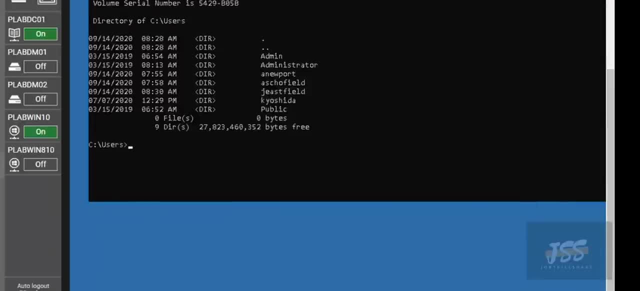 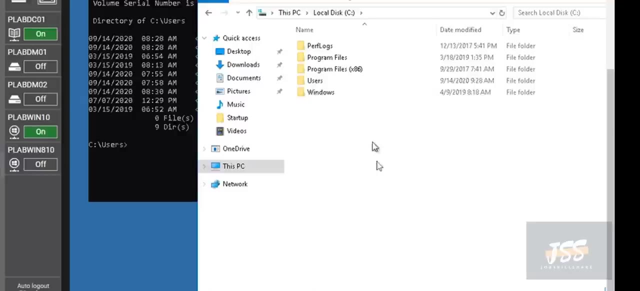 a new poet is co field, g's field. these all are what? the user account. this is the same folder that we access in a gooey way. let me show you if you are getting confused. if you go to this pc and go to the c drive and there's a user and here you can see the list of directories, the folders that 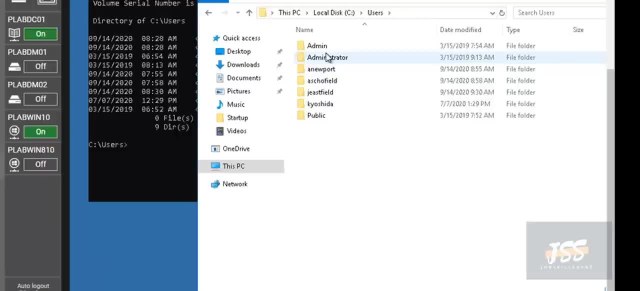 are actually the account folder. they contain all the data, all the activity does in the account, like the pictures, videos. let's say, if i open the, a new port, so you will see the content, like the desktop documents, download. so whatever the user is doing, like you know, downloading files, making documents, 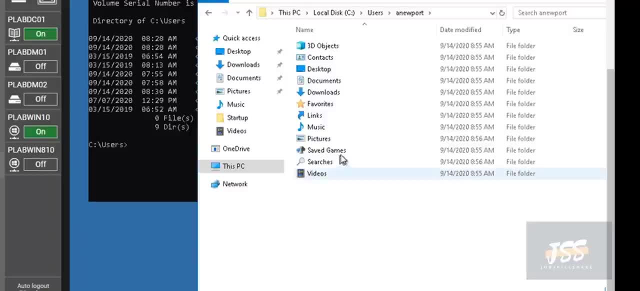 or just downloading music or making pictures, so you can access all such content from your account. so you can access all such content from your account. so you can access all such content administrator account from your c drive. so this is that specific user folder that we are dealing. 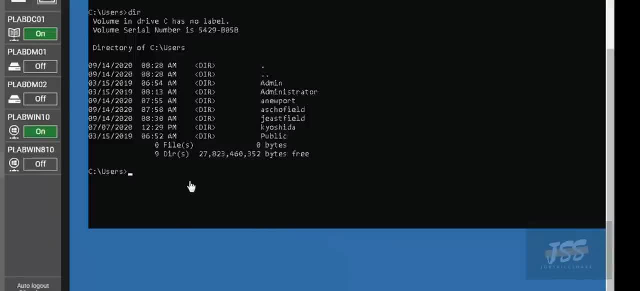 right now in the cmd. so so here what you're gonna do. so if you want to go to any of the directory here listed, so what you're going to do is just type cd space, admin, and press enter, so you are in this admin directory. so which command is? 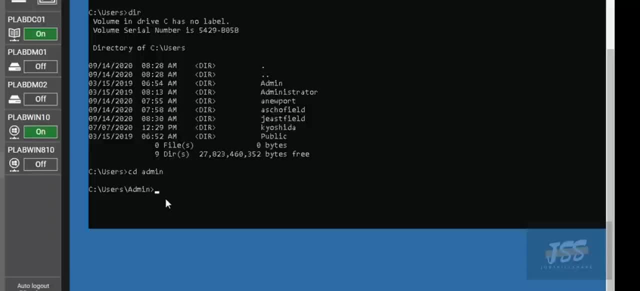 used to go in any directory to open any folder, cd space and that specific folder name. and let's say, if you want to go back to your parent directory, which is the c here, so you're going to type cd backslash, enter, so it gonna took you directly to your parent directory, which is the 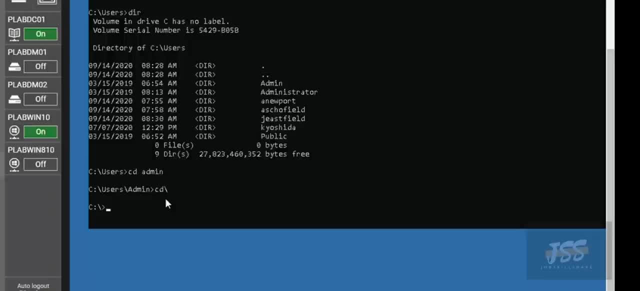 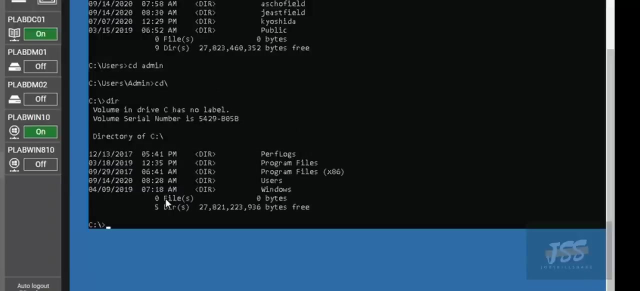 c. so have you got this idea that if you want to jump directly to your parent directory, so you're should use cd backslash? so it is simple. so let's say, if i want to see the contents of the c drive, so what command i'm going to use? is dir directory, right? so here we have. 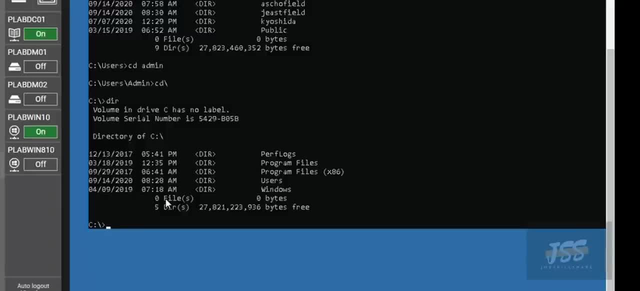 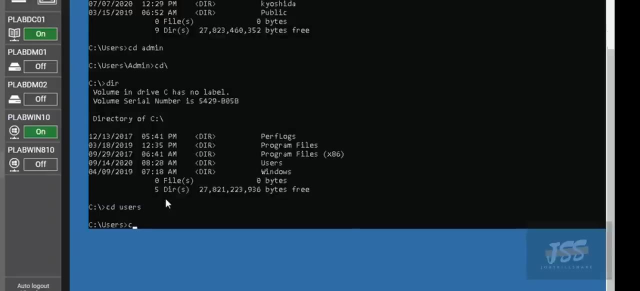 preferred: logs, program files, users, windows. there are four, three or four folders here, right? so let's say, if i want to go back to the user, so which command i'm going to use- cd users- right then. if i want to go to the administrator account, so what i'm going to type. 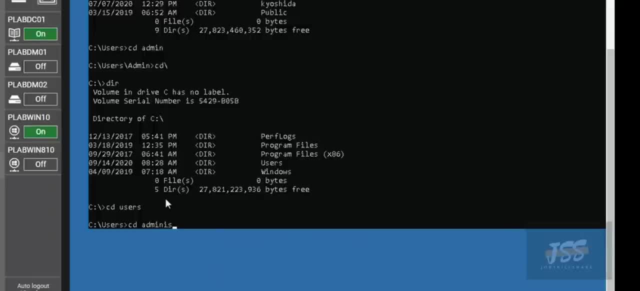 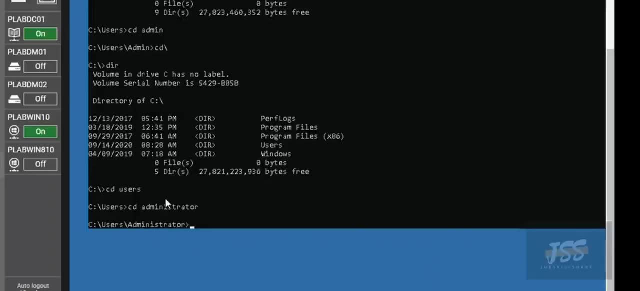 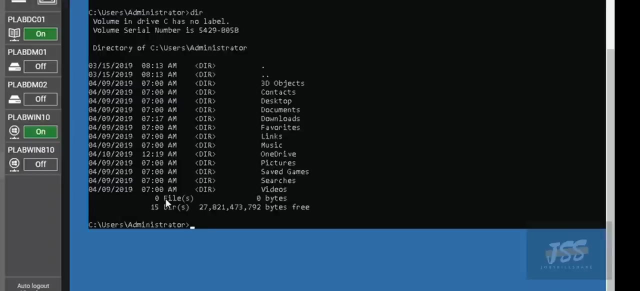 add administrator: admin. this trader enter. now you are on the administrator account. so if i want to check the directories, the sub directories of the administrator, so i'm going to find these. so right now i want to go to the desktop to do some other stuff, cd desktop. so here you can see. 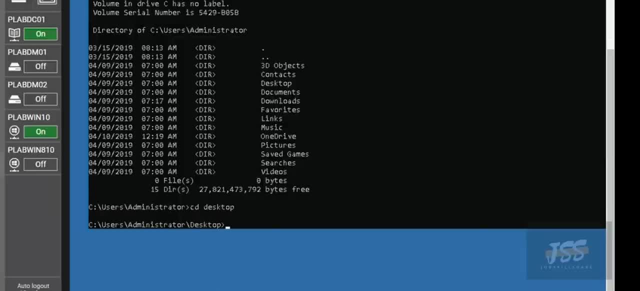 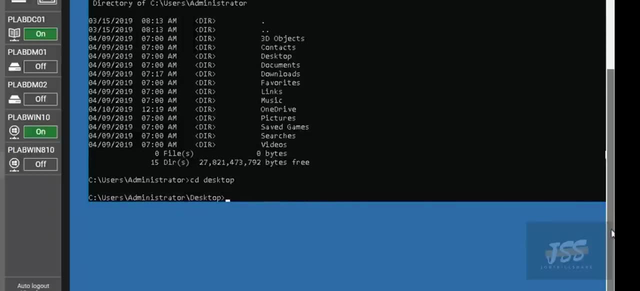 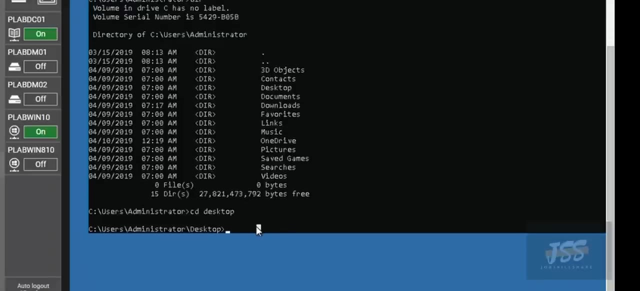 i am in this desktop directory. this is the same desktop you are seeing here behind the cmd application. so let's say, if you want to make any new folder in the desktop, so which command you're going to use. and you want to create a new folder in the desktop, so which command you're going to use. 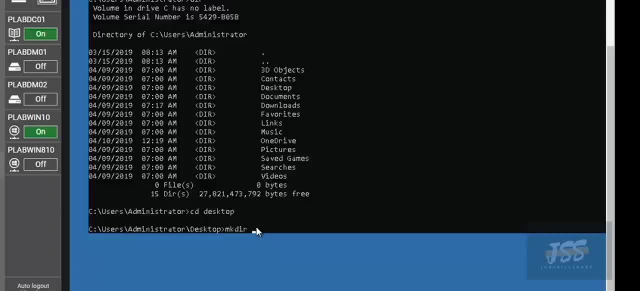 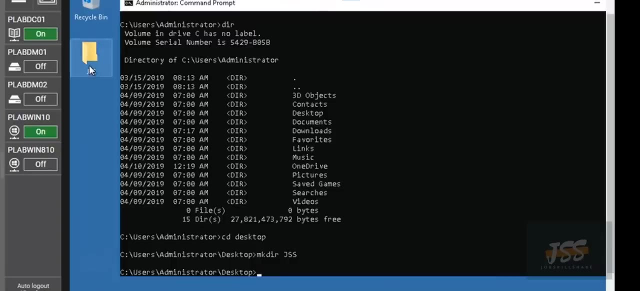 mkdir and that specific name. let's say i'm going to type jss, enter. so there's a folder. gss has been created at the back of your screen, means on the desktop folder. let's look at here, right? so if i want to go to that folder, 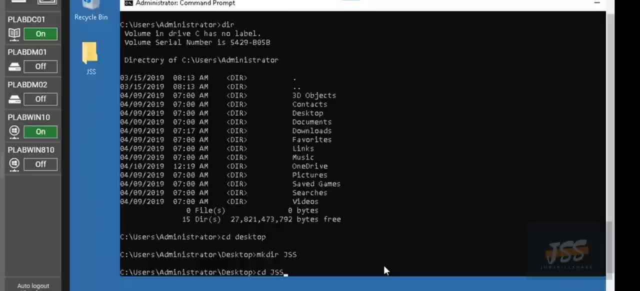 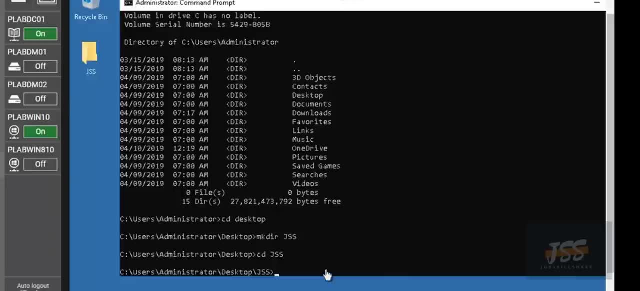 so which command i'm going to use: cd, jss, enter. so there you go, i am, and i'm in the directory, I'm in the JSS, so so it's simple. now let's say if I want to change the name of that folder and, as you can see, if I want to go back one step back to that directory, what I did, cd. 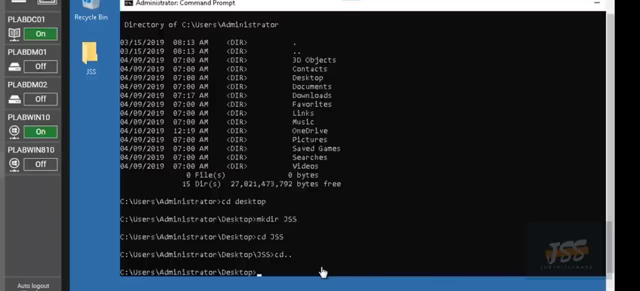 double dot. that means it will take me one step back. directory to the JSS. so if I want to change the name of this folder, so what I'm gonna type is our en space JSS, which is the previous name, and type P labs, enter. so there you go, the file name. the folder name is totally changed with the. 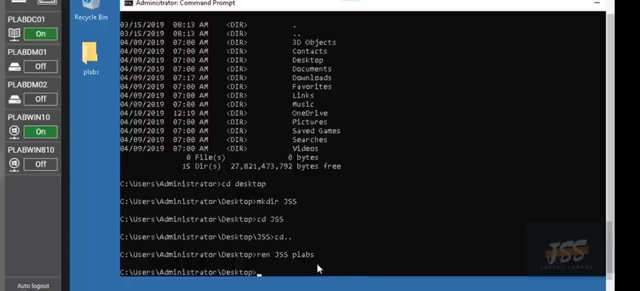 execution of enter. so that's how the command prompt work. that's how the command line works. so let's say, if I'm gonna create a new file in this JSS, in this P lab, so what I'm gonna do is type CD space, P labs, because the file name is chain now and let's get in that directory. now here what I'm 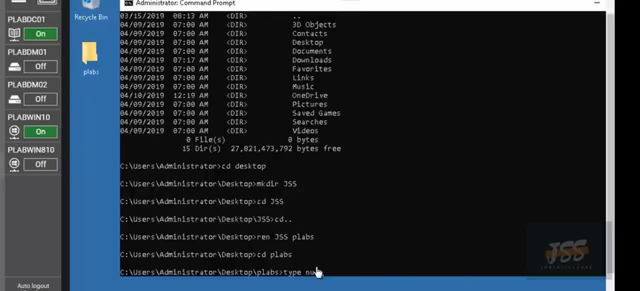 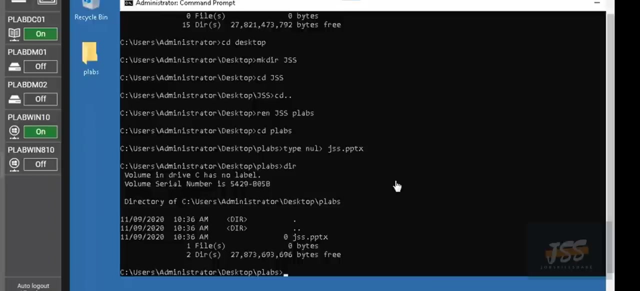 gonna type type space null greater than sign space. type the file name, and this would be JSS dot PPT X. enter. so it gonna create this file and if you want to check, just type dir and there you go. this is the file you recently created. so let's say, if you want to change the file name, so you will use the. 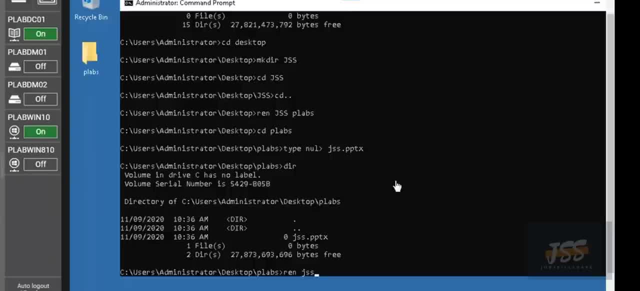 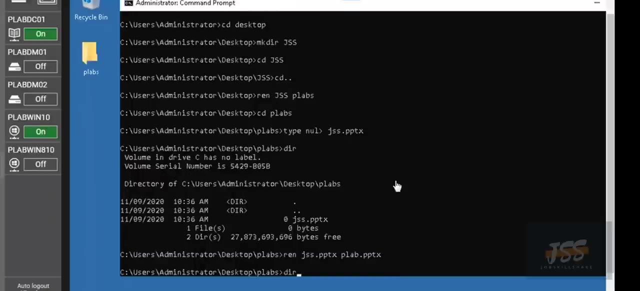 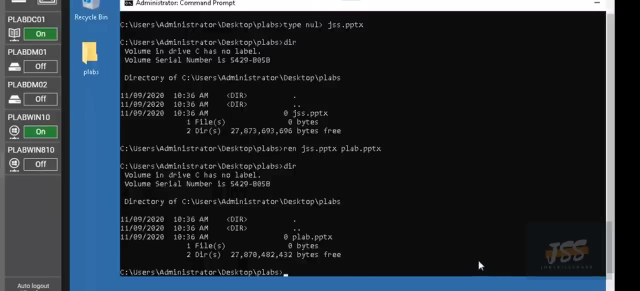 command run re and rename is space JSS dot PPT X. it's space and you could name it as P lab dot PPT X. enter. so there you go, the file name is change and if you type dir so you can easily view that file here, that the P lab dot PPT X. so this is the change happen once you execute this rename. 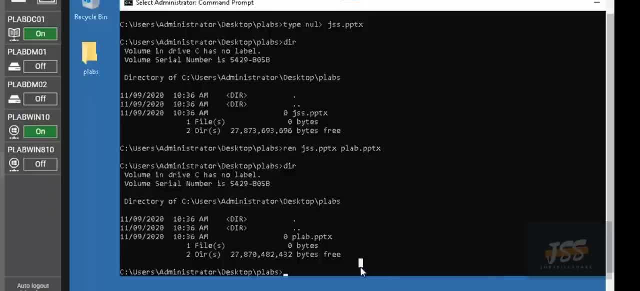 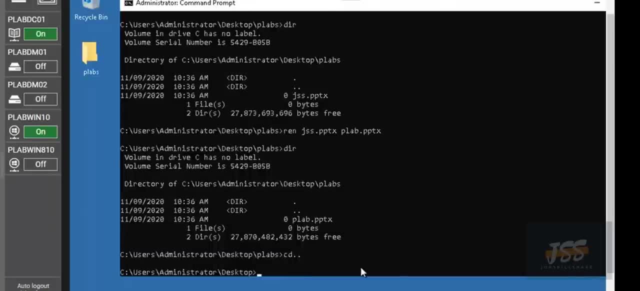 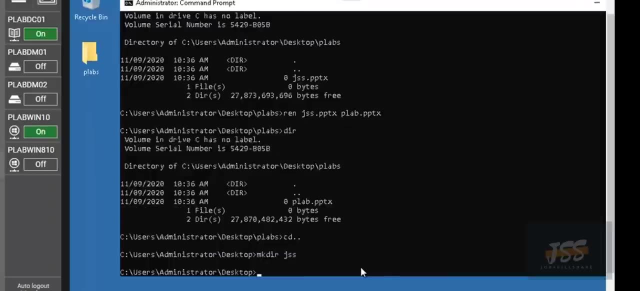 command. now let me show you how to copy the file, how to delete and how to move the file. so if I want to go back one step back to that directory, I want to make another folder. so which command? I'm Katie or your space, JSS. now you will see another folder on your desktop and why I created this. 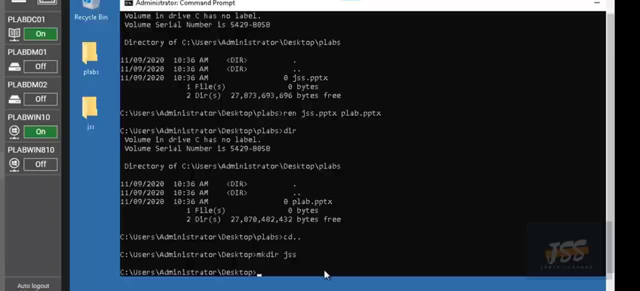 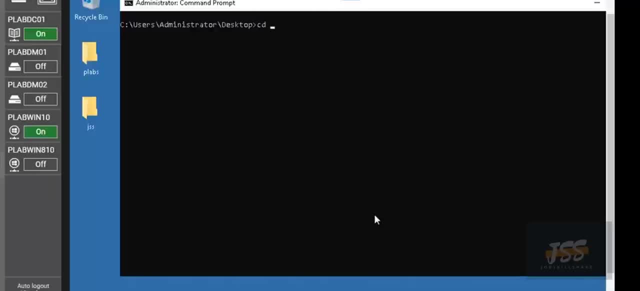 folder to copy and move the file from P labs to JSS. alright. so to copy the file from any folder you must go to the CD P labs. this is the folder that contained the file, and the command I'm going to use is I'm going to change the file name to P lab dot PPT X space and the destination folder. so 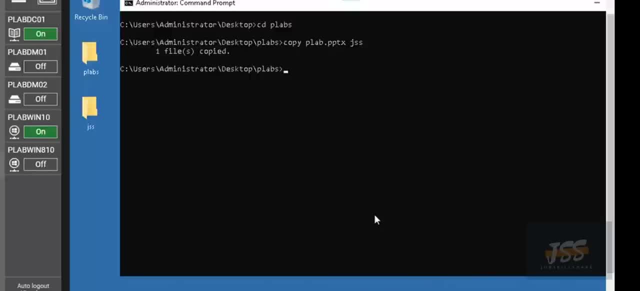 you can see, the fun file is copied. that's the process to copy any file from any location. now let me show you how to delete the file. so first I will go to the DIR to check the file existence. yes, there is one file is a P lab and under file is JSS. we have two files here, so we will make a. 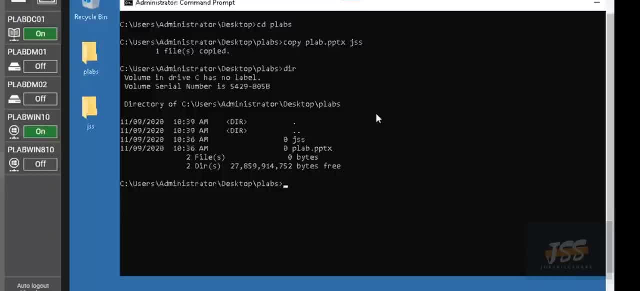 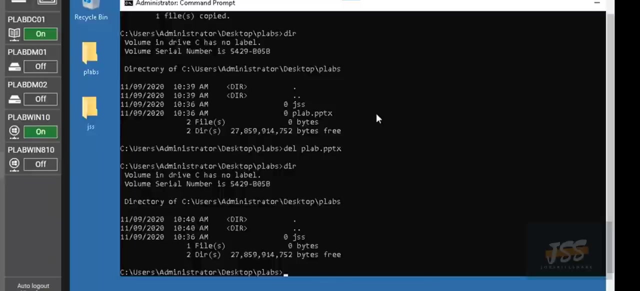 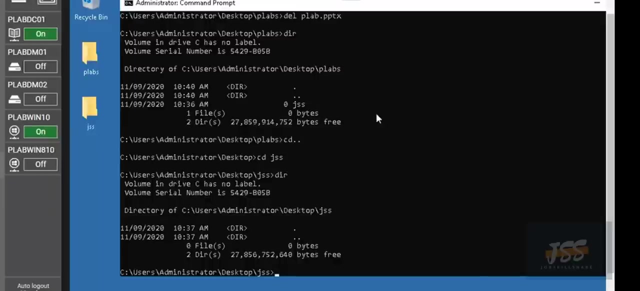 so what I'm gonna do is simply delete the file. type del space: P, lab dot, PPT, X. enter and there you go, the file is successfully deleted. now, if I type dir to see so there's only JSS folder here and there's no any other file located here. so here there's nothing know any file. so let me. 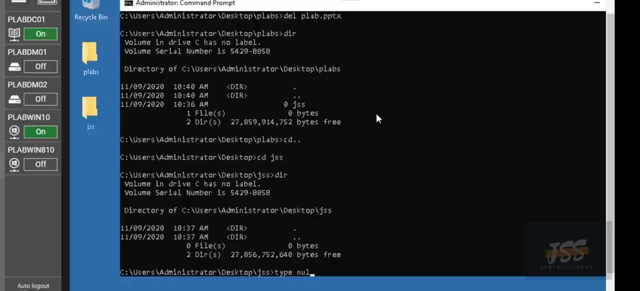 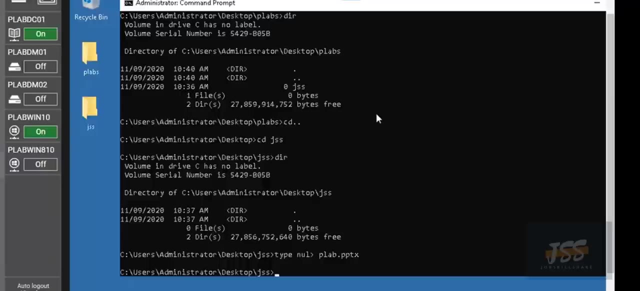 create the file. first, type: space no greater than space P, lab, dot, PPT, X. enter. so there you go, the file is created. now it's time to move the file, because we show you how to copy, how to delete, and now it's time to learn how to move the file from one folder, from one directory, to another. now 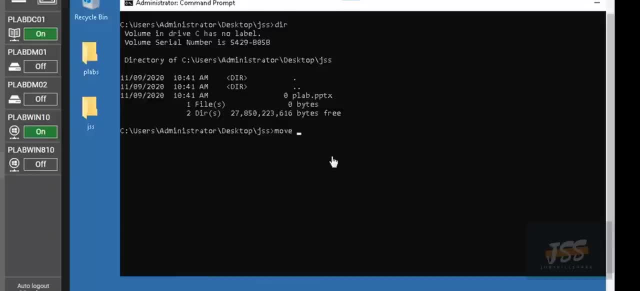 there's the file and I'm gonna type: move space P lab dot. PPT X. all right, PPT X space. and now here I'm gonna type the new folder name P labs, enter. now the one file is move. now here in the last, let's cover the last command and that the command is used to remove the directory and the folder and 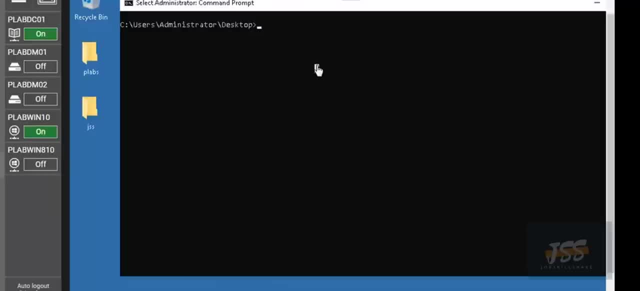 the command is RM. if you want to delete any directory you should type RM, dir, space, JSS and it will quickly delete the directory. but before that you need to clean that directory. so let's go to that directory- CD, JSS- and type dir to check the content. and here you have P labs file. so let's start type del space P laps. 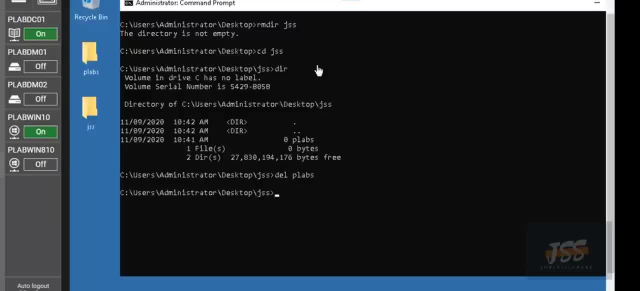 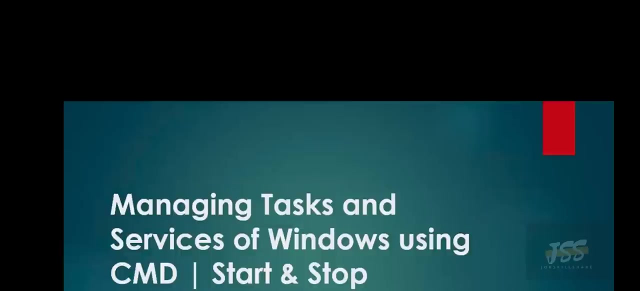 enter. now the directory is deleted. it's not the file, that's the directory. and then it's time to delete the CSS. so CD and then type RM, dir, space, JSS, Enter And now it's going to totally clean, totally delete that directory from your desktop. How to manage tasks and services in the Windows? but by using the command line, the CMD. So let me take you to the practice labs portal and then show you what I'm talking about. 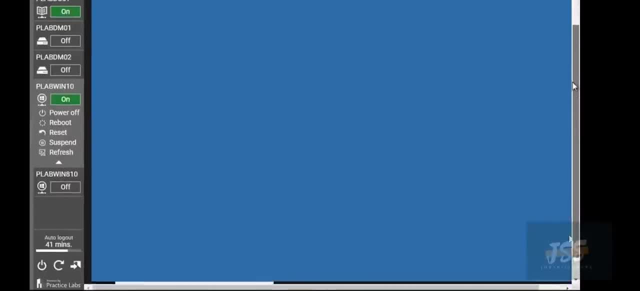 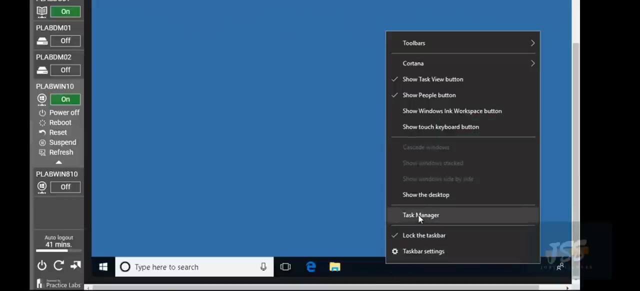 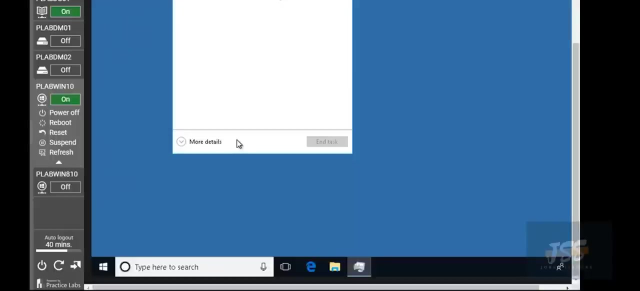 Okay, So here I have this Windows 10 machine and let me explain you that: what is tasks and what are services? If we talk about the GUI, the graphical user interface, so if you right click on your task bar so you will find this task manager. And if we explore what tasks, tasks mean there is something going on, means you are doing something and activity is going on in your machine. 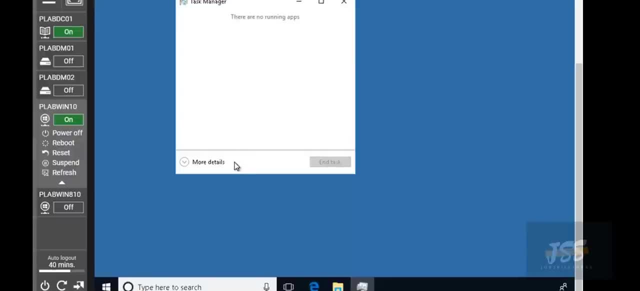 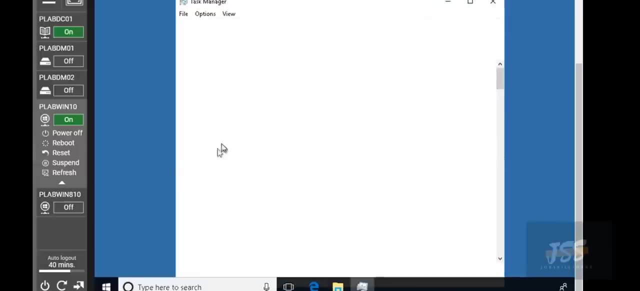 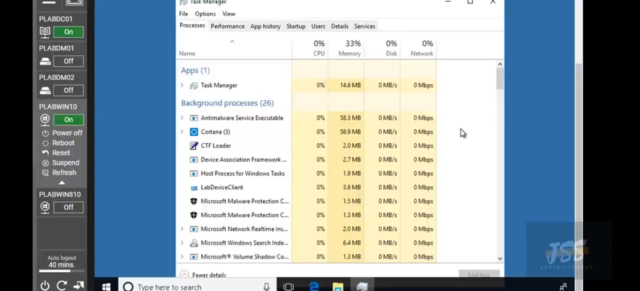 Like in your daily life. tasks is what you have to do, what is your intention to do something. So tasks is that. In the same way, in a computer system, there are a lot more tasks, a lot more services that started with the logging on of the machine. 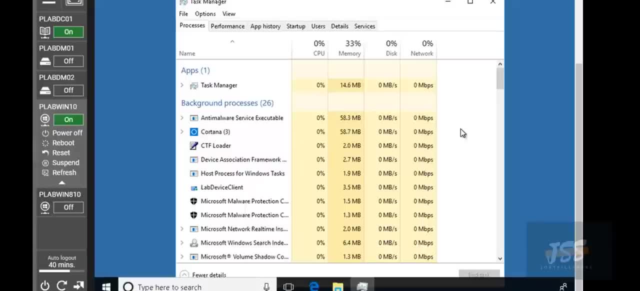 Let's say, for example, when you type your password and username to log on, there are pre built in services and tasks that needs to run To show you the proper graphical user interface desktop. So right now, if you are easily watching your desktop like that, because there are a lot more services that are running in the background and there are a bunch of tasks, there are those are also running in the background and making it possible for you to easily use this graphical user interface, because it is not the colors right now. 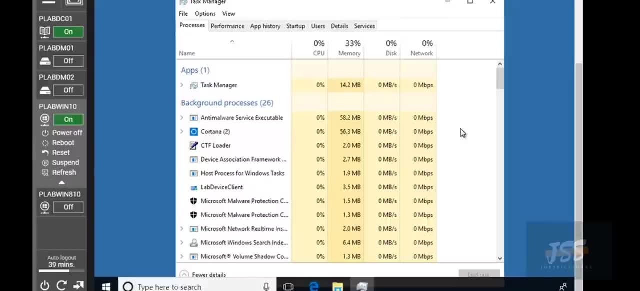 There are. There are a bunch of services and tasks making it possible for you to see things like that. So here in the task manager you can see that even we didn't open any application, we didn't started anything. but there are a bunch of tasks are running here and a lot of processes are going on. 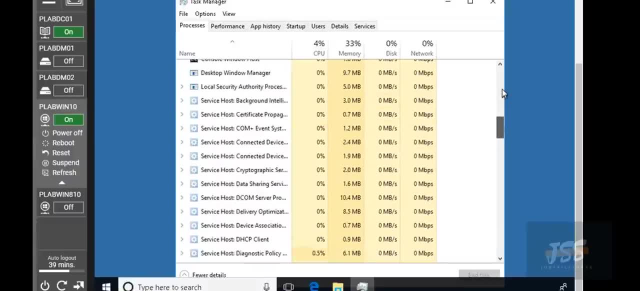 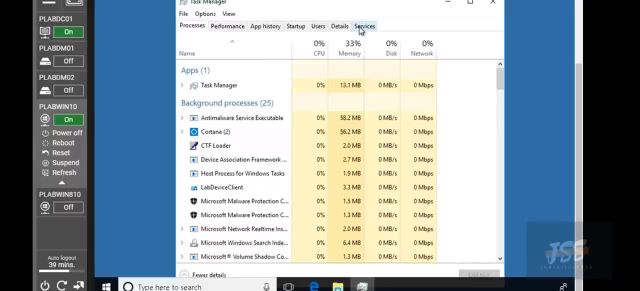 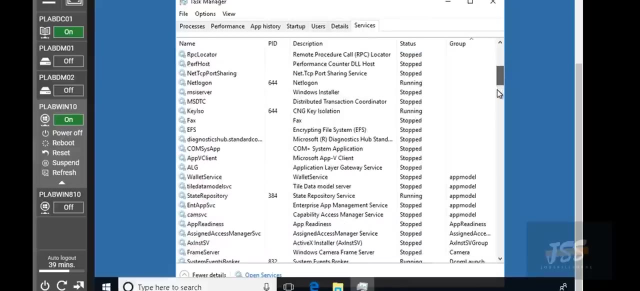 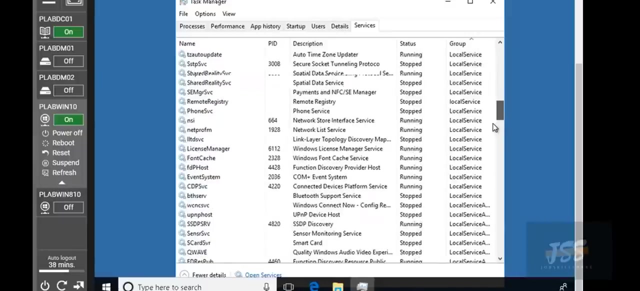 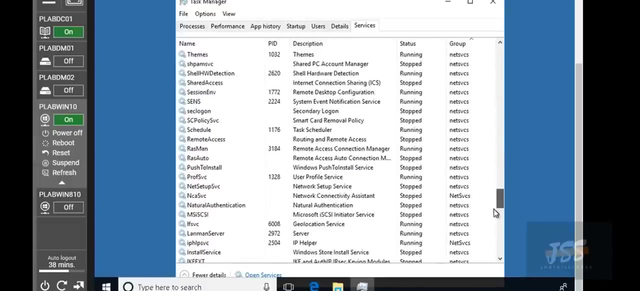 And these are the backup and supported tasks and services that are supporting this desktop feature, This Graphical user interface Thing. And if I click to the services, the last tab, so you'll you're going to see that there are Bunch of services that are running here you can see, and a couple of services are stopped and some are ready to start, but there are in majority, there are in. the vast number of services are running. 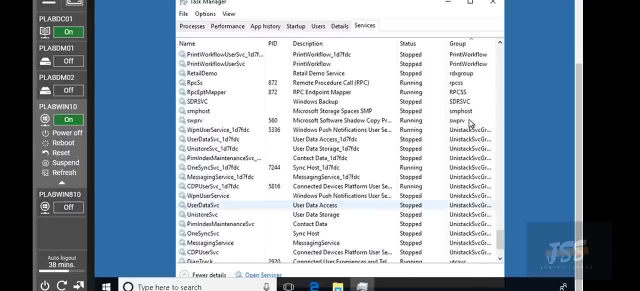 Why? Because these services are running in the background And And just maintaining and managing this whole user interaction based desktop. That's why those all services are really needed and essential to use this graphical user interface. now, As for this video, I'm going to show you how to control, how to manage all those tasks. services to CMD, the command line. 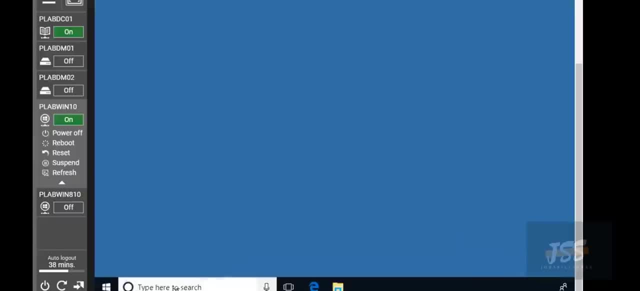 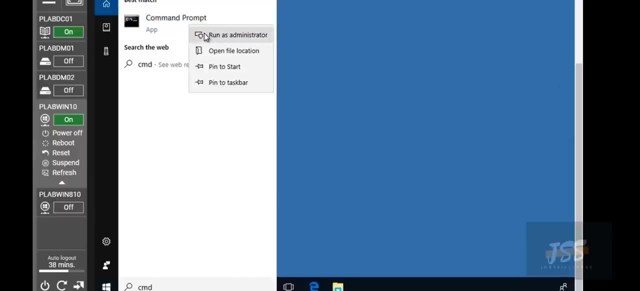 So let me close this Task manager from here and there. I'm going to type CMD, type here on search and this time I'm going to open it as administrator privilege. by The question is raised why I'm opening it with the administrator privilege. because we have to deal with the services, with the task and in lot more. 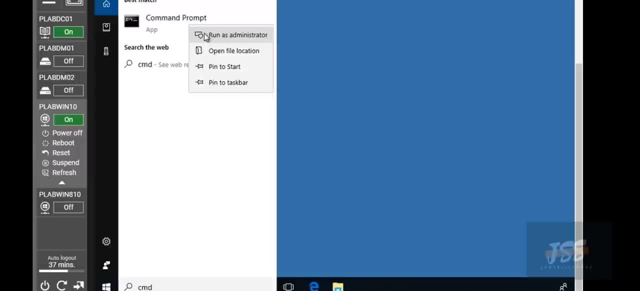 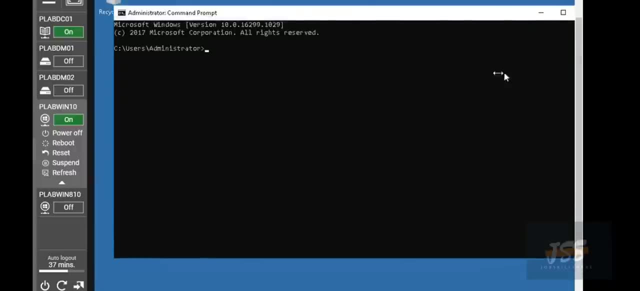 Situation. you need to be the fully controller of the device. That's why we need to run as an administrator, because there are Lot more services. Windows system doesn't allow a basic user to stop or terminate that service or task. That's why we run this command from as an administrator privilege. 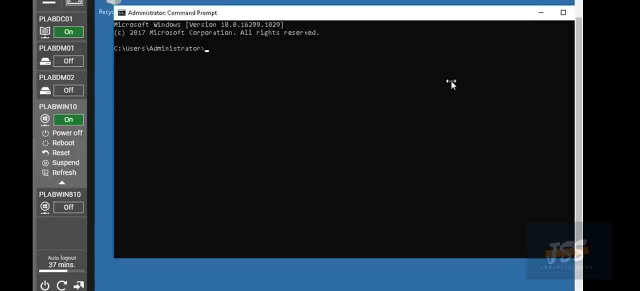 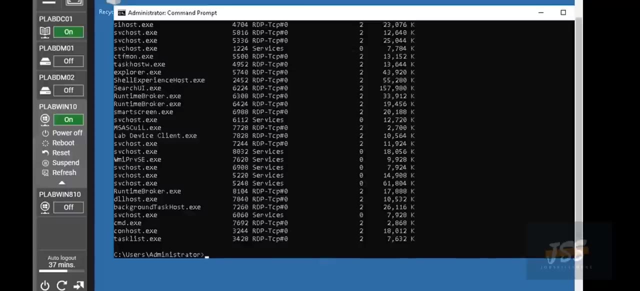 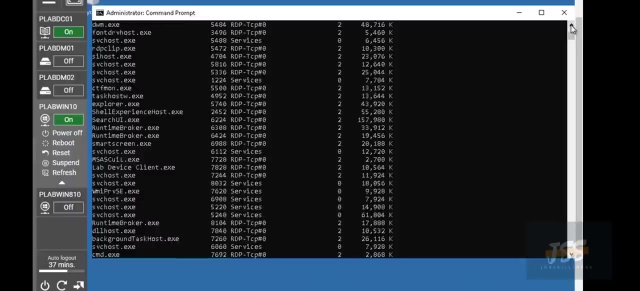 So here on the command from I'm going to show you. the first command of this video is the task list. So if you type task List and press enter, So you will see the list in that form And it It is a copy of what you have seen in the task manager, but there you can see that it is with the black background, the white text, totally. 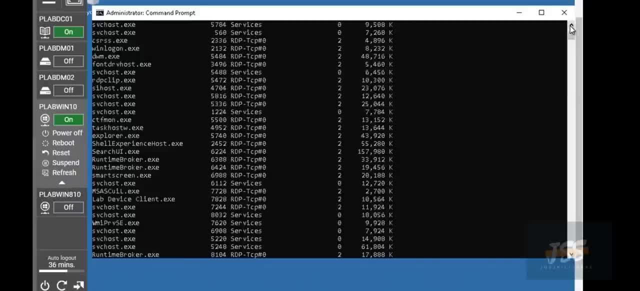 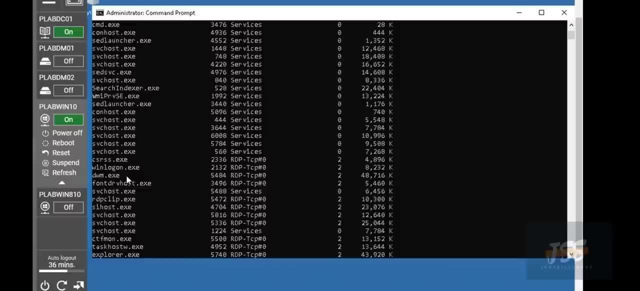 Traditional command line environment and here you can see there are a lot more services are running and all you can see here The extension is dot. XC means the files are right now running in the execution mode, because in your desktop You Always click to the executable file. 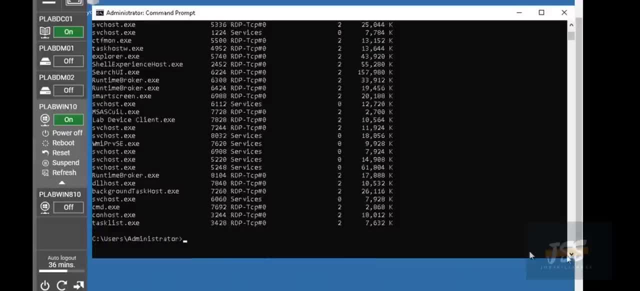 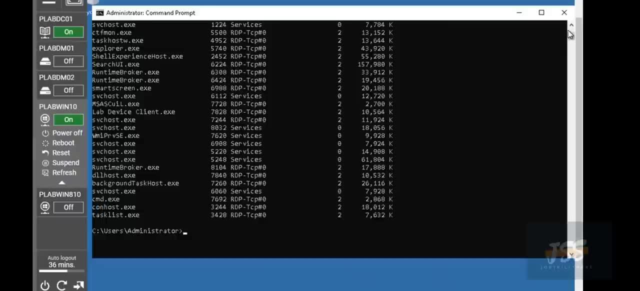 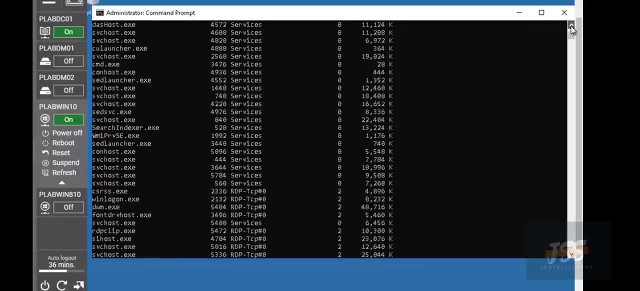 That's allow that application to run. And here you can see that we just opened this command prompt and it is also visible here in the task list. That means Another task is added. once you run this command prompt, this command prompt process is also added to your task list. 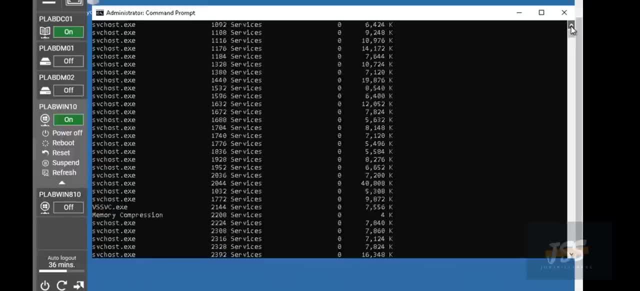 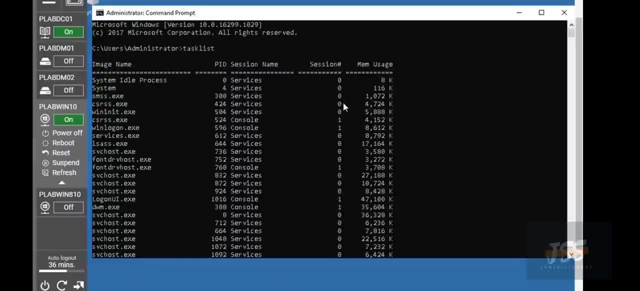 And if you scroll up to the top, So you Scroll up to the top, So you Scroll down to the top, so you will find The columns that will Actually need to know, before proceeding in this video, that the image name is what it is, the application name. but there is another thing called the PID. 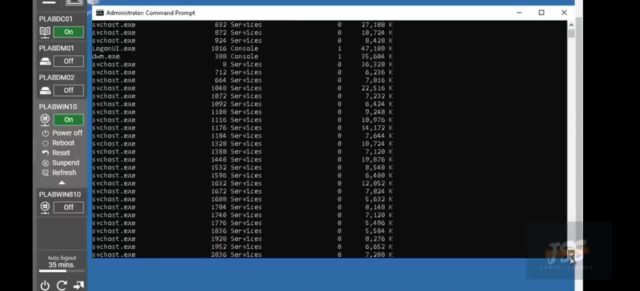 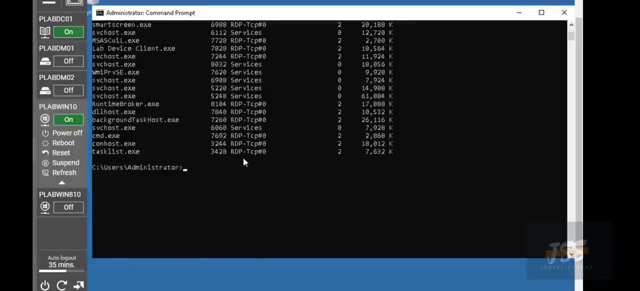 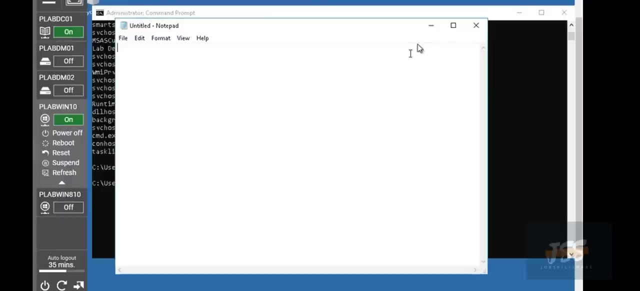 This is the ID we need to record when we want to terminate any service, Any test here. So let me show you What I Mean. you can easily terminate and stop any service. so let me open another application and make it clear to you. let's say, if i type notepad because i want to execute the notepad, so there you go, the notepad. 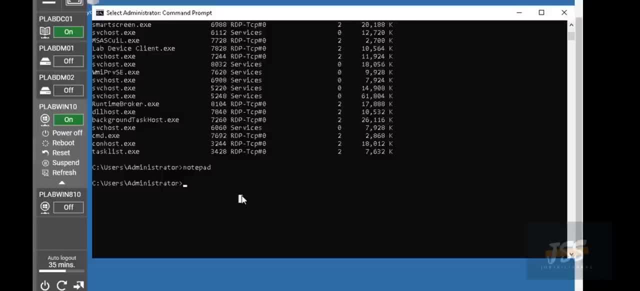 just appear on the screen and then if i run the test list. and one more thing for your help: that if you want to retype the command that you actually typed, so you can use the up cursor key to go back to the previous command that you use or execute it. so just type up cursor key and if 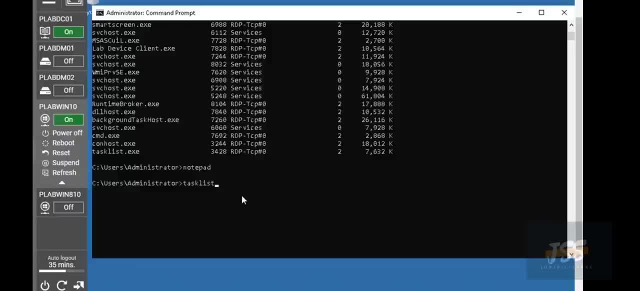 there's a lot of commands you already use in the single command line session, so you can easily do what. just use the up cursor key and the down cursor key and you can easily find out the previous command that you used. all right, so let me issue this command test list, and this time we're going to find the notepad. 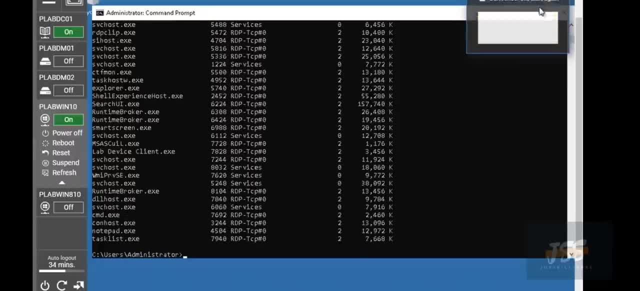 the part of the task. and there you go. the notepad is mentioned here. so what it means? it means that you run the notepad, you execute and it is added in the test list. now the thing is how to terminate and stop this notepad task with the help of command line. so we're going to type: 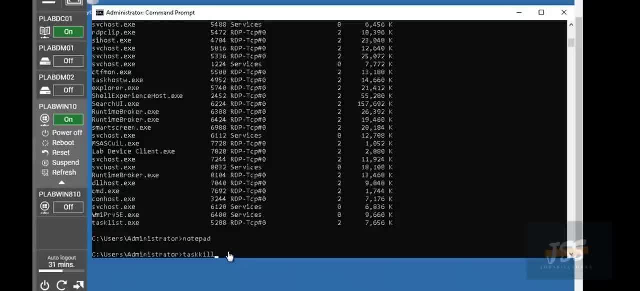 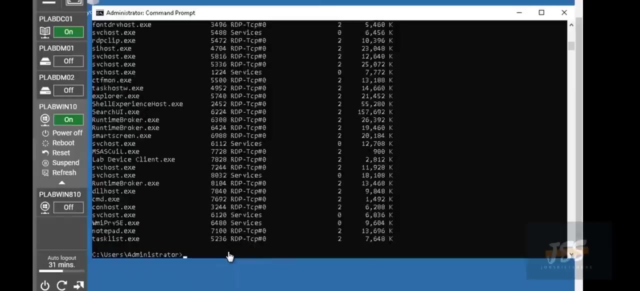 write tasks, kill, space forward, slash p id and need to notice that the notepad node, pad id is what. and if you didn't figure out the notepad by the id, so remove the command and then rerun the command test list and just make sure that you have the valid pid, in case, if you didn't have this valid pid, it won't stop that. 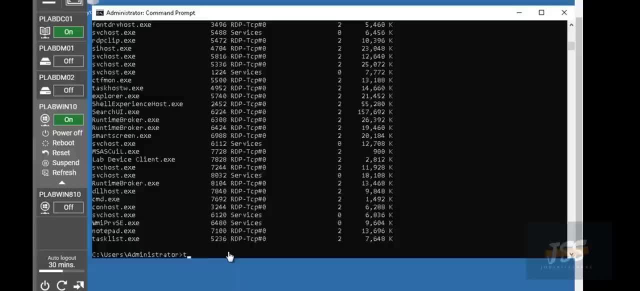 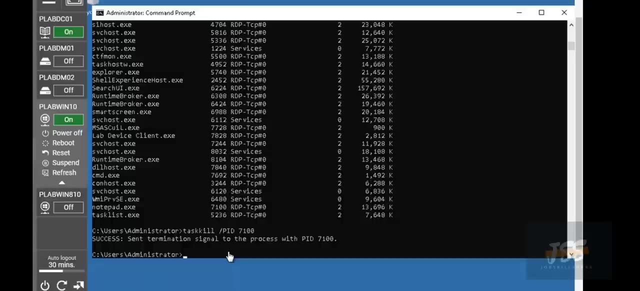 task. so then we're going to type task kill space, follow slash PID, and there you go, type the PID, and which is 7100 right now, press enter and there you go, you get the success message that tells that you have successfully stop and terminate that task. so we learn two commands: task list and the. 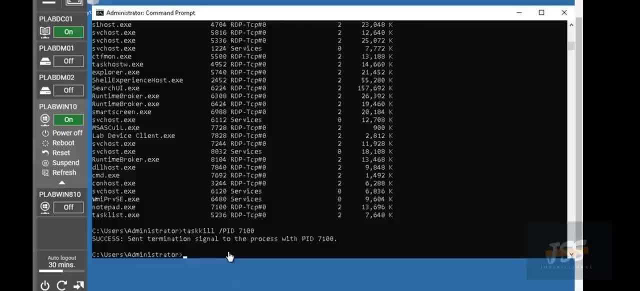 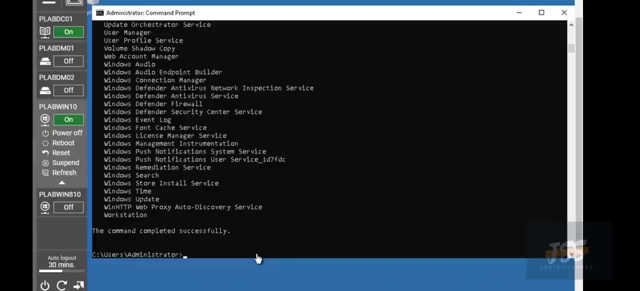 task kill to easily kill and stop any test that is running on right. then let's move to the service section. so there's a command: net start. if you type this command, so you will see all the working services that are running behind in the background of your desktop, of your operating system. so you 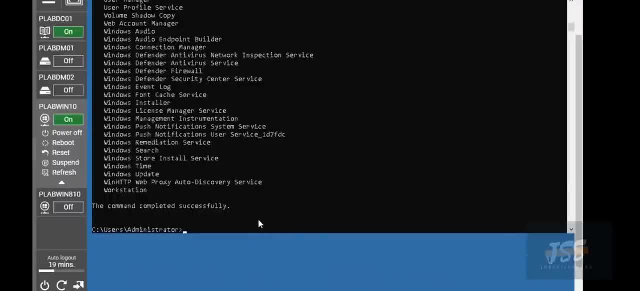 can see, there are a lot more services, and so let's stop any service, and for that we're going to type net, stop space, start then with a comma and type windows time. right now we're just doing this experiment, so we are stopping windows time service and then press enter, and here it is. 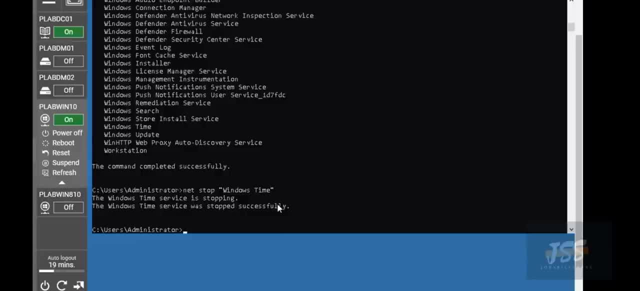 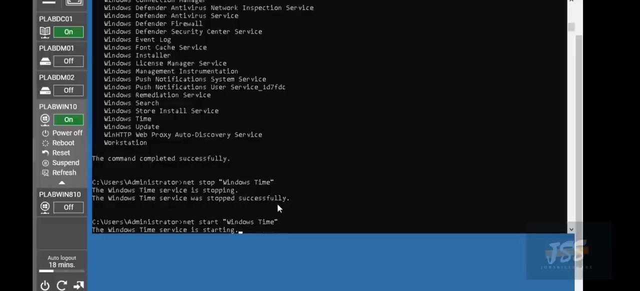 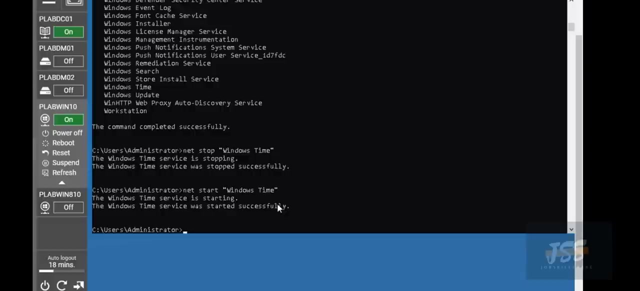 making a time and it is successfully stopped. and what if you want to restart this service? so you can change this keyword stop to start and then this service will restart immediately. so there you can see, let's stop windows time and it is successfully started. so this is about the services, how you can stop and start any service in your computer. 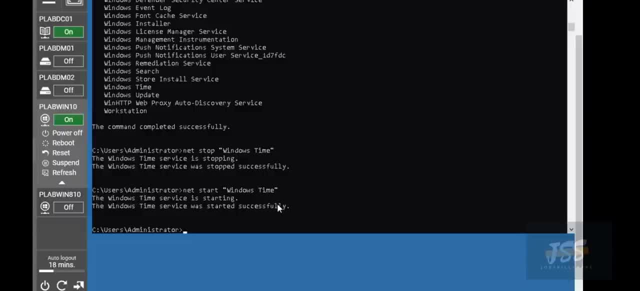 system. then the thing I need to share in the last is the driver query. there is another command, driver curiosity. so what? this command helps you if you want to know the driver set are installed. if work is finished, then you just need a quick click and just see what happens. it starts changing that. tab as always, and once again I want to just explain it to you, and a huge thank you to the work獲 teachers. thank you so much for watching till the end to our topic for today. two, two n? special cultureieux astonish nerdhelp工ώρα Для use of Arduino, and I'll leave you so. 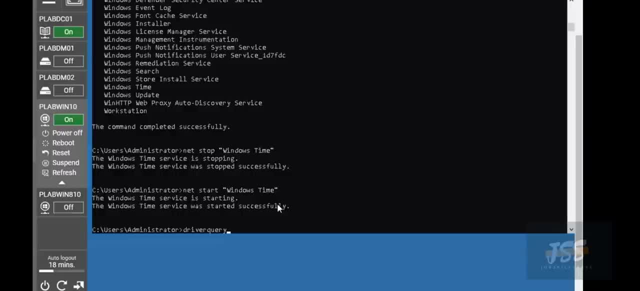 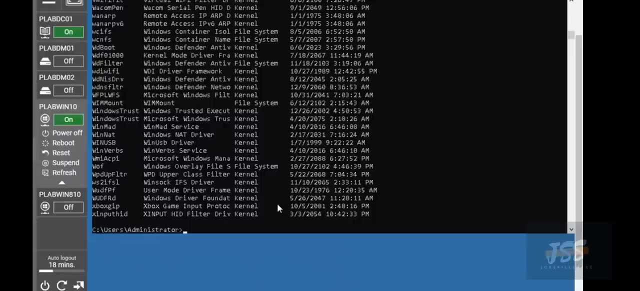 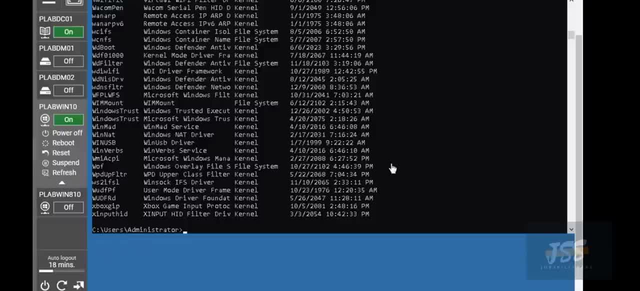 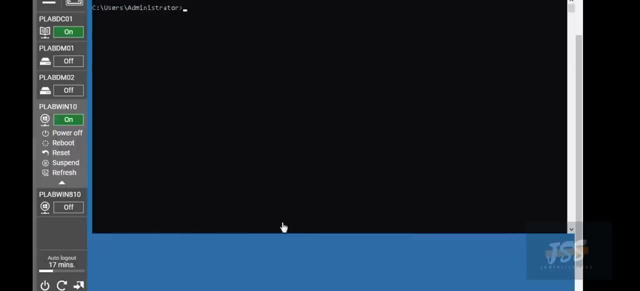 commands from task list, task kill, net start, net stop and driver query. and along with that, the last command, and really helpful, it's a CLS: clear the screen. if you want to clear the screen, just simply type CLS and it will clear all the stuff, all the text from your screen, and the one more. 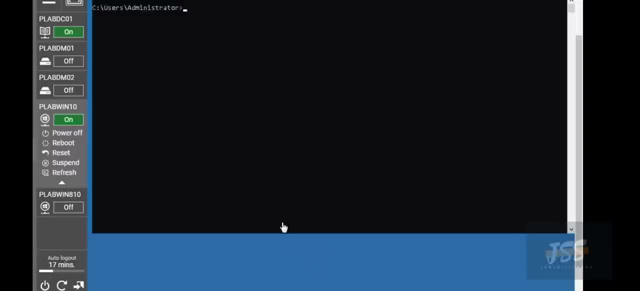 thing in the last, for the hint I need to prove, I want to provide you, is why we are using command prompt. because in the hacking side, in the ethical hacking, you will get the command line interface of your victim. so where you doesn't have the GUI based environment, all controls and all tests. 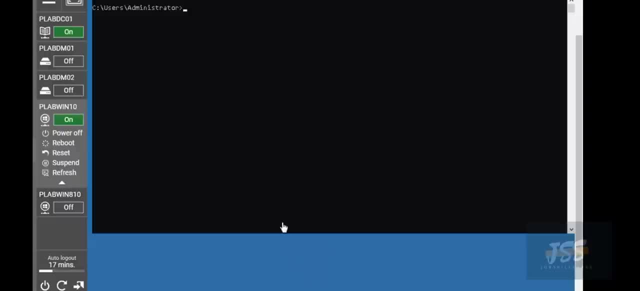 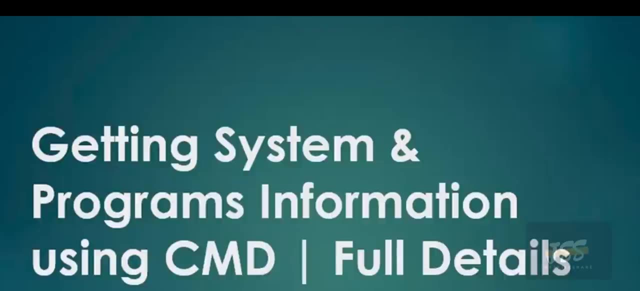 each and every activity if you want to perform on the victim machines, you have the command line and in this video we're going to discuss and I'm going to show you the basic commands to get system details and program information and definitely those commands really going to help you to getting the details of the 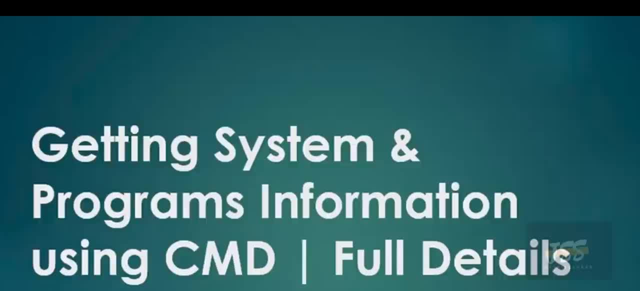 system. and also these commands are really helpful when it comes for the hacking. let's say, if you have any system, any machine and you want to see the details, so where you don't get this GUI method, this desktop screen, where these command are really going to help you and, moreover, these commands are also helpful to do things in a 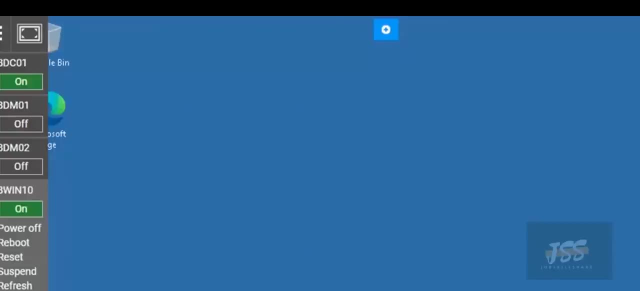 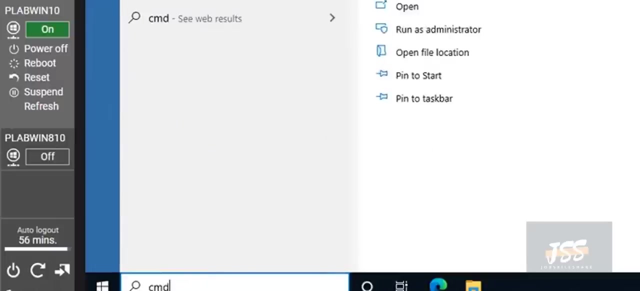 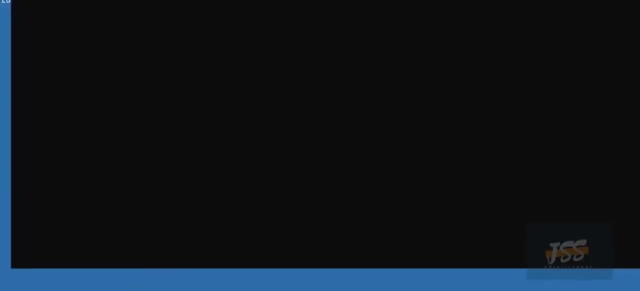 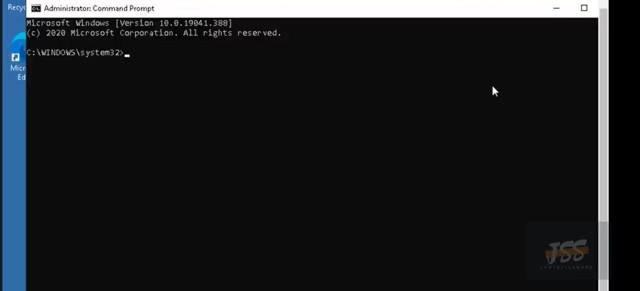 quick and a fast way. so let's go back to the desktop screen and here let's first launch the CMD from here. so what? I'm tapping CMD, then right click to run as the administrator and here just click yes to the yuck user account access control, your access control. so here in the command prom. 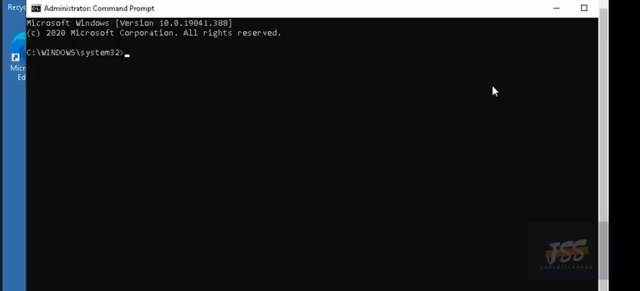 we're going to start the command with the command that gonna tell you. it will create a notepad file for you and it will analyze and detect all the softwares or the products that are installed on your machine. and after execution of this command, you will see all such details in. 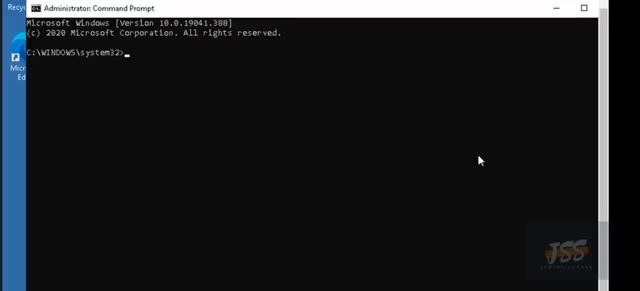 the separate notepad file. so let's start with the command. first we're going to type wmic and it's going to start another menu, another series, and here we're going to type forward slash output. then we're going to add column C. C would be the directory. you can change this directory as per your need. 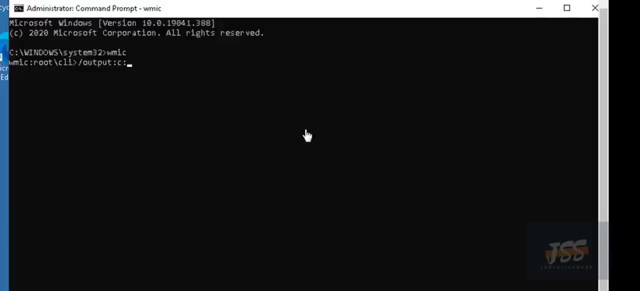 then put column- see column backslash, and then you have to type the file name. so I'm typing GSS, then add dot text, because in the command prompt you can only explode the text file, the notepad file. so you definitely have to put this extension just right after the file name and then after typing. 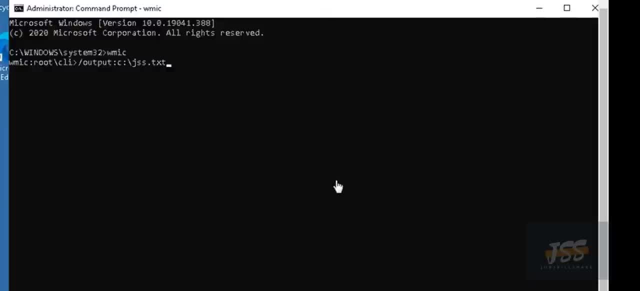 this detail you add. you need to add something with the in the end of the command because we need to know the products and the software. so we're going to type product, get name, comma, version, right. so when you press ENTER, it's gonna collect all the products name and the details of the software and then create a text. 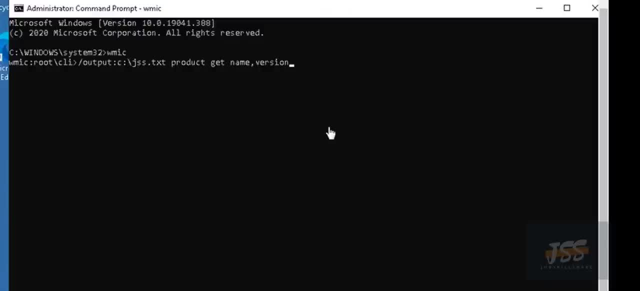 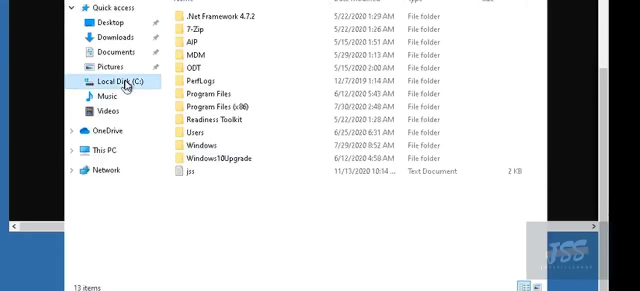 file and it will go to that location which you provided here. so let's press ENTER to execute and once you see the next prompt, then just go to that directory and check the file if- because if you go before returning back to the prompt, you won't find anything, because you will find the 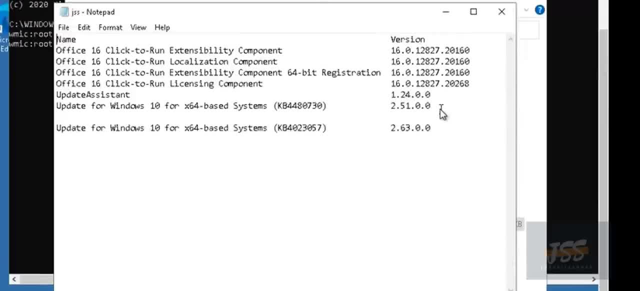 text file, but it doesn't contain any content. so just wait for the next prompt and then go to go to that directory and check this text file. so there you can see, because this is the practice labs machine, that's why it contain little program, some few products like 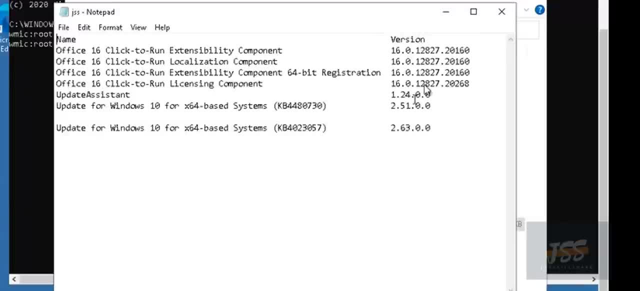 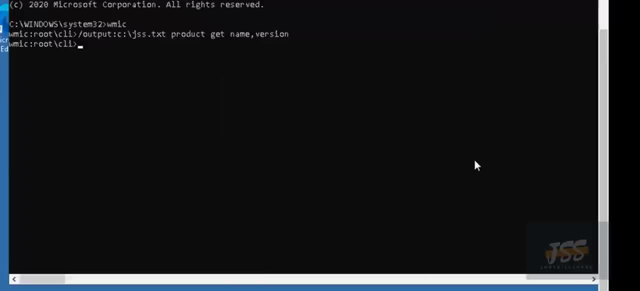 office 16 update assistant and the Windows 10 update. so this command really helpful when you need to collect product details and you want to collect some software details within your machine. now, within the same command, if you wanna know your CPU details, let's say you wanna know the core, the family of the processor and each and. 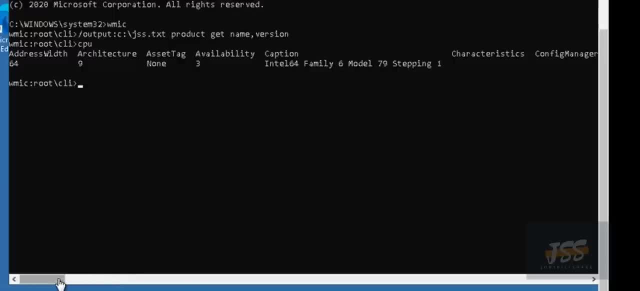 everything so you could type CPU. but when? when you type WMIC command, then it will take you to this prompt and then you can type CPU to collect the CPU details. what about your processor and how many cores and clock rate, and each and everything inside out you can easily find. 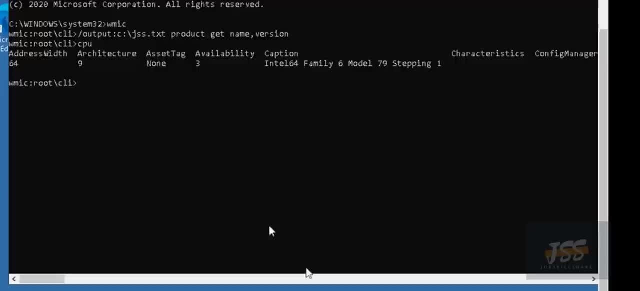 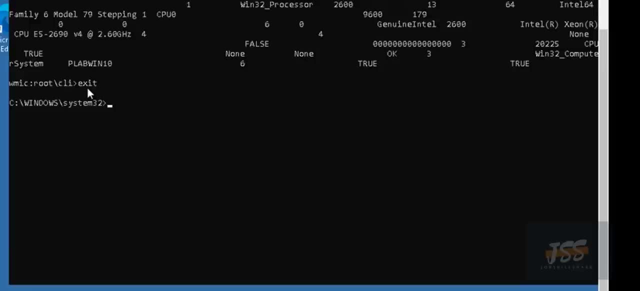 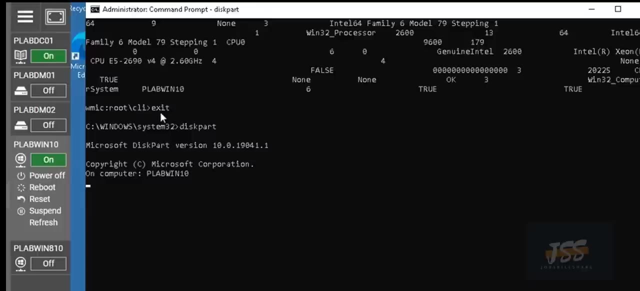 after typing the CPU command: now then we need to exit from this prompt. so we're going to type exit, enter and we return back to the normal command prompt and here we're gonna type this part and this command also change the prompt and here you can work out. on the disk you can find out. 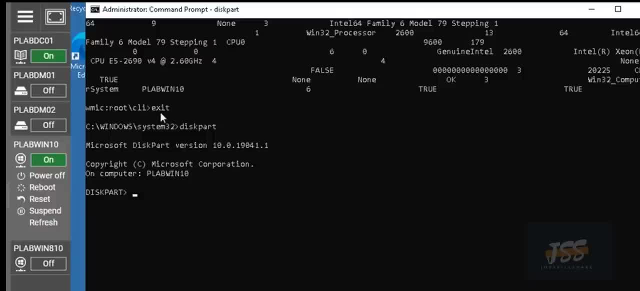 the details of your disk and this disk pod section will dedicate it. to know the details about your disk, to get the information about the disk, the number of disks that is currently installed in your machine, all you can gather and know from this disk pod section. so the first command, 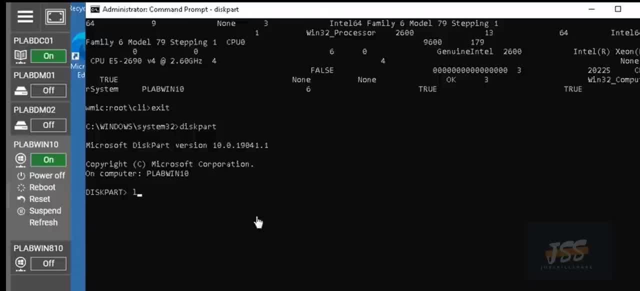 we're gonna type is LISTDISK. so L I S T LIST D I S K, LISTDISK. so first, once you type this command, this list disk command, you know, this command will inform you and it will provide the output about the number of disks that are currently installed. so you know, here you can see that you have this. 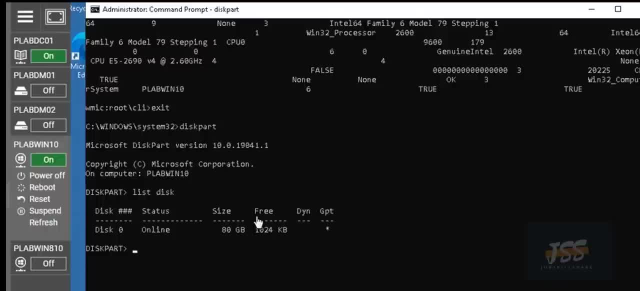 zero and status online. so you have only one disk. you see that is attached to your machine right now. so this is actually telling you that the physical disk in your machine is one. only one physical disk is attached now. if you want to further go to this disk menu, you would type select disk and the number. 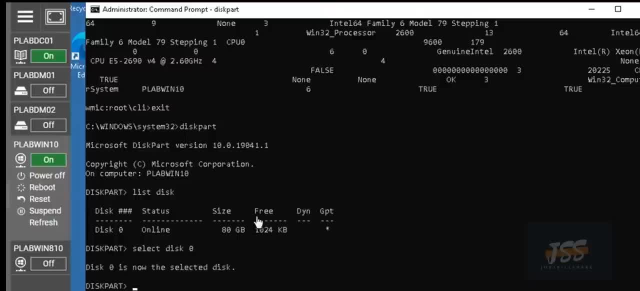 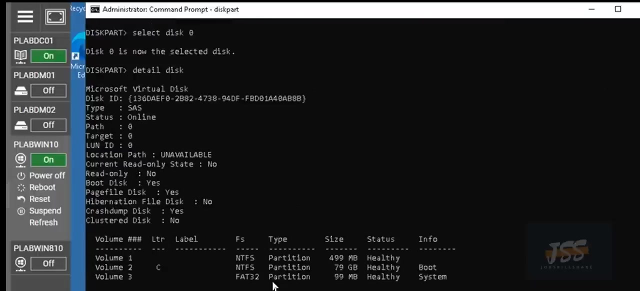 0. and there you go, you have a message that 0 is now selected and from here you can go further forward to get the details, like because we want to know the details of the disk. so the command is simple: detail, disk press, enter. so here you have these information, these details that tells that your single disks have three. 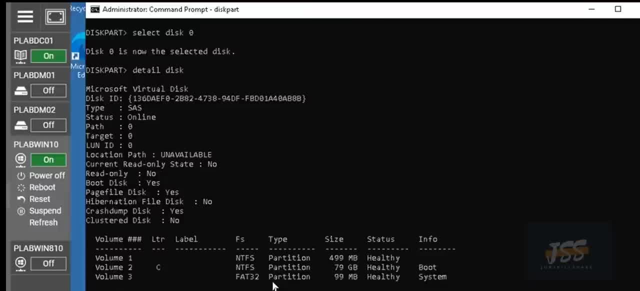 volume. first is for the recovery. second, third is a recovery. first is the basic normal volume. second is the 79 gigs. it's your C and you're also getting the label, the file system, the type it is mentioned, that partition and the info tells once is the boot. 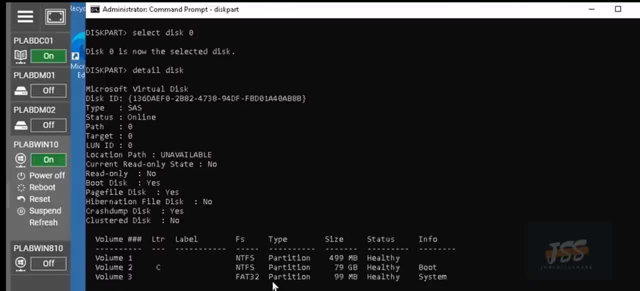 and under is the system. so this command is really helping you to know about the disk, because when you do these things with the graphical user interface you need to go on the computer management and that's then you select the disk management console to collect and gather these. 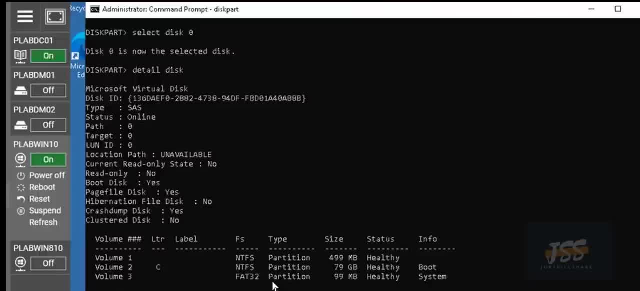 details. but here, with typing few keys, with pressing few keys, with few letters, you're getting these details without even moving your mouse and your cursor. so that's the benefit of the command line, the CMD. now to exit from the disk pod you're going to type: exit. 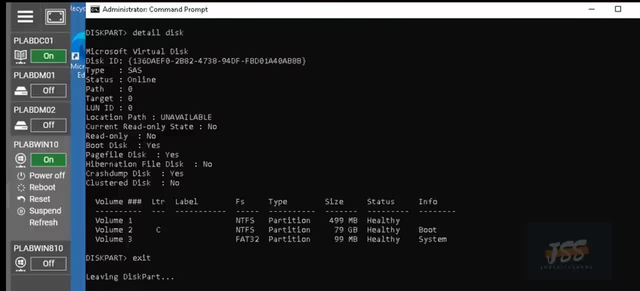 and it will take back you on the system 32, on the basic normal command prompt. now, then, there is another command related to the disk. it's a CHK DSK, the check disk, and and, as the name suggests, this command helps you to check the errors and the issues happening within. 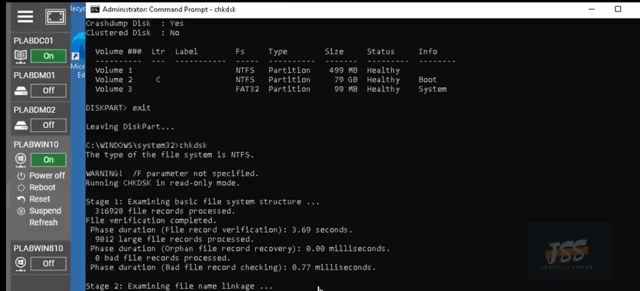 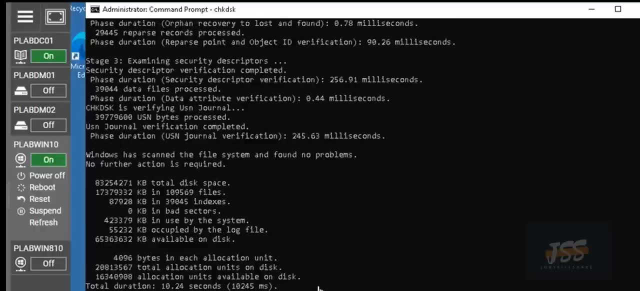 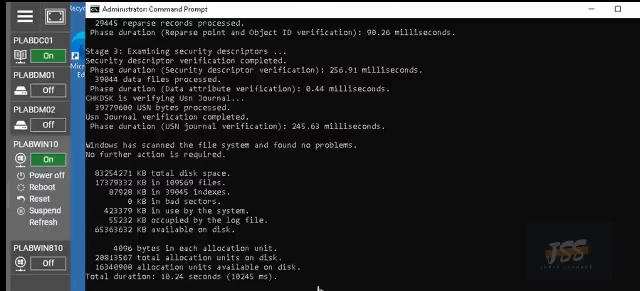 your system and once you execute this command, it will automatically start to scan errors and the bad sectors within your disk, because you know when you install and delete programs from your hard drive, you see there are some spaces got corrupted, because what happens when you download or install. 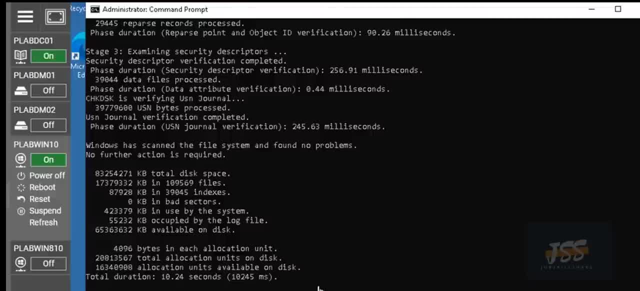 any file in your C drive and then you start to delete that area that is reserved for that particular application. that's written back to the free space when you're deleting that stuff. but what happens when you delete that stuff and it doesn't get done correctly, by means that it doesn't delete perfectly in a correct way? so this: 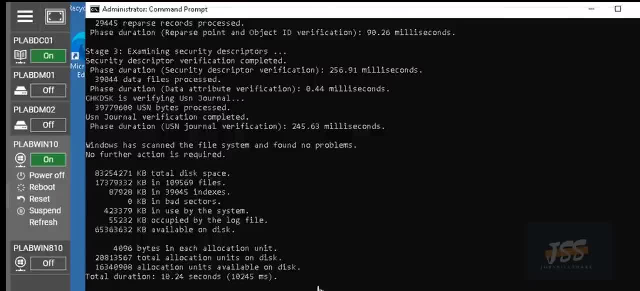 area become bad sector because this area enabled to change with the free space. that's why these parameters, when become in numbers, it will impact your disk, it will start making issues with your disk speed and other sort of things, and you will see and you will find out that your disk is full. 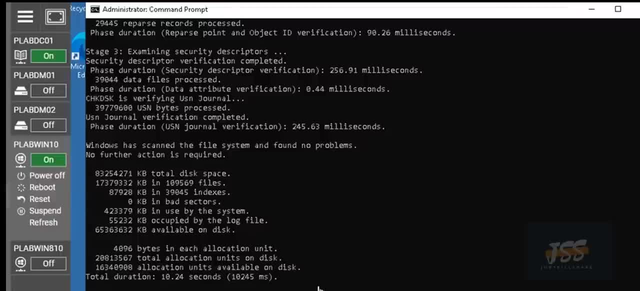 without any data. so at that moment, if you use this CHK DSK command, so it will provide you all details and then you could easily repair your disk by adding some arguments against the command CHK DSK, C column, and then you could put any of the argument like R, so it will start recovering your 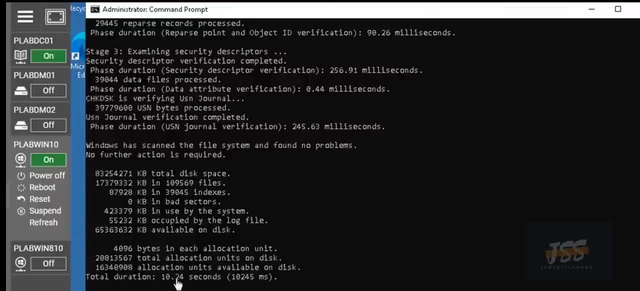 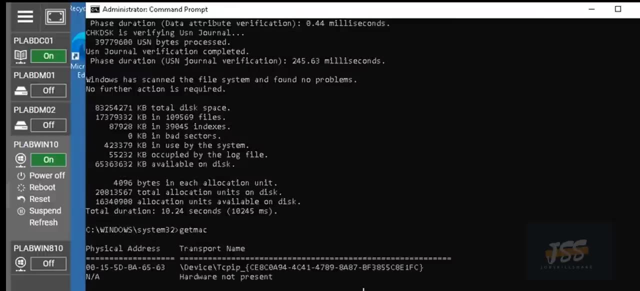 disk, but right now we don't want to recover over this. so you can use this argument. then, if you want to know the Mac address of your machine, so we have a simple command: get Mac and if you type so you will get the physical address of your machine. let's say there is a 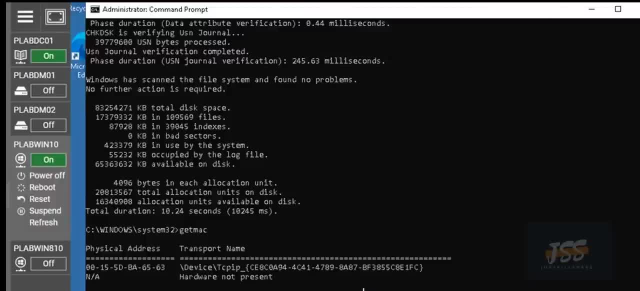 connection and you're working, or you have a home router and you want to make some restriction to your machine, that this router will connect to that machine, right? so you see, in that situation you must know your physical address and if you want to know the physical address in a glance, in an instant, so 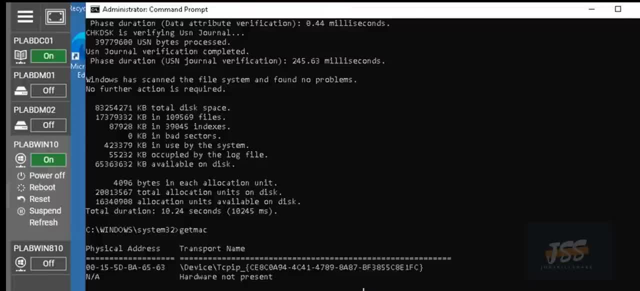 just go to the cmd and type get Mac, because when you want to check this Mac address through the GUI method, you need to open different sort of dialog box boxes and you need to go on different windows and they it required a lot of clicks, but here it. 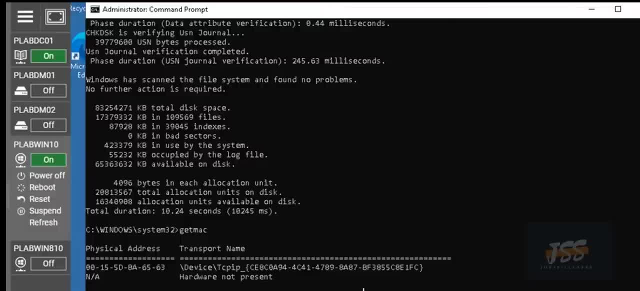 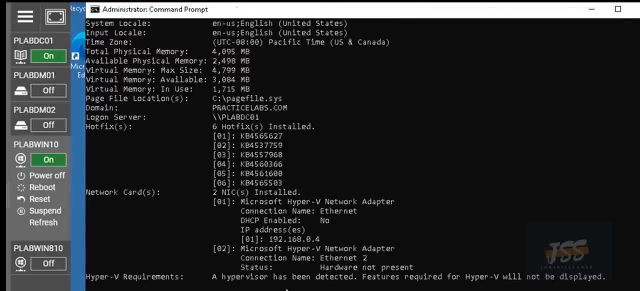 required only your pressing of the keys and you will get your details then. after that, if you want to know the whole system, details like what drivers are working, what is a network situation, what is your IP? what, what? what about your network card, your RAM, your other sort of stuff related to your 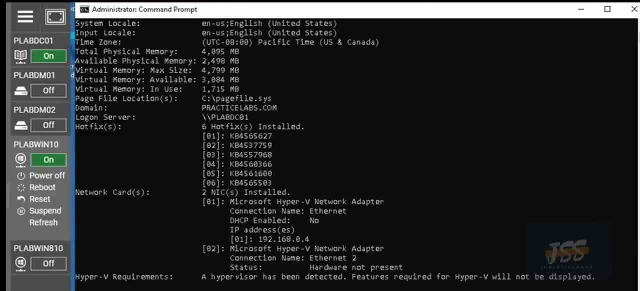 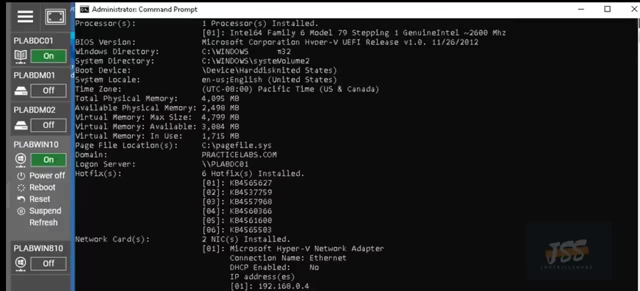 system. so the command you're going to use use, is the system info and here you can see. the output is there. the network card number are two. two cards are attached at the moment. one is a hyper-v network, second one is a hyper-v network. both are the hyper-v and there is a availability of hypervisor also. you're getting some other. 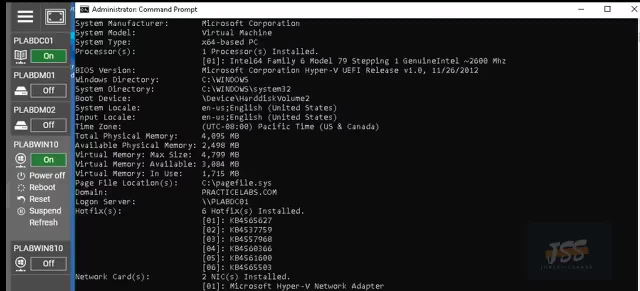 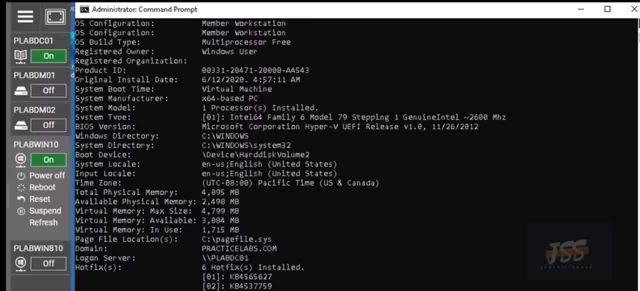 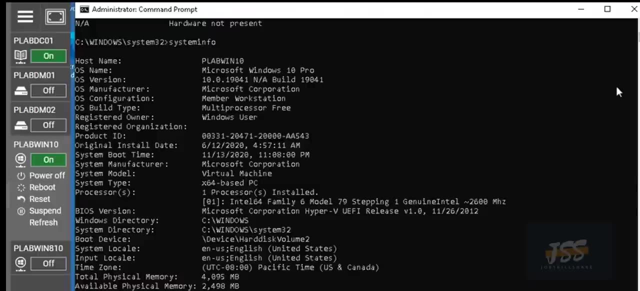 details like where's your system, which is your windows drive right, and then what is your ram and how much ram has been used, and the machine name and the workstation and the windows version, the os details. so you're getting plenty of the details that you need to know in fixing things. 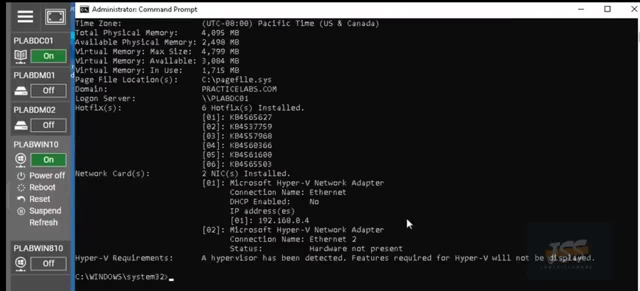 and in dealing with the system issues. so you can easily get those details by typing this system info command. then in the last, just similar to this command, but this command is used to know about the drive and the output are the same, so you can see the same thing as that in the oldfile. 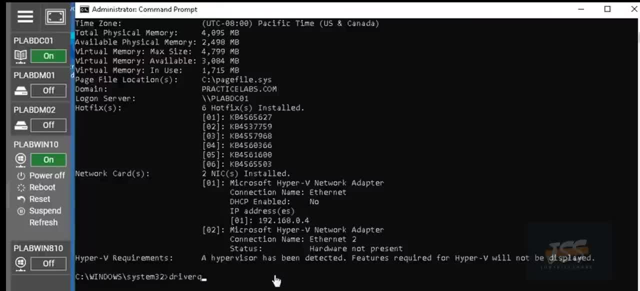 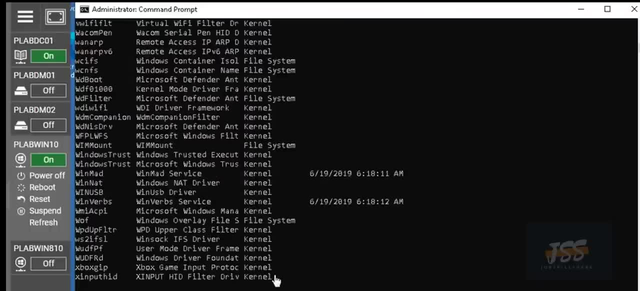 details. so if you want to know how many drivers you have and which driver you need to add, because there are certain features and certain programs and mostly with the games- some games are quite some high updated drivers and you want to know that, which driver you need to install and add in your machine so you 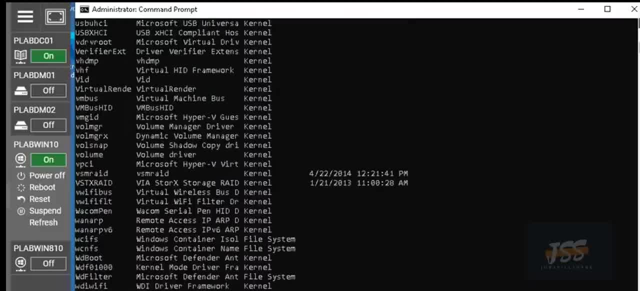 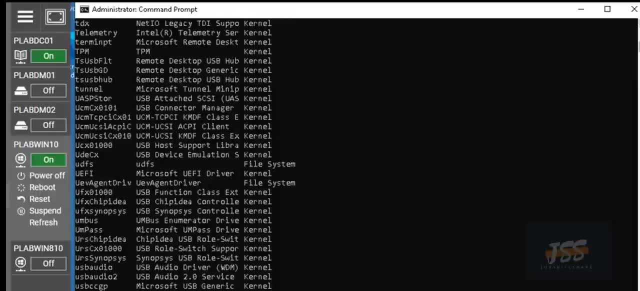 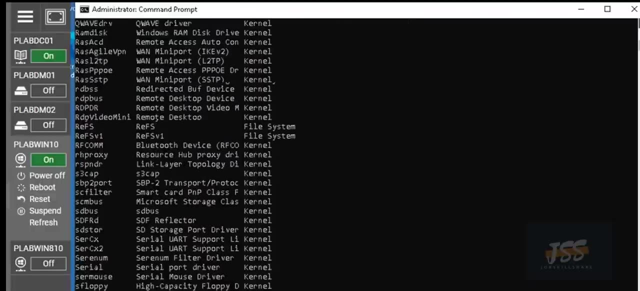 could type this driver query so it can tell you and it will provide you the output with all the details of the driver that are currently working and installed in your machine and this is too much details to verify and troubleshoot your driver related issue. and if you are not getting that driver, 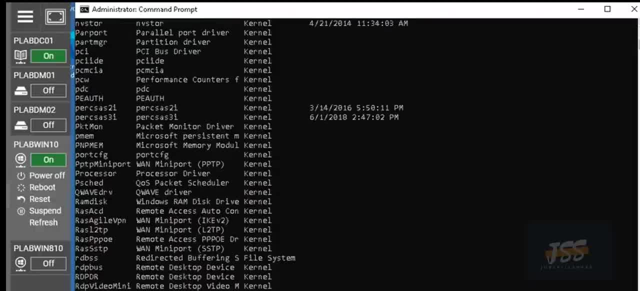 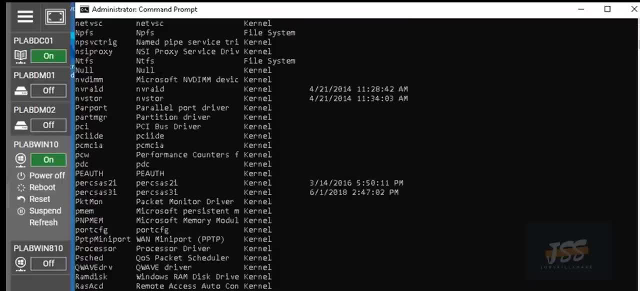 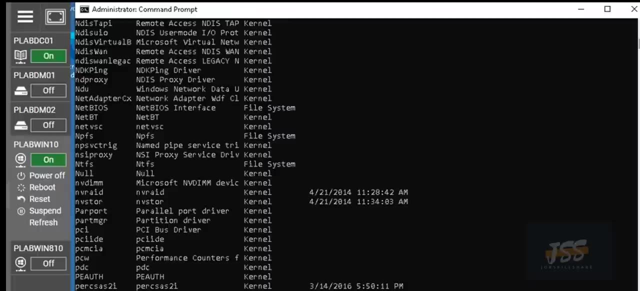 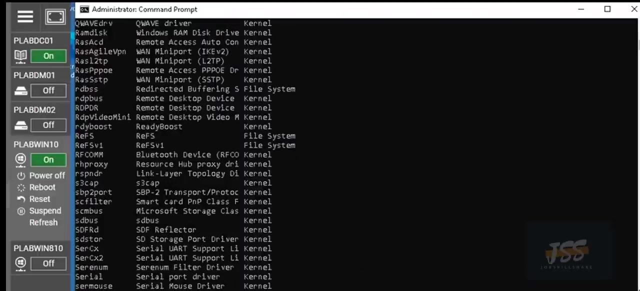 installed. so definitely before fixing other issues you must install the driver and 50 and 60 percent chance that your issue would be resolved. so you need to know that these came in. and most important thing that I want to add here, that if you are familiar and perfect and good at command line, so you could easily work on the 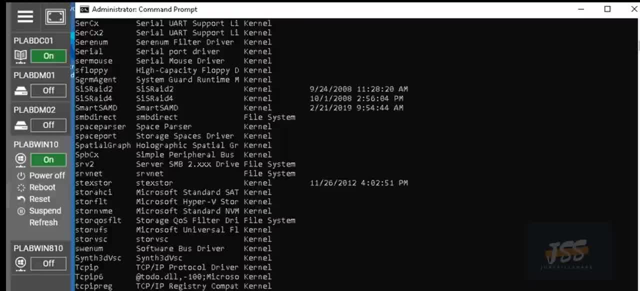 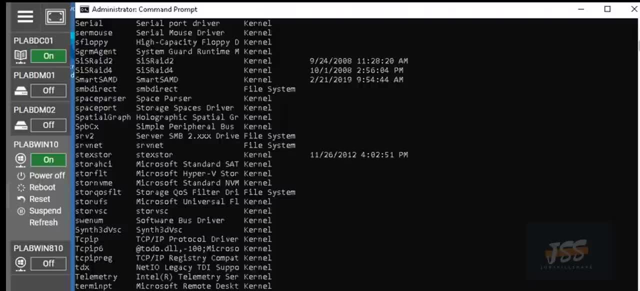 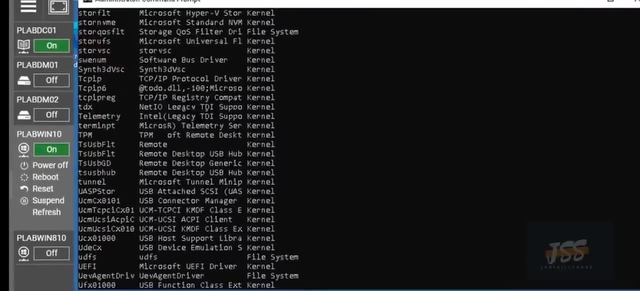 PowerShell also, you could easily work on the server core product and also if you have any interest in hacking and if you know about the ethical hacking and you know how to get the remote session of any machine by doing some hacks, so the command line skill really gonna help you, because there you only find the 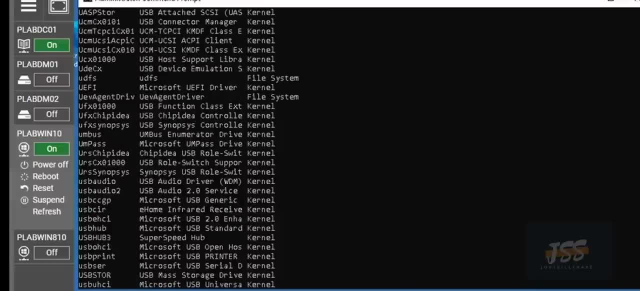 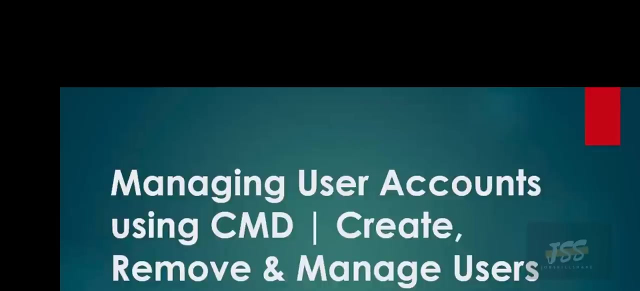 command line, the black screen with the white text. so it definitely helpful for you to go in that machine and check the details and transfer file from here to there. so this command line skills really help you to easily work on any remote machine. I'm going to tell you the six command so you can manage your user or 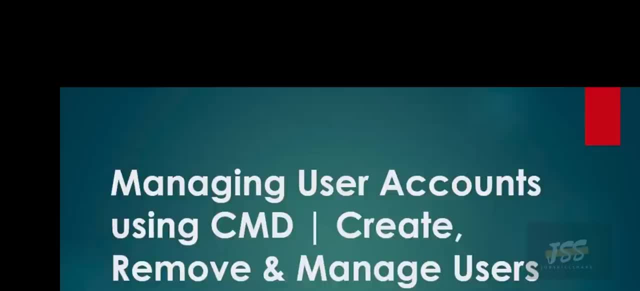 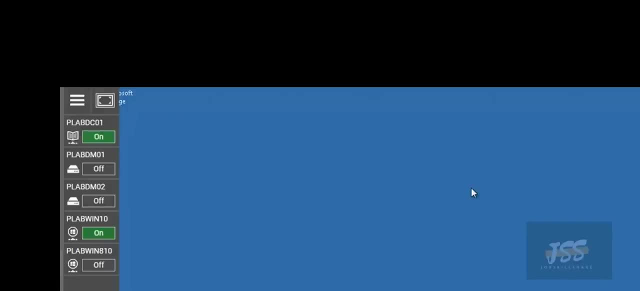 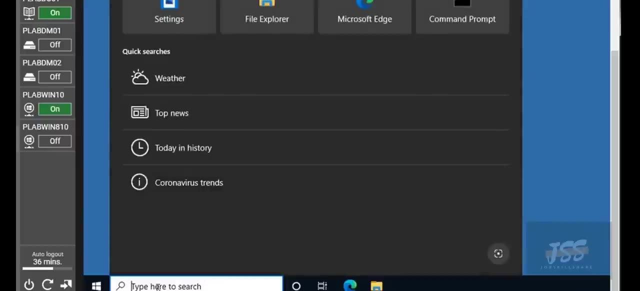 remove and you can create password. even you can know how many users you have in your machine. so let's start with this practice labs machine. so first let me tell you another command to check the users on the graphical user interface, so you can acknowledge all the users and all the account settings. so what's the 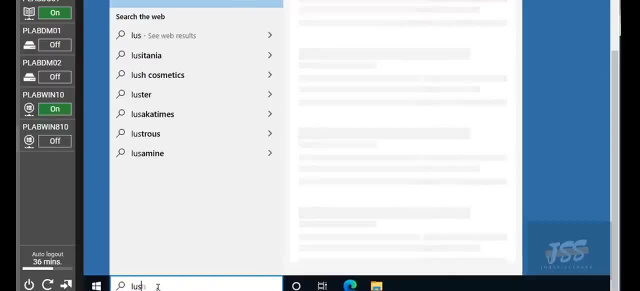 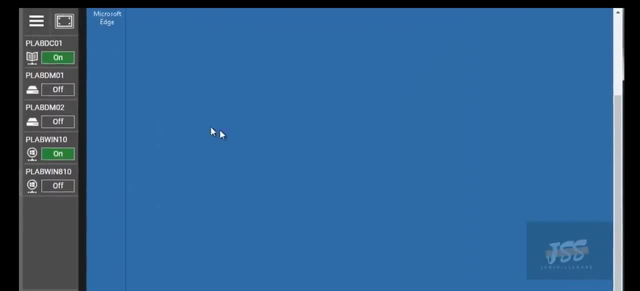 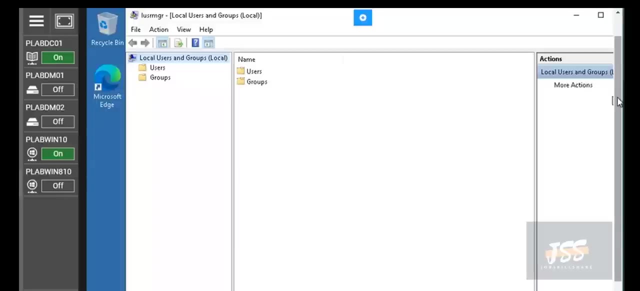 command is L user, you as our MGR dot MSC, and if you type this on run or here, type here to search, so you will find this user console. and if you want to go on that window, that manager, user manager, so you need to go with the computer management and then you're. 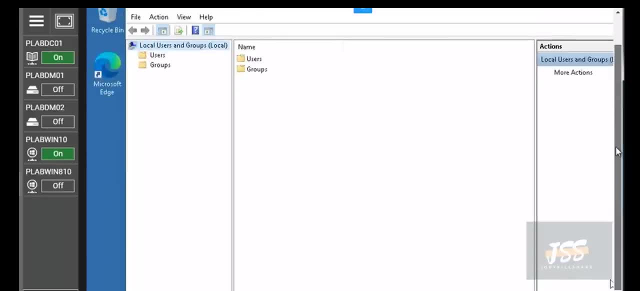 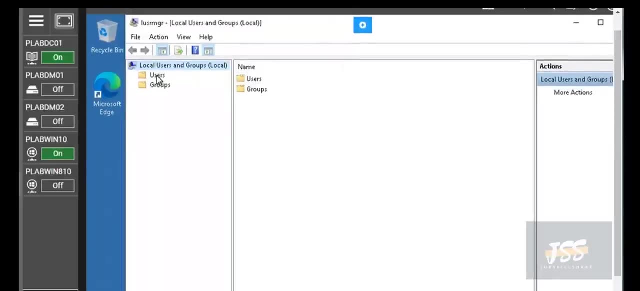 going to select the user section, but with the help of this L user, MGR dot MSC, you will directly get into this user manager console and if you click on the click to the user, so you will see the details of the user. so this is what the 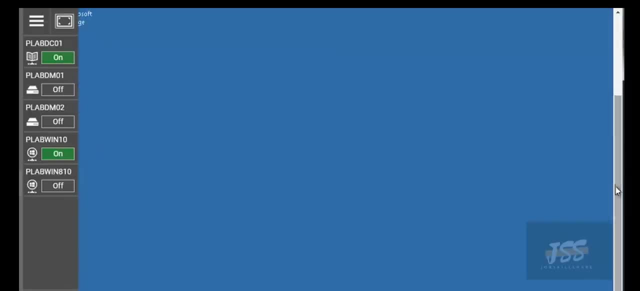 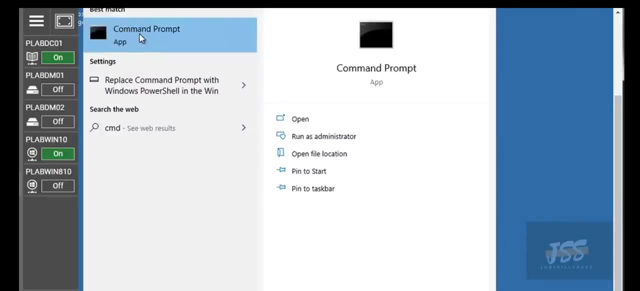 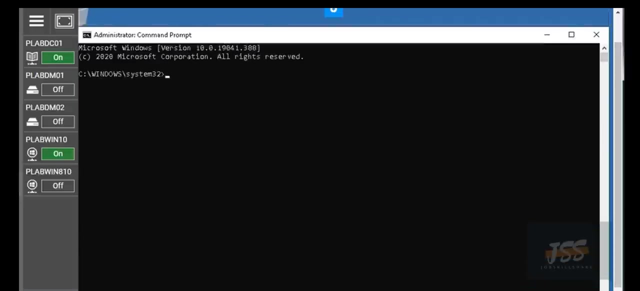 graphical user interface to check your user right now. here we're going to check those things with the CMD, so what I'm doing is just typing CMD and I'm gonna execute it with the administrator privilege now here. now the first command is what? how to check the users, that, how many users you have in the same machine. 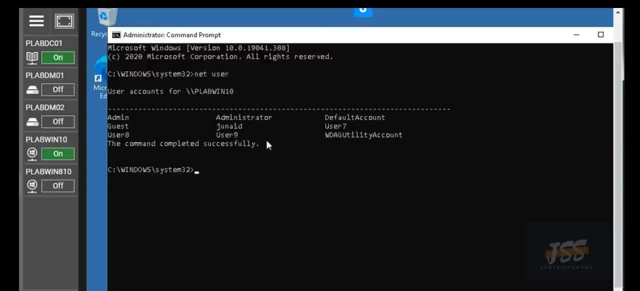 so the command you're going to use is net user and press enter. so here you can see. there are three columns here. that these three columns tells you all the users you have in this physical machine, not the domain user right now. so here you have: admin, guest, administrator, donate user 9, default account user 7 and 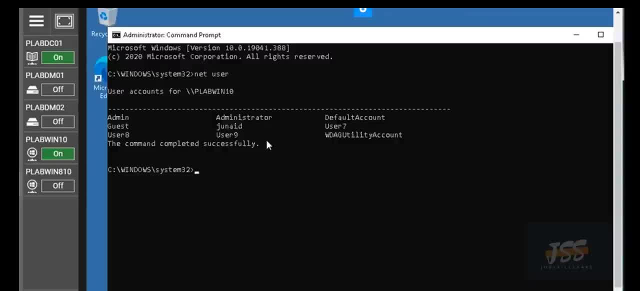 some system accounts. now, if you want to make a user account, if you're going to create a user account, so what is the command you're going to use? is net space user? then type the username, the exact name on which you're going to create the user account. so let's say I'm going to 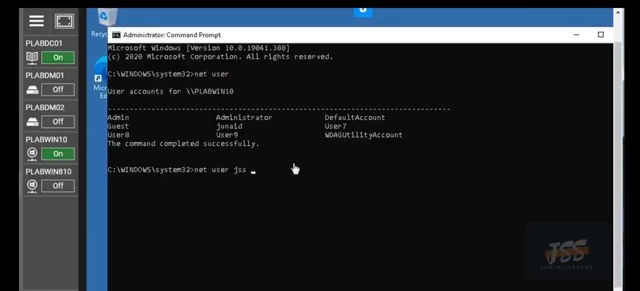 name it JSS. after space, put forward slash, add and the exact password you're going to use. so I'm making it the password P A, double S, W, zero, R, D, enter. the command is executed successfully and you can check this user account simply by the two ways. first, you can run net user command so it can tell you that. 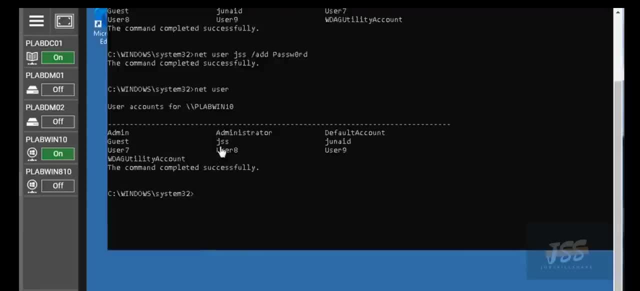 you have this new user and right, we have this JSS user. right now under the administrator it tells the account is created successfully- then if you want to delete your any of user accounts, so you have the list on top and you can select any of them and you will type net space user. 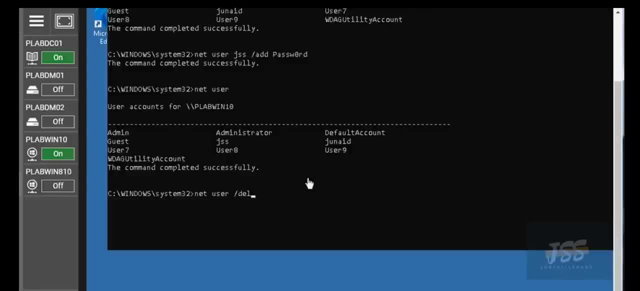 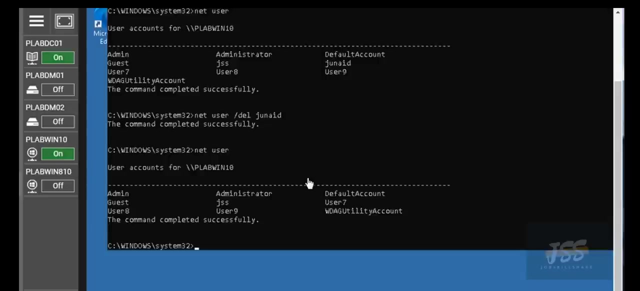 and then we're going to put this specific keyword is Dell, Dell is space, and we're going to delete this Junaid account. J U N A, I, D. enter so it is deleted successfully. and let us verify now. there you go: the account is deleted and it is not in the list right now, so the account is created successfully then. 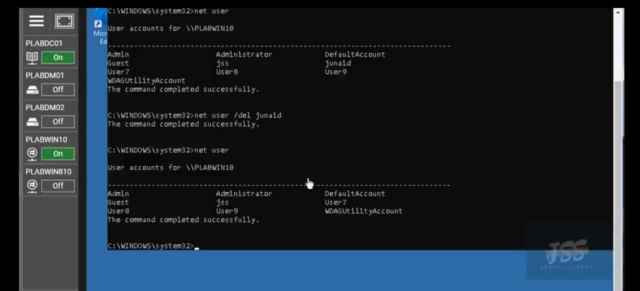 we set the password along with that, and then we learn how to delete any user account by using the CMD. now, then, sometimes in Windows 8 and Windows 10, or might be in Windows 7, the administrator account disabled by default. and if you want to check this thing, if you go to this user manager and right click on the 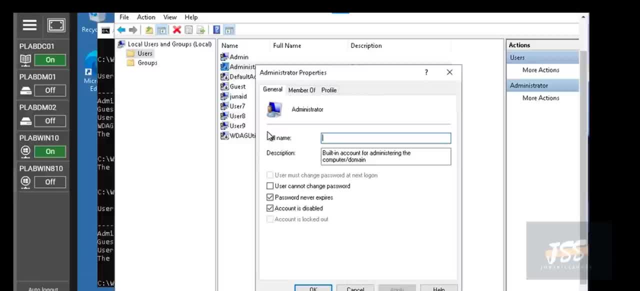 administrator and go to the properties. so often you find, check on this option, account is disabled. so mostly the local administrator is disabled by default in Windows 10 and Windows 8. so what we does all the time if we want to enable this account we just removed. 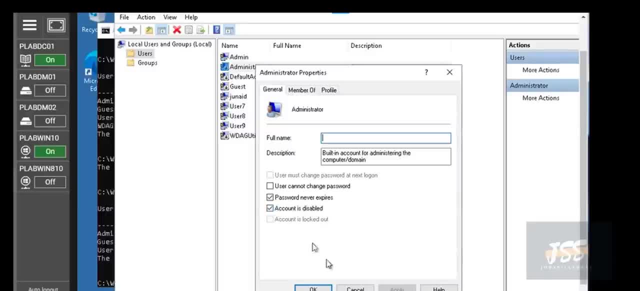 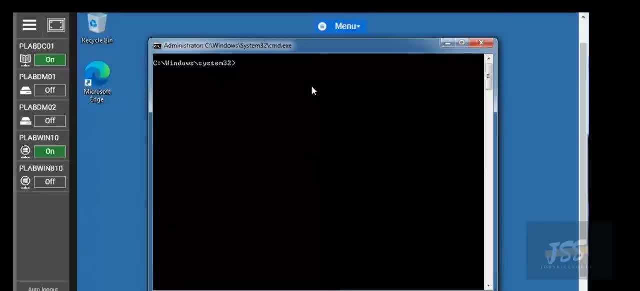 the check by using this user manager console, but how we can do this action with the CMD. now let's look into the next command and that is to enable administrator account that I already show you. sometime this account get disabled and I showed this thing in the beginning, so the command is net user. 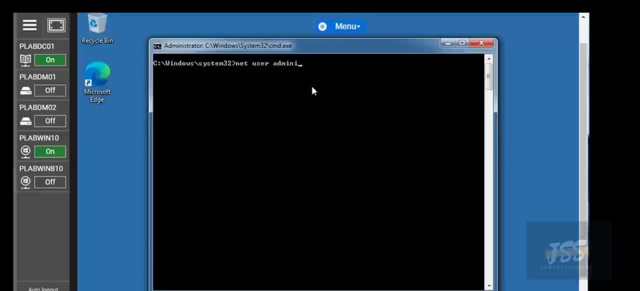 space- administrator space forward slash active column. yes, so it can enable the administrator account and, the same way, if you want to disable that account, you could use no and it will disable your administrator account. if you don't want to change your password and just make your account simple, click to login. 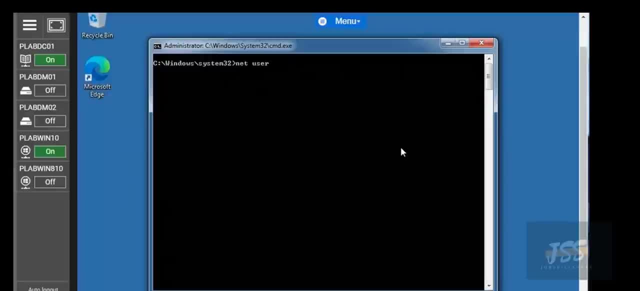 so you're gonna use the command that user space, the user name, put the double inverted commas. let's say I'm going to change my administrator as a passwordless account, so I'm gonna type steric, and here I'm not pressing any key for the password, just pressing enter and the command is successful. 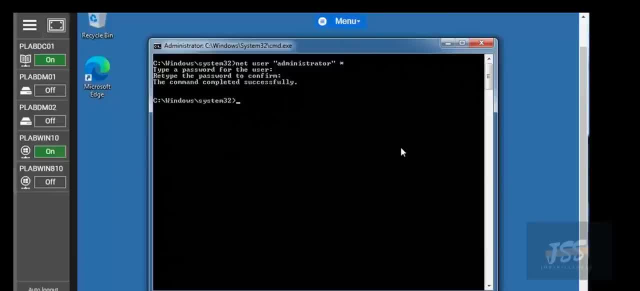 now you can easily log in with your administrator account without the need of password, and so that's all about this CMD video, and in this video you have seen we've covered six different commands that you you could use for managing your user account: your password settings to delete your 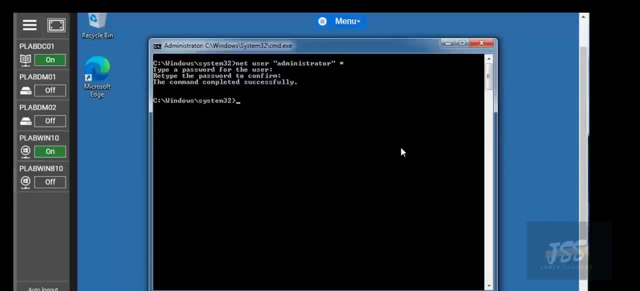 user account and all these commands really help you when you only have the command line mode, and mostly in the server core product, or while you're doing hacking and you got the remote controls of any system so you could easily manage things by using the CMD. I'm going to tell you some commands that you can use to hide your. 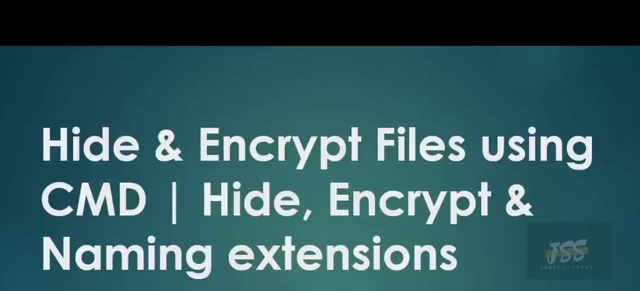 files and encrypt your file by typing some commands. and why I'm telling you these commands? because there are other ways to hide your file by using GUI. but there are certain other ways and techniques to show those files and if I show you in this thought, so you could understand what I'm. 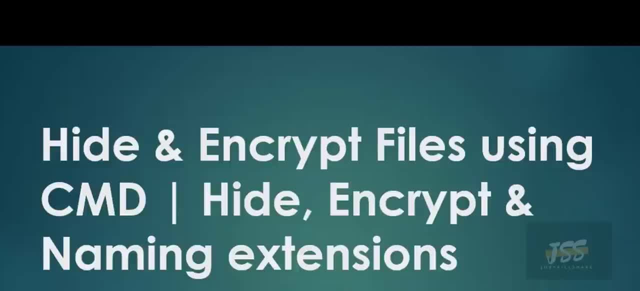 talking about. but with this commands you can easily hide your file and nobody can access your file until you type another command to show all those files. so let's start this video with the GUI interaction. then we will move to the command line. so here on this Windows 10 machine, let me show. 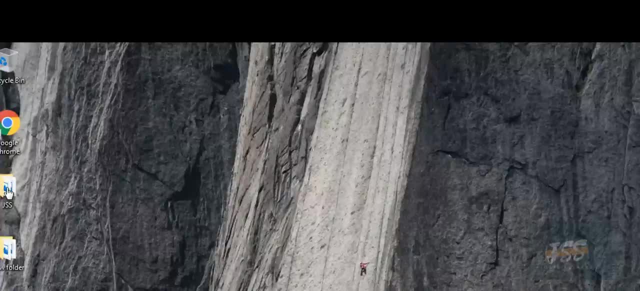 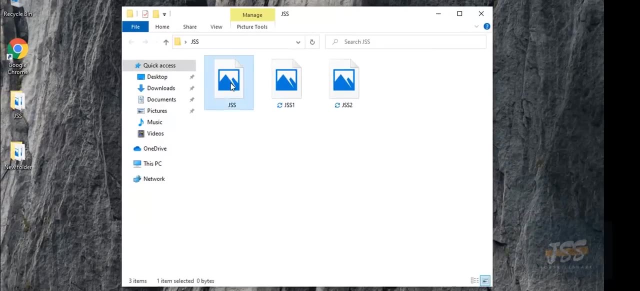 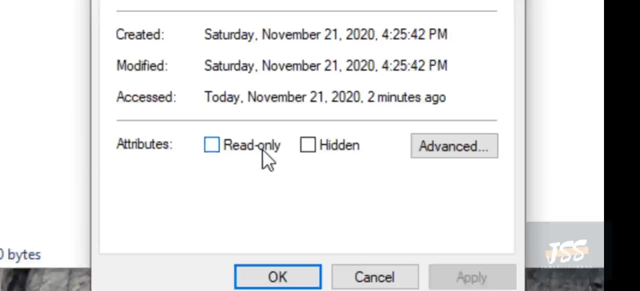 you how you can hide your file by using the GUI methods and how you can easily access those file after hiding. so this is a GSS folder and if I right-click on that file and go to the properties and in the last section against the attributes, you will find the read-only and hidden. if you make check on the 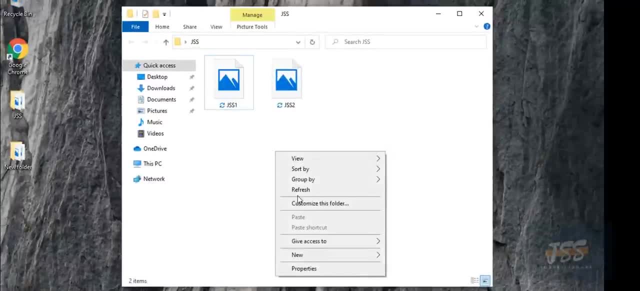 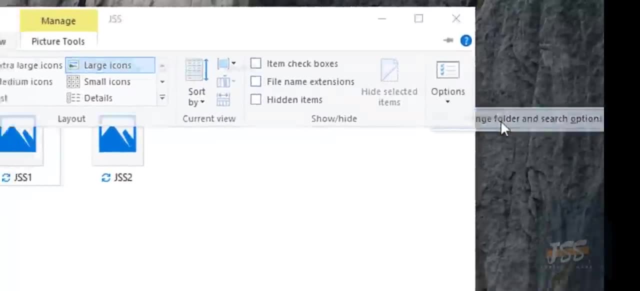 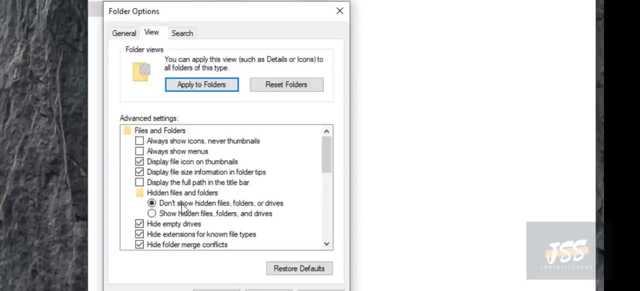 hidden, so this file will hide and you no longer access this file. you no longer see this file. but if anybody knows how to see the hidden file, so he or she, that guy, can easily go to the folder options, switch to the View tab and make check on. 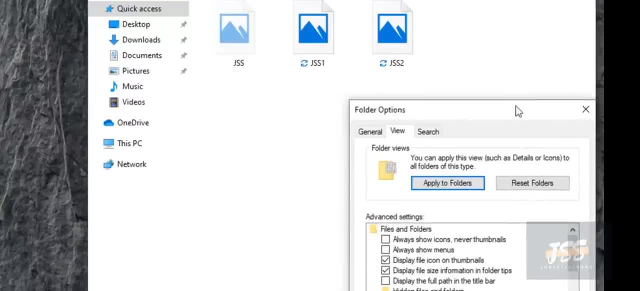 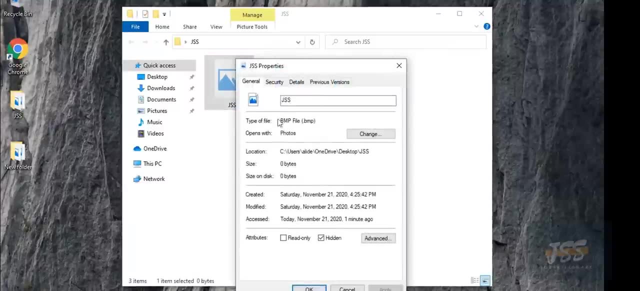 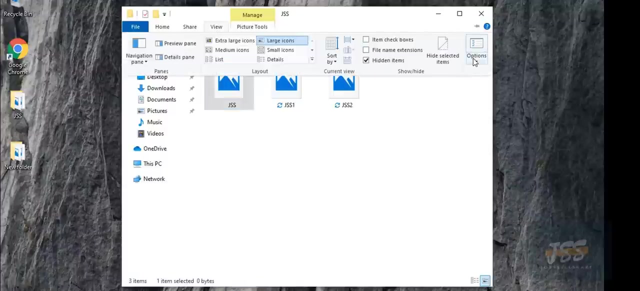 show hidden files. and then there you go, the file is there to access. so this thing are not helping in hiding the file in the way you want to hide. so just show the file and remove the check and make the settings defaults so you see the View tab. don't hide, don't. 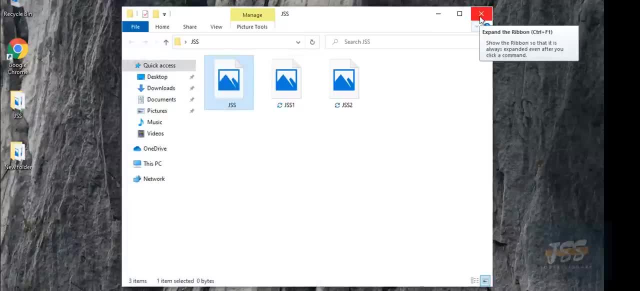 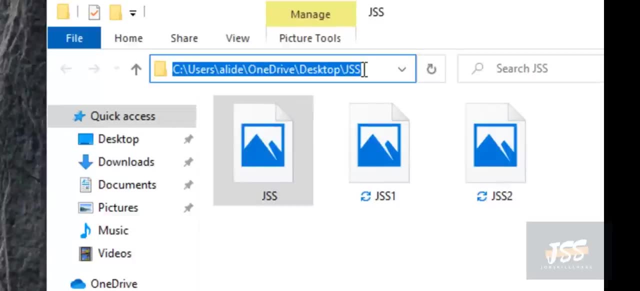 show this in files. so let's move to the command prompt and just do some wonders in the command and hide those files totally, and it can only be visible once you type the command again. so I'm going to learn the CMD and why I'm typing here. 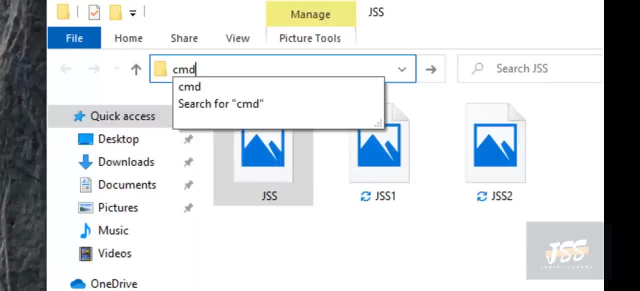 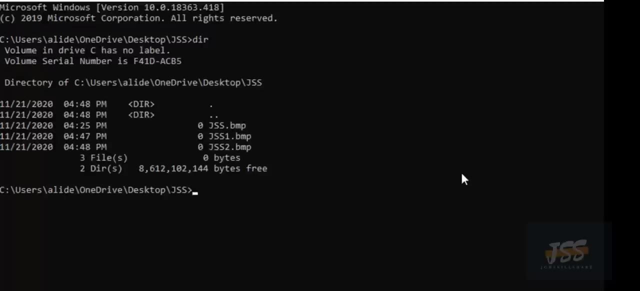 on the address bar of G of this GSS, because when I'm launching the CMD from this GSS folder it's gonna open the debt GSS prompt so it will locate this prompt on the jss folder. so if i first run the command dir, so there are three files. we have now the 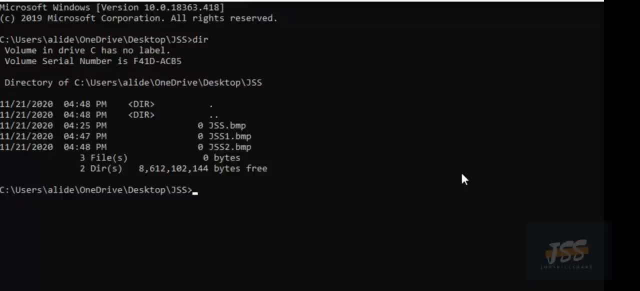 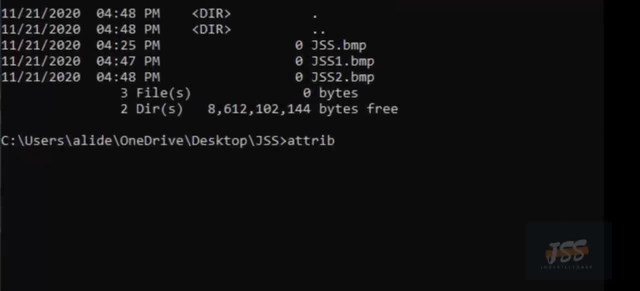 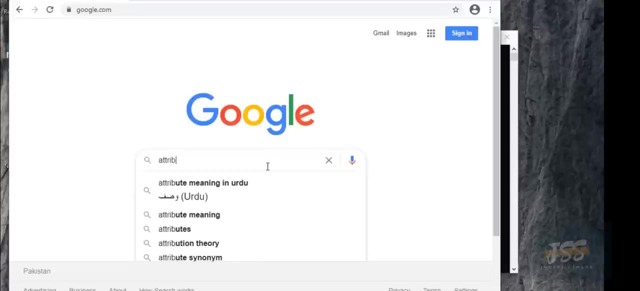 command we're going to use to hide those files is a double t atrip attribute. full form is attribute and you can search this attribute here in the google. you will further get know about the file attribute command if you type that and press enter, so you will get plenty. 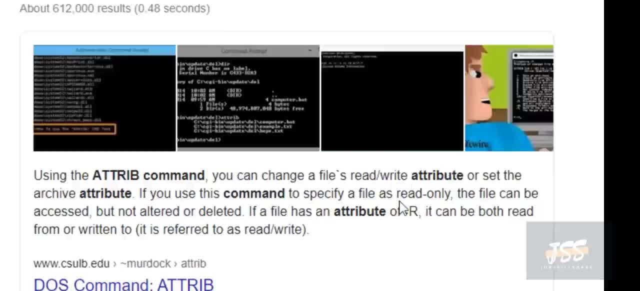 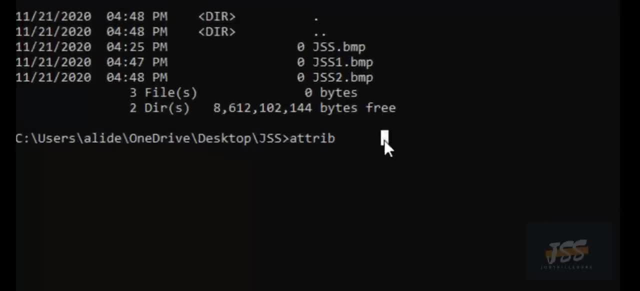 of information about this command and this keyword and what are the other arguments you could add with this attribute command. so let's go back and here what i'm going to do is just type plus h- h means for hidden, then plus r- read only. r for read only. 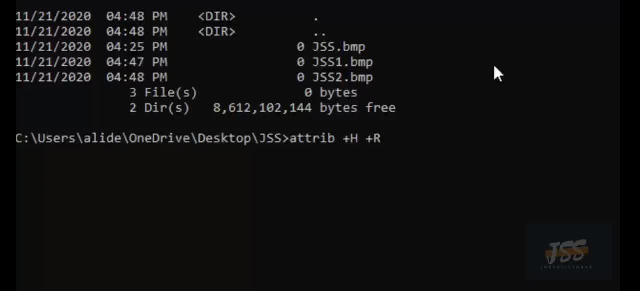 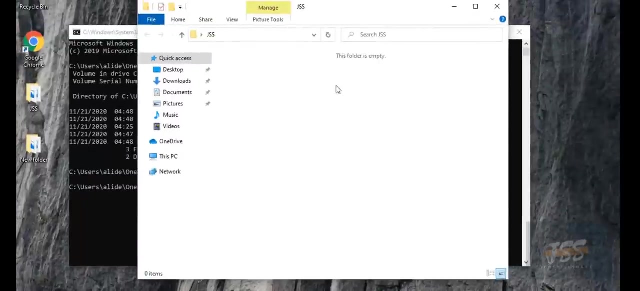 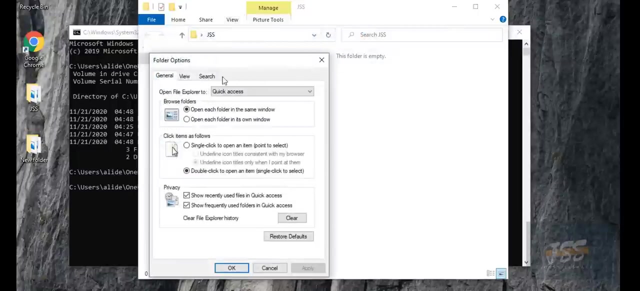 means file needs to be open and it needs to be check and click only. and then i'm going to add plus and s. as for the system, and if i press enter, so you will see if you go back to the gss all files are totally hide. and if you again go to the option and go to the folder option, 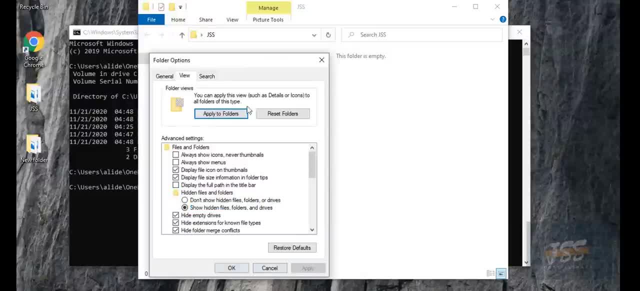 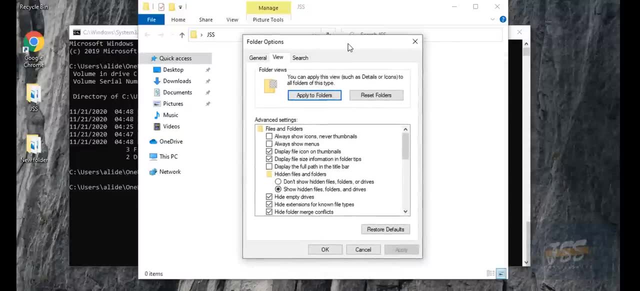 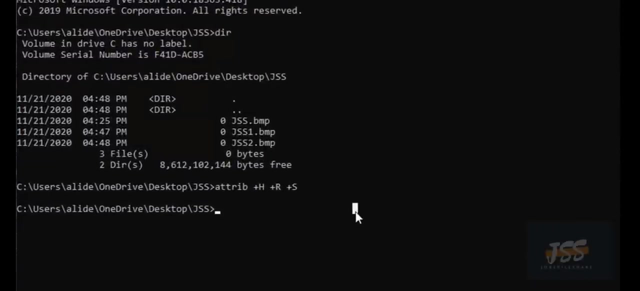 view and make check on show hidden files, you will see those files back because you totally turn off those files for access. so that's the thing i want to show in this video. so if i'm making those setting defaults, so what command really helps you to make those files visible again? so what you only have to do is just type minus. 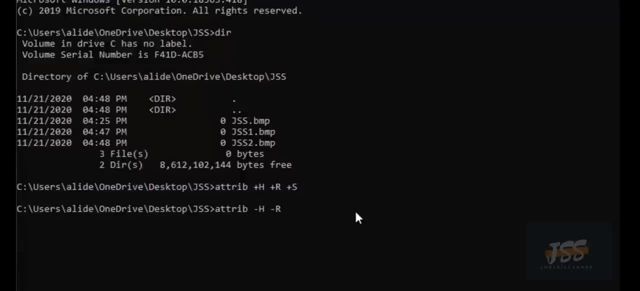 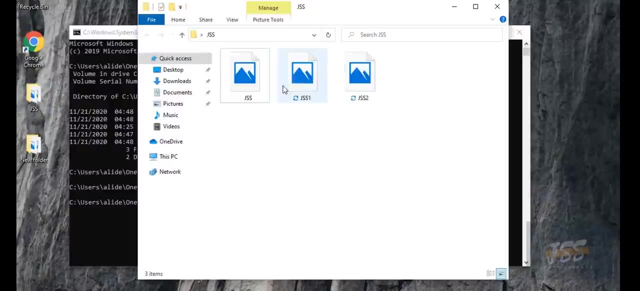 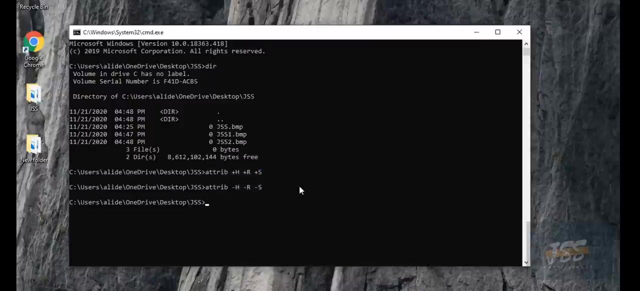 means just changing the sign. you're reverting the sign and then type the same command and press enter and if you go to the gss you start able to see those files as they were. so this command really helps you to totally hide your file and you can only the person. when you run this command, you can easily make visible those files. 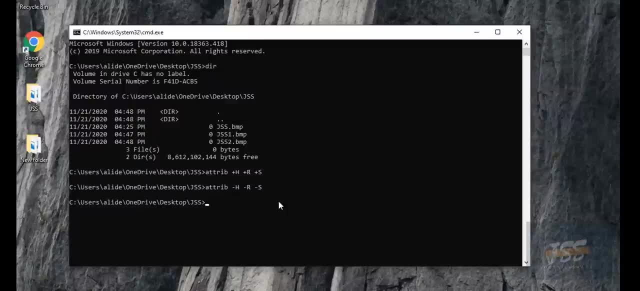 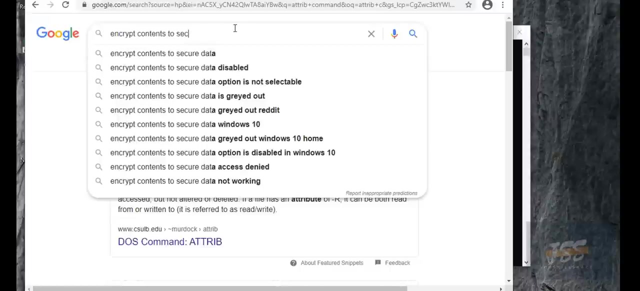 because nobody knows where you install your file, where you copy your data. so you're the one who knows on which directory you hide something now. after that, we have another command to encrypt file, and if you want to further research about the encryption, just go to the google and type encryption, so you get plenty of details. what is the? 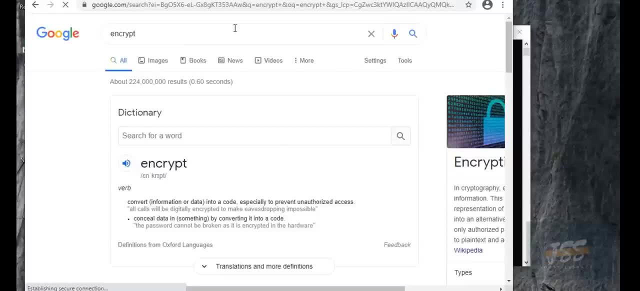 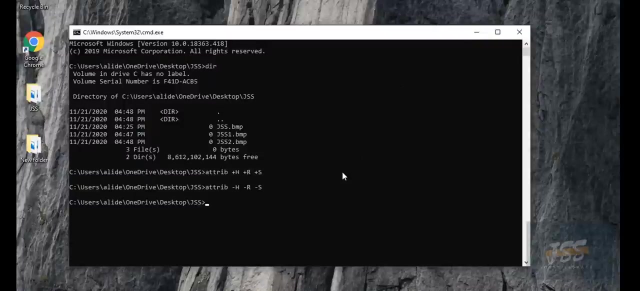 encryption and how it works. the basic definition you got is to convert information into a code. so encryption is what it converts: your file, your text, your, any information into unsensible form, in a form that cannot be readable. so, for example, if you have a file in your machine and you want to transport that file in somebody's usb or some other, 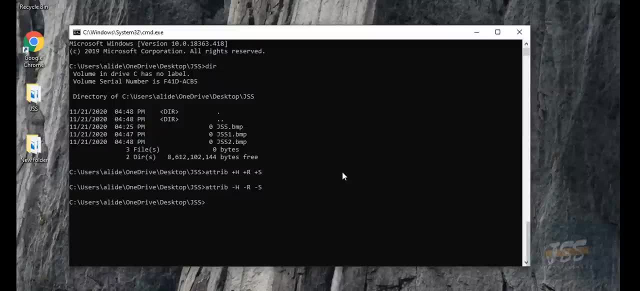 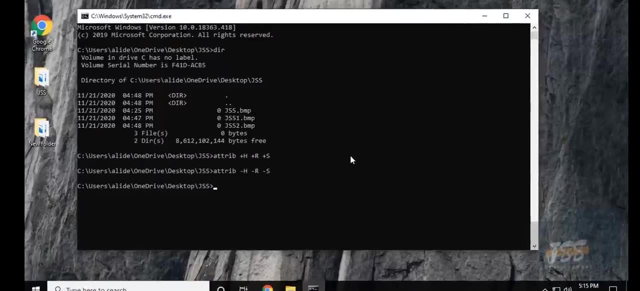 media and you don't want to just share this file with anybody. or there is a chances of recovering back of the data from that usb if you delete the file after copy that file to any machine you see. so in that situation you can encrypt your file so it will become a anonymous. 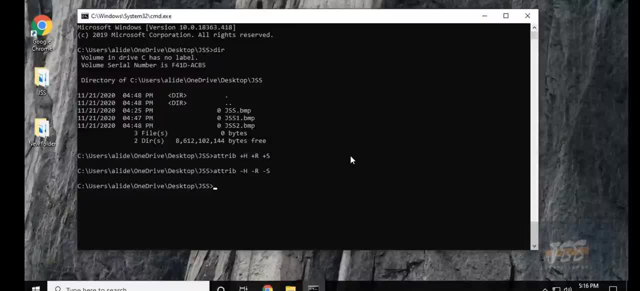 file, the file that is not useful, and then you can copy that file from your machine to that pen drive or removable drive, then paste anywhere else. so it's going to help you to totally hide the data within that file. so if you want to do that, you can copy that file from that usb. if you want to do that. 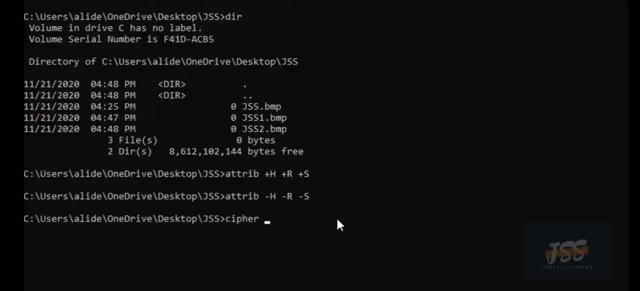 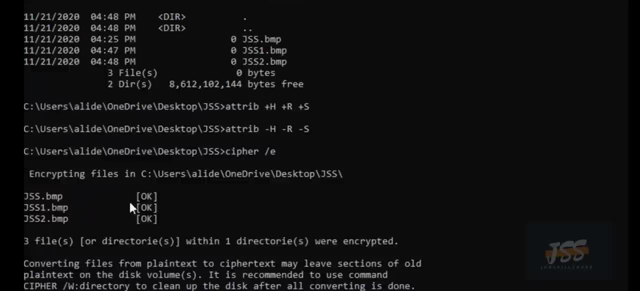 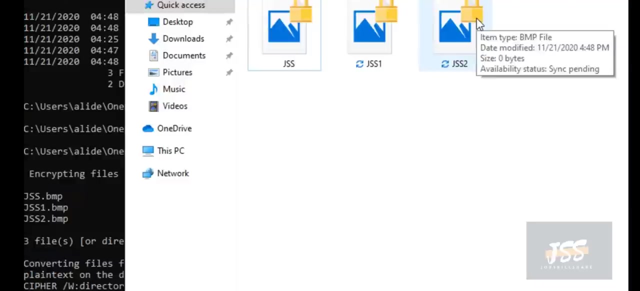 so what is the command to do that? cypher space forward, slash e and press enter. now there you can see. it tells that all three files are encrypted. and if we go to that folder you will see this lock on all these three files. that tells that all these three files are totally encrypted. 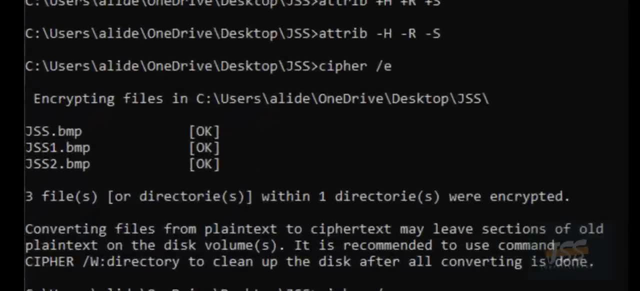 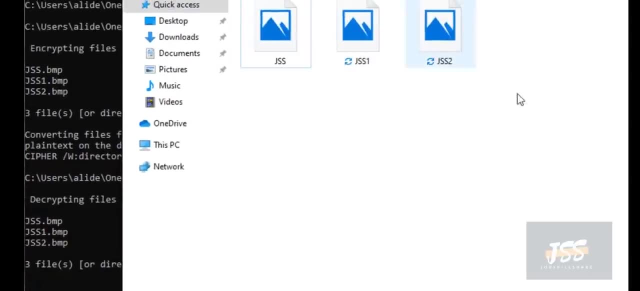 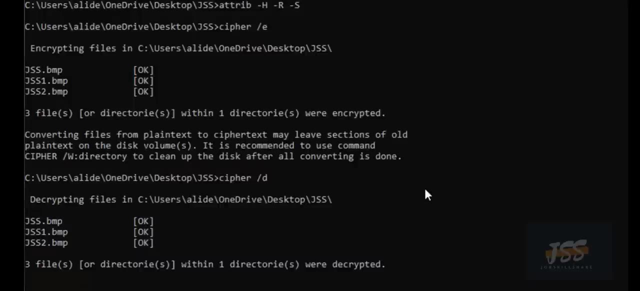 and let's say, if you want to decrypt all those files, so you can add d just after the forward slash and you will start seeing all those files normally. so this command will help you to encrypt your file and these files can only run on your machine. but if somebody try to copy those files, 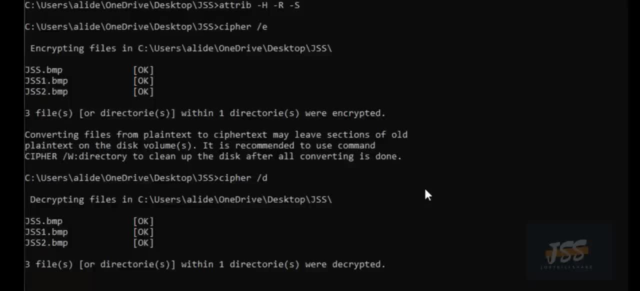 from your machine to another machine or another device, so that guy, that person unable to run this file because it is encrypted. and then we have another command to upgrade this encryption system, this encryption firmware that is added, and the command is: cipher forward, slash reiki. and then you press enter. 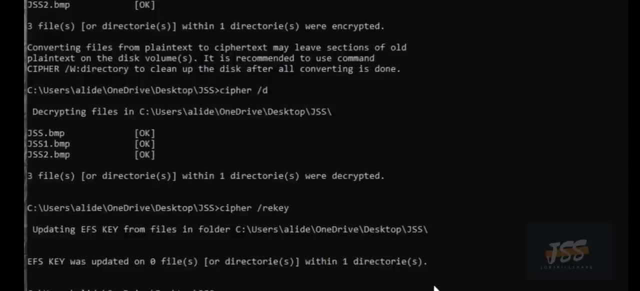 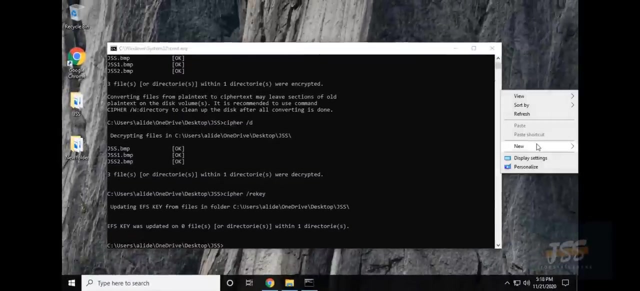 so it update your efs key from files in the folder, because once you encrypt your file, so there are definitely some keys created because keys, let's say, for example, if i open a notepad to explain this concept, what is the key in a little- i'm not going in the detail- 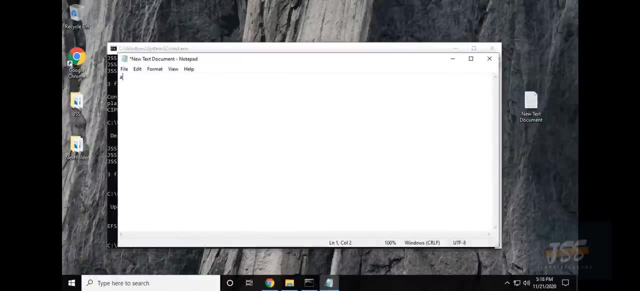 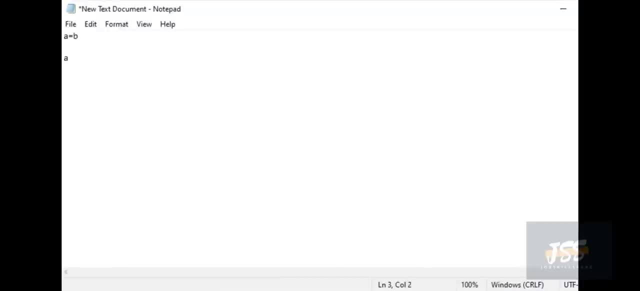 for example, I type a equals B, right, and then I type a, a and then I ask you what is the answer? you could reply: reply instantly that because equals to B. so the answer is BB. so a equals to B is the key. so if I send some data in the form of a, a, so the person right behind that communication and able to 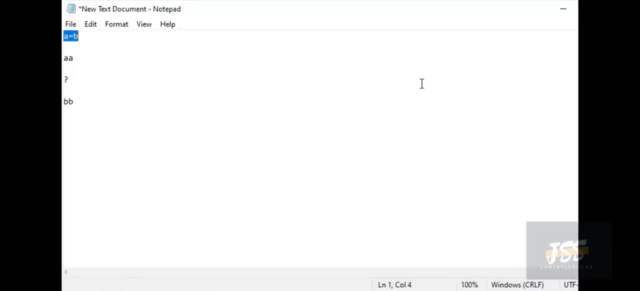 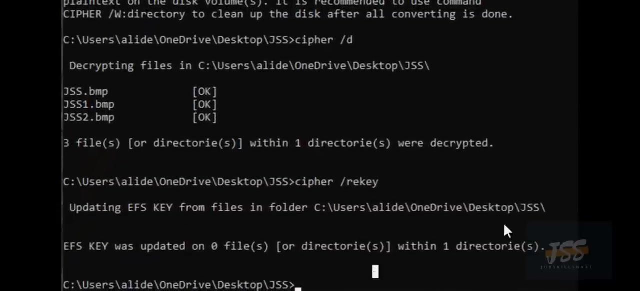 understand because he doesn't know about how and what is equals to a. so this is the key and this is a little concept I want to clear in this command-line course. this is actually the key. so if you want to update your keys of the files that are increasing, 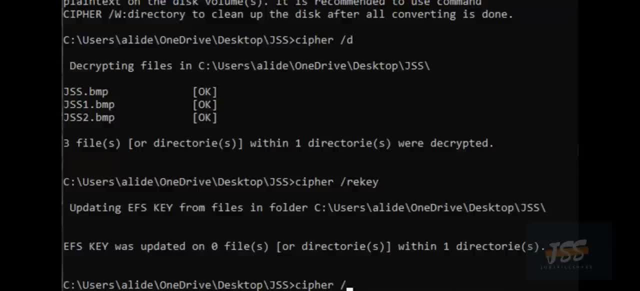 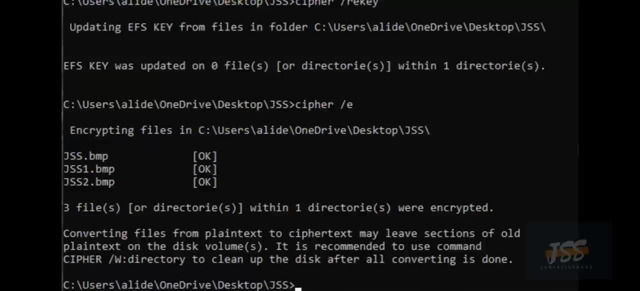 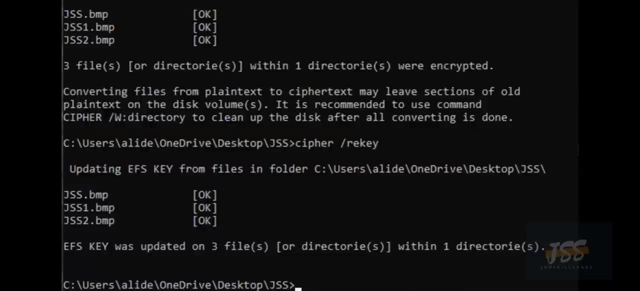 encrypted. let's say, if I encrypt my file by running this cipher forward slash e command- and definitely there are some keys created to decrypt those files, but in any case, if I want to upgrade those keys, so I run this cipher for side reiki command, so it's gonna upgrade all the 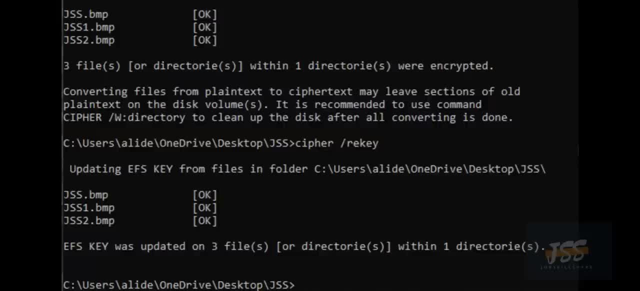 keys to decrypt those files. so if anybody, if any sort of guy able to know the keys of your file to decrypt, and when you run this reiki command, it will change all those keys. so the bad guy, the intruder, unable to decrypt your file again. so that's the purpose of those commands. 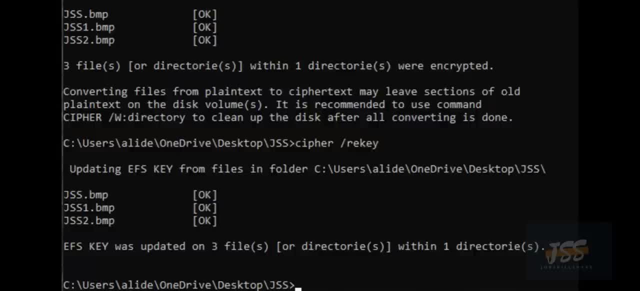 nonetheless, a command which we used to know about the file detail. let's say, if you have a file and you only able to see the extension of that file and you don't know that this file is related to which application, so you could run the command soak. and let's say, if I have dot, text extension. 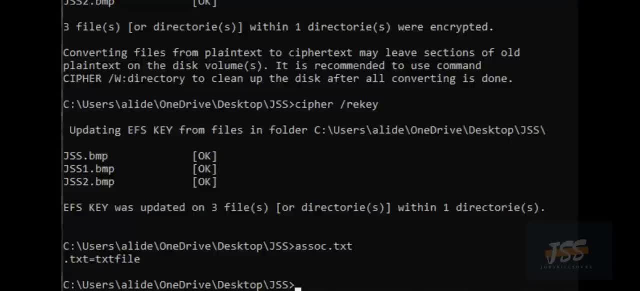 file. so it will tell me dot text equal to text file, which means it is a notepad file. so this command really helps you to know about the parent application and software that is handling that file and you could run any of the extension against this. so command association, this is: 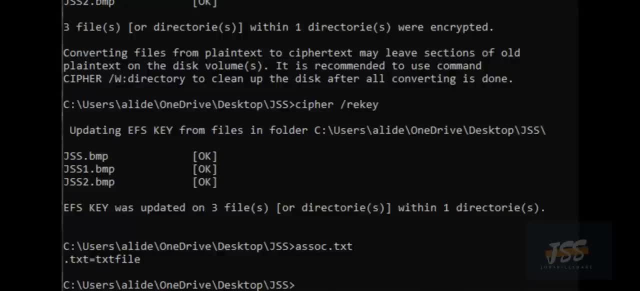 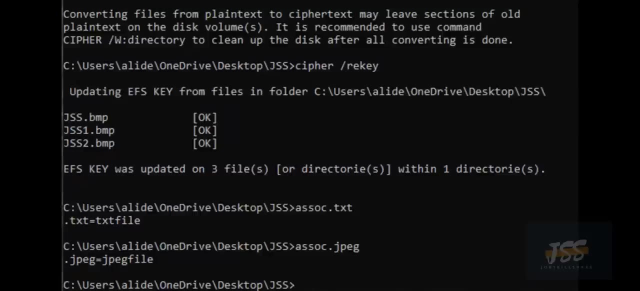 this awsoc full form is association, but here we need to write awsoc, so dot tags and dot jpeg, whatever you want to know. let's say we type jpeg, so it will tell us this is the jpeg file. so this command really helps you to know about the file detail with the extension, if you only 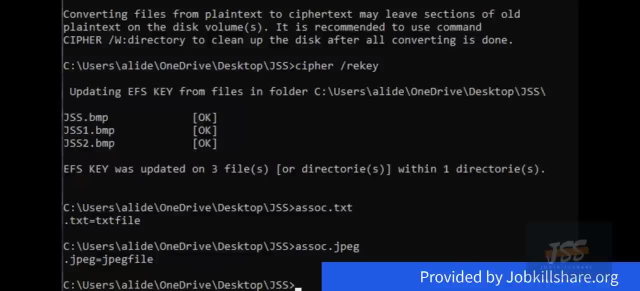 have the extension detail and you want to know that. which file is it? because these are the simple and basic extension. most people knows about those extension but in contrast, there are other extension that are so difficult to understand, to know, so you can simply type a soak dot that specific extension. 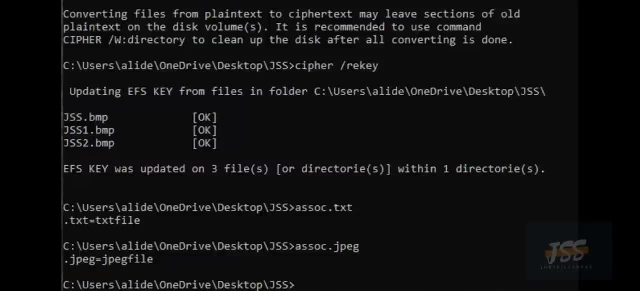 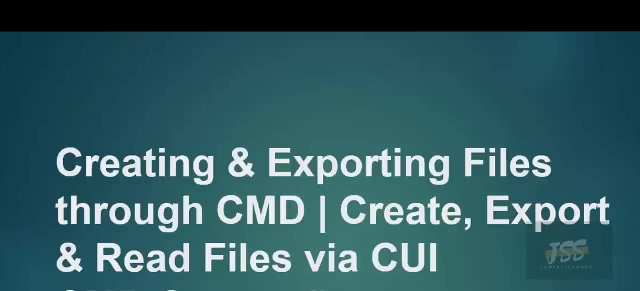 and then this command will tell you that it is related to which extension, in which file form, creating and exporting files through cmd. and in this video we're going to show you how you create, export and read files by using command line cui. so let's move to the desktop. so here on the win10 machine. 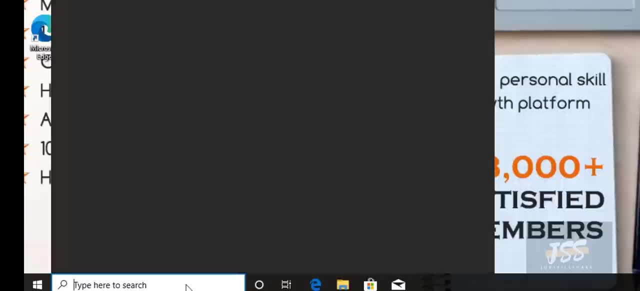 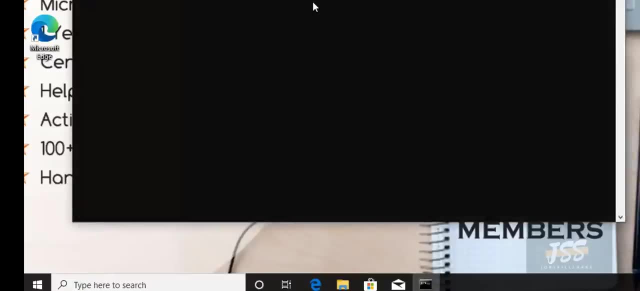 first we're going to launch the cmd. so I'm going to type cmd on type here to search and run as the administrator, and here you can see it is prompting to the administrator. but what I recommend during this practice that you should change the prompt to the desktop, because when we are creating files and 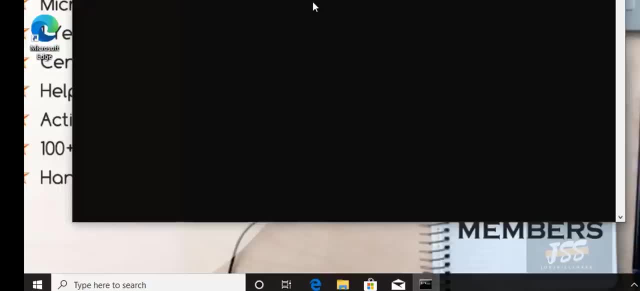 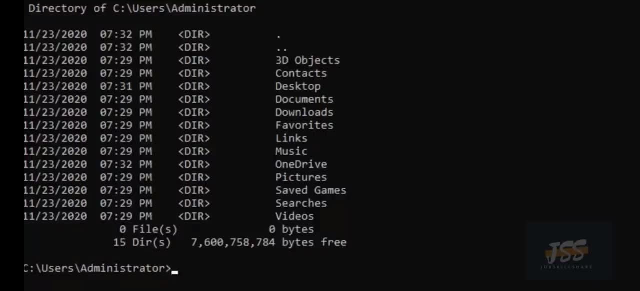 creating other things. so you will see the output in an instant on the background. so for that let me type dir to see the content that other territories we have in this administrator folder. so here we have desktop. so type desktop and directly jump into the desktop. now here, whatever the file, we're, 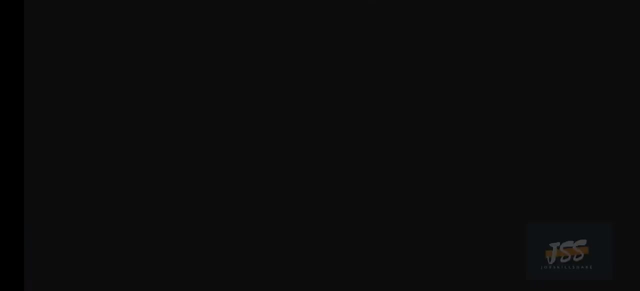 going to create will just get located here on the desktop and you can easily see on the background. so the first command I'm going to show you right now is the. let's say, for example, that if you open any service like the task list and you want to know that what sort of tasks are being running on the 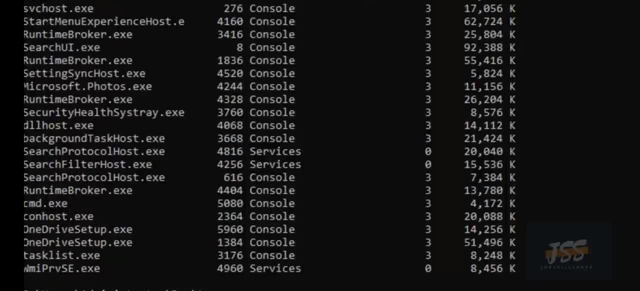 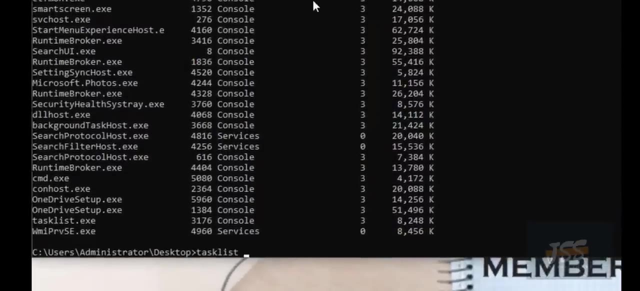 background of your machine. but here you can see there is a plenty of entries and there's a bunch of detail, and you want to export all these details in a separate text file. so the command you're going to type is: task list is the same, but you have to add some arguments. so put this greater than sign. 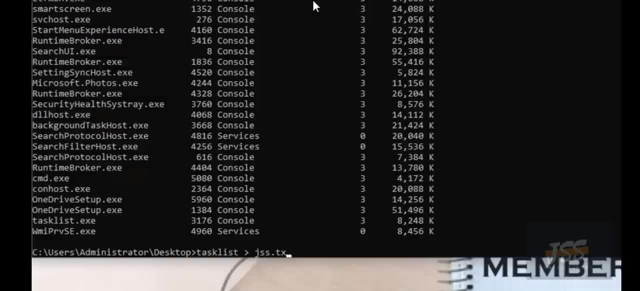 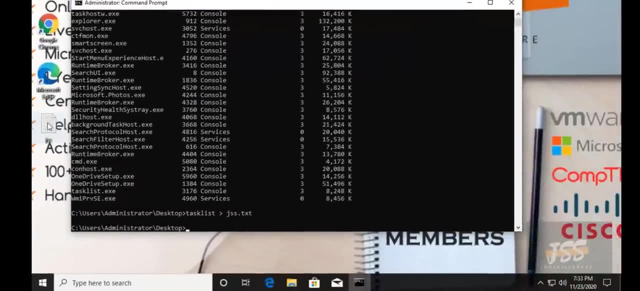 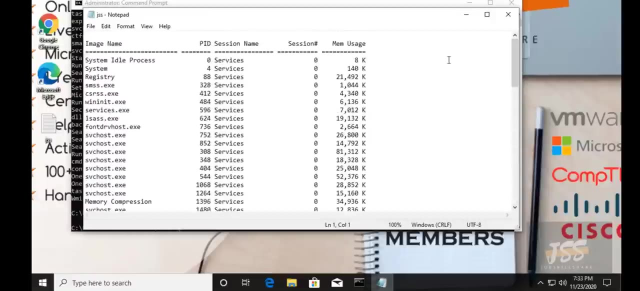 then type the file name and the extension and press enter. so it will create a file in an instant and you can see in the desktop background. and there you go. all the details and all the tasks are being created in a separate text file now. in the same way, if you want to. 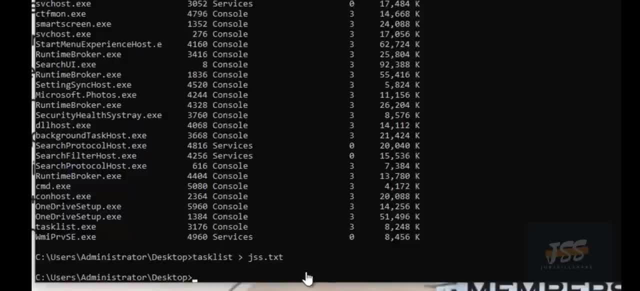 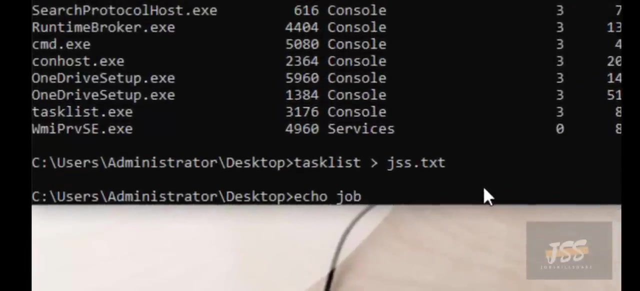 type any message, any details in the text file and want to export in your current directory. so you're going to type echo, ECHO, echo, and then you could type any of your message detail. whatever you want to type, it's like GSS or might be like type the website name, job, skill shareorg. 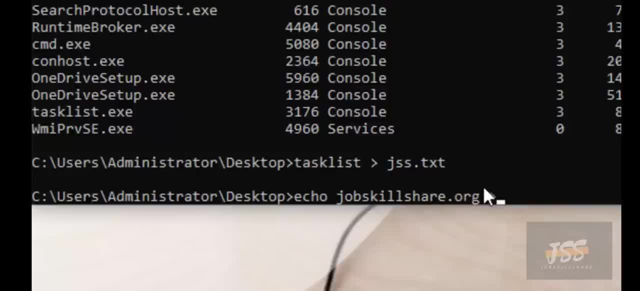 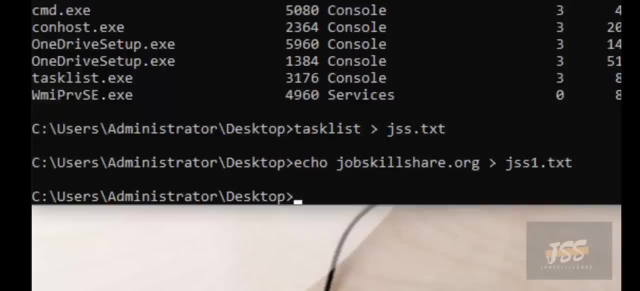 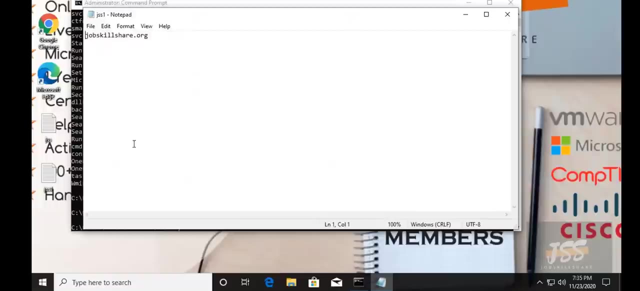 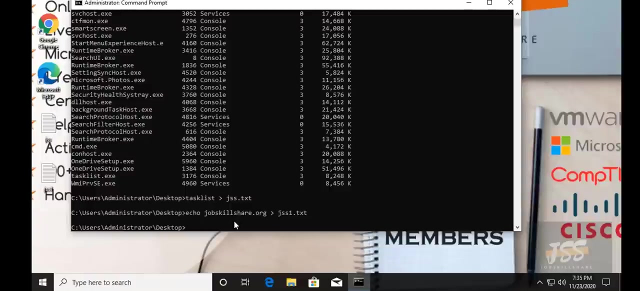 and then put this greater than sign, then add the file name gss1.txt, press enter. so it's going to create another file that contains the exact text you type here and if I open this gss1 so you will see that exact text that you mentioned in the command line is totally exported to that specific. 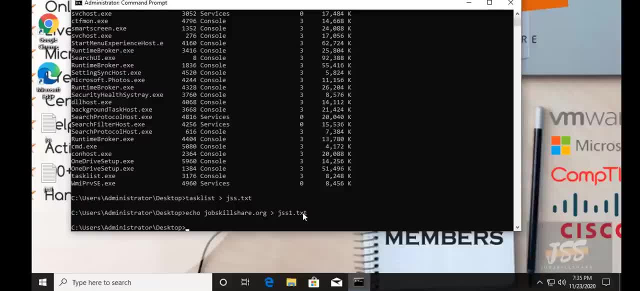 file. so this command really helps you to send and type any of your detail when you're in the CLI mode and you want to type any sort of message, you want to make any reminder, any memory, any sort of file, detail, IP addresses, whatever the stuff you want to export, or you want to type in a separate text file so you can use this command to export. 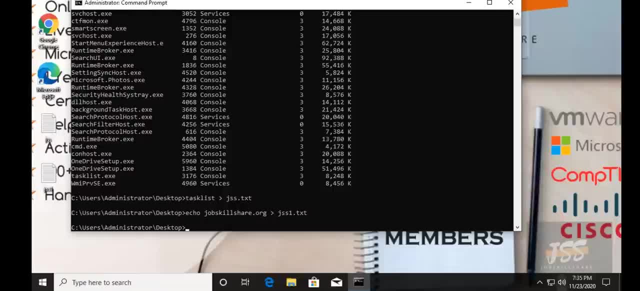 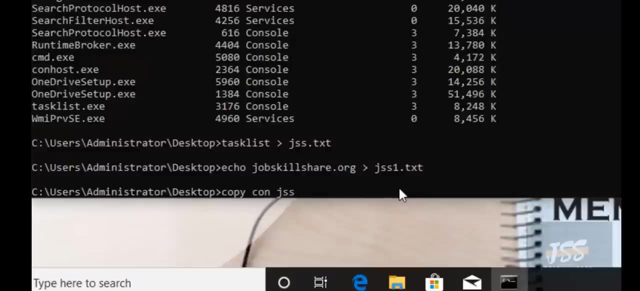 your text within a separate text file. now there is another command that allows you to type multiple lines, and you could go so much in detail while typing things like. the command is: copy, con space and mention the file name gss2. I'm changing one to two because gss1 and this is already created, so this commands this command. 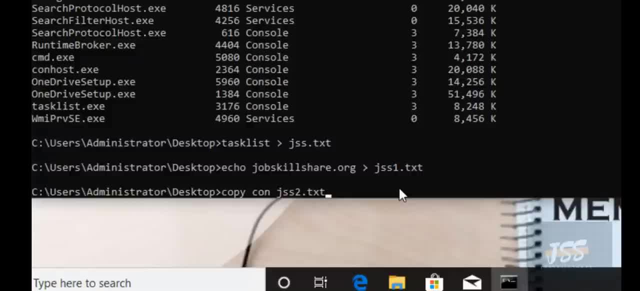 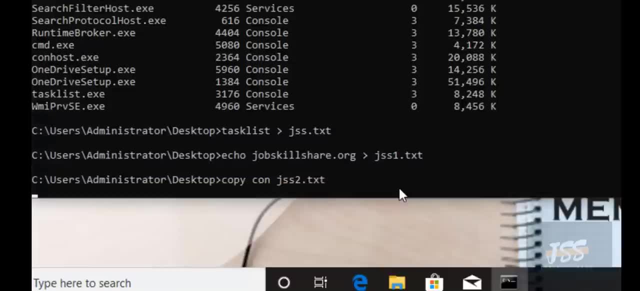 will allow you to type plenty of text, and once you stop typing by pressing the control Z, it won't stop you for typing the text. so here you can type anything like. please subscribe our channel right and after that, if you want to stop this editing mode so you can type. 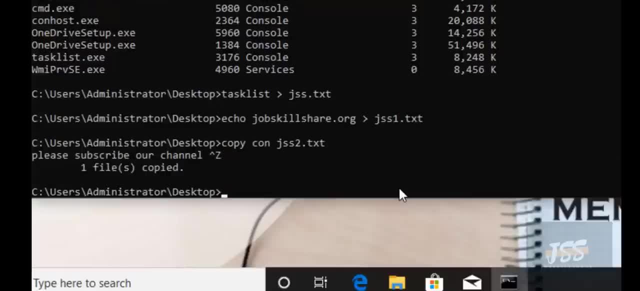 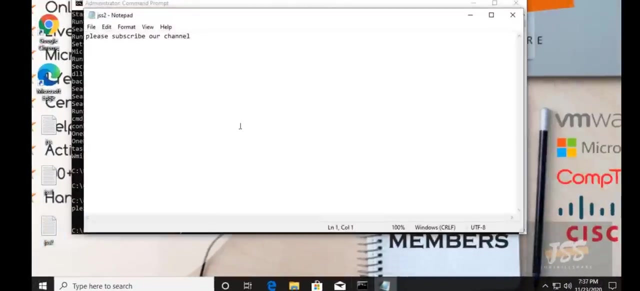 press ctrl Z so it gonna stop and then press enter. once you type ctrl Z it will show this Z here on the screen. then you need to type press enter, you need to press enter and then it will take out from the editor and the file is created as you want. you can see here on the back on the desktop you can see the text is there. 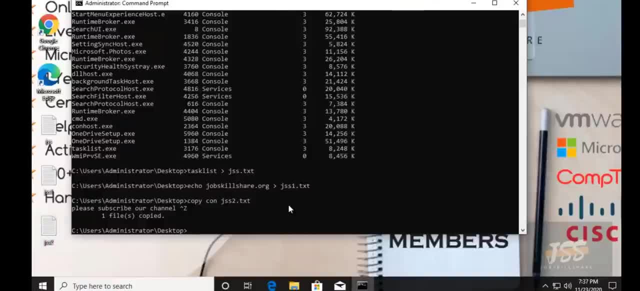 and the file name is the same. so you have two commands to type your message, your details, your text. but the copycon is allow you to type plenty of lines and multiple sort of words and whatever the bunch of details you want to export within the file name. so you could type here and you can easily. 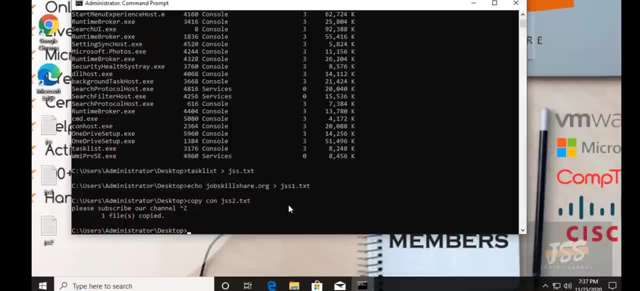 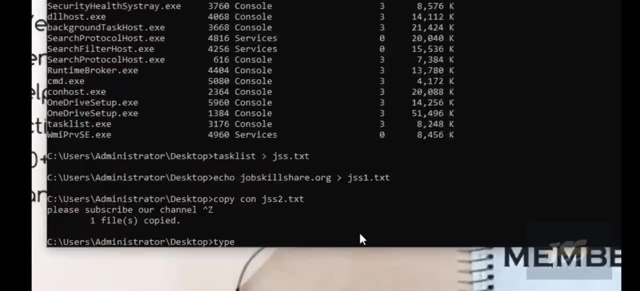 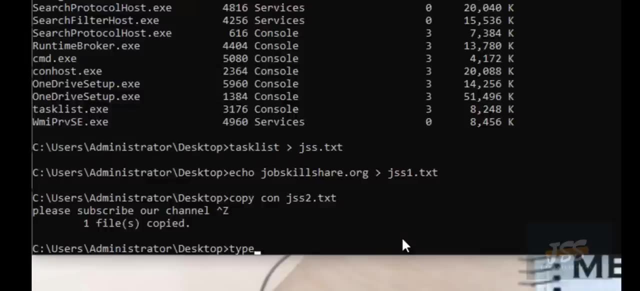 find out that file, where you create this file now, after creating those file. if you want to check the content of the file, definitely in the command line you can see the text. but if the command line, command prompt, is related to your Microsoft OS, so here you can execute commands from the CLI and it will execute. 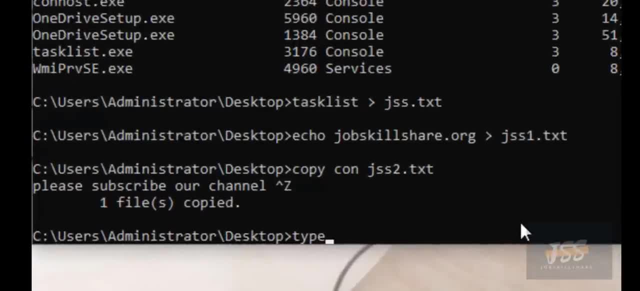 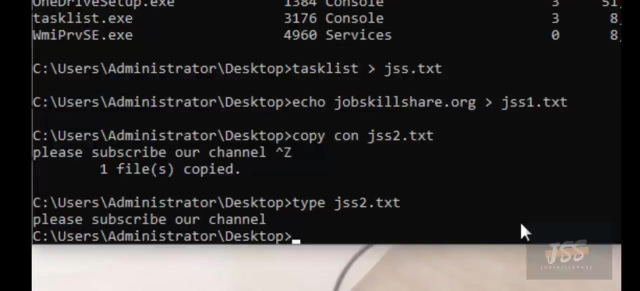 on your Microsoft operating system. but as for the text, if you want to see the text here on the CLI of the file, any text file, so you could type type, type type and the file name jss2 dot text and must add the extension so you will see the content, the text, the con, the thing that you put in that file, in the 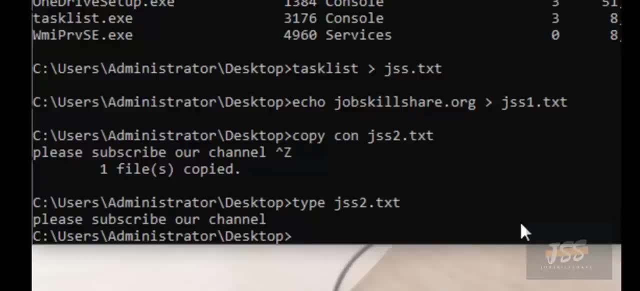 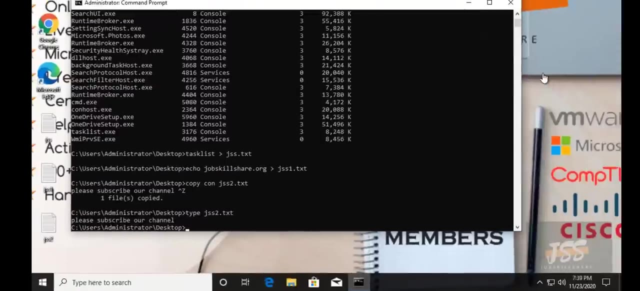 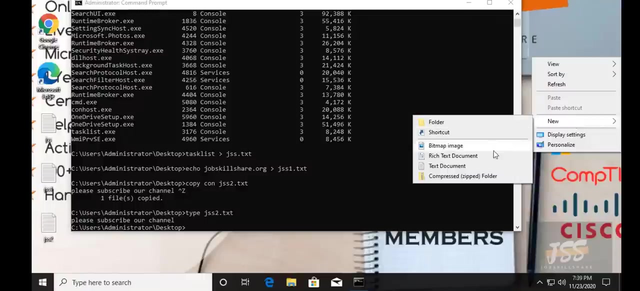 text form you can see in the CLI in your command prompt. so this command help you to open your text file in your command prompt in a CLI. so mostly time we want to create a new text document and we want to create new JPEG file and we did this steps, these things and so many, so many times. plenty of time to create a new text document. 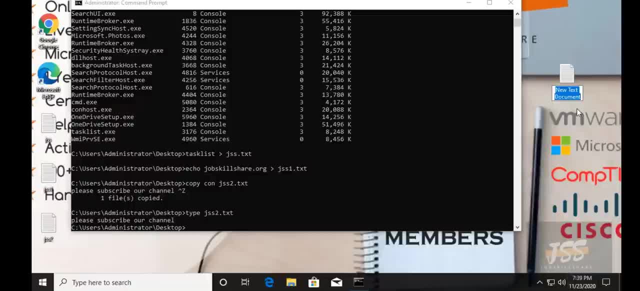 and it will create a totally new file for us and then we start typing and copying a stuff from the website and they're sort of places. so create a new file by just doing some GUI based steps. but what if you want to create a new text document kind of file by using the CLI? so the simple command. 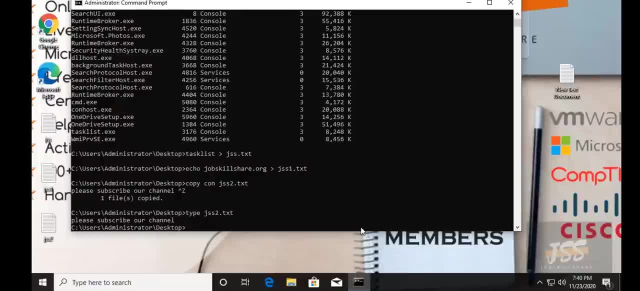 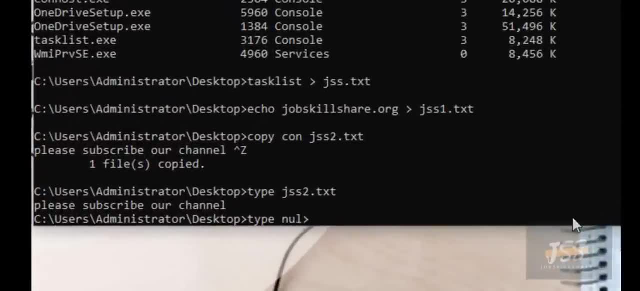 you need to execute is you're going to type type no, no means new stacks, because you don't want anything written on that file. it would be totally new text document based files. so type null space and just type the name already, because here you need to rename the file, but here in the CLI you are typing the name. 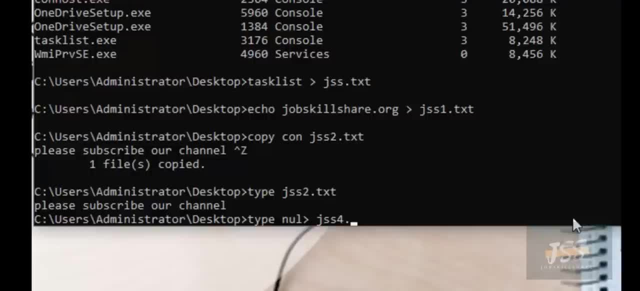 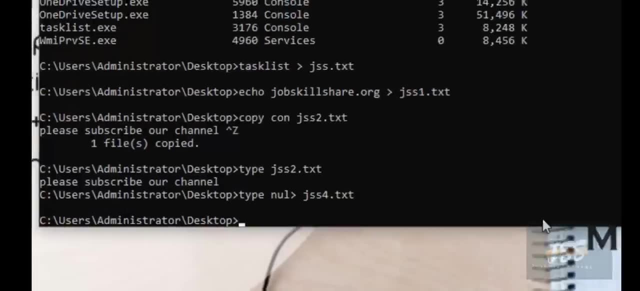 prior creation of the file. so: type: null greater than space. CSS for tax at the extension and you can see the CSS for is created and it's totally clean, a new text file. in the same way, you can create a new text file by just doing some GUI based steps by using the CLI. 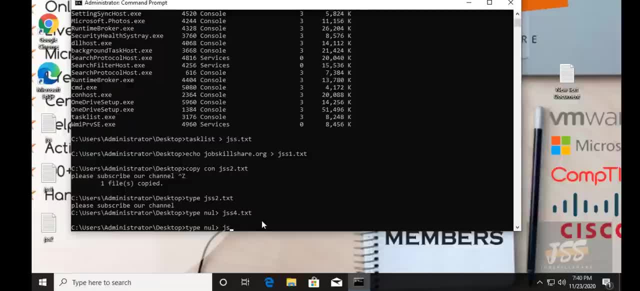 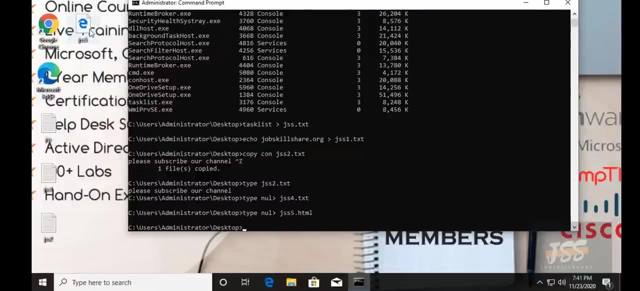 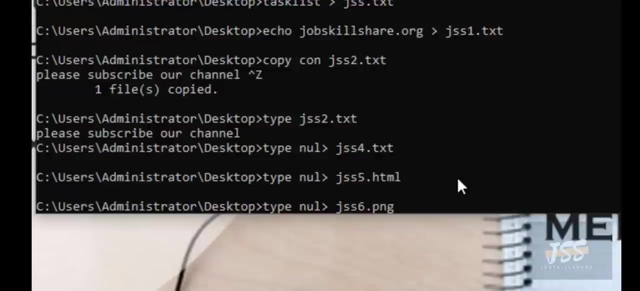 other extension based file, like, for example, if you want to create HTML new file so you could name gss5 dot HTML, you must be familiar with the extension. while using this command- and you can see here- new file is created. or you can type PNG and add six, so it's going to create a PNG file. so what you are just. 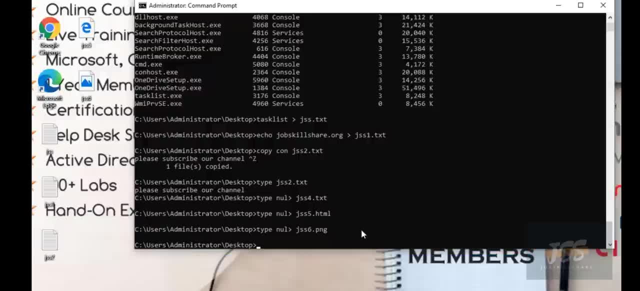 covering here is that by using this command you can create a new file. in most of the time we in the desktop, in the GUI environment, we create new text document and then we start copying it stuff and typing other details quickly. so by using the command line you can create this new files by typing these. 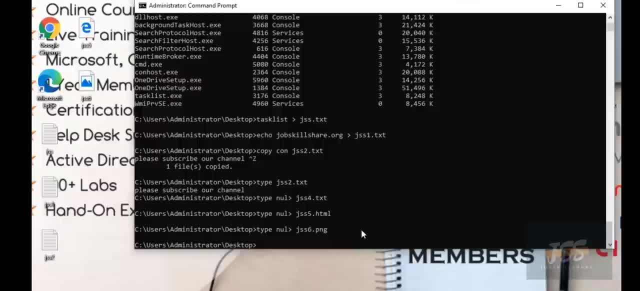 command would did those argument and with the extension and in the last, if you want to execute any text file, if you want to write a text file, the last important thing here- and I am going to leave the text fill asoud- to run any text file or any other file on your OS by using the CLI, because here 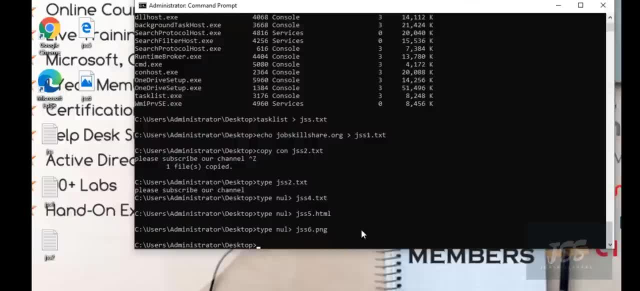 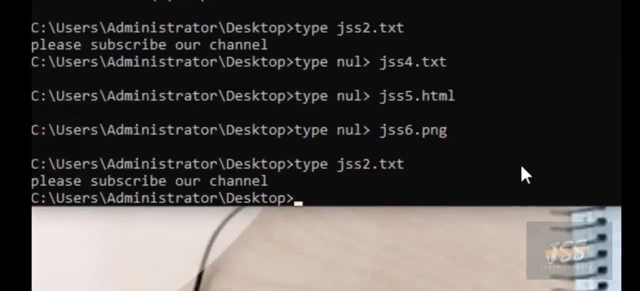 on top. I show you if you want to open any file in a CLI, like I show this command: type CSS to the text. so what? this command did? it just open the text. it orient the text on your CLI. but what if you want to open it in an? in that? 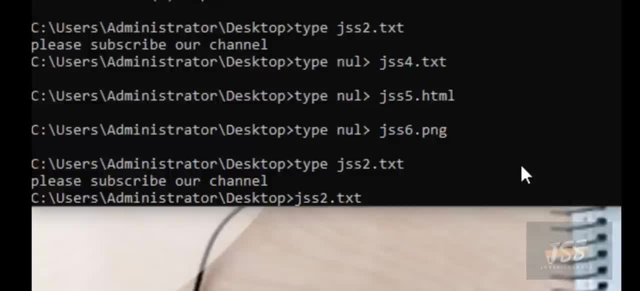 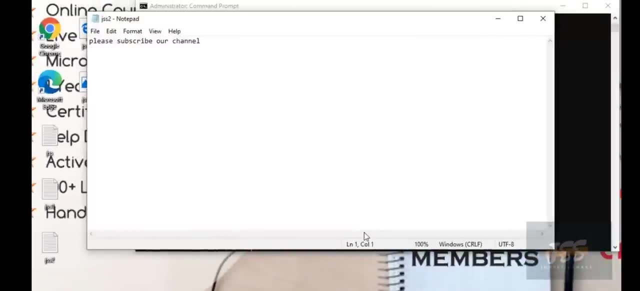 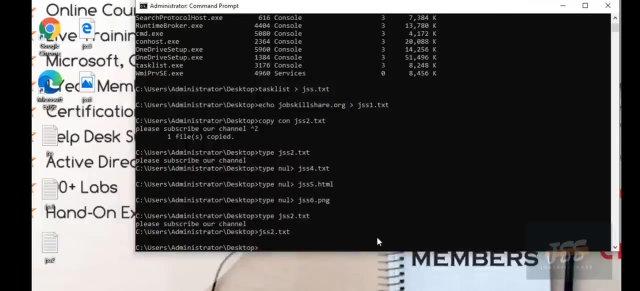 specific application in a GUI way, in a GUI. so what you have to do is just type the file name and press enter so it can execute the file and open it in. in an application, for example, you have pain files, so it can open that pain file in. 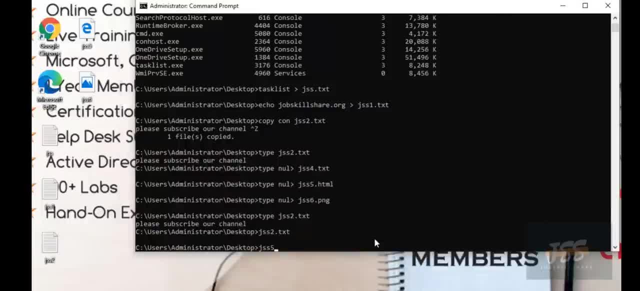 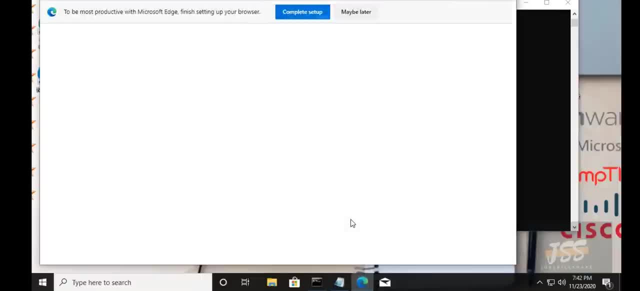 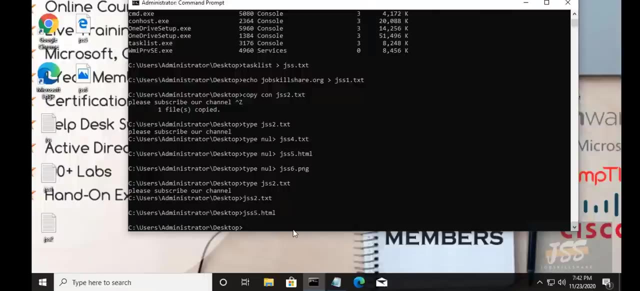 that, for example, we have gss5 dot HTML and if I press enter so it can open it on the Microsoft Edge or whatever the browser you're using in your machine. so this command will open the file on that specific application from which this file is originated. and if you type type, space and the file name with 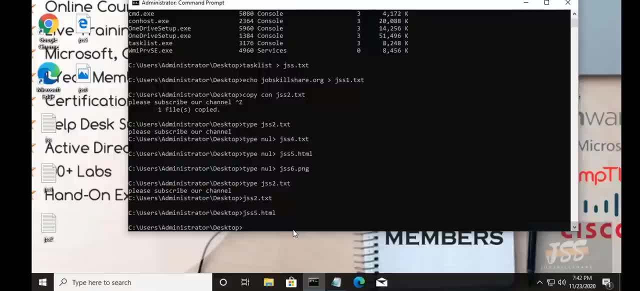 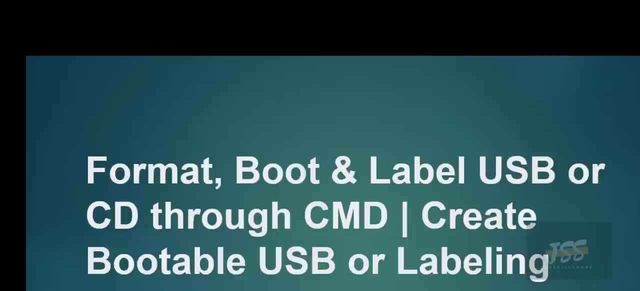 extensions, so you will see the text on the CLI. so this is a little difference. to manage your disk and if you use the GUI, so it require a lot of clicks and a lot of windows to open. but in the command line you only need to type some commands and the magic is on. so let's move to the Windows 10 machine. 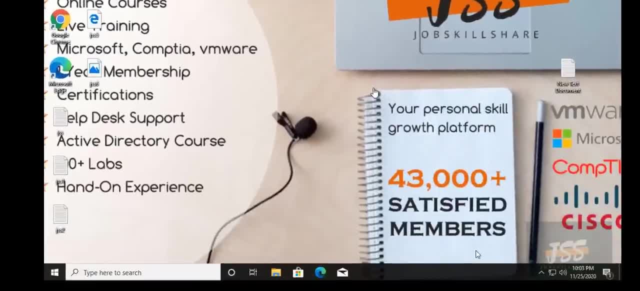 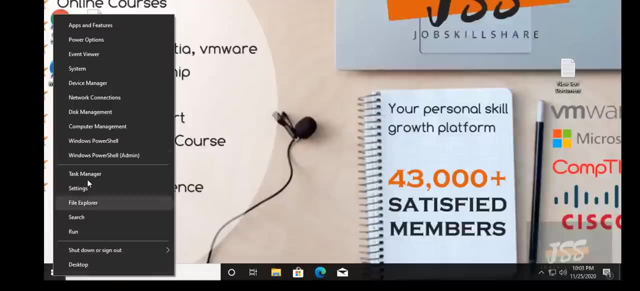 now here on the Windows 10, let me show you, if you use the GUI and you want to manage your disk with the graphical user interface, so which menus and which console you need to open if you right click on the Start window and there you will find this management console. so if you go there, 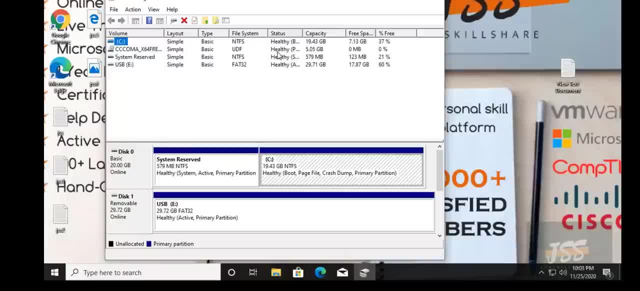 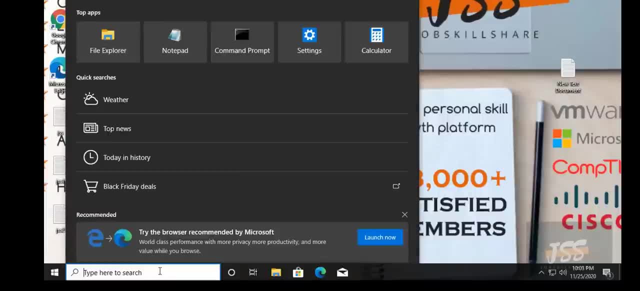 so it require a lot of clicks and a lot of options to select. but if you want to do your work directly with the commands and in the quick way so you could run command prompt and then they click to the type here, to the search, I will get. 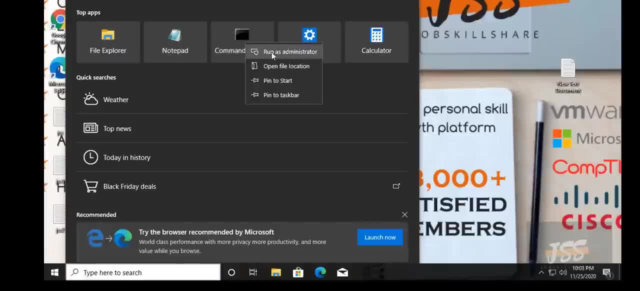 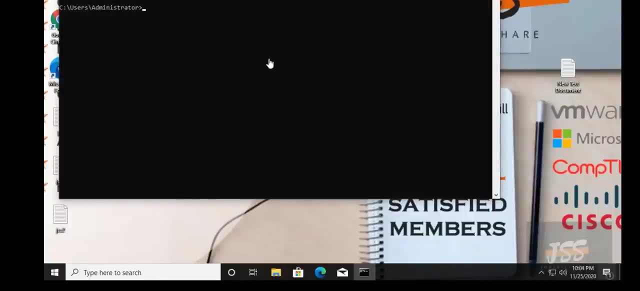 the command prompt automatically. so right-click on the command prompt and run as the administrator. so here in this test, I'm going to show you how you will format your USB, your pen drive and your USB cable to work in the command prompt. so I'm going to show you how you will format your USB, your pen drive, your USB and your pen drive, and your pen drive and your pen drive. 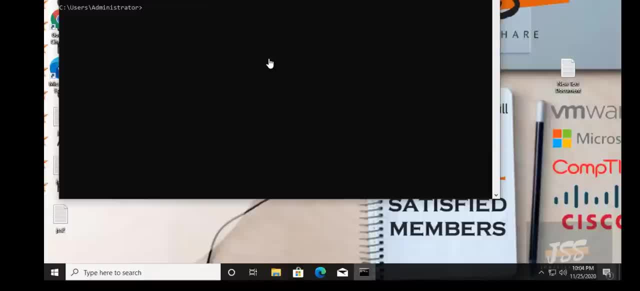 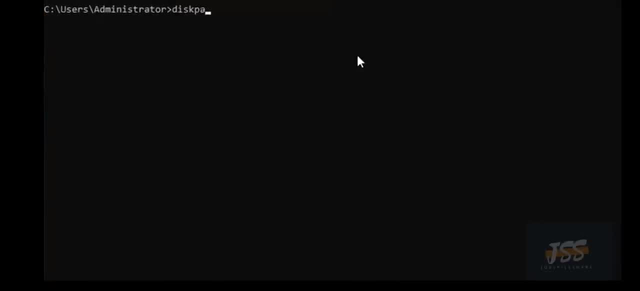 and how could you label that drive and how could you manage that drive? by using the commands. so the first command we're going to execute and run here is a disk part, and this command actually took you to the disk management environment. and here there are: after getting in the disk part command, you 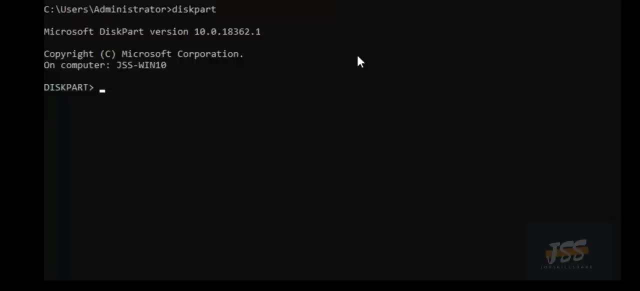 have only few commands related to the disk management you could run here. you cannot run all the commands here after get in the disk part environment. so here if you want to check the number of disk you have, so you will run the same command that we covered previously in the task. 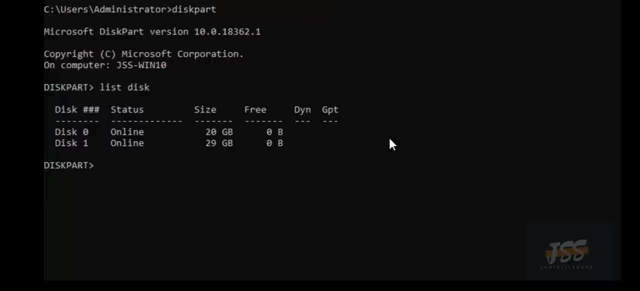 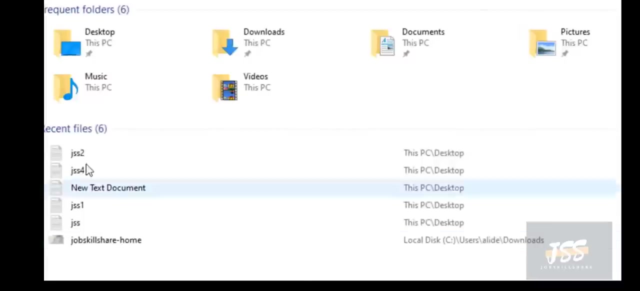 list disk so it will show you the number of disk you have and the disk 0 is a 20 gigs. that's our primary disk that contain the operating system. and this one is what is the removable drive. it is the usb. and let me show you in the gui, if you click to the file explorer and click to this pc. 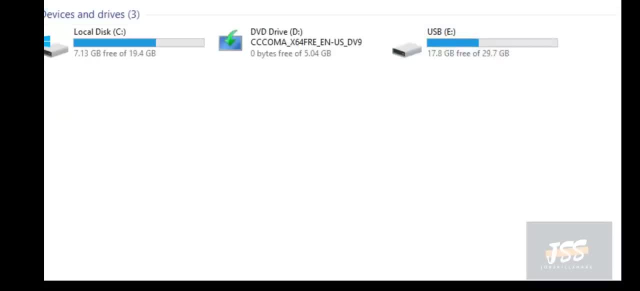 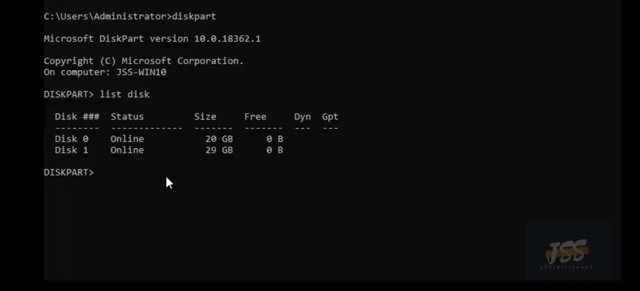 this is the usb that i attach for this specific video to show you how to format and label that disk. now, after typing this command, you have another command to select the specific disk, and the command is select disk 1 and it depends on the number of the disk you want to select. so you 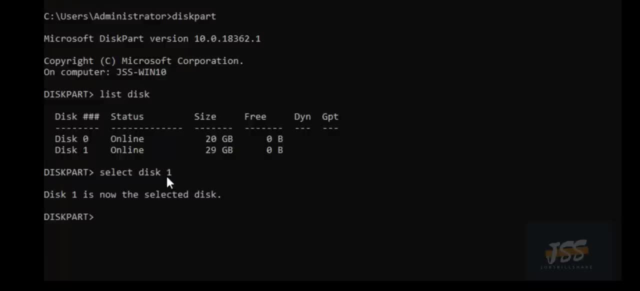 you could write that same number here. so i want to select the disk 1. and now here the disk 1 is selected. now we're going to run a command clean to just do a quick check over that disk and after cleaning that disk, once we get this successful message from the command line that the 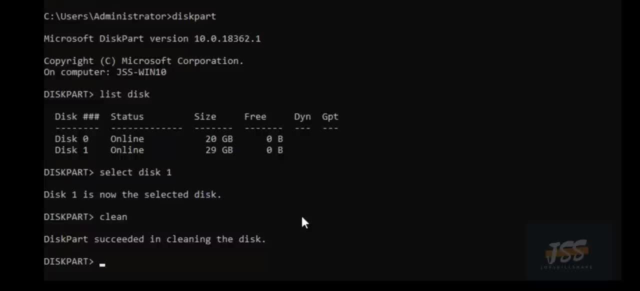 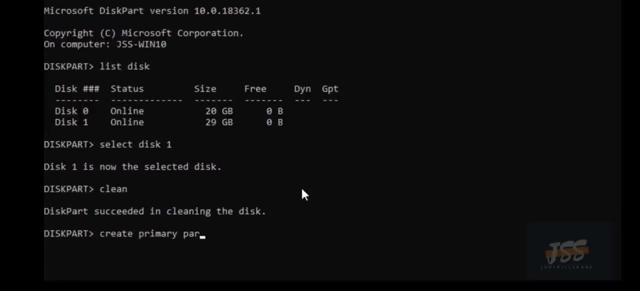 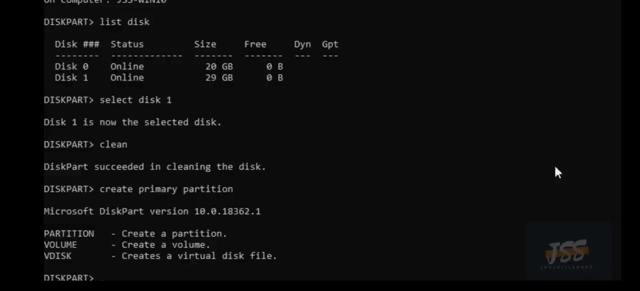 disk is clean, then we're going to create a primary partition of the disk and for that we're going to run the command create primary partition enter. so this is the command range we have and, as you can see that i misplace the name, the exact key, like create partition primary, is the exact command and i run create. 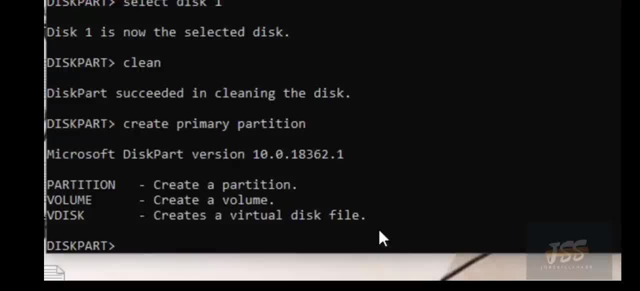 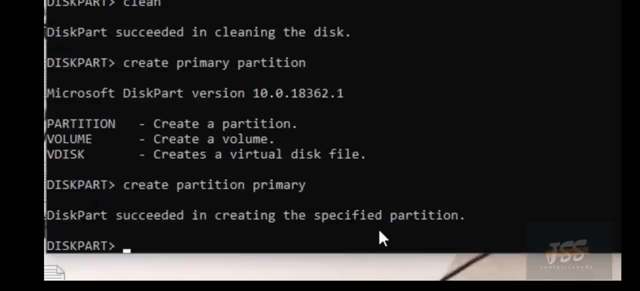 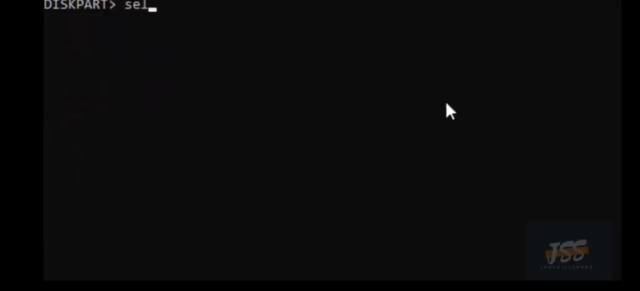 primary partition. so it will tell us that you need to put that word, that word, that specific command word before that one. so we need to add: create partition primary. press enter and there you go. you get the message that the primary partition is successfully created. now we're going to select the partition one. so the command is: 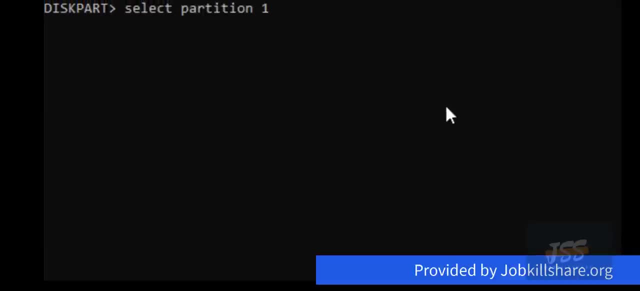 select partition one. so after creating the partition, we just in the selection of that specific partition and now we're going to do other stuff and the stuff is to find the desired partition format. and this is the main and the main part of this video, that how you could. 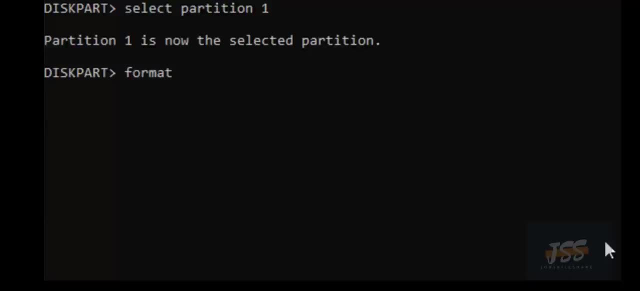 format your partition, your removal drive, your pen drive with the command line. so the command is: format FS, file system equal NTFS and then space, add the keyword quick. so it will do this whole part quickly, but late, take a little time, but after all, in compared to the normal format, it does this work quickly as 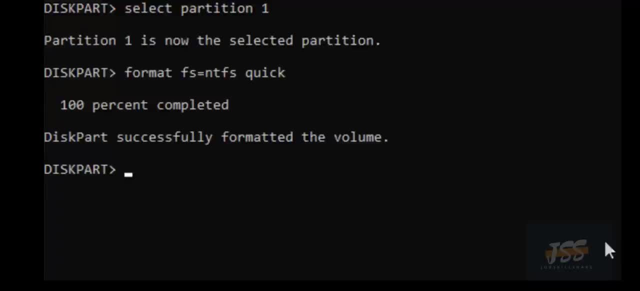 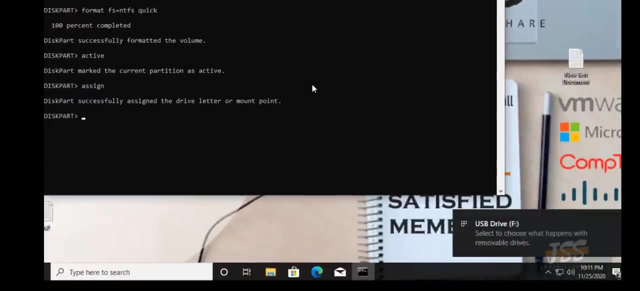 compared. now, there you go, it is hundred percent complete and formatted. now it's time to active this specific drive and it is now markets active and then we're going to assign that partition and there you go, it is attached and now in a working position, but here you can see, is still it. this drive don't have any name. so after: 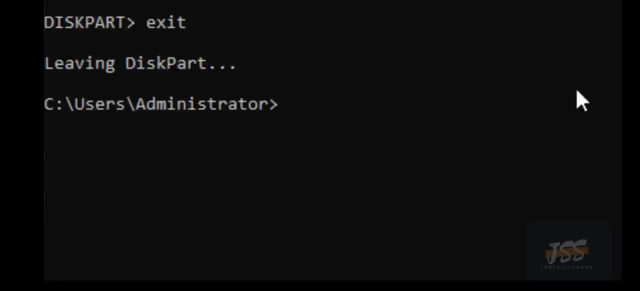 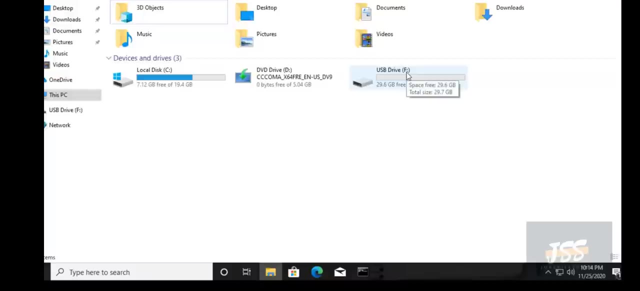 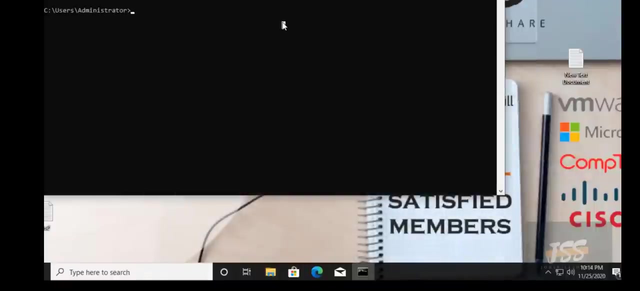 assigning. we need to exit from the disk part by just simply typing exit. and if we go to the GUI, we're going to find that the we have F drive, the USB, but it doesn't contain the label. so to name it, to make a label on that drive, we just 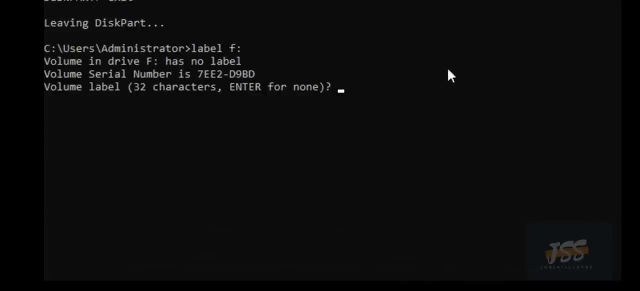 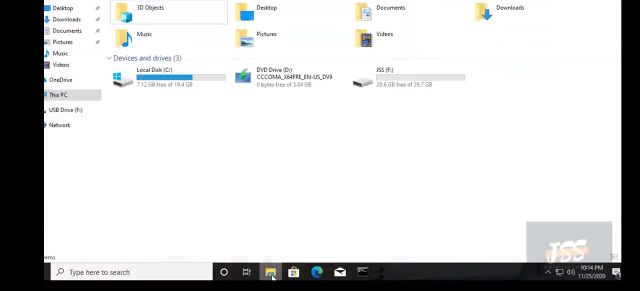 simply type label and the drive letter F. now there's a mode open for you and you can type any of the name. so I'm going to name it JSS and then press enter so the label is changed to JSS and you could verify here too that the chain name is changed to JSS from the simple F drive. 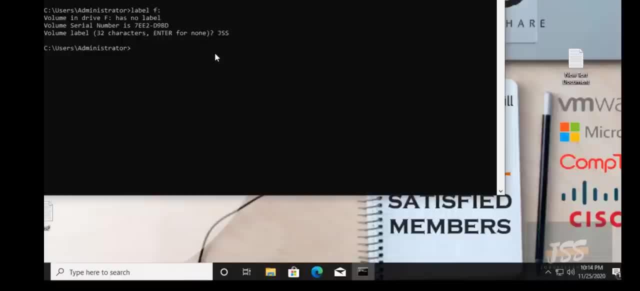 so by the help of these commands, you can format your pen drive. you can simply select, you can change the label, you can clean your disk, and I'm going to show you some of the commands with this program in the video description. another cool thing is that everything is six single digits. you're using an entire memory and untraded IT. storage. so this program allows, if you need, you can step up the mode and copy all the contents of that, the question you have. so before we go further, let's take in a time up group one you have, uh, but let's name this code. that is actually the disk management. 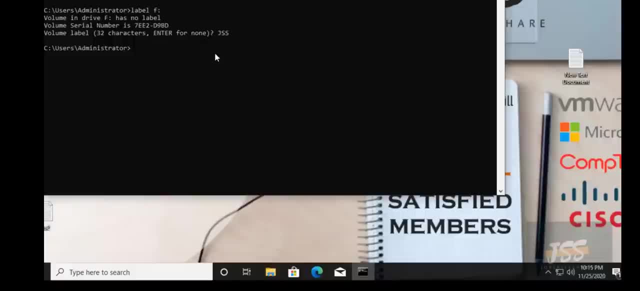 commands all. now the question is if you want to make your USB a pen drive with a bootable USB for Windows operating system. so the process is simple: just follow all the of that ISO in the same USB, the same pen drive, and it will become a portable USB. 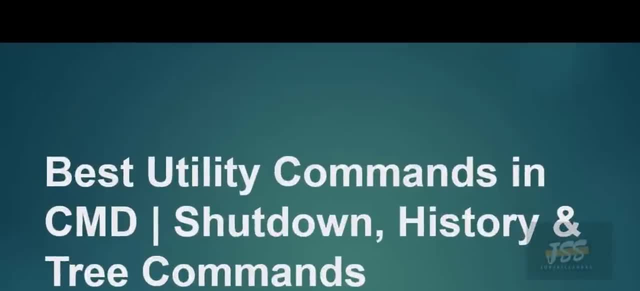 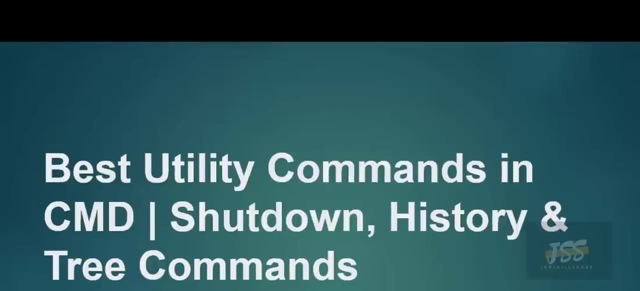 for Windows installation. we have the command tree shutdown history, so we will cover those command that can already help you to check the previous command you executed and the command related to check the whole directory of any drive, of any folder. so, without any wasting time, let's quickly move to the Windows. 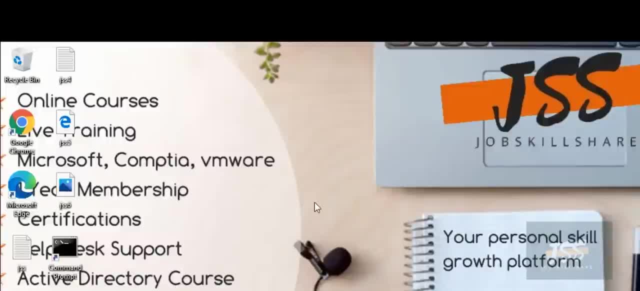 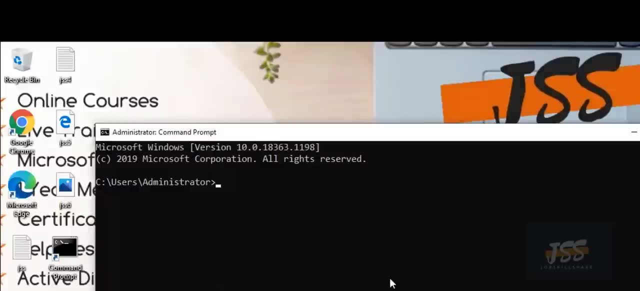 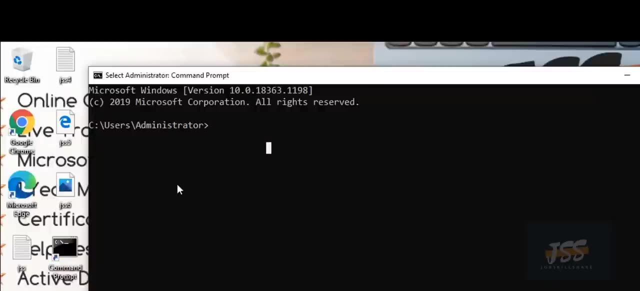 10 machine here. let me run the CMD with the administrative privilege. so it's simple. as you know, right click on the CMD and run as admin. now, there on the CMD, the first command we're going to execute here is a tree. so let's say for. 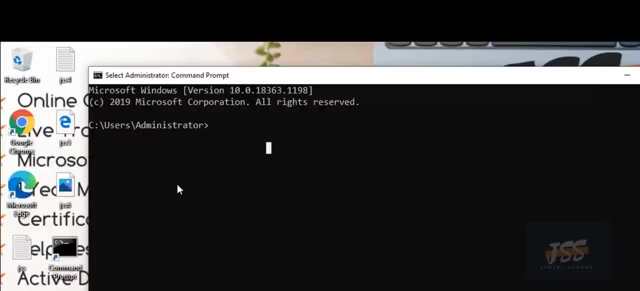 example, if you want to check the folder, the directories and the subdirectly, because you want to check the folder, the directory and the subdirectly, because you want to check the folder, the directory and the subdirectly, because you know, in any of your folder you also create some other folders and even with 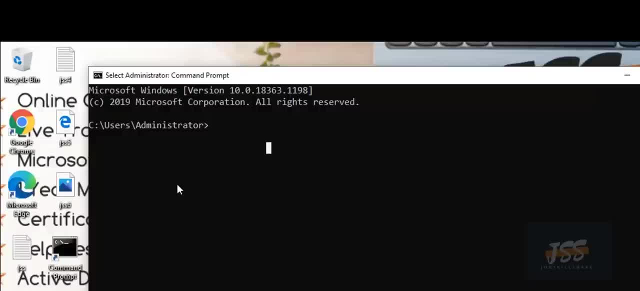 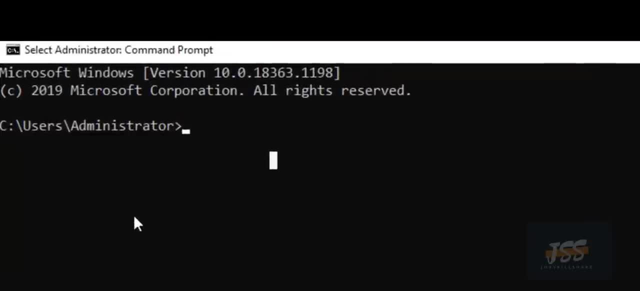 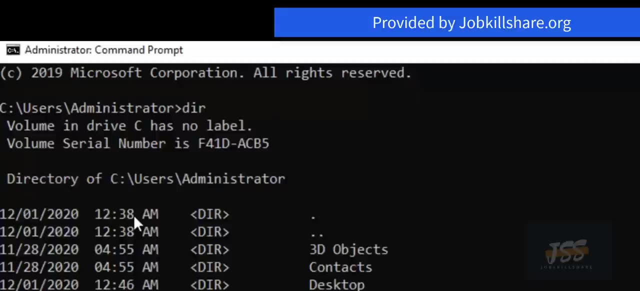 the file when you install any program, any application into your machine. it also created folders, then the subfolders, and that that subfolders contains your executable files. so let's say, if I type dir under this administrator folder, you could see these folder, but definitely there are some other subfolders that are 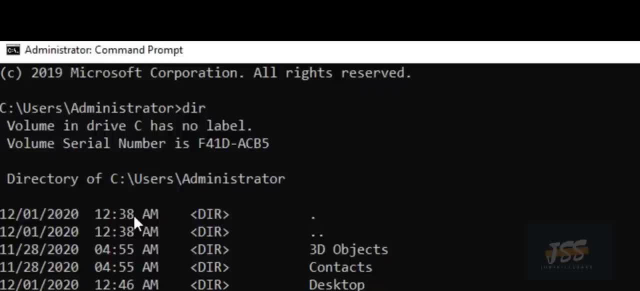 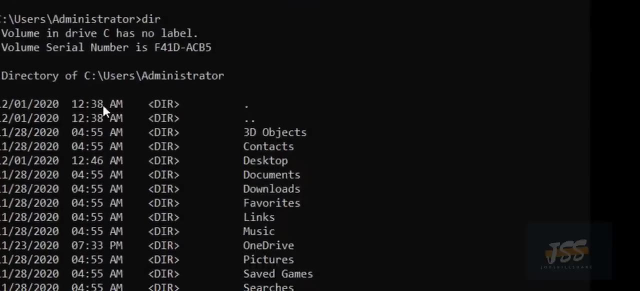 in that folder. so let's say, for example, if you want to check any directory or any executable file and you are guessing that this might be here in that sub, that main folder, and you are not sure about the subfolder or the exact location of that file, so the command tree will help. 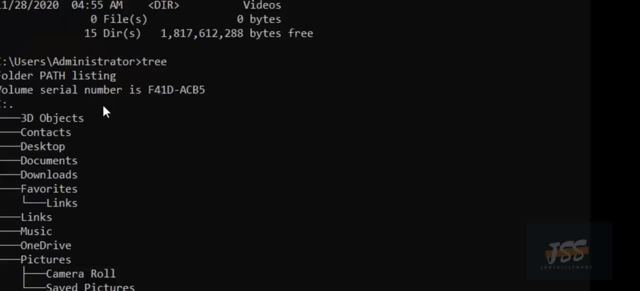 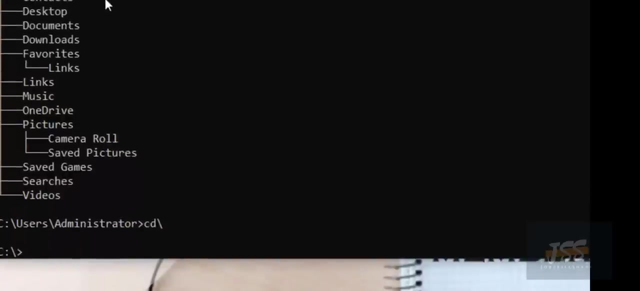 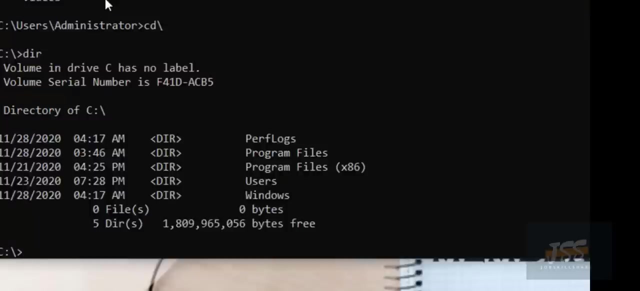 you to know this and you just only type tree and press enter. so there you can see. it is providing you the subfolder detail within this administrator folder. let's say you wanna know about the whole directories having in your program files or in your windows, so which command you're going to? 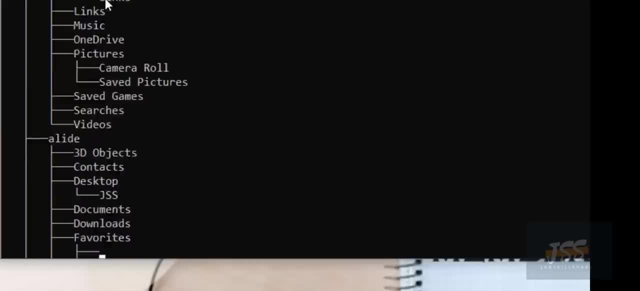 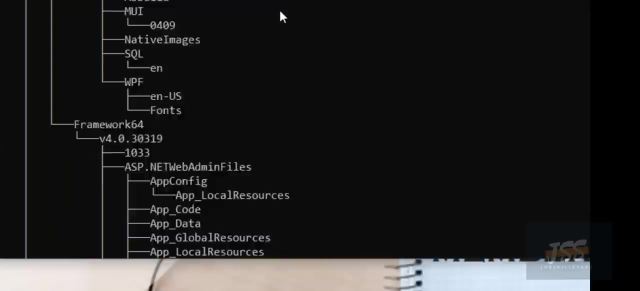 use tree. so what it will does? it will collect every file, every subfolder, and display to you in a form of three, that in which folder there's a subfolder, and then other folders, and then it will reach, it will show you that which executable file and. 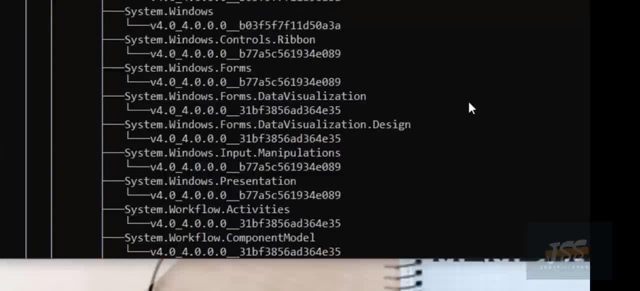 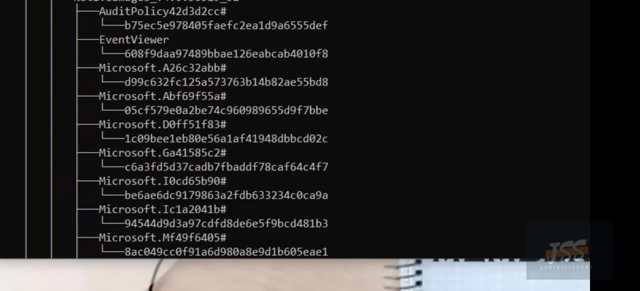 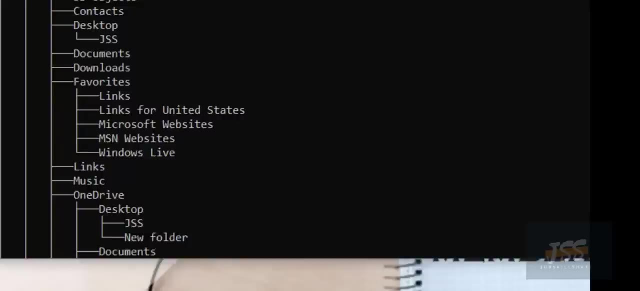 which file is located and at which subfolder and which is originated with that specific folder. and you can easily figure out by using this tree command and as you can see here, that it cover any, every folder of your C Drive and provide us the file locations and all the structure you could say, and this is 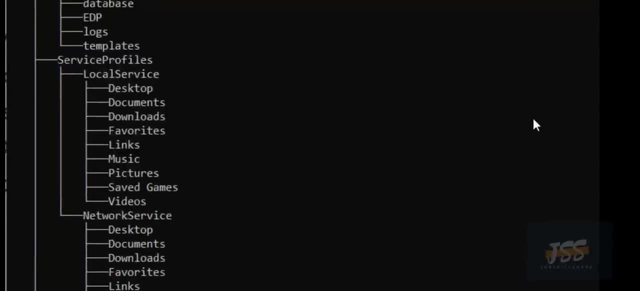 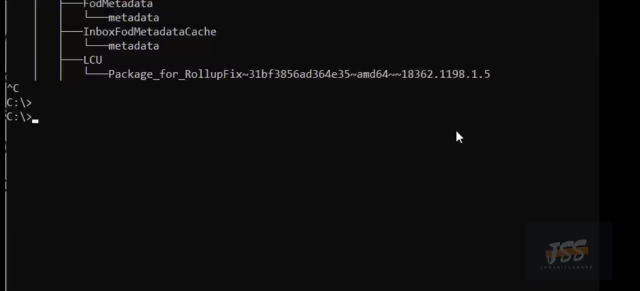 the tree, what we call so. in this way, you could easily use this command to know about the directories you have in your any folder or in any drive. now, after that, we have another command, and the command is simple: date. if you want to change the date of your 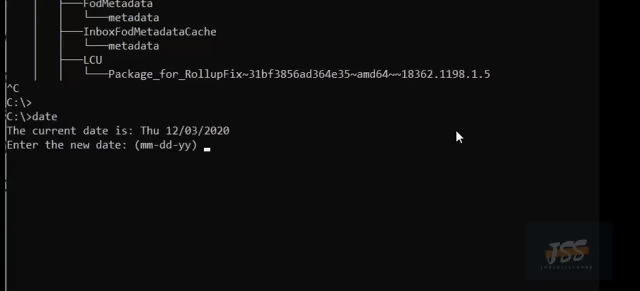 system. if you feeling that the date is change and it's not correct, so you can change, and if the days days dates it's already correct and you don't want to change that, then you can simply copy that provided day under this new provide it section so it will set this new date as the current date and in this way we have. 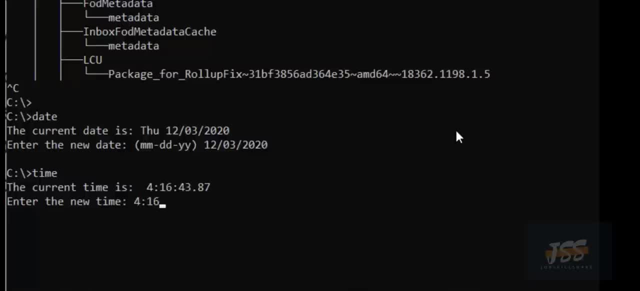 a similar command time. so if you feel that the time is not correct on your system, so you could change otherwise. if the time is right and really on your standard time base, so you could do that. so the time made new date is correct and could still maintain as given with that. so the time is scored back in the end. 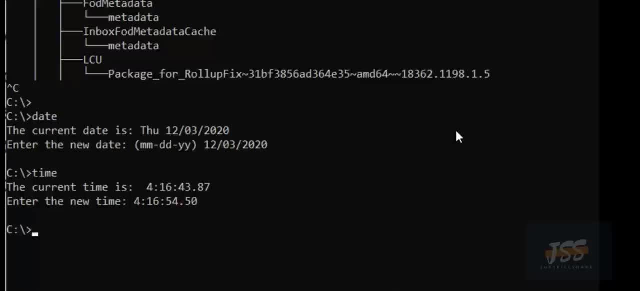 So the time is changing that way because most of the time when you're using your browsers and if the date and time is not correct, they start providing error and they stop working and the error is shown like that. The place must change your time and set according to your standard time. then this browser or internet will work. So in such situation you get stuck and you get in that mess where to open the time settings and you could open control panel and it definitely it will take time to reach on that specific window or GUI option. 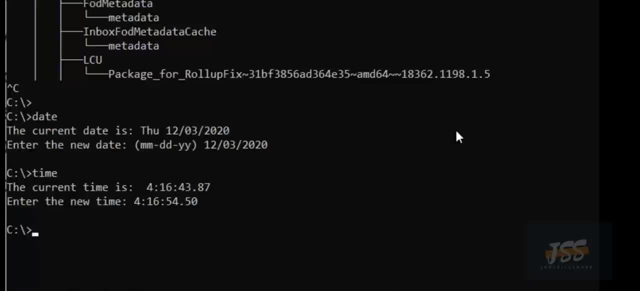 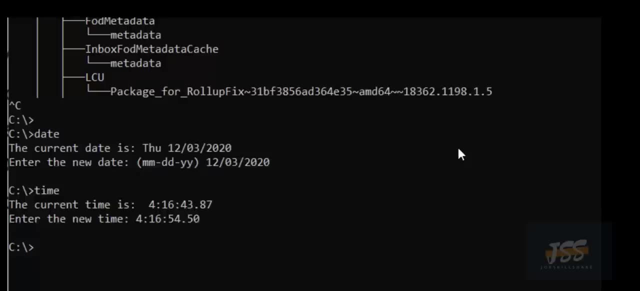 But here in the CMD you have basic commands- date and time- and in this way you would easily set the time and just set the time, Just update your date and time settings. So then after we have another command to check the history of previously executed command. let's say you run a lot of commands and somehow you missed any command, or you want to see the CMD, that which command I use before that command and that sort of things, and you want to be sure about all the commands that you executed or run. 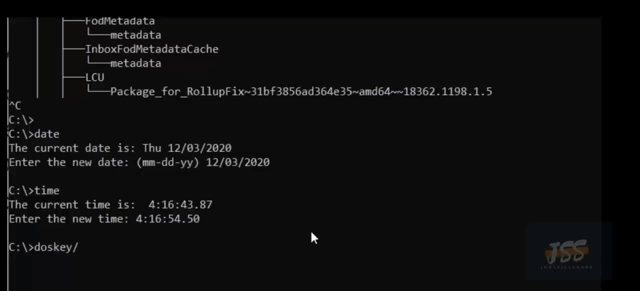 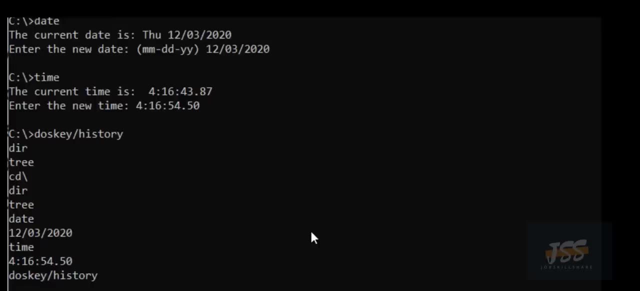 So there's a command- DOS key, Follow slash history, press enter so it can list for you all the command you want to see, you want to write down, you want to notice that all such commands that you executed will be displayed in a form of list and you could easily watch. and if you're creating any document, you're preparing any sort of file and history of the commands so you can prepare from that command. 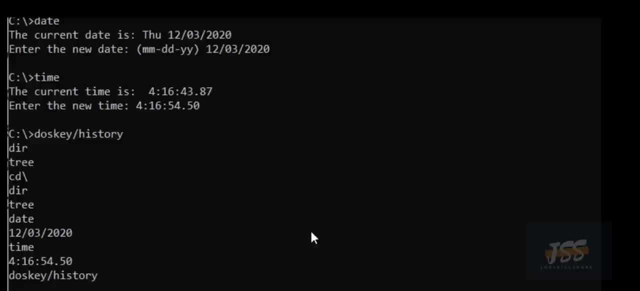 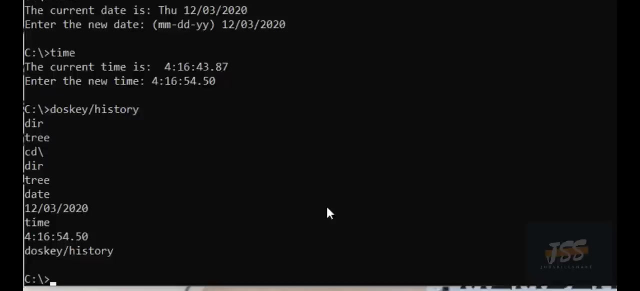 So it will help you to track your history. After that we have another command, and this is quite different and typical, because this command will shut down this machine. So it is related to turn off and power off the system, but there is some argument that you can add that make it more logical and more helpful. 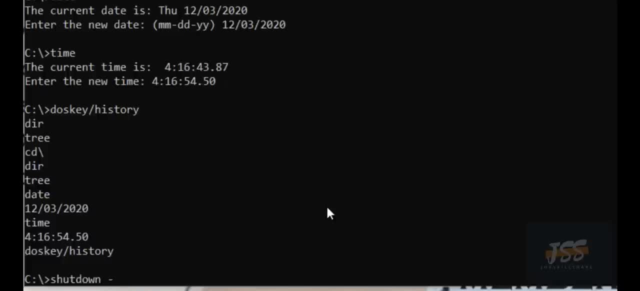 So the command is shut down. and if you press shut down dash S, So this Definitely means that you want to shut down your machine. but there is another argument you could add. here is dash T. So if you add this dash T, it will allow you to add seconds, that after what seconds you want to shut down your machine. 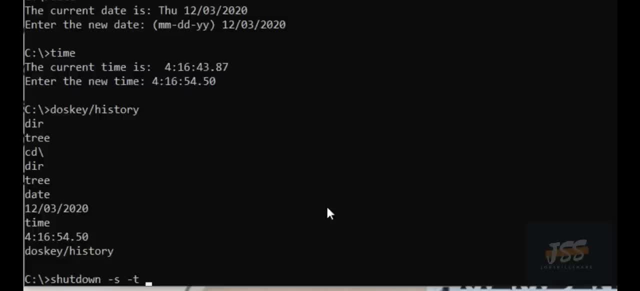 So you can add if you want, if you doesn't want to add any seconds, you just want a quick shutdown and an instant in an instant, So you can type double zero, So it will take no time to shut down your machine. But if you have planned something or you're leaving for something and the required timing for that installation- let's say, for example, you're deploying a software and it is providing the estimated time for that deployment- 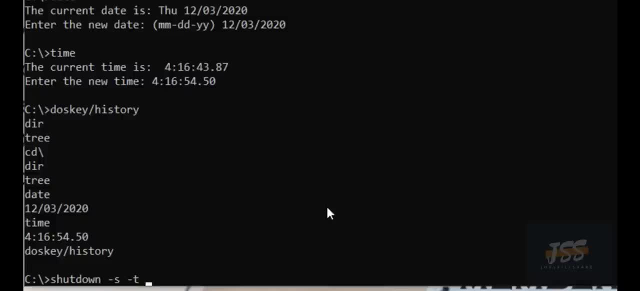 It is about 10 or 20 minutes and you know how much seconds in the 10 and 20 minutes. So then you can easily add some more time considering that estimated time and provide That seconds here in the form of seconds second unit. then what will happen after that time reach? the machine will go automatically shut down, and that's the best way to shut down your machine when you are from your desk. when you are not on your desk and you feel that I won't come on that specific time. 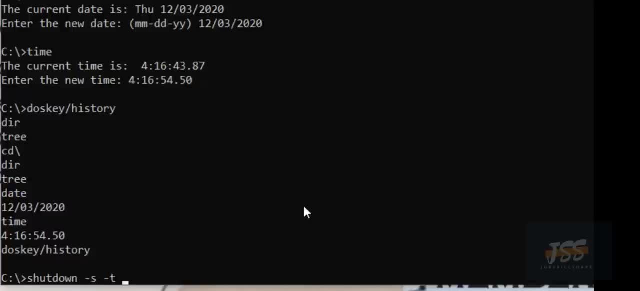 So once this whole deployment, whole process is done, my machine is supposed to be shut down. So in such cases you can use this command and add the timing to automatically shut down your machine. So I'm not going to do that because you know this will shut down my machine. 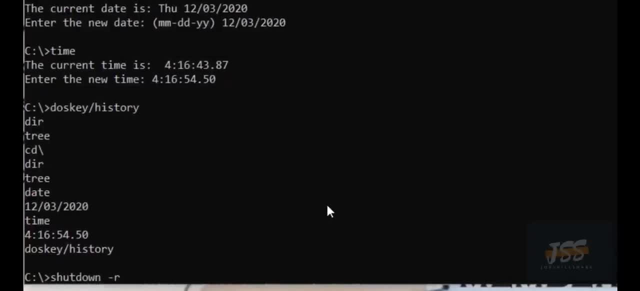 And in the same way you, if you add dash R, so it will restart your machine. in the same way, If you add time T for time and provide some seconds for restart, so it will do the same, but it won't shut down your machine. 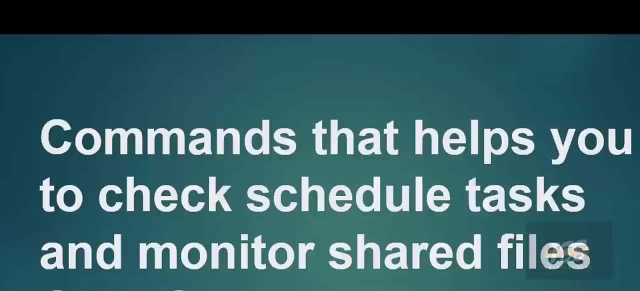 It will restart your machine. So video I'm going to cover some command that's help you to check schedule tasks, as well as your shared files- And most of the time you shared any folder and if you want to check and how many user at the real time using that file have access the file. 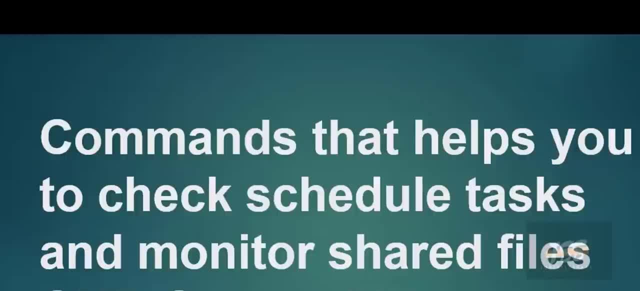 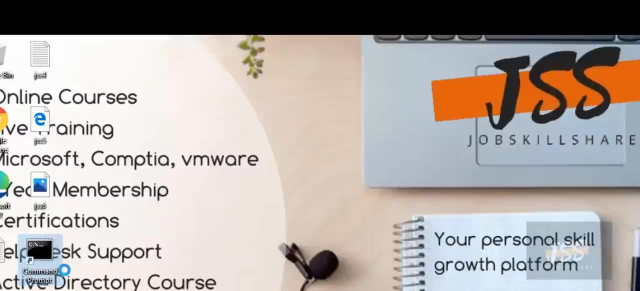 So we have some commands through you can easily monitor the status, that how many user at the real time are accessing the file, Accessing that specific file. So let's move to the Windows environment. Now here let's run the CMD with the administrator privilege. 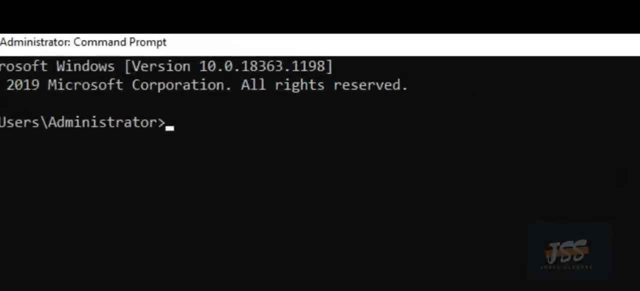 As you know. So here on the command prompt, the first command we're going to show here is check ntfs. So what's new in it? Most of the time you use the command chkdsk to check this, and it is very helpful. 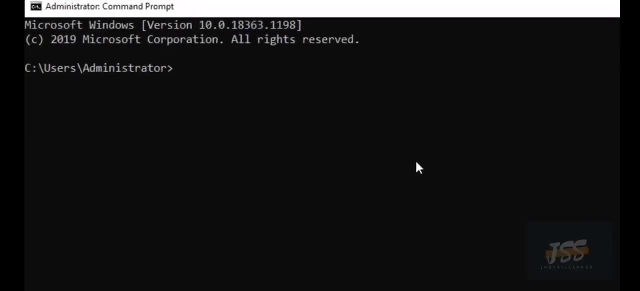 And use so many times and most of the it personal are known to that command. but there is another command where you're just changing this dsk to ntfs, so actually this command checks this file system, the ntfs file system. so the command is: chk ntfs enter. so here the thing you need to add after this: 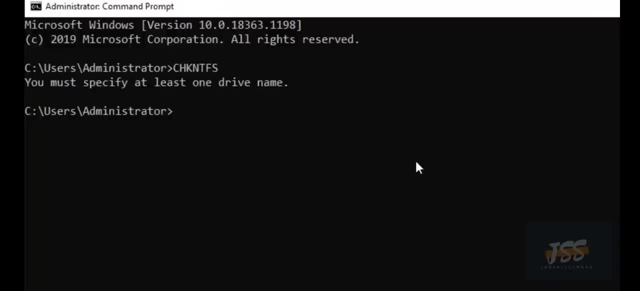 command, because in the chk dsk you mostly provide the drive letter. so in the same way you have to provide the drive letter, and this time it would be c for the testing purpose. and here you can see chk, ntfs, space c colon. so it is telling that this ntfs file system is correct and it's not dirty. 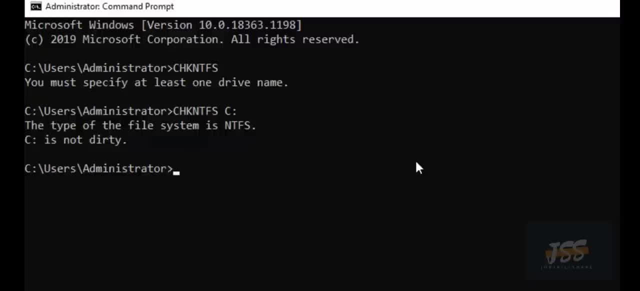 so the dirty means that it's working correctly and there is no any sort of issue and error regarding this file system on the c. so how you can see that here, how this output really helping you to totally judge the system file, and also you are monitoring and getting output about the status of the disk. now, after that, we have another command. 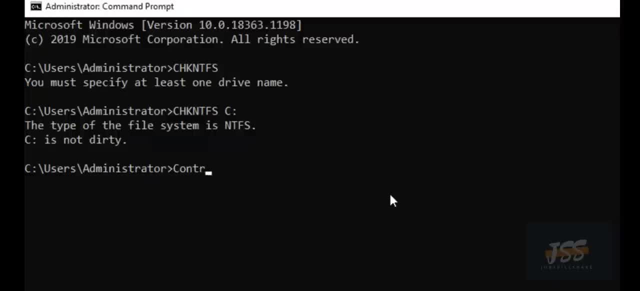 and this command really helps you to open the control panel. so if you want to open your control panel, for example, you can just open the control panel and it will show you the status of the disk from the command line. so you should type control and press enter. so what it will do? it will open the. 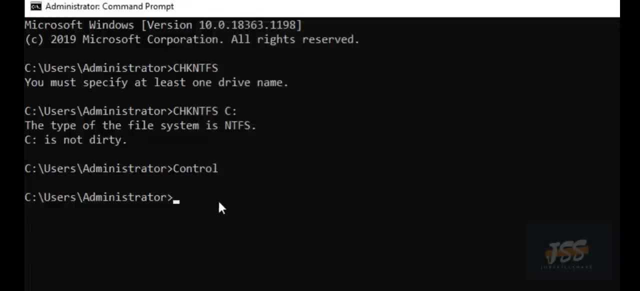 control panel on your gui. so most of the time if you are using command line and you have to do something in a quick way and you want to launch your control panel, so just type control in the command line and it will display the control panel in an instant and most of the time there are. 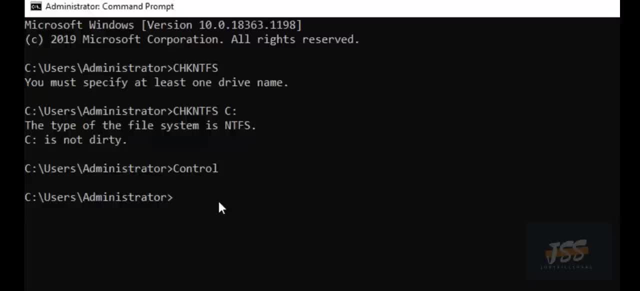 a lot of tools. we have the windows in the green environment in the control panel, so we have to access the control panel to fix those things, even to show, to view such sort of options. so for that purpose you can simply type control the command line and it will open the control panel. now the command is schedule. 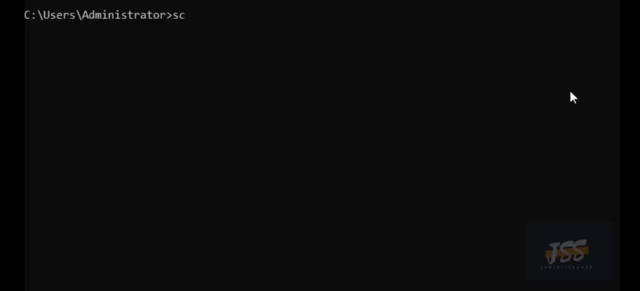 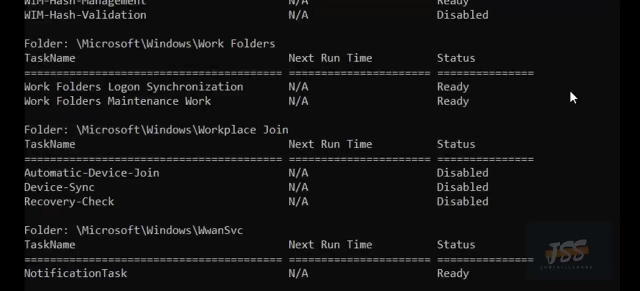 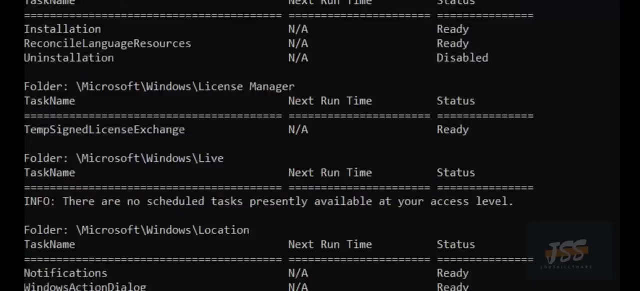 task and this command does what. it helps you to see and check and monitor all the tasks that had been scheduled in your windows operating system. and here you can see there are plenty of tasks here that are already scheduled in your windows environment and if you want to see those tasks in 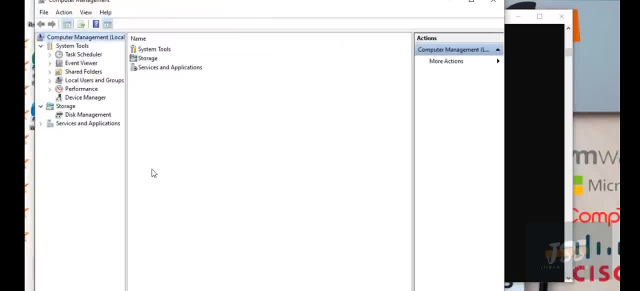 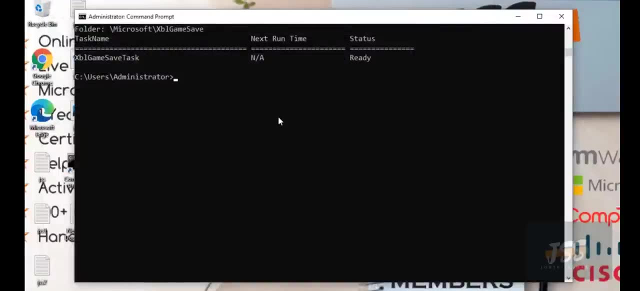 your gui, so you have to go to the computer management and here if you click to the task scheduler So it's going to display all the tasks here. But if you want to see all the tasks in the command line, so you should type the command schedule: tasks. 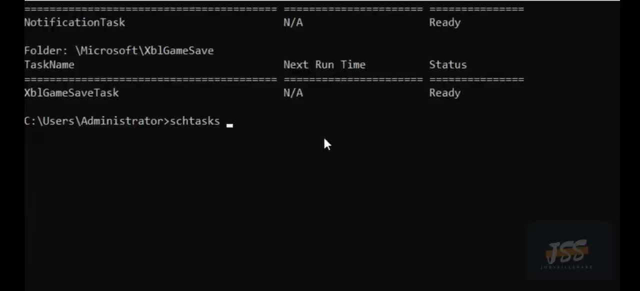 And what if you want to create a separate file where you want to export all the scheduled tasks? So you would write schedule tasks greater than sign and then name anything to that file and press enter So it will export all the tasks to that directory, so you can access that file and you will get all the list of the scheduled tasks in a separate file. 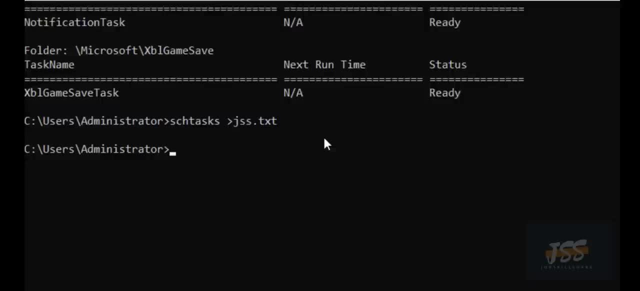 So that's the best thing it is offering in the command line: that you can easily export the list of all the scheduled tasks in a separate file. We have another command, ver, and, as the name suggests, as the short form suggests, the version command. 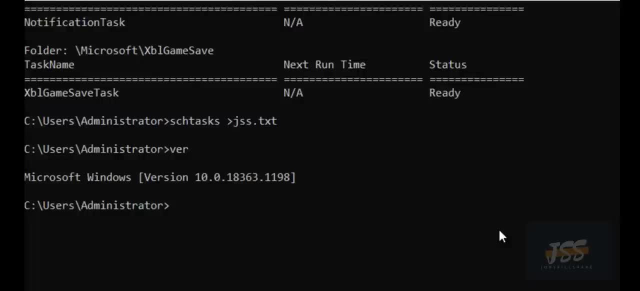 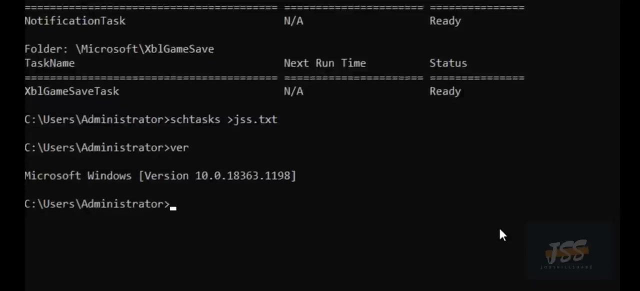 And it will tell. It will tell you that which Microsoft version is currently running in your machine. So you can easily in an instant, find out that which version is installed and deployed in your windows, in your currently in your machine. So you should type ver to find out that specific version of your operating system. 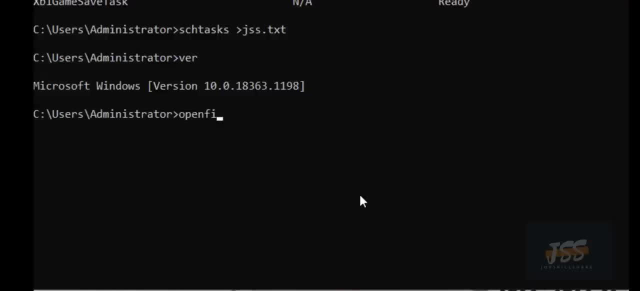 Now the last command of this video is open files. When you run this command, And so this command will tell you the current sharing. Let's say, for example, you created a folder and shared within your local network, right, And you want to see that how many users are currently using that file, right? 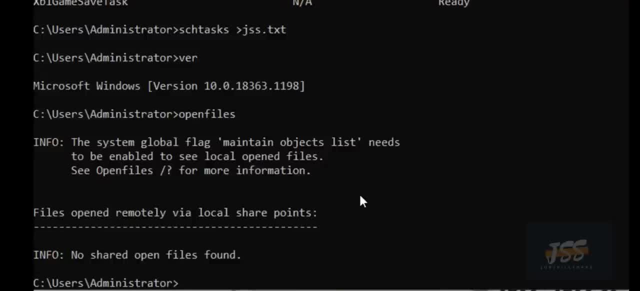 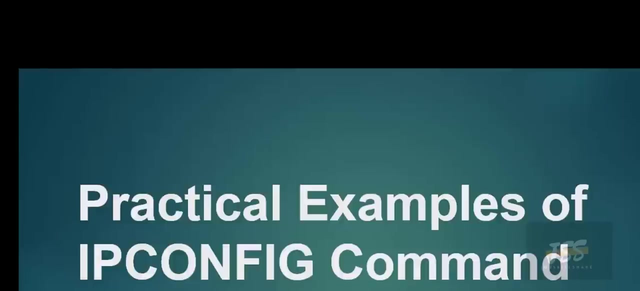 How many persons right now are accessing to that directory. So for that you can simply type open files and it will provide you the data and the user, Which are the number of users who are using that file currently in that output. Some practical examples of IP config command with other keywords that are mostly used as an ID help text, personal or with the IT support person. 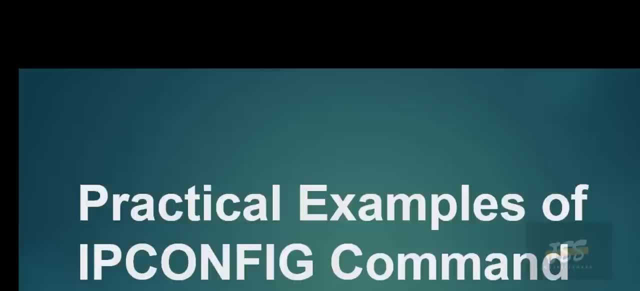 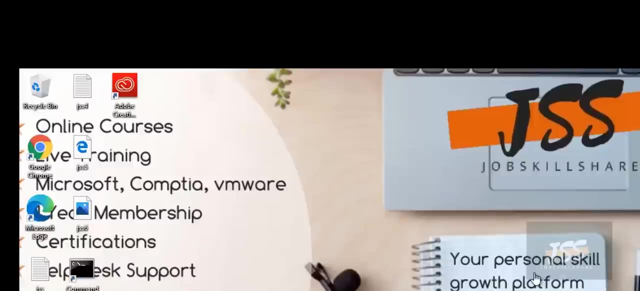 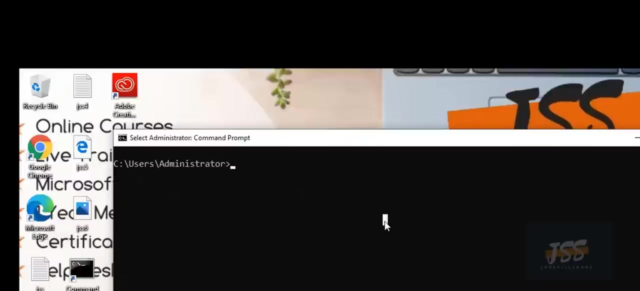 So we're going to show you all such examples in the command and the usage of IP config. So let's start the video, But before that, please subscribe Our channel and press the bell icon so you won't miss any update. Now here I have this Windows 10 machine, and let's open the command prompt that I already open for this video. 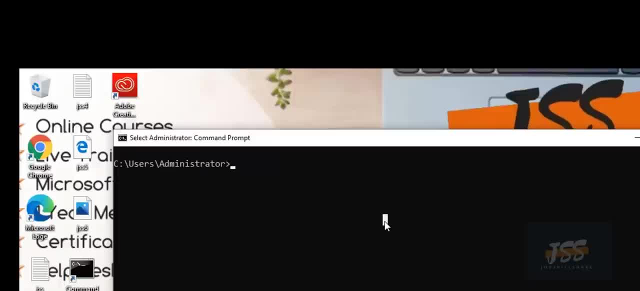 Now here let's say, for example, that you want to know about your network details and that with stuff- let's say the IP address- right, Or you are fixing any trouble that the system is Facing, like it is not getting Internet or there's no connectivity. 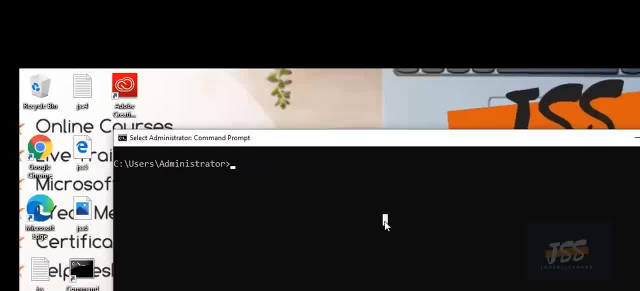 And in the first hand on the troubleshooting side. you must know the network configuration, whether the configuration is correct, whether the IP address is provided or being set. So all these network information you need to know And in most cases there might be some issue with the default gateway. 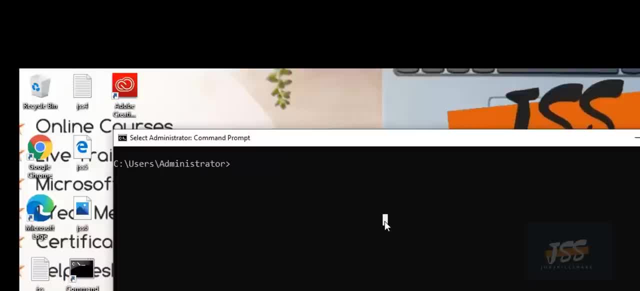 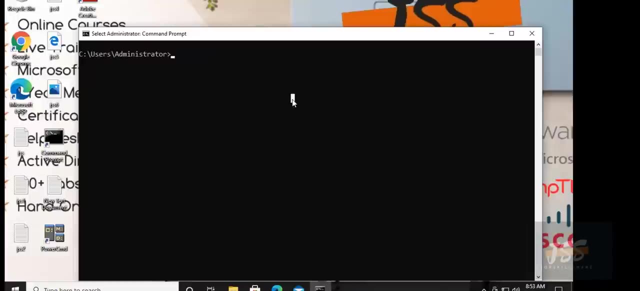 That's why the machine is not getting The Internet, the packet. the machine- Let's say this- is specific machine enabled to reach to the server, like the Google server. It is unable to do browsing And this is definitely happens when the machine doesn't have the default gateway. 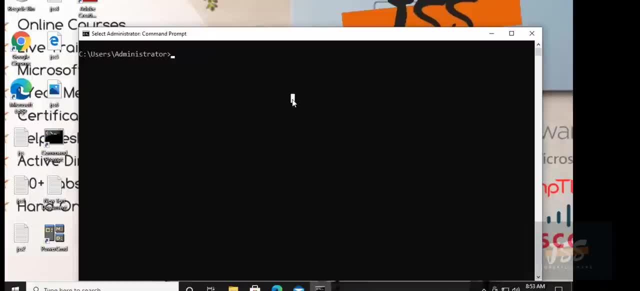 But how could you know that this machine having any correct IP address, or there might be some sort of default gateway- is not available. And there are some issues happen, Like in the organization where the computer are connected with the server. Sometimes the same IP is being leased to the same computer, to the one computer. 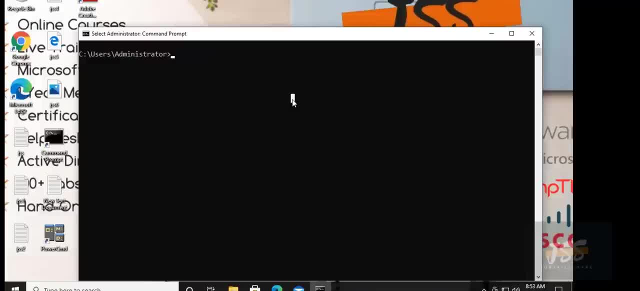 And then when this computer just turn off and another computer turn on, So it leases that IP to this new computer. So in that case when this previous computer turn on, there must be in. there is a kind Of IP conflict happen. So how could you know those information? 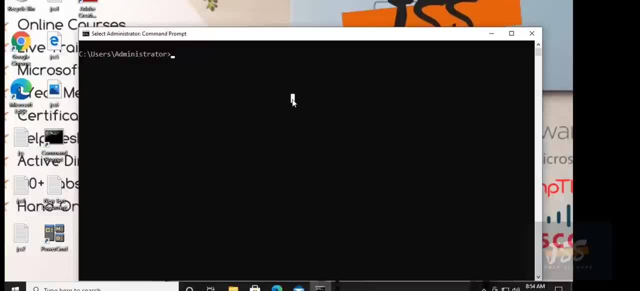 How could you gather and collect This input and then to process and just applied some your tools, some of your techniques to troubleshoot this issue? So all sort of basic details and investigation? You could start with the IP config command, So the best point you could remember. 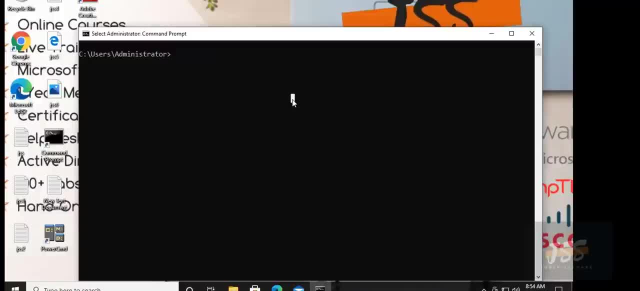 For practical example of IP config, that it is the initial and the first tool You should apply to investigate your network details and from this point you can even start your investigation. So let's start with some practical work. and these are all the practical examples. 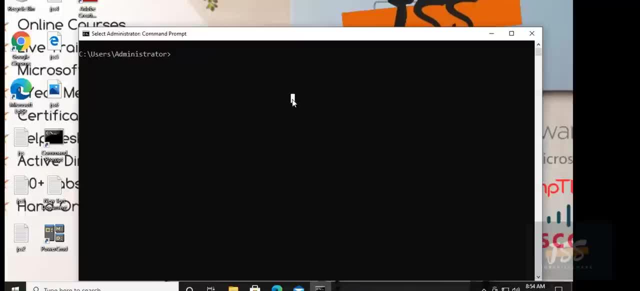 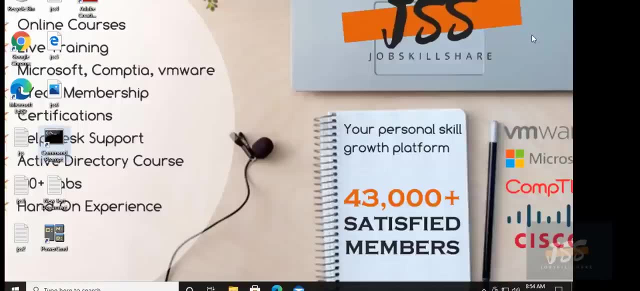 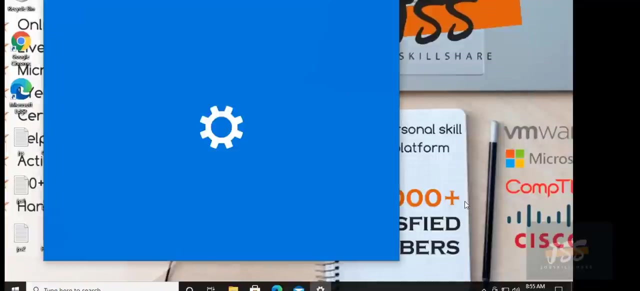 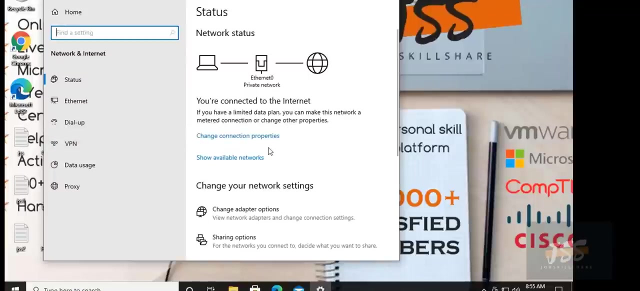 You could follow and apply in a different way with the environment or with the trouble. So right now, If I don't use IP config, Let's say, and if I want to know the network details of what should I have to do is just right click on the network and internet settings, then open this window where it contain the network details and that after detail, and definitely it takes a lot of clicks and a lot of windows to open, to reach to your exact location from you can collect information and you need to. 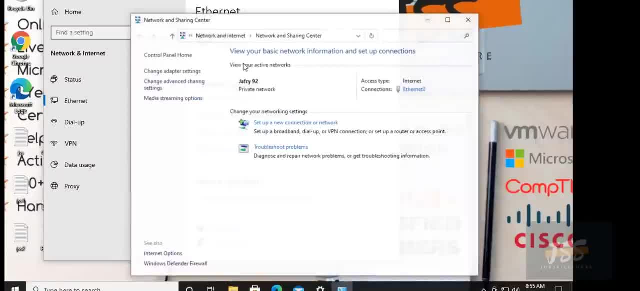 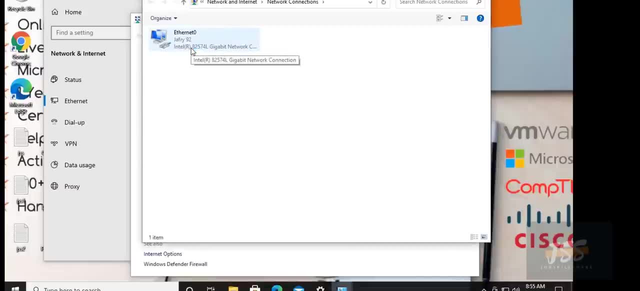 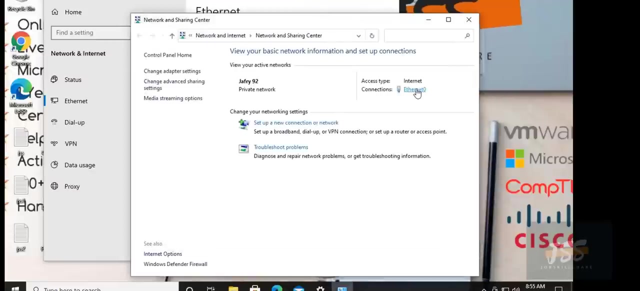 Just Go there to get the basic details. after getting this input, then you can realize that what should You need to apply here to troubleshoot this issue? so here what? what I did is just click to the, change it after settings and go to the doctor, or might be I can click to the doctor directly and it will show me this window that contain that. 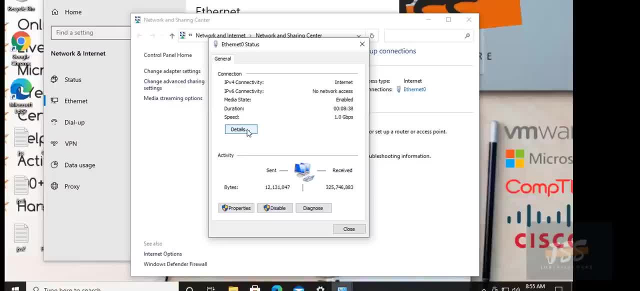 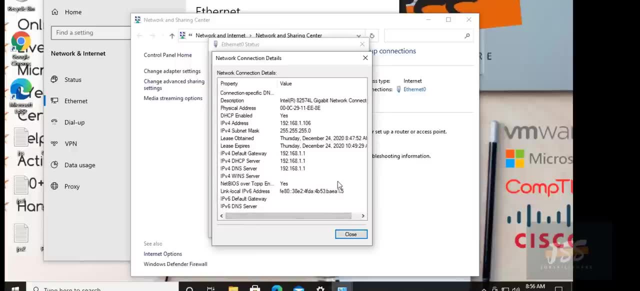 Adopters and the receiving and the send packets. so I click to the detail so I can easily get the details of The network parameters, like the IP address, subnet, the DSP server right, the DNS server and most of the important details I could find here, like the physical address. so here you can see that. 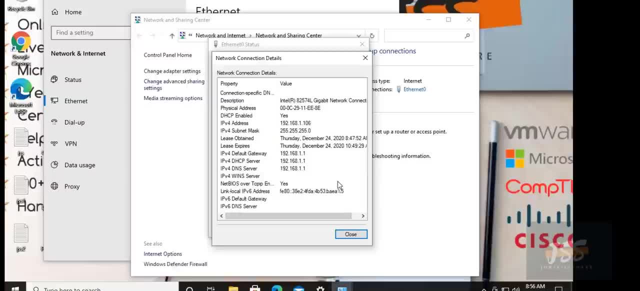 It takes a lot of steps and a lot of clicks and you need To Open certain windows and certain locations to get the details. but here you can see, you cannot transport this, all details, into a notepad file. all you need to do is to just 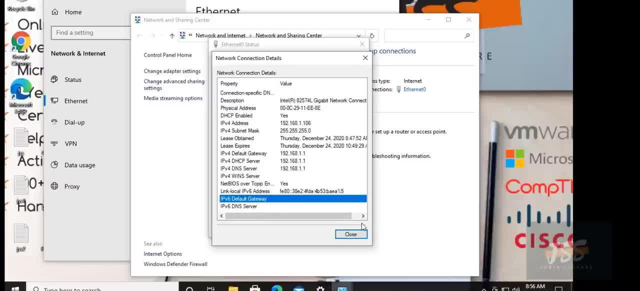 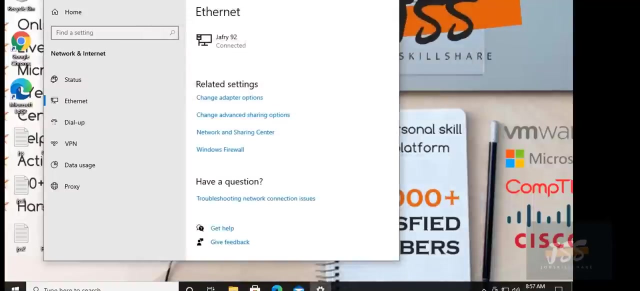 Close this one or you can take a screenshot. but if you are doing some kind of documentation and you want to transport and you want to create a separate file, so you, if you want To export the all details that you collect on any system, so the command line is the best to do this, to do so. so let me close these windows and show you the IP config command and its uses. so here's the command. 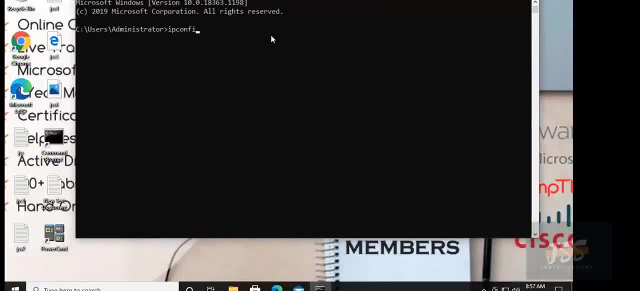 Prom and if I type IP config here, Press enter, so immediately you will. in the first look You can easily realize that how many adopters you have in your system. so sometimes adapter were Hided in your network and sharing center. let's say, if I open it again for you to just make sure that how this IP config command is useful to. 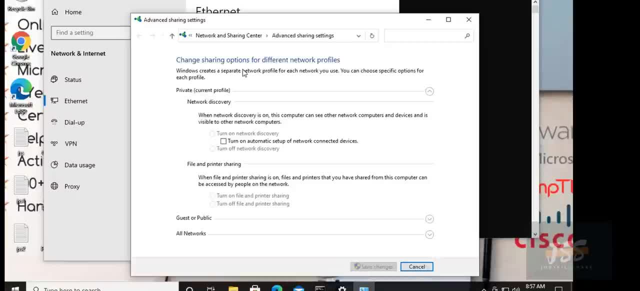 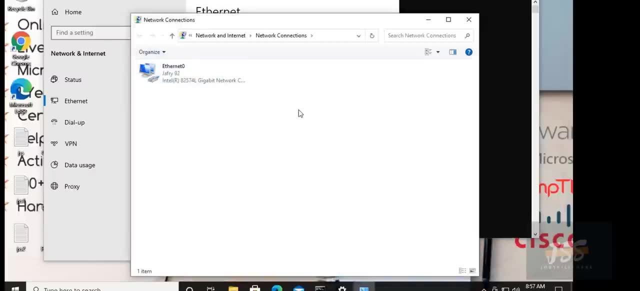 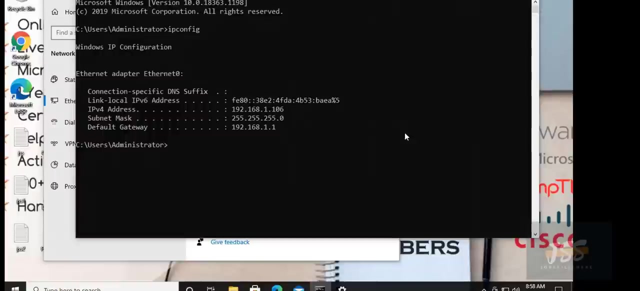 Collect information about your adopters, about your network parameters. so if I click here and open the Adopter settings, change that after Option, sometimes that after were hide, and you enable to see that how many adopters are working and are attached to this same machine. but by using this IP config command it will list down all the adopters that are currently working, so it will not. 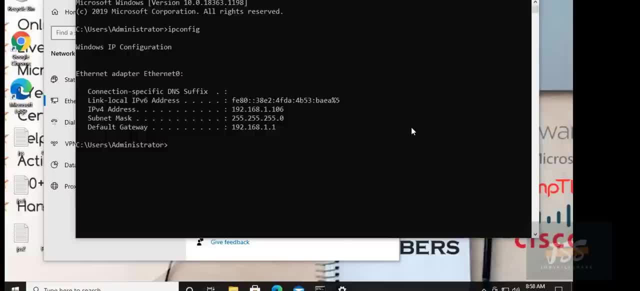 Just hide all those adopter that might be hidden due to any sort of settings or windows General Behavior. in the response, somehow some files got hidden in the operating system. when? but the best thing in the CMD that whenever the file is not available in the GUI, in the graphical user interface, you can still 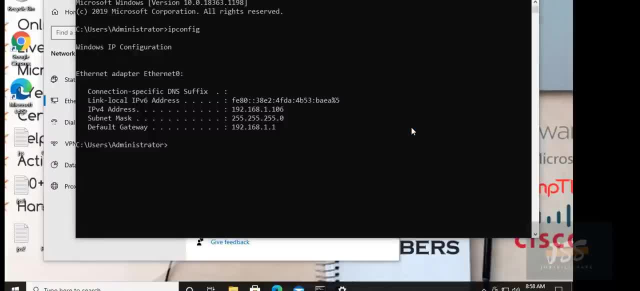 See that file, access that file, and it must be visible because you're using the CMD, but there are certain commands you could use to hide those files. Now, here in the first look, you are getting the information about The number of adopters you have. so right now we have this single one, Ethernet adopter Ethernet 0. so Ethernet 0 is the adopter name. 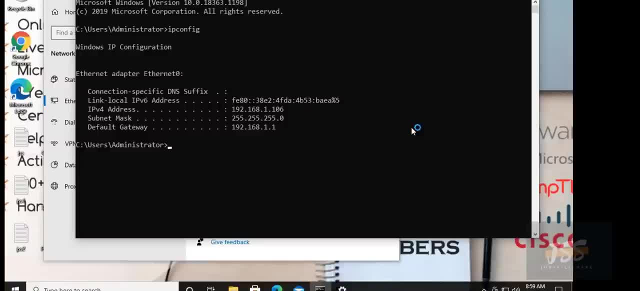 And the second thing you are getting is your IP address, your subnet, in the default gateway. so it is providing you little detail, but it is useful somehow, and from this IP config command, without any keyword and argument, you can easily assess That this machine Have the IP address, it have the default gateway. so that's the best part of this command. 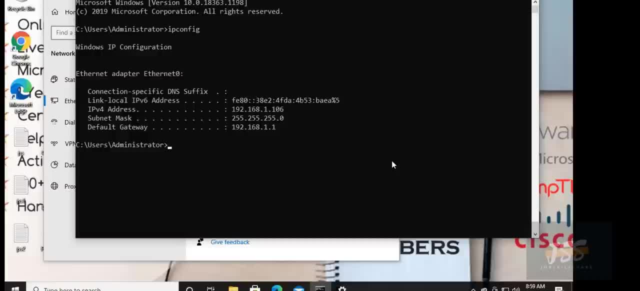 But In contrast, you unable to find out the DHCP setting, the DHCP server, DNS server, your physical address, that after MAC address. so this command actually telling you the network detail, but not In brief, it is just Pieces of information of your network. So if you want to collect the whole detail and like if you want to know the DNS address, the DHCP server address, whether the DHCP is working or not, because this command is not itself. 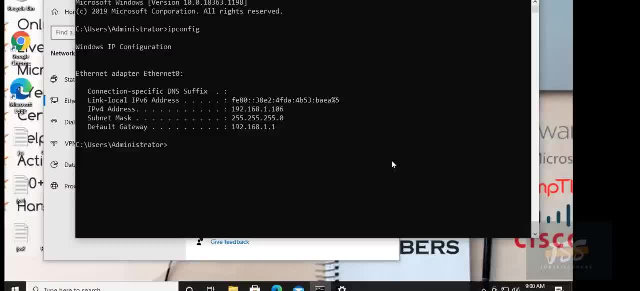 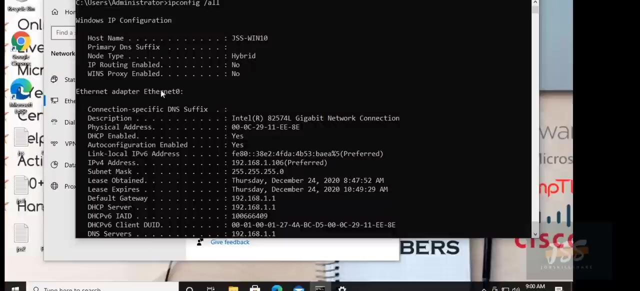 Capable of providing the DHCP server detail, like whether the DHCP server is working or not, or the IP is set manually or dynamically, like automatically. So for that you need to run another command In the IP config Space: forward, slash all, And once you press enter, so definitely you have the single adapter working here and by pressing, by pressing these keys and executing this command. 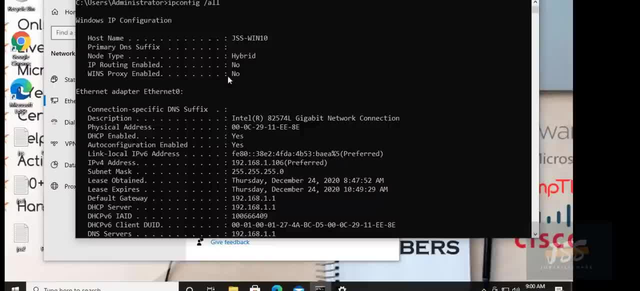 In a glance you will see This output and if you start from top to bottom, so first you will see the host name, the machine name, and here you can see that the details are More Explored and in a Huge way, like you're getting. 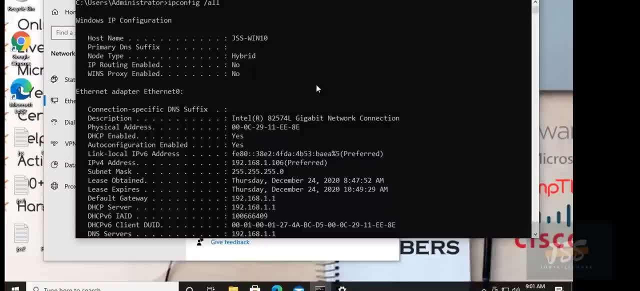 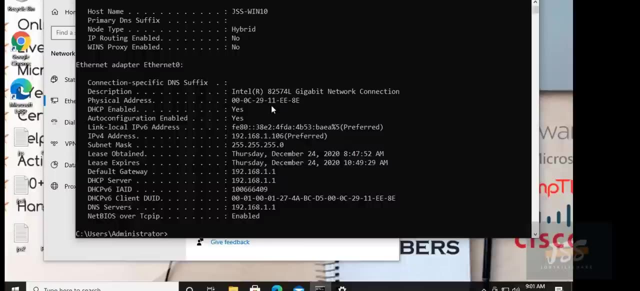 Bunch of details, Unlike with this, with this just IP config command. so on the top you have the host name, so with this command you could easily know the host name and then Description that contains the adopted name and the physical address, your MAC address, and this is different with each adapter. 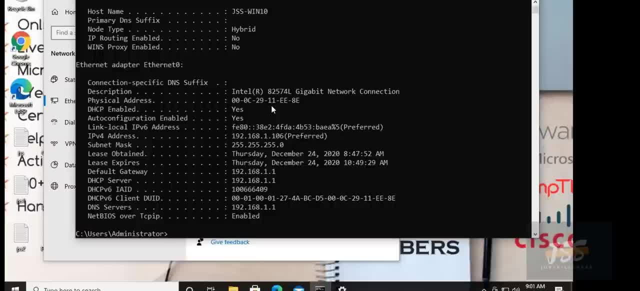 So currently you need to just Make sure that you are on the correct adapter that is providing you the internet connection, So you will get the adapter detail once you scroll down to the each adapter. so currently there is one. That's why we are getting this output related to that one specific adapter. 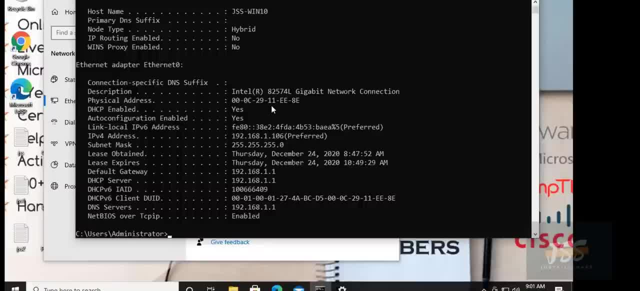 Then another line that contain the DHCP enabled. that is yes, so it is Straightforward and quickly telling you that your DHCP is enabled And this machine Receive the IP with the DHCP server. Then you have the IPV6 addressing detail than the IPV4 in the subnet mask and the interesting part is it is telling about the lease time. 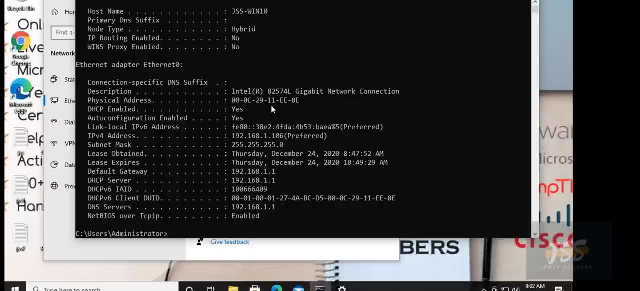 And also the lease expires in the default gateway and also it is telling about the DHCP server in the DNS server too. So all you have, all the details you have, All are required and helpful to assess and start your investigation from this point. Let's say your user complains that the use I'm, my machine, is not getting IP address. 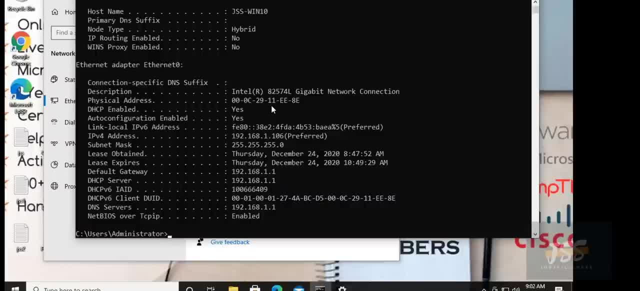 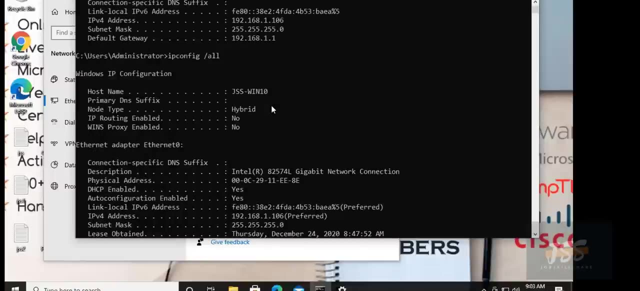 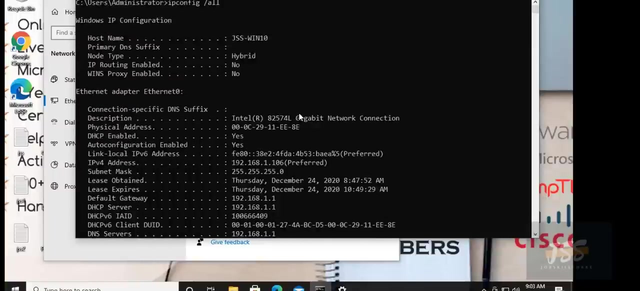 So what should you have to do is just run this IP config command and first check whether this machine getting an IP address. And let's say, if you type IP, IP config and you didn't get any IP address, Let's say You get answer, you get, the output is 169 and that's something. it means that this machine didn't get any IP address. so 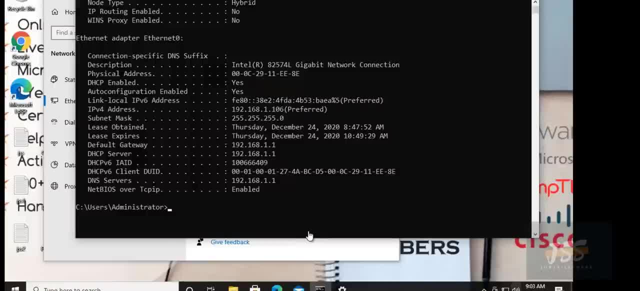 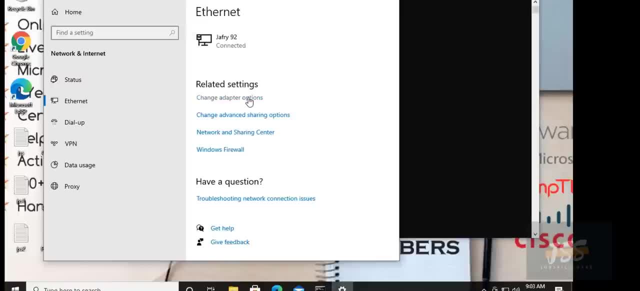 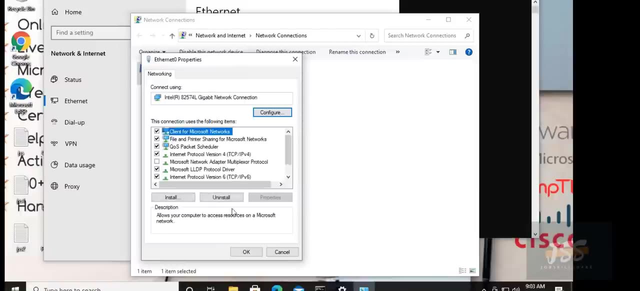 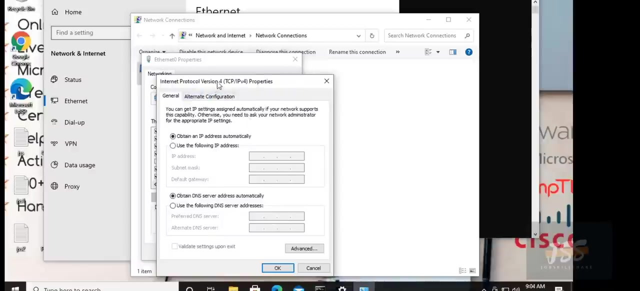 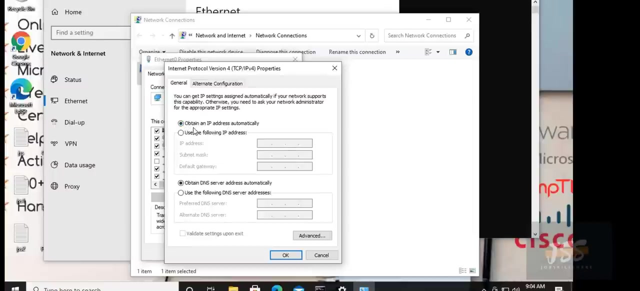 That could be the best way to determine whether this machine is getting IP from the DHCP. but in contrast, if we go to the GUI and if you want to know that, whether this machine is Getting IP Address from the DHCP, so you have to do so many steps and you have to open so many dial up boxes to know whether this machine is getting IP address automatically. so if you open this dial up box and in this window you can see the check is made on opt in and IP address automatically. so here it is telling that the DHCP is working. but here in the command line there's a straightforward answer. 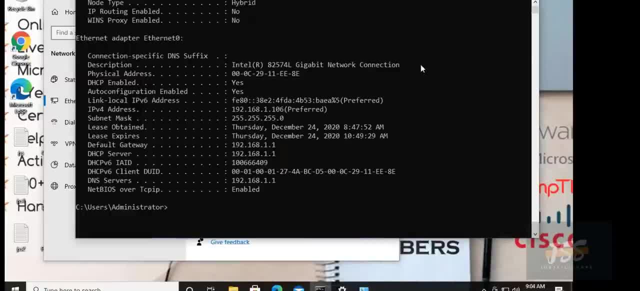 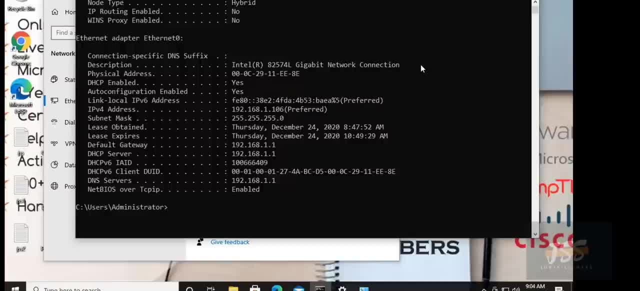 So this is the best part of the IP config: forward slash all command. Provide you a direct answer. Then the least thing and the DHCP server. also, you can locate the DHCP server from here and find out which DHCPServer is working, And also: 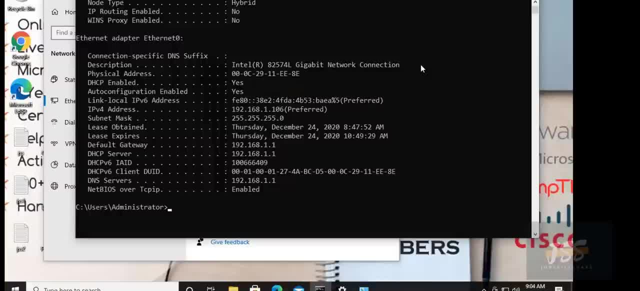 You are getting the DNS server detail And In The next video I will tell you about How to find out the IP address of your computer fqdn of the dnn server. this is the topic of another video, so i'm not starting this topic. 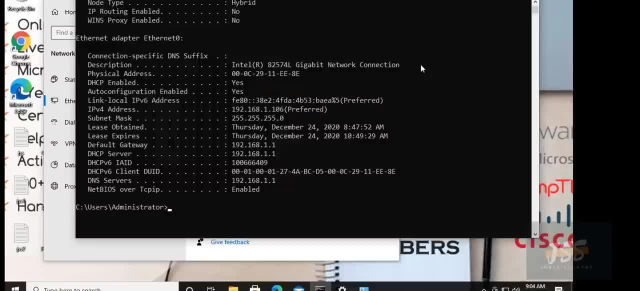 right now. so how this ipconfig space forward, slash all command is helping in troubleshooting issues, that you are getting enough detail in the beginning to investigate the problem, that, whether the problem is with the machine or with the other part of network- that might be the router or switch. so after getting this basic detail you can analyze and you can assure yourself. 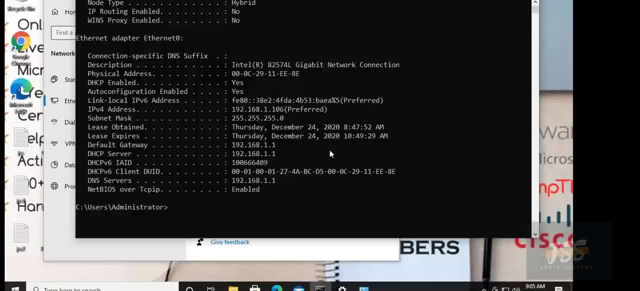 and you can done that. this machine is perfect. everything is configured correctly. so there might be some issue with the cable right or with the other network devices, like the switch or like the router. so you can easily confirm yourself at this point by getting this output, like: if the dhcp is enabled, if the ip address is correct, if the dns server 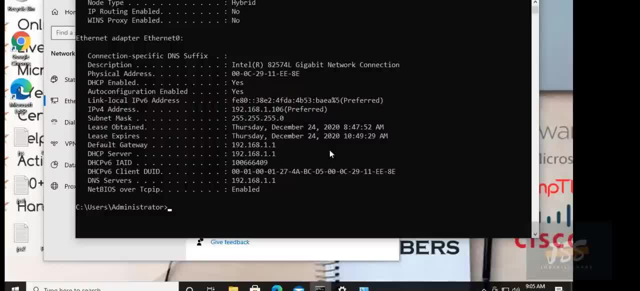 if the dhcp server, the default gateway, all are correct, all are the one that you provide or you set in your dhcp server, then you could easily assure yourself that everything is working good here. so definitely there must be some issue with the other network devices or with the cable. 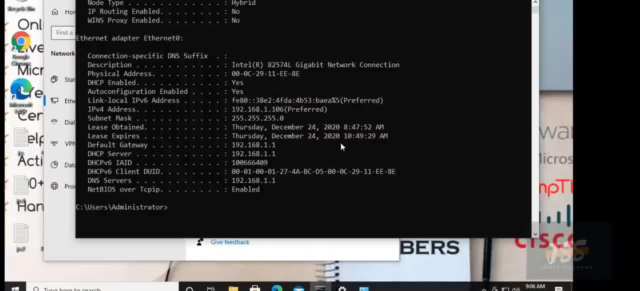 nonetheless, i'm going to add some keywords with the ipconfig to show you other options and other sort of function of this command. let's say if you want to renew the ip or if the user calls you and asks that i'm getting this dhcp conflict issue in my machine. so if you, 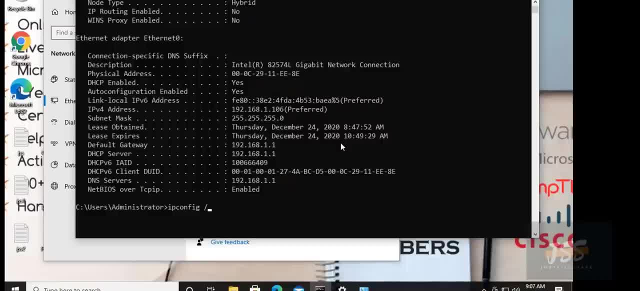 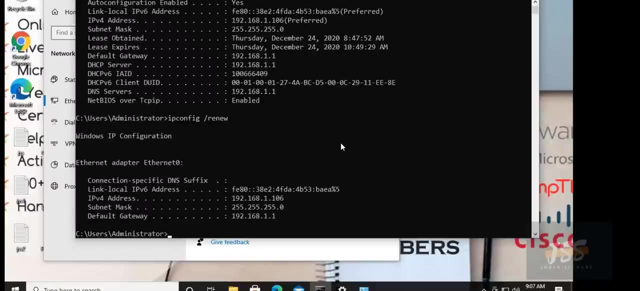 want to fix this issue remotely so you can take the remote or you can tell the user that go to the cmd and type ipconfig, space, forward, slash, renew. so what this command does? it just refresh the ip. or just made another query to the dhcp server that just refresh my ip. so if 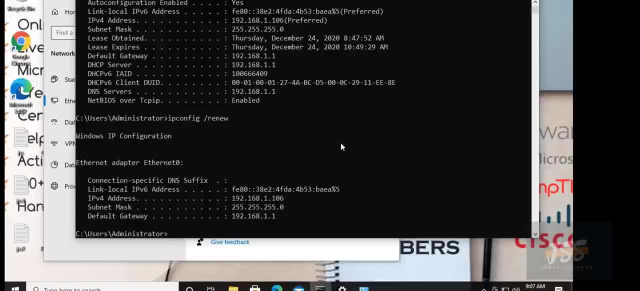 the ip is in conflict on the dcp server, that in the same time ip goes to the two machine and if if there is a conflict, so it will resolve and it will totally refresh the dhcp server, refresh the ip for use. right now there's no conflict. so it returned the same ip back to this. 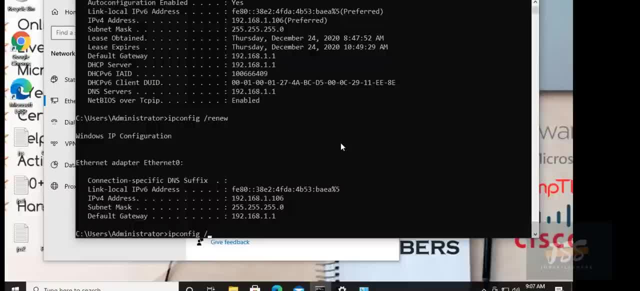 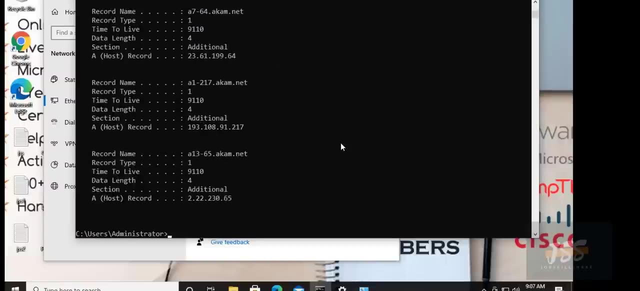 machine. then another command and that you use, and somehow you may require that command to execute, is a display dns. so once you execute this command it will tell you all the dns that are used or might be used in the dhcp server. so if you want to make contact with those dns or if the machine, let's say, 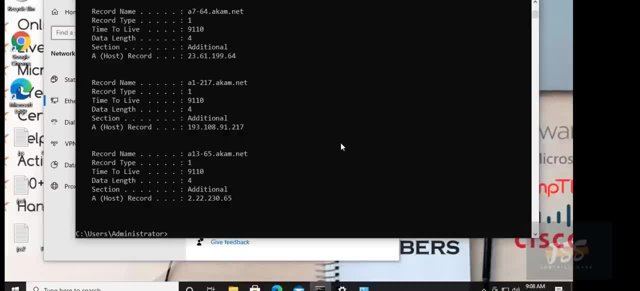 for example, you want to know that this client machine is doing what. let's say you get a complaint or you just saw some sort of threats and malware and some sort of. you found some sort of downloading right. you got some report about that machine, that this machine is doing some. 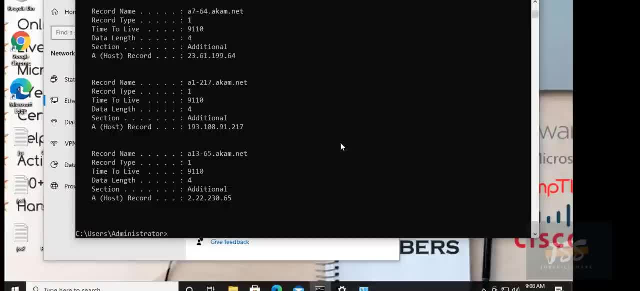 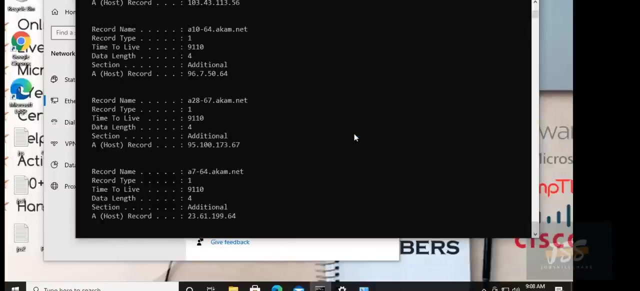 activities and you want to know that on which web server this machine is connecting or which other web server are in contact with that specific node in specific client. so you could run this ip config space for display dns so it will tell you all the dns details. in the past it just contained. 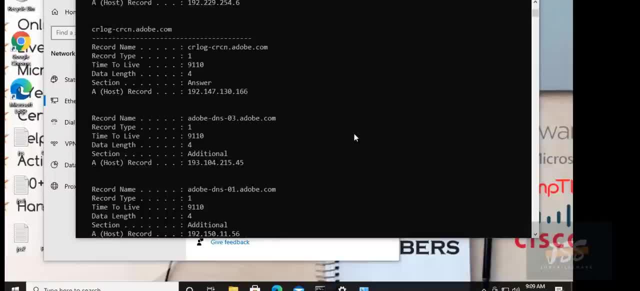 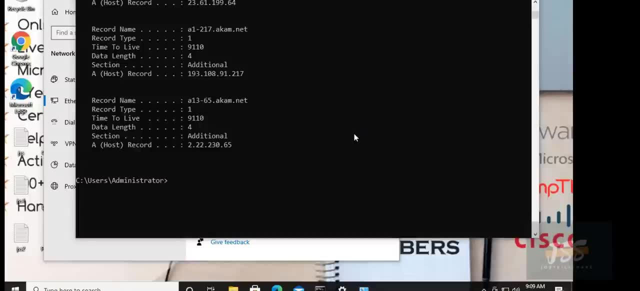 the history of the dns that were and that provided the exact web server location where this client machine had connection. so in this way you can judge and you can specify that definitely this machine is doing some malicious activities. so this command is really helpful to find out the dns connection and if somehow 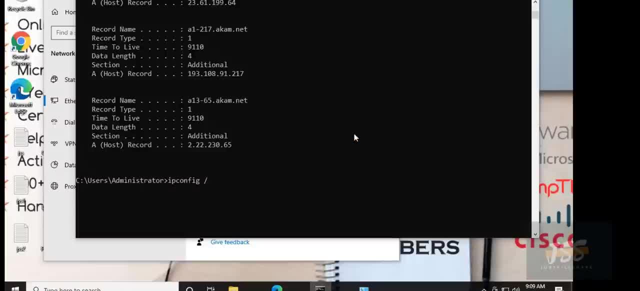 your client is unable to contact with the web server, with your dns server. let's say your client is unable to get the details from the dns server right. or if the client is unable to, let's say if he opened some file with the administrator privilege and he's typing his password, his account name, but didn't. 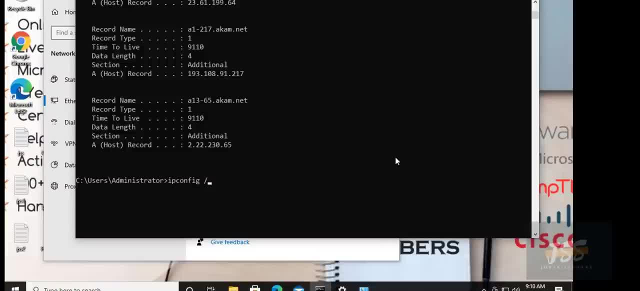 getting any response from there and there's sort of error like the dns issues or other sort of, for example, if the client is trying to ping or share file with another web server, another server within the network, and there is no connectivity with that location. so there's a command: flush dns, and if you type this command so it will do what it will. 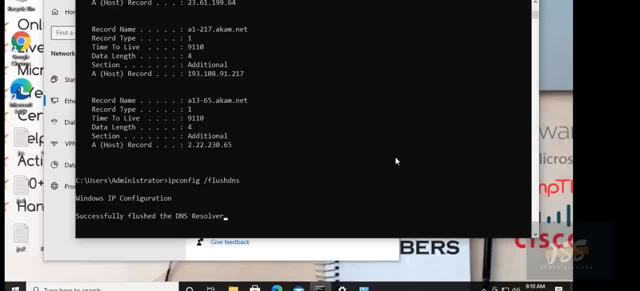 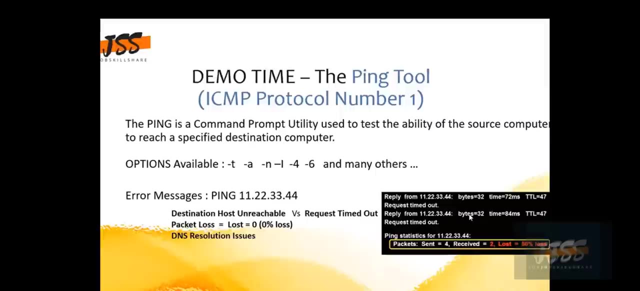 flush the dns cache and just refresh the whole dns cache and it will just refresh the whole dns cache activity and definitely this dns related issues would be resolved. so this you know, uh, just don't take this. uh like the simplicity of this tool. uh, we use this even in the cci labs. this is uh the. 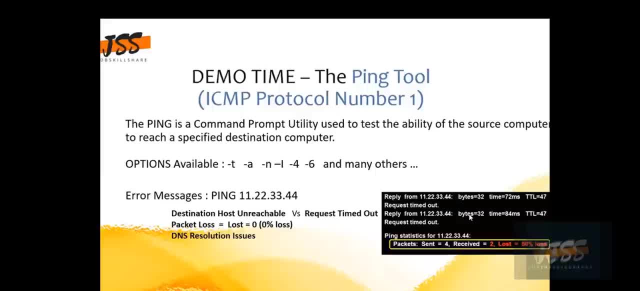 basic tools, but very important to consider, to be a very important tool in our networking environment and as a network administrator. personally, i have been using ping tool all the time. all day long i'm using ping. so, uh, let's talk about a little bit about the ping tool, then we will hit the lab. 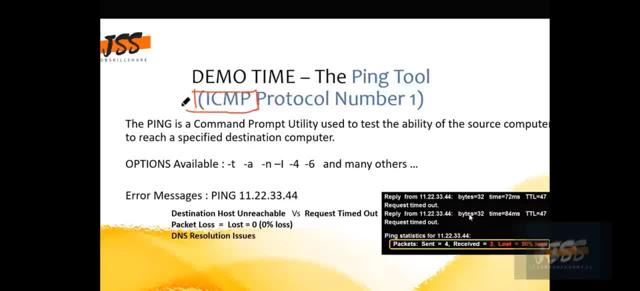 it comes under the protocol called icmp, because we are going to check the reachability of this icmp protocol. the ping is a command prompt utility used to test the ability of the source computer to reach the destination. so let's suppose we have two computers connected with each other. 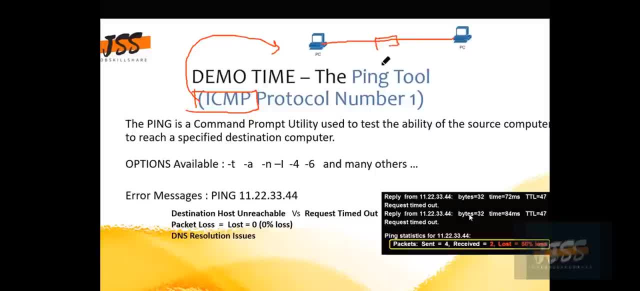 with any mode. i have no idea whether it's route or whatever, and they have some kind of ip addresses. i want to see whether this computer, this one, is alive or not. this computer is there on my network or not. this could be the pc, this could be my server, this could be even my access point, because all devices have some kind of 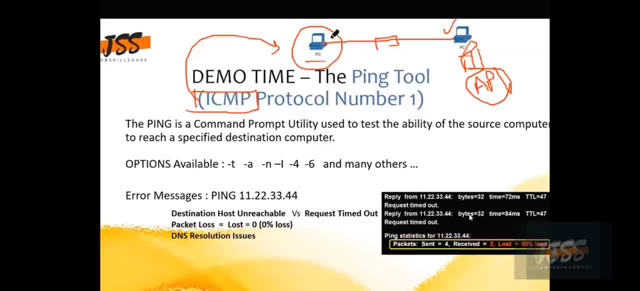 identification, which is ip. so, with the help of ping tool, i am just going to hit this device with a ping tool and this device is going to give me a reply back saying that i am alive. so this is how, instead of going to that computer that is maybe some far away in a floor two, and you 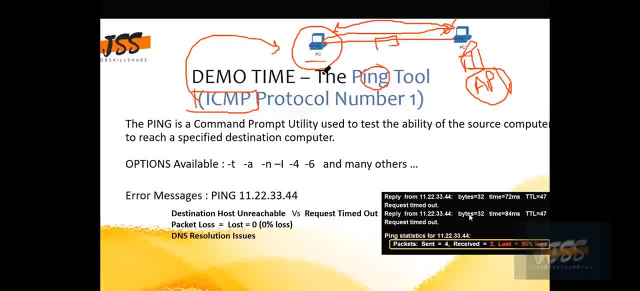 are in a floor one instead of. i will go into the computer and i will see everything is working fine in that computer. uh, this computer is on or not? i just try to ping that computers directly from my floor one and if i receive the reach abilities mean that computer is alive. 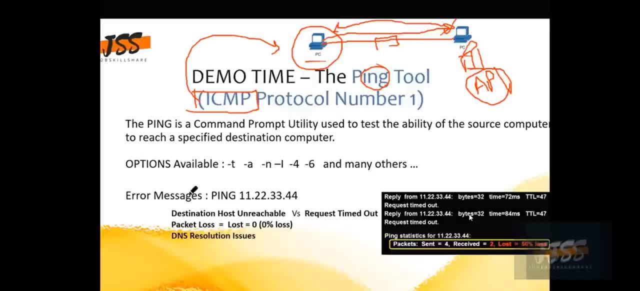 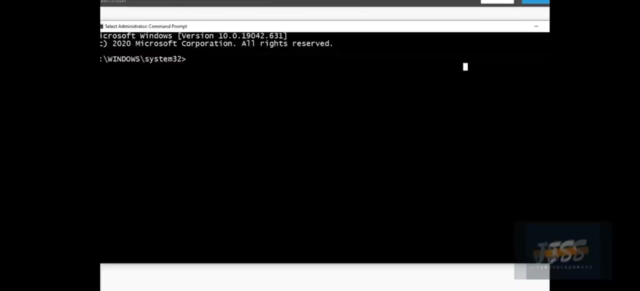 it has some options available. we will discuss a lot in detail in this demo and we will talk when we will hit these options. let's go to the demo and then we will talk about these error messages, leather this. then this will make sense. so i hope everybody is familiar with uh, the setup of the computer, ideal, and now we'll talk about. 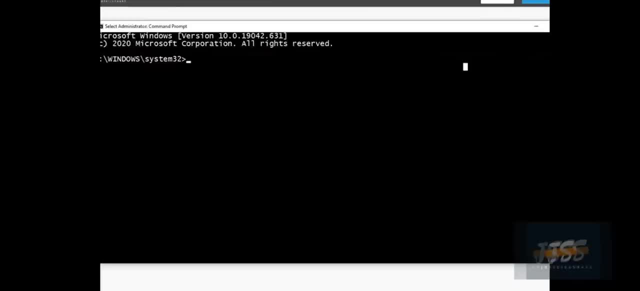 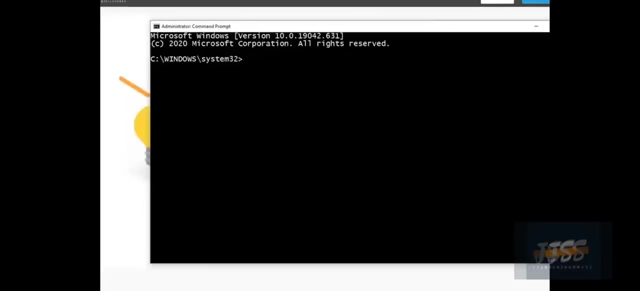 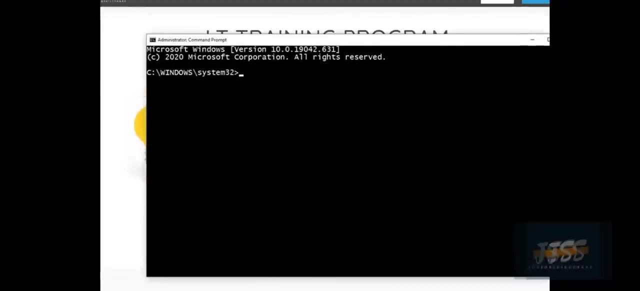 this domain: static model. we haven't done that a lot, but the whole idea of auto disparities and then this particularcamera are originally the command prompt. what is it? yes, it is. it is pre-installed in your windows machines, and even in the linux as well. um, in the linux we sometimes call it shell or console. uh, and in windows 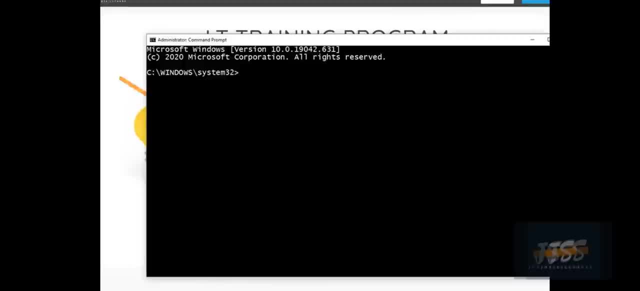 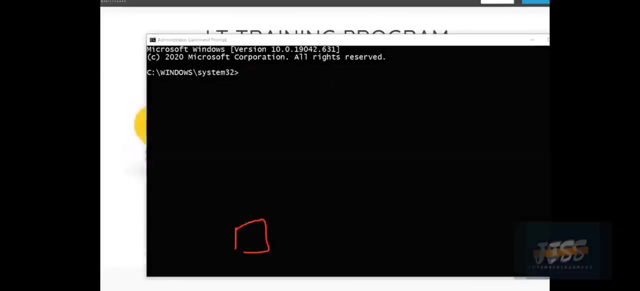 environment. we call it a command prompt. if you type on your search bar and type command prompt, or just type cmd, you will find this black console kind of application. just click on that, okay. so, um, first of all i give you the scenario. i have my device, which is connected on ip 192 168.100.3. 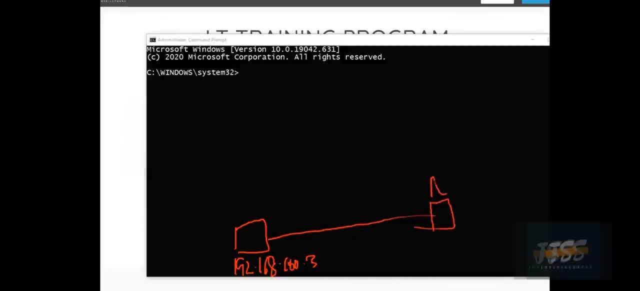 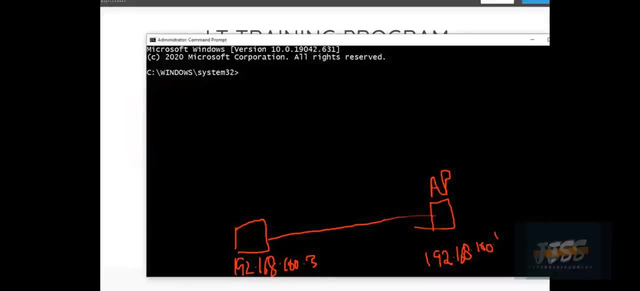 then for this demo i'm using my access point or the modem which is connected at 192 168 100.1. so let's try pinging my access point first of all, so i want to see end-to-end reachability type ping, then the ip address of the device which is in question, which is my access point. 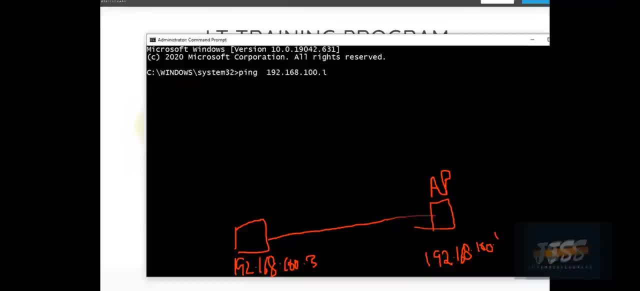 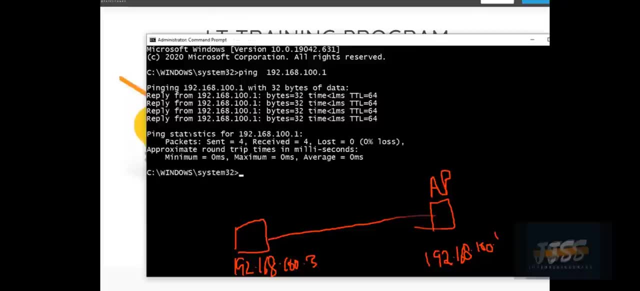 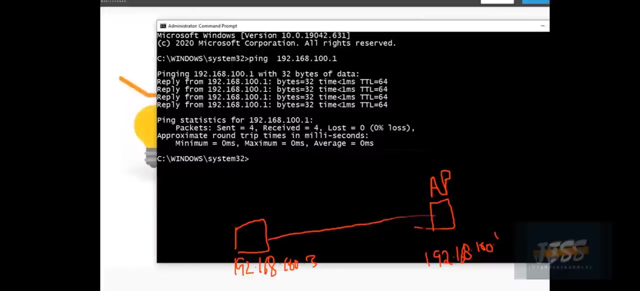 so, type 192, 168, 100.1, which is the address of my access point, and click, as you can see, we it will generate uh, one, two, three, four replies, basically saying your access point is alive and it is giving me reply, so i have reachability. and to end with the access point, 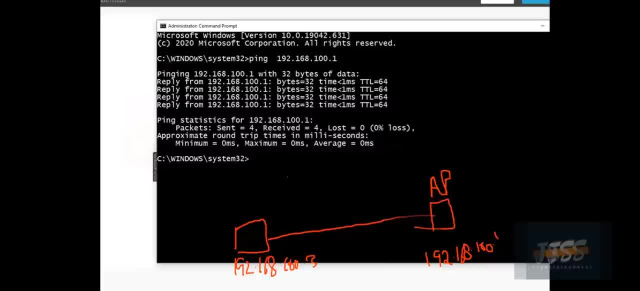 in the same fashion, if you have 100 devices attached in your local area network and you want to see the reachability, you can just do pinging all these devices one by one- one, two, three, four to check the connectivity. then, if i want to go a lot in detail, what else ping can do. 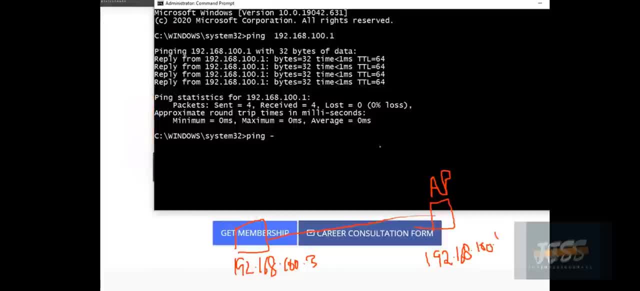 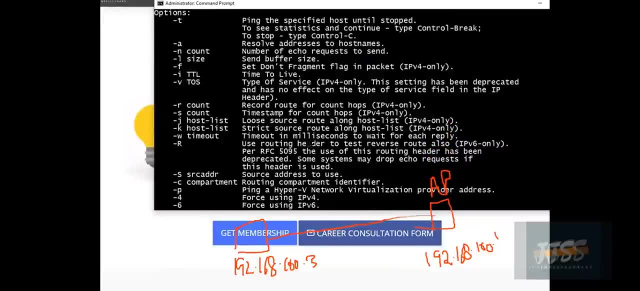 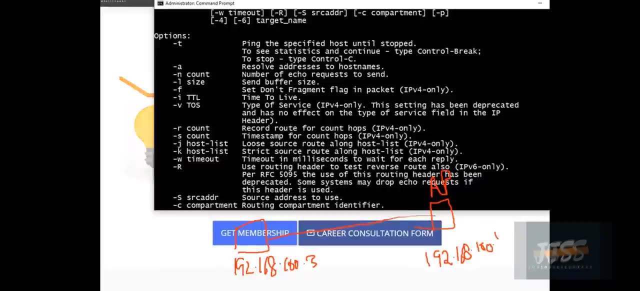 just type ping, then hyphen or minus with a question mark and hit enter. it is going to show me another option. what else i can do with this ping. come on, as it is mentioned, minus t. let's see what it does. so i am not going to go all a lot. 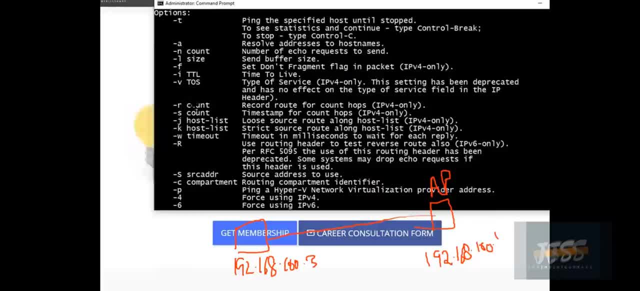 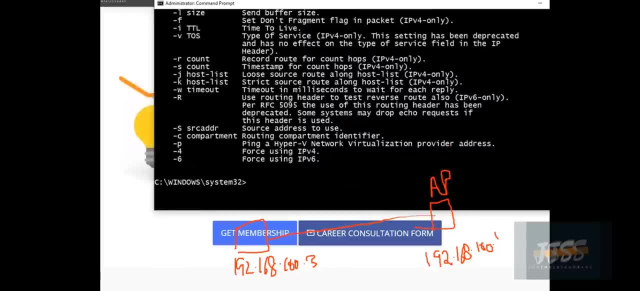 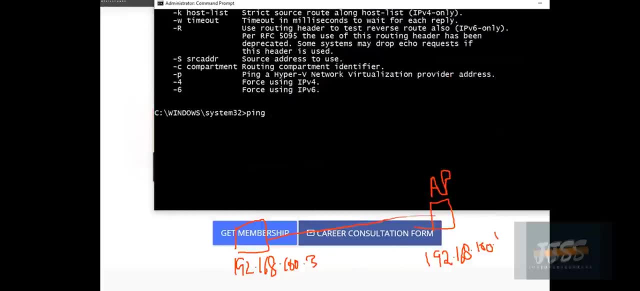 in detail about, with all everything, what it is doing, but just the important options that we most often use in our working environment, like minus t. if i ping the same, my access point device, with the help of option minus t and type 192.163.100.1 and hit enter before my reply stopped at the fourth. 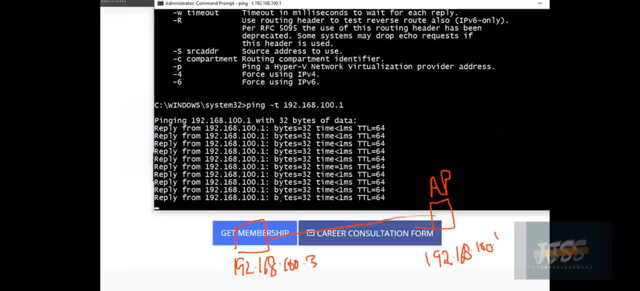 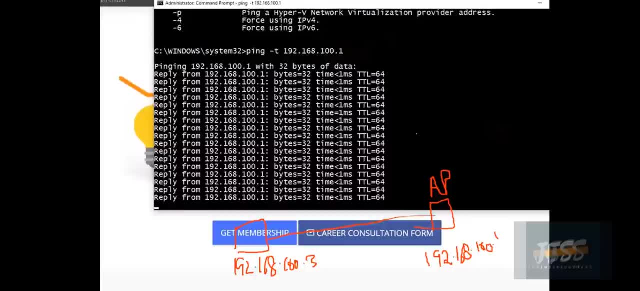 point. but now, as you can see, it is on and on and on. it is just keep pinging that device. why we need this minus t option? because we want to keep, because this is giving me a reply, but sometime it happens, some device is not not giving me reply. if it is not giving a reply, 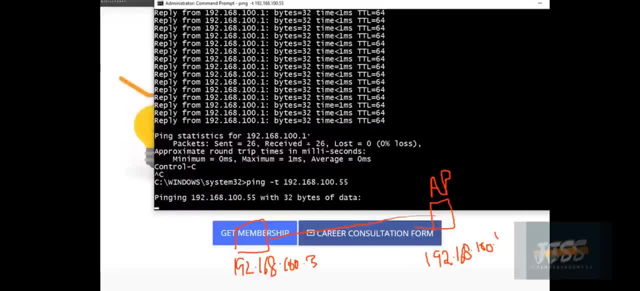 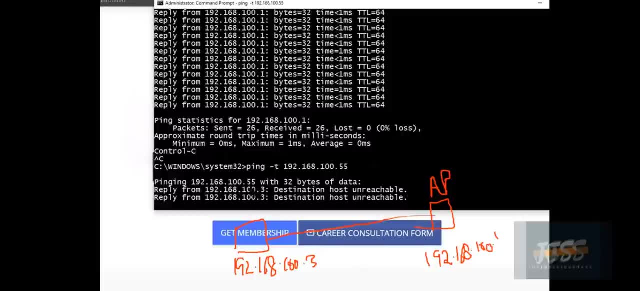 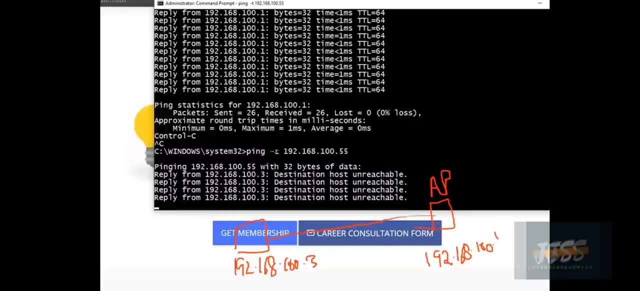 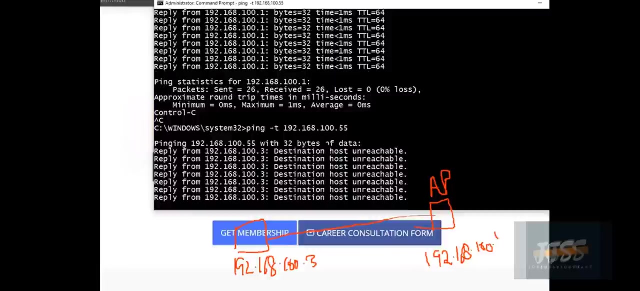 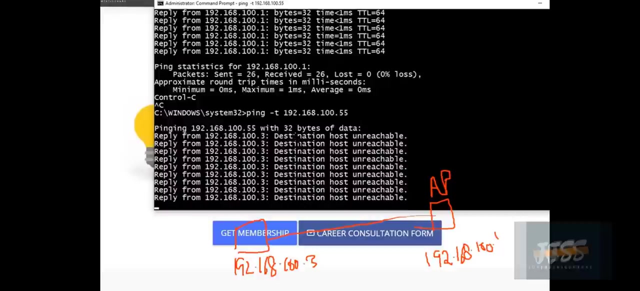 it will be like this: let's suppose we have 55. now you can see reply from this device saying destination host unreachable. so it means this is unreachable. now, with the help of minus t, i kept my uh, this ping, uh on control continue. so you know. so i just kept continue my ping. so why? because then i will go to the another. 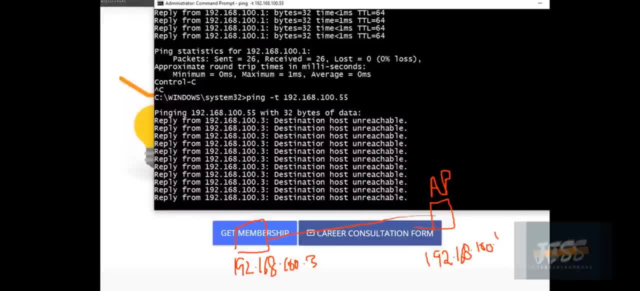 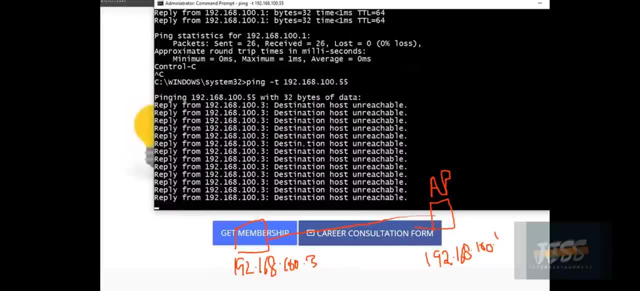 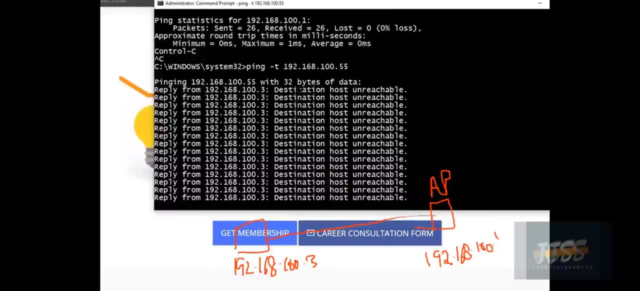 device which is not giving me reply, i will try to find the solution and as soon as i will start to see the replies coming from that device, it means it is: uh, there is end-to-end connectivity. so that's why we keep minus the options that will just keep pinging that device all the time. 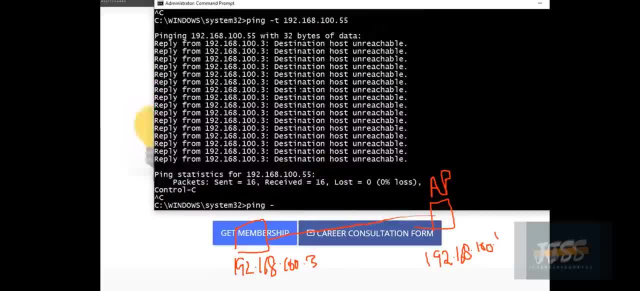 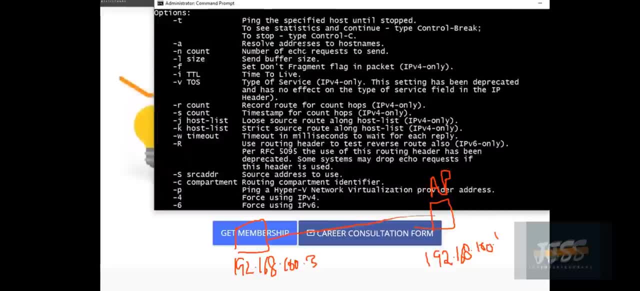 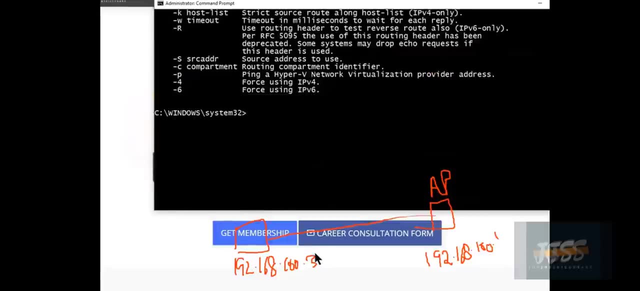 then we have some another option: type: minus and question mark. then we have minus a resolved address to post name. first of all i try to ping my own computer, which is on 192 168, 100.3, so it is give me, giving me a very simple reply and i have some another option. 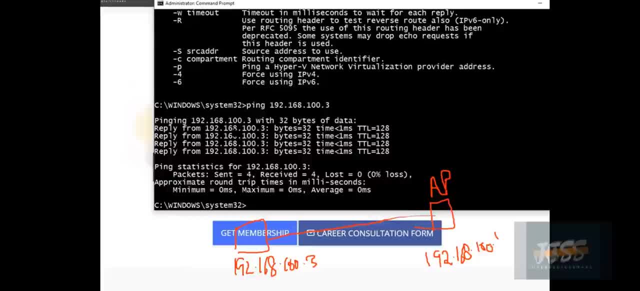 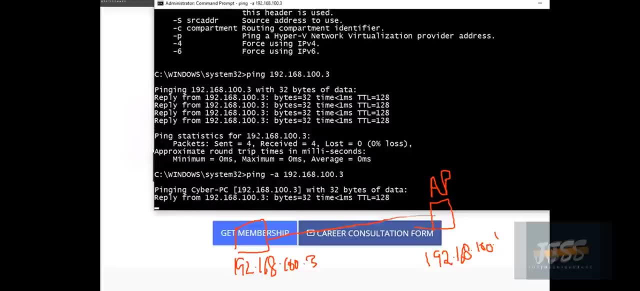 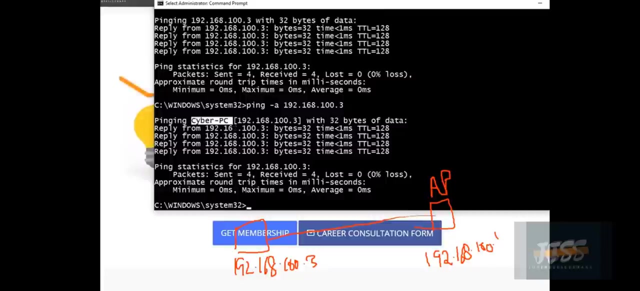 and i i'm totally blind at this time. i have no idea this reply is coming from which device? what is the name of device? because we know these devices by name. so, minus a option basically going to give me the information about the pc as well. so the name of my computer is cyber pc. so just by looking at this name, 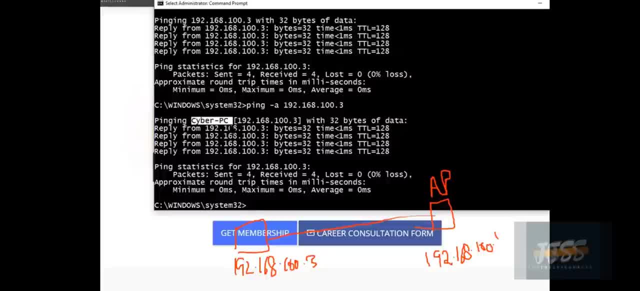 i will know that. okay, this computer, this belongs to this, so you can have like in a real production environment. let's suppose you have four or five servers, uh in your uh it closet, and then you can ping those devices, but you have no idea what that server is for. let's suppose one server is running. 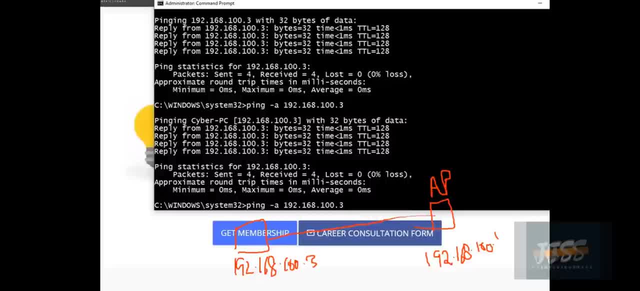 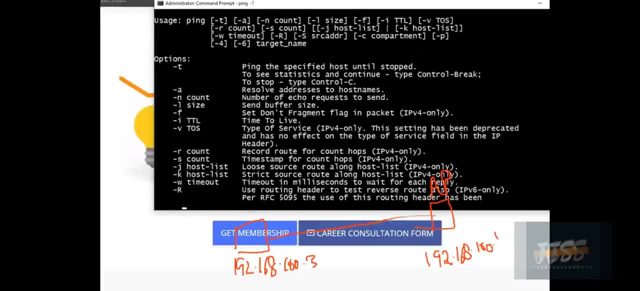 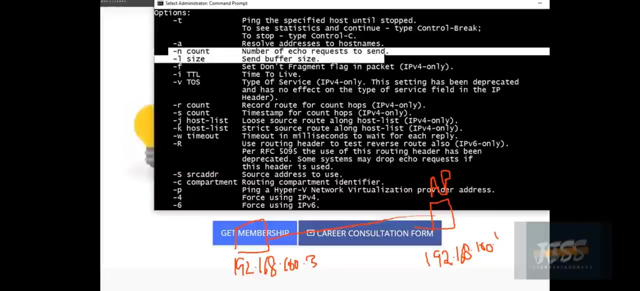 uh, your hotel management application. another server is running. uh, sql server. another one is running, let's suppose, your finance application. so with, because you have given some kind of name to this, i'm sure. okay, let's go uh some another options. um then, what else? this is the number of uh things we 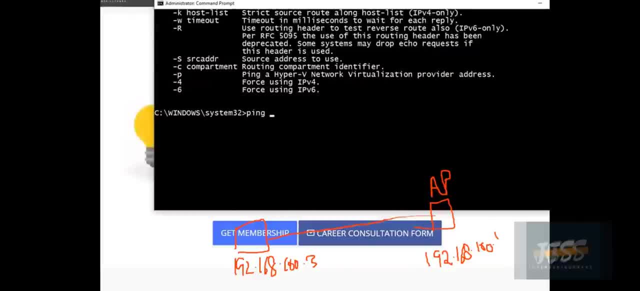 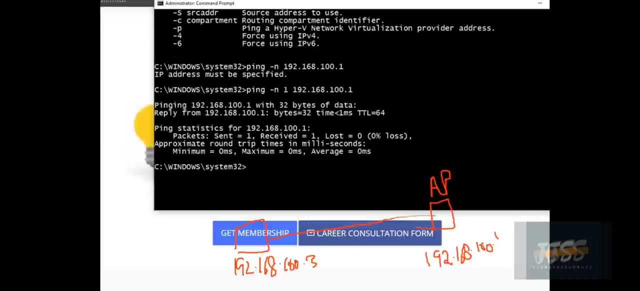 can send, for example: uh, i want to send just one ping, just for some purpose. oh sorry, uh, you have to mention many things you want to send after minus n. as you can see, it just said one thing. okay, so there could be some reason, valid reason, the purpose that we want to send only one thing. 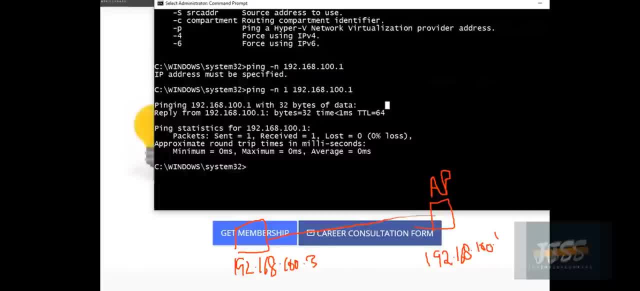 so this thing should come around. can we use? can we use this uh, specific one for less, a cabling issue? i know that sometimes there's a cable issue and we we want to run a command for long time to see if the cable is fully working. is this the command that you would prefer, as a network engineer, to use, or the other? 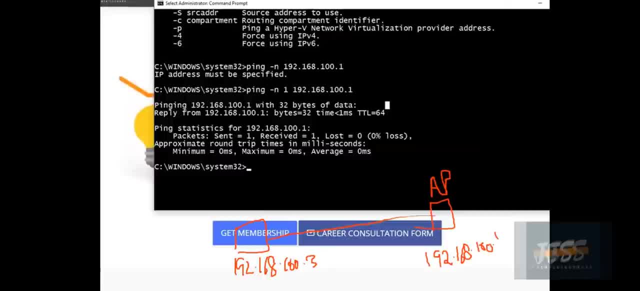 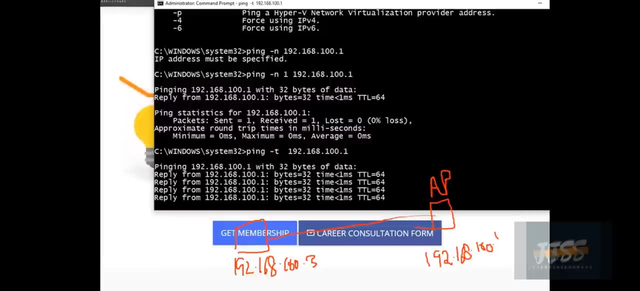 one, exactly this: uh, ping minus n? um, you know there is no any specific reason using minus n, but the one that is most being used is minus t. it will kept pinging and we can see. like you know, if i show the my internet connectivity right now, 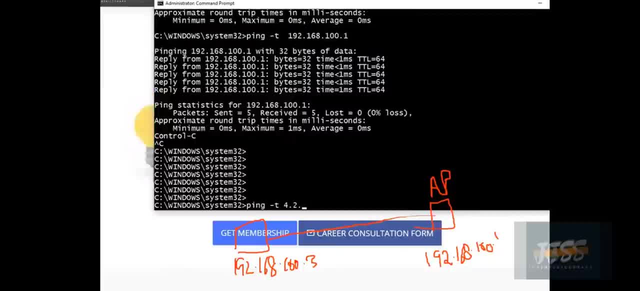 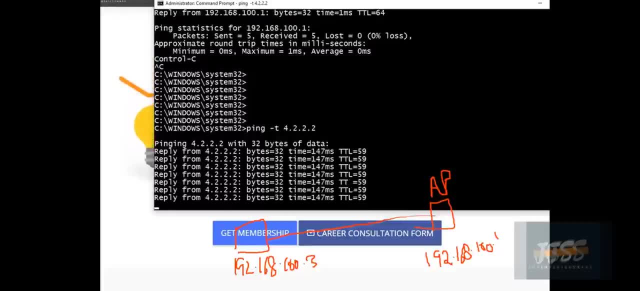 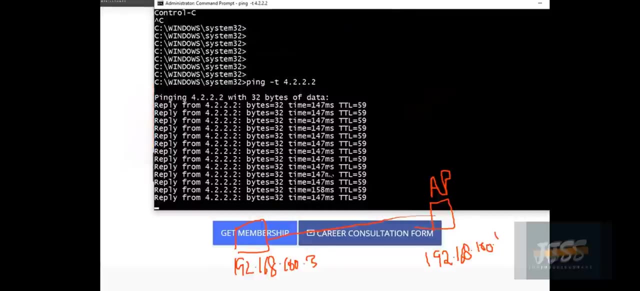 if i try to ping minus t with the help of four: dot two, dot, two, dot two. so basically it kept on pinging and i can correlate with my ttl and times. if there is any kind of delay, i can see here. okay, can you explain to us? or for hyphen crystal: how does? how do you determine these ms? what does? 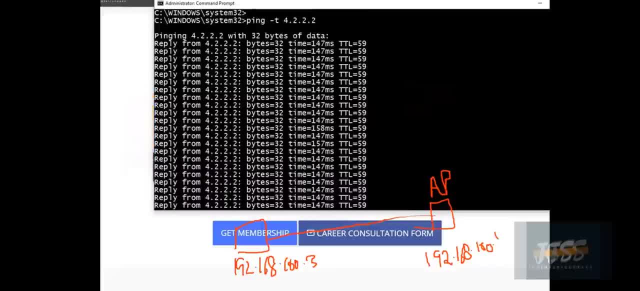 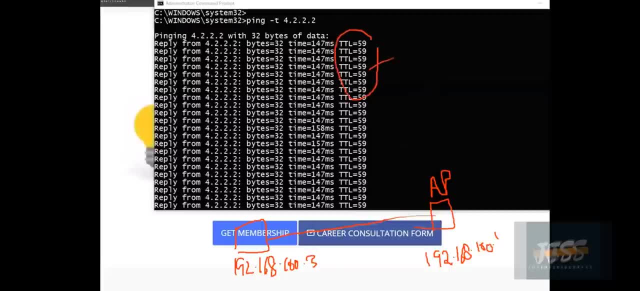 this gives us any information. if it says ms this much or ttl this much, how would you know? i will not use this ttl part because we are going to cover next okay, so we will be specific to this time. these are the time slots. basically is trying trying to hit this device in this millisecond. 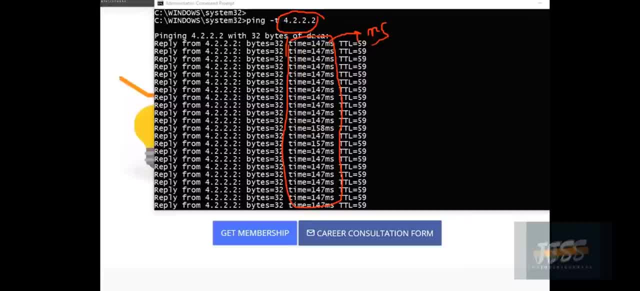 it means my first packet went in 147 milliseconds. it hit that server and returned back to 147. it means my internet connectivity is so stable. but, as you can realize, here hit something happened. it hit 140, 58 milliseconds. it means some kind of application which is running in my 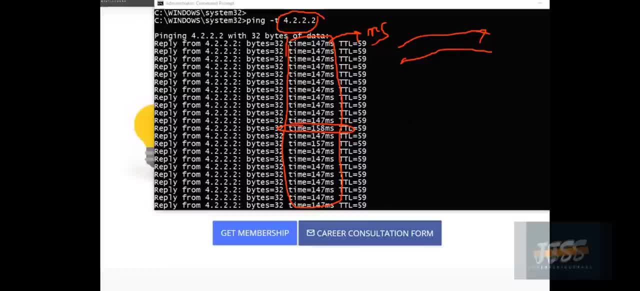 background. maybe it is taking some kind of data. so this is one a very good method, you know, to identify your internet connectivity as well. sometime you will, you will get a lot of data. you will find that reply is coming, then there is no reply. request timeout. reply again coming, then again request timeout. reply is coming again. request timeout. 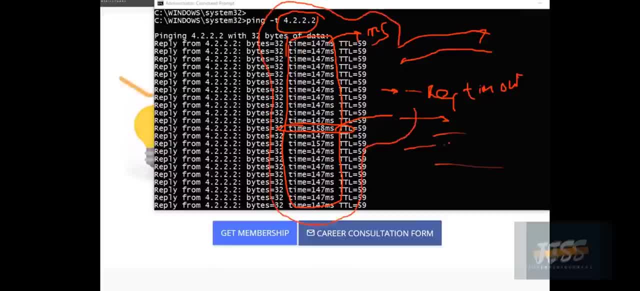 so this is a very pure identification that there is going something happening in your uh uh with the either access point or with the cabling or with the network interface card. so this kind of troubleshooting you can do with the help of displaying minus b command clear. thank you, yes, okay, that's good. 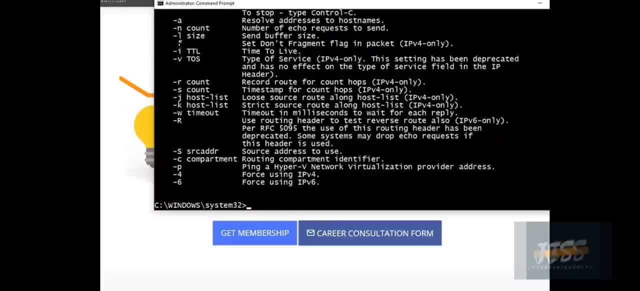 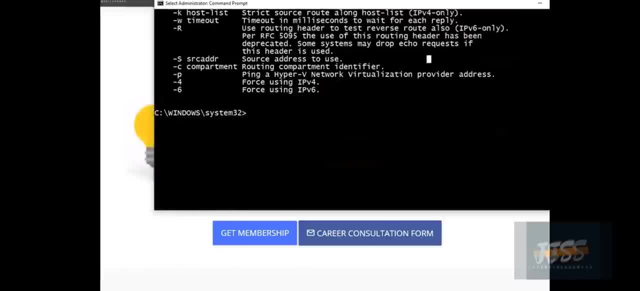 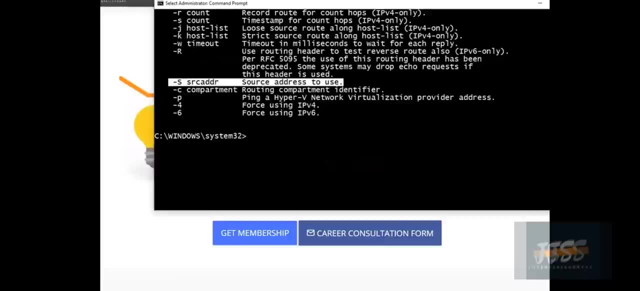 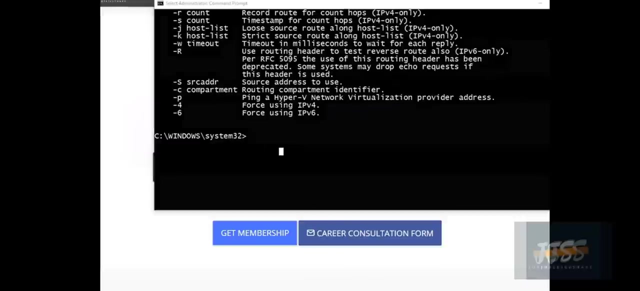 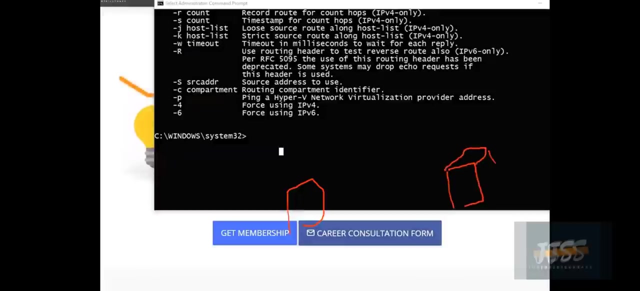 then we have some other options. these i'm not gonna tell these are so advanced, uh, uh. then this is also very informative, which is saying source address to use. okay, uh, i think i have removed that. so we have this, uh, a simple topology where we have a server and we have a host machine. 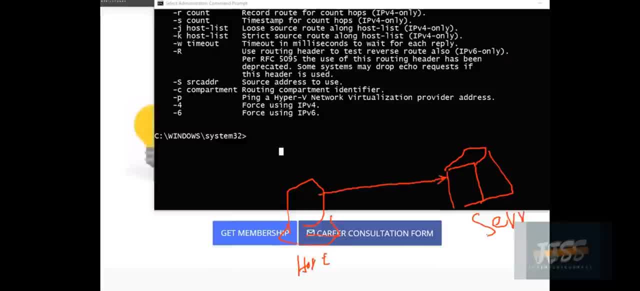 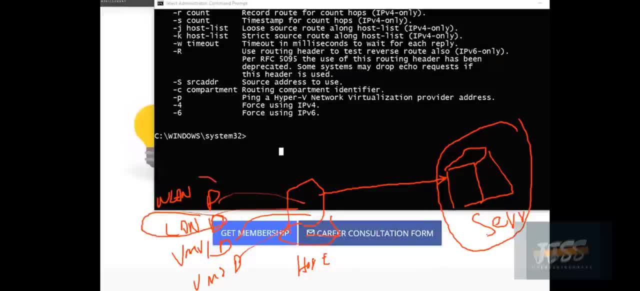 i have one for vmware, one for virtual machine two. so what if i want to ping this server? i have one for vmware, one for virtual machine two. so what if i want to ping this server using my default land interface dot. but using my default land interface dot. but 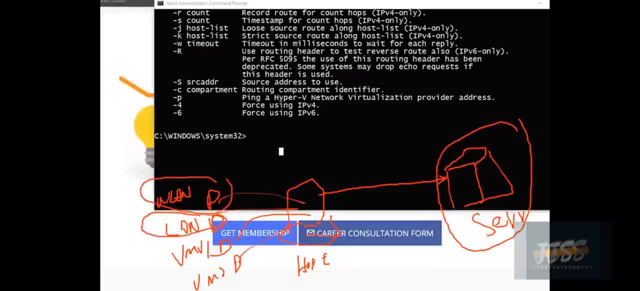 using my default land interface, dot, but from my wireless land, then this thing will help us minus s. then this thing will help us minus s. then this thing will help us minus s, which is basically telling me from which, which is basically telling me from which, which is basically telling me from which source you're gonna. 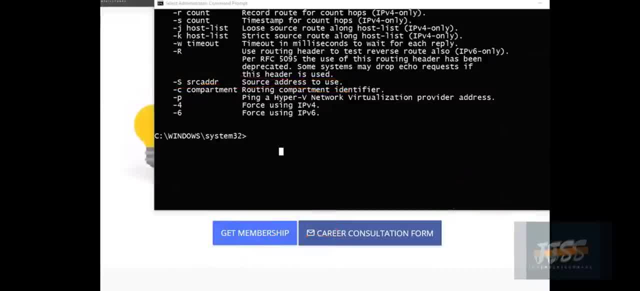 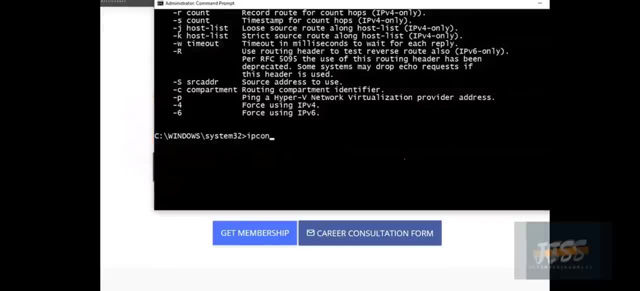 source, you're gonna source, you're gonna ping. so let's do this example here live. so let's do this example here live. so let's do this example here live. uh, uh, uh. let's suppose if i go to ipcon, fake slash. let's suppose if i go to ipcon, fake slash. 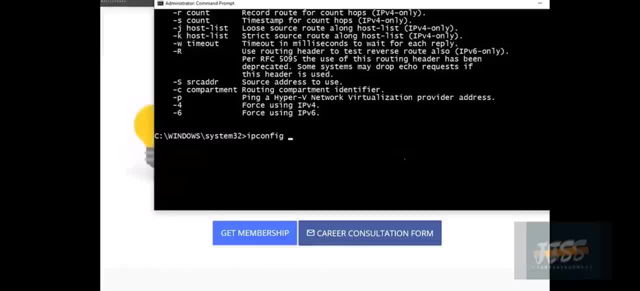 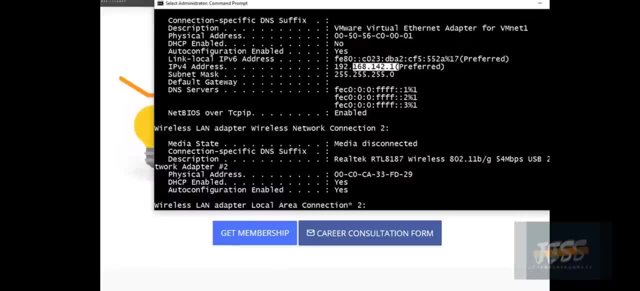 let's suppose, if i go to ipcon fake slash all to see all of my ips, and let's pick uh the ip. and let's pick uh the ip. and let's pick uh the ip, let's this one. 192.162.42.1. 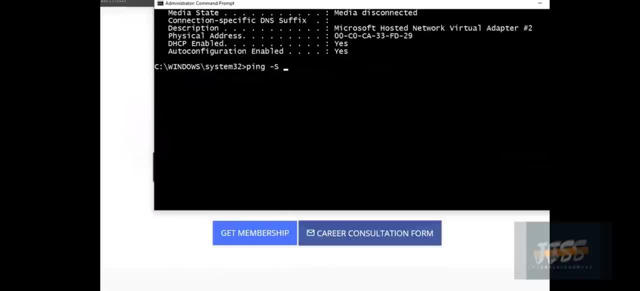 let's this one 192.162.42.1. let's this one: 192.162.42.1. and if i want to ping, and if i want to ping, and if i want to ping, i will type minus s with. i will type minus s with. 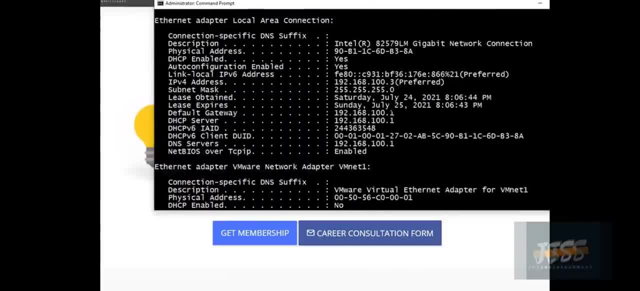 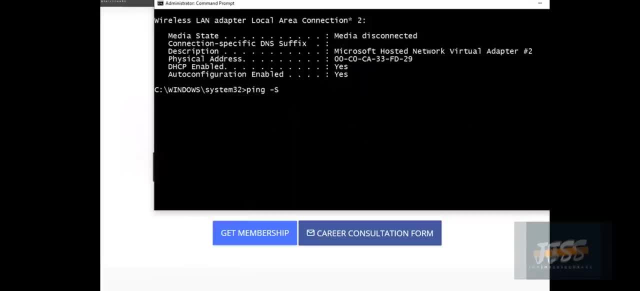 i will type minus s with: uh, uh, uh, this, this, this as a source, as a source, as a source which is: uh, yes, this one, yes, this one, yes, this one, and i will try to ping and i will try to ping and i will try to ping my access point. 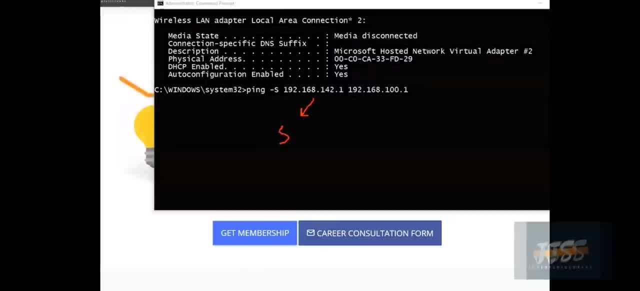 my access point, my access point, so so, so, this is going to be my source, this is going to be my source, this is going to be my source and this is going to be my destination, and this is going to be my destination and this is going to be my destination. but, if you notice, earlier i was trying. 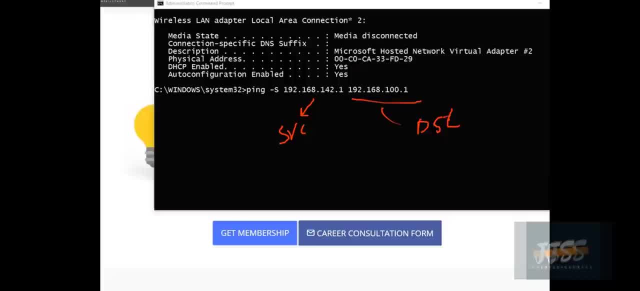 but if you notice earlier i was trying, but if you notice earlier i was trying to ping, to ping, to ping, uh, uh, uh from the same subnet, from the same subnet, from the same subnet, from my lan device, basically the lan, from my lan device, basically the lan. 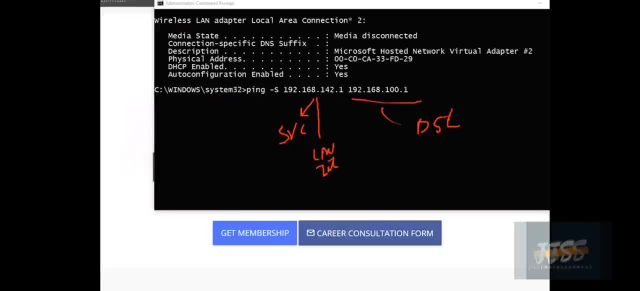 from my lan device, basically the lan network interface card, network interface card, network interface card. but this time i'm trying to, but this time i'm trying to, but this time i'm trying to uh sourcing from the vm machine. but there is kind of some, let's say, 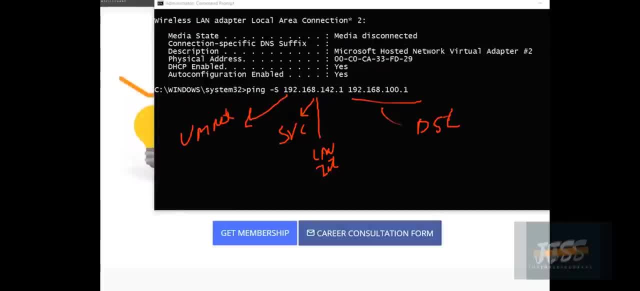 but there is kind of some let's say: but there is kind of some let's say some requirement that i want my vm, where some requirement that i want my vm, where some requirement that i want my vm where to access my, to access my, to access my access point. 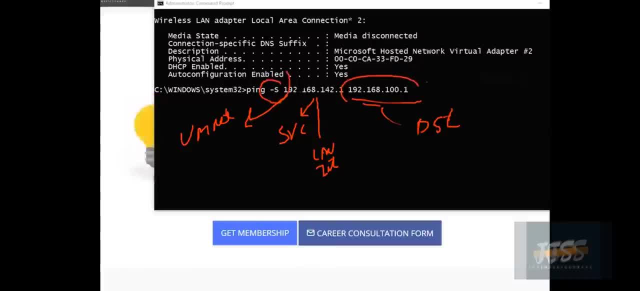 access point. access point, so you can use minus s option with the. so you can use minus s option with the. so you can use minus s option with the help of this help, of this help of this um vm net ip address to ping this um vm net ip address to ping this. 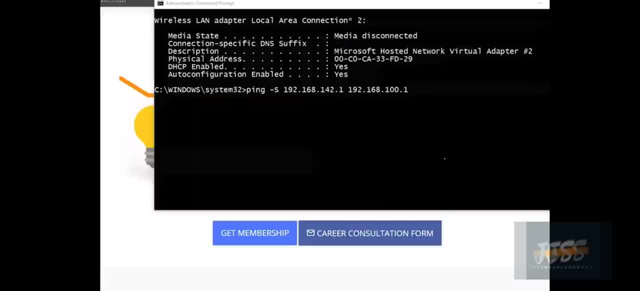 um vm net ip address to ping this? uh access point, let's try pinging. does it? uh access point? let's try pinging. does it? uh access point? let's try pinging. does it work or not? work or not work or not? as you can see, transmit failed because 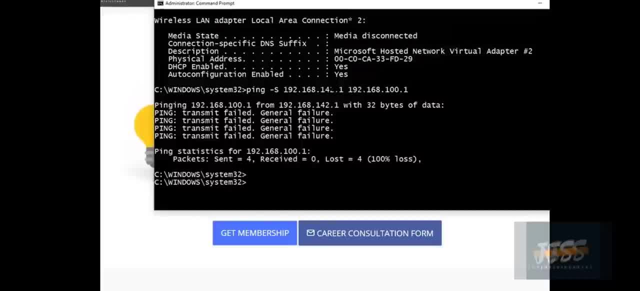 as you can see, transmit failed because, as you can see, transmit failed because my router does not have any information. my router does not have any information, my router does not have any information about this one, about this one, about this one. but if i will do the same thing, 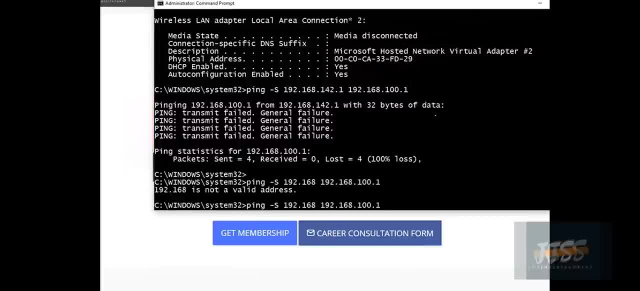 with the same subnet. with the same subnet with the same subnet, oh sorry, and. and the ip of my device is 100.3, and and the ip of my device is 100.3. and and the ip of my device is 100.3. this time i try to ping. you can see the. 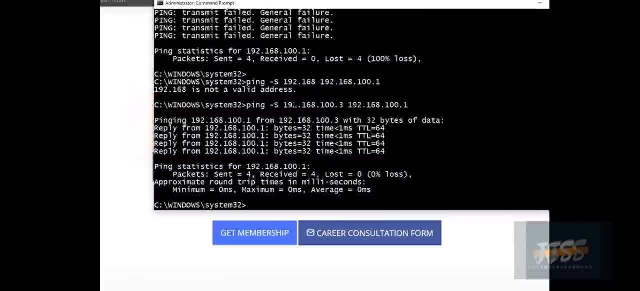 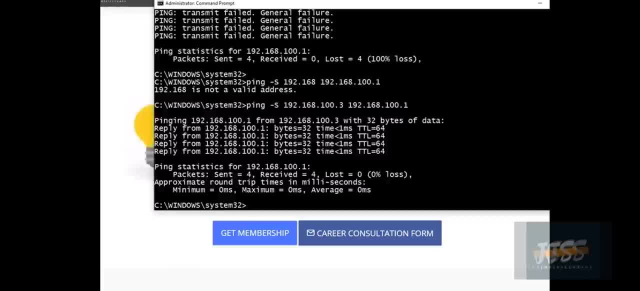 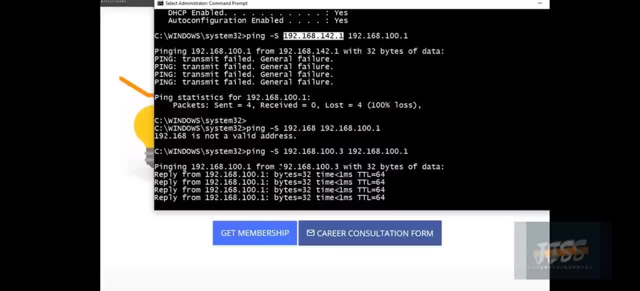 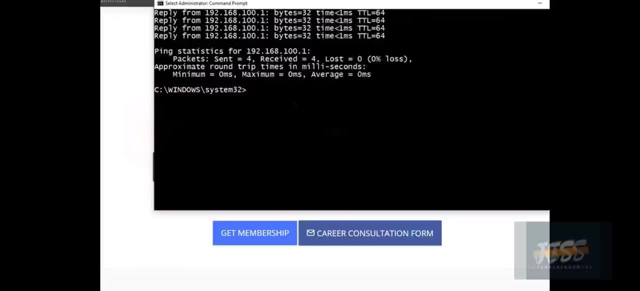 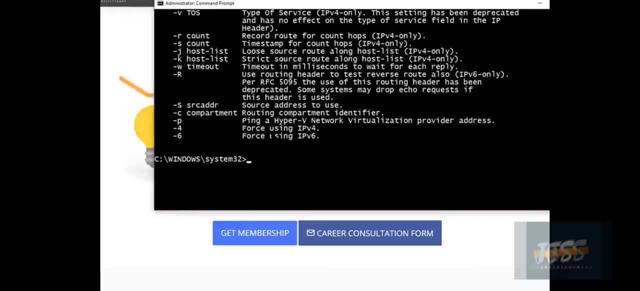 uh, the difference between these two ips. uh, the difference between these two ips. so i am sourcing from different location. so i am sourcing from different location, so i am sourcing from different location. basically, if i try to go some other option, if i try to go some other option, 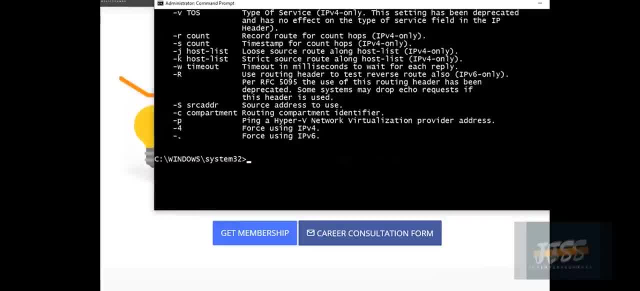 if i try to go some other option and i'm not gonna go uh and i'm not gonna go uh and i'm not gonna go uh. do the demo for this one if you have uh. do the demo for this one if you have uh. do the demo for this one if you have uh. ipv. 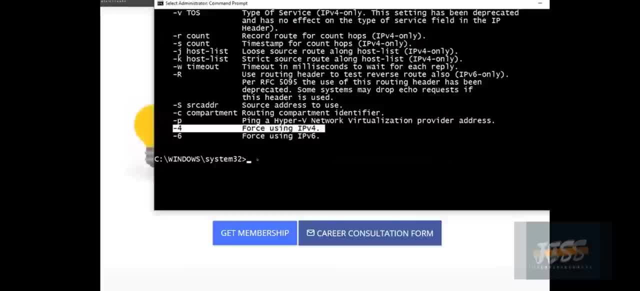 ipv- ipv4. this is by default. we will type minus 4.. this is by default. we will type minus 4.. this is by default, we will type minus 4. and in case of ip6, what if i want to 4? and in case of ip6, what if i want to? 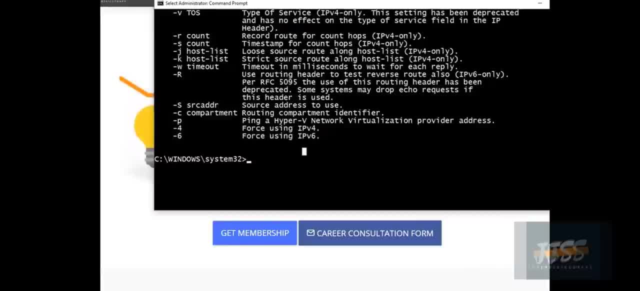 4 and in case of ip6, what if i want to ping ipv6 addresses, ping ipv6 addresses, ping ipv6 addresses you can use like my ping minus six, you can use like my ping minus six, you can use like my ping minus six. and then this very long ipv6 address. 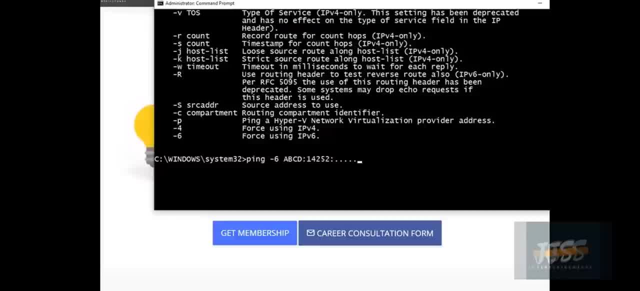 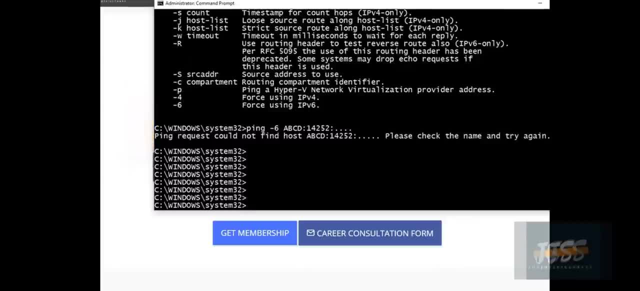 and then this very long ipv6 address, and then this very long ipv6 address, something like this, something like this, something like this, and then you can pay this address, and then you can pay this address, and then you can pay this address. okay, so the demo for your ping section. 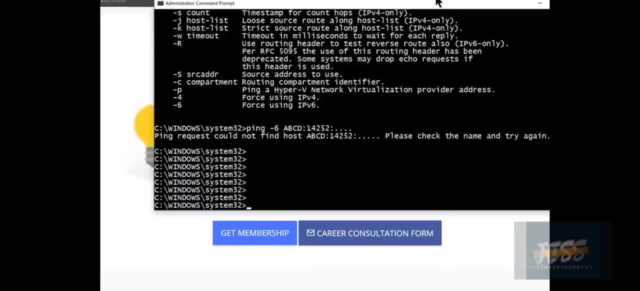 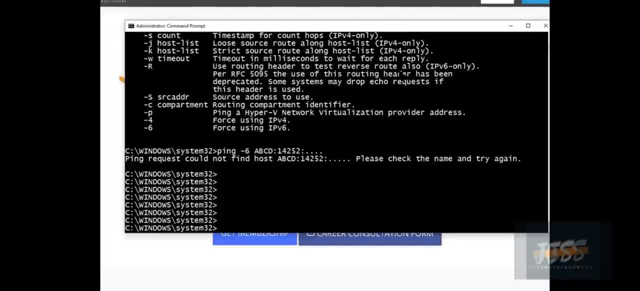 okay, so the demo for your ping section. okay, so the demo for your ping section ends here, ends here, ends here. if you have any question, you may ask: hello, hello, hello. no, we're good. no, we're good, no, we're good. i'm not getting any replies, so that's. 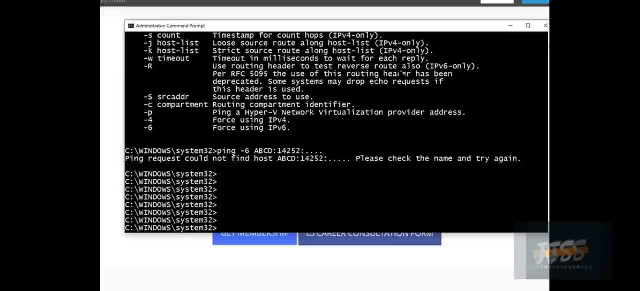 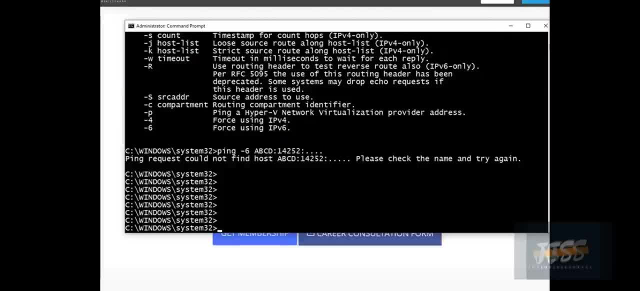 when you don't hear a reply, when you don't hear a reply, when you don't hear a reply from someone, from someone, from someone, like that you can move on then. okay, like that, you can move on then. okay, like that you can move on then. okay, that's fine. 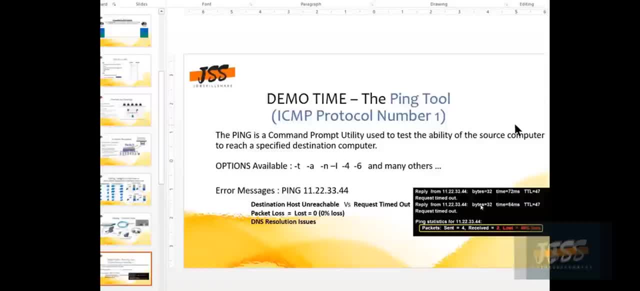 that's fine. that's fine. well, sometimes it happens that there is well. sometimes it happens that there is well. sometimes it happens that there is internet connect connection issues. maybe internet connect connection issues, maybe internet connect connection issues, maybe. uh, i'm connected, but you are not so. 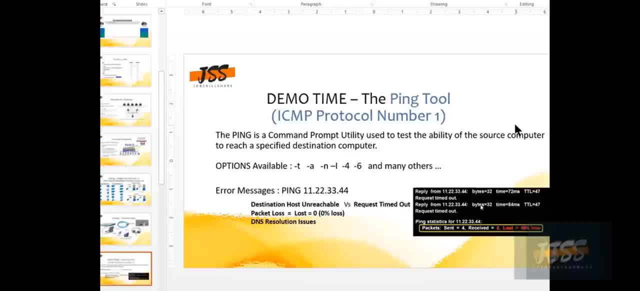 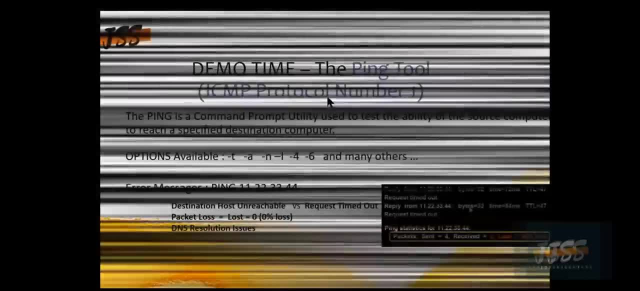 uh, i'm connected, but you are not so, uh, i'm connected, but you are not so. that's why you know, that's why you know, that's why you know, i just want some echo from you. okay, so the ping has: uh, we have done okay. okay, so the ping has: uh, we have done okay. 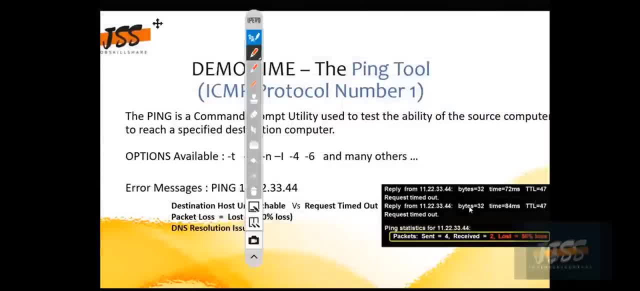 okay, so the ping has. uh, we have done okay, so, so, so, uh, and again this the, and again this the, and again this the. i think for you guys, you, you should, i think for you guys, you, you should, i think for you guys, you, you should, after this: 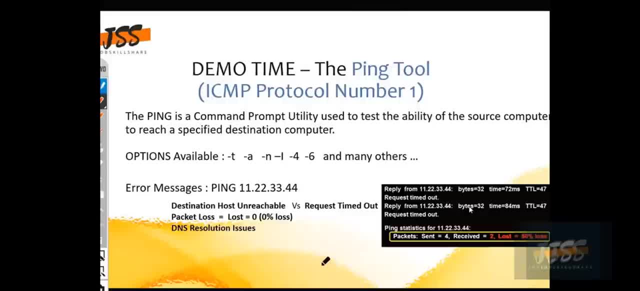 after this, after this, you know, try to ping your own home. you know, try to ping your own home, you know, try to ping your own home. network, try to understand because you network. try to understand because you network. try to understand because you have such a good, have such a good. 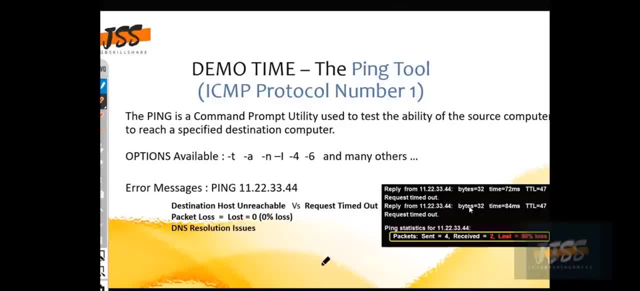 have such a good example right there. you have so many example right there. you have so many example right there. you have so many devices. you have a router at your home devices. you have a router at your home devices. you have a router at your home because you're going to have to start. 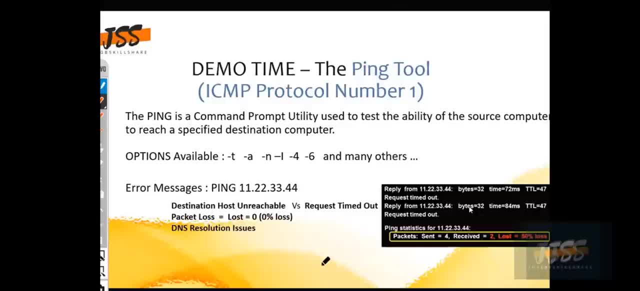 because you're going to have to start, because you're going to have to start with extreme basics like that to with extreme basics like that, to with extreme basics like that, to understand your, even your home network, understand your, even your home network, understand your, even your home network. that level of ping, a ping. 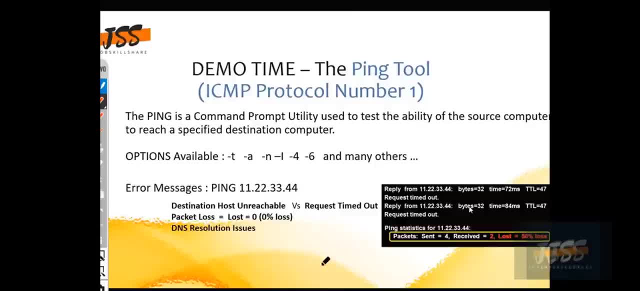 that level of ping a ping. that level of ping a ping jss website. try to ping it for a long jss website. try to ping it for a long jss website. try to ping it for a long time. try to understand what's like you time. try to understand what's like you. 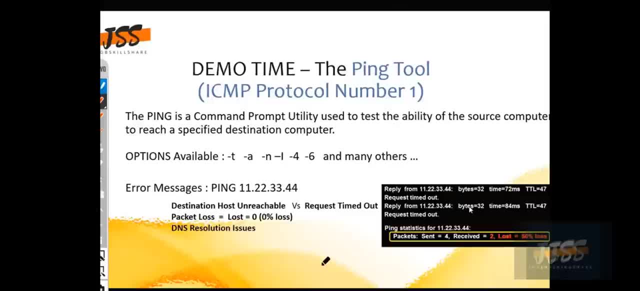 time. try to understand what's like. you know the time, know the time, know the time, things like that and after this, you things like that and after this, you things like that and after this. you should be doing your own research, should be doing your own research, should be doing your own research. they do a lot on ping side because 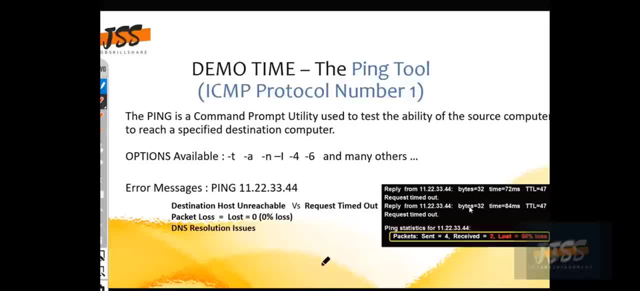 they do a lot on ping side. because they do a lot on ping side, because it's great to get started like this. but it's great to get started like this, but it's great to get started like this, but again, it's great to get started like this, but again, you're always going to be as a 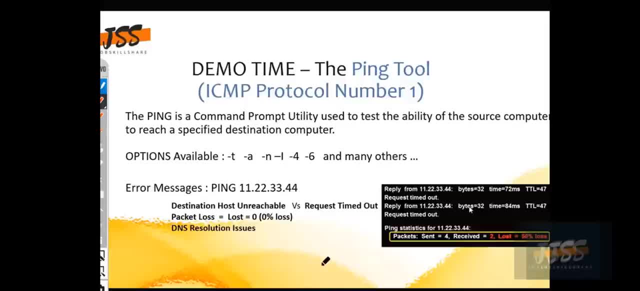 you're always going to be as a you're always going to be as a network engineer, going to be using the network engineer, going to be using the network engineer, going to be using the same concept, even in routing, even in same concept, even in routing, even in. 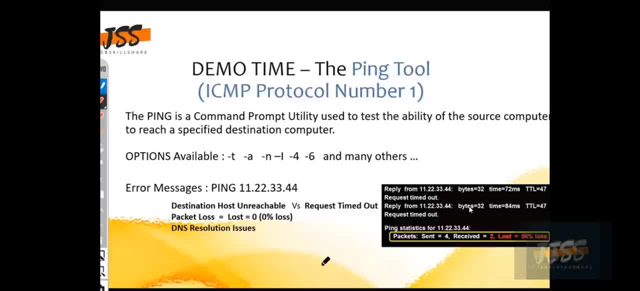 same concept even in routing, even in switching. you have to do ping uh other switching. you have to do ping uh other switching, you have to do ping uh other. devices for for you to do your work, devices for for you to do your work, devices for for you to do your work. you'll have to do that from their devices. 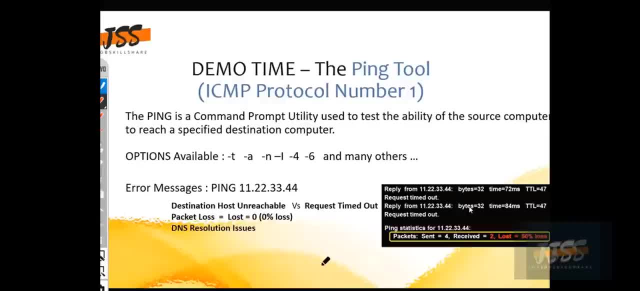 you'll have to do that from their devices. you'll have to do that from their devices as well, but as well, but as well. but that's where i think you guys should. that's where i think you guys should, that's where i think you guys should start with extreme basics, move up to 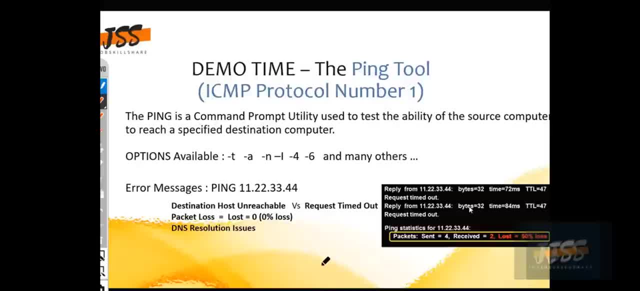 start with extreme basics. move up to start with extreme basics, move up to your home network, and then, after that, your home network, and then, after that, your home network, and then, after that, when you start the packet tracers, and when you start the packet tracers, and. 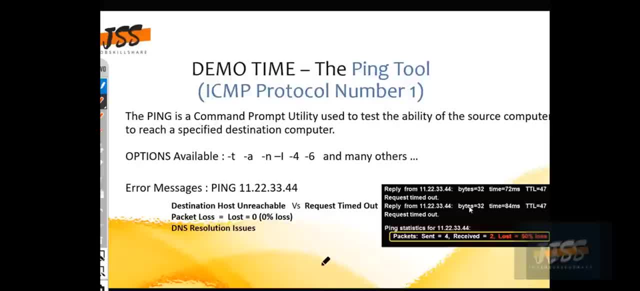 when you start the packet tracers and all that kind of stuff and your labs, all that kind of stuff and your labs, all that kind of stuff and your labs, you should be then using. you know same. you should be then using you know same. you should be then using you know same, same method, same. 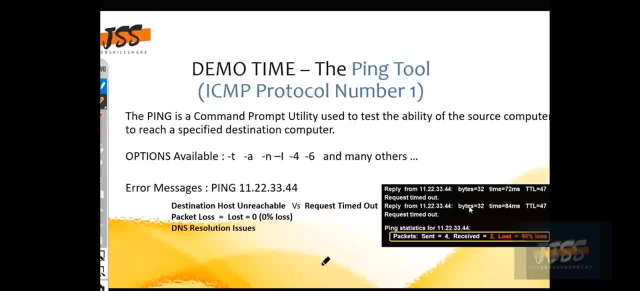 same method, same same method, same concepts in those type of devices as concepts in those type of devices, as concepts in those type of devices as well. okay, okay, okay. so we come across some another error, so we come across some another error, so we come across some another error messages you need to understand. one is: 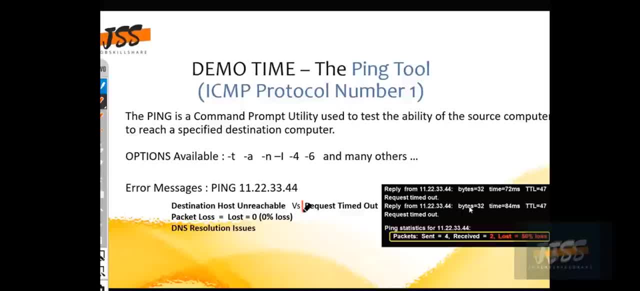 messages you need to understand. one is messages you need to understand. one is: destination host unreachable versus destination host unreachable versus destination host unreachable versus request time now. request time now. request time now. so most often you come across these, so most often you come across these, so most often you come across these errors. so you must have an idea what. 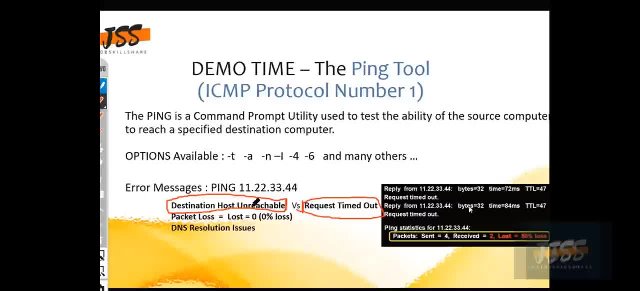 errors, so you must have an idea what errors, so you must have an idea what. what is the different difference between? what is the different difference between, what is the different difference between these two, these two, these two. post unreachable, basically. post unreachable, basically, post unreachable, basically, when we are on the same network. 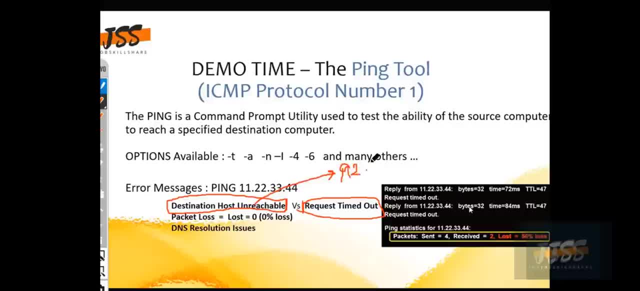 when we are on the same network. when we are on the same network, let's suppose in my case. let's suppose in my case, let's suppose in my case we are running 192 168, we are running 192 168, we are running 192 168 dot 100. 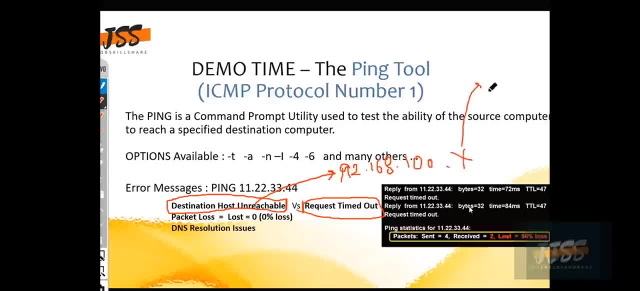 dot 100, dot 100, dot x, dot x, dot x. x means whatever the host, x means whatever the host, x means whatever the host. identification number. you can do but one identification number. you can do but one identification number. you can do but one, two, three, two, three. 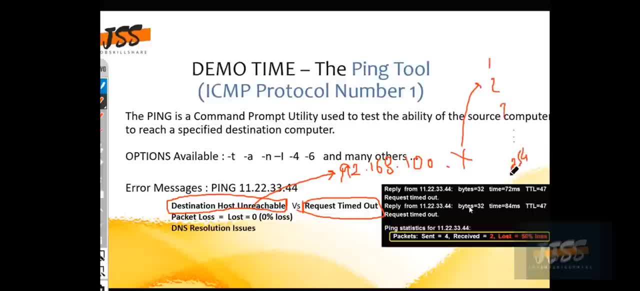 two, three, all the way up to 254. you can assign all the way up to 254. you can assign all the way up to 254. you can assign. so, if i'm trying, so, if i'm trying so, if i'm trying to ping, to ping. 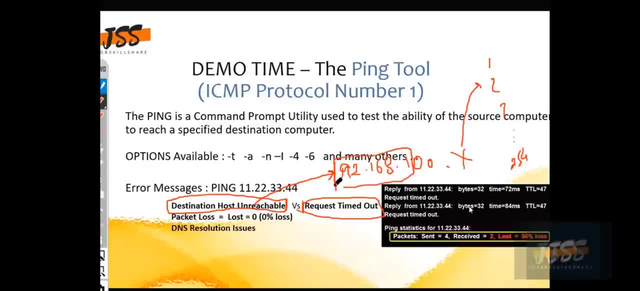 to ping some id, some id, some id within this subnet, within this subnet, within this subnet. i'm going to receive both unreachable. i'm going to receive both unreachable. i'm going to receive both unreachable. it means we are on the same subnet. but it means we are on the same subnet, but. 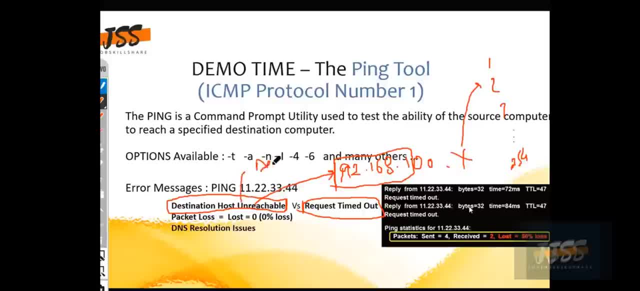 it means we are on the same subnet, but maybe this computer is maybe dead. maybe this computer is maybe dead. maybe this computer is maybe dead- uh, maybe shut down. uh, maybe shut down. uh, maybe shut down. or maybe there is cable issue network. or maybe there is cable issue network. 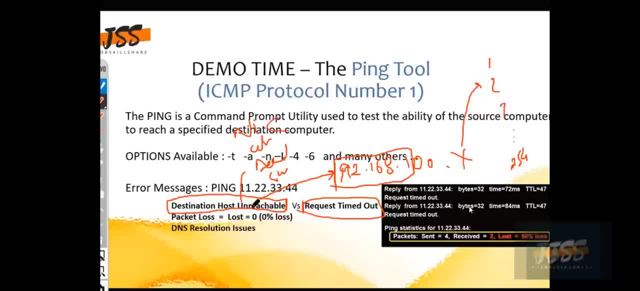 or maybe there is cable issue, network interface card issue, interface card issue, interface card issue. okay, so you are going to receive. okay, so you are going to receive, okay, so you are going to receive unreachable, unreachable, unreachable. request time out. request time out. request time out when, when? 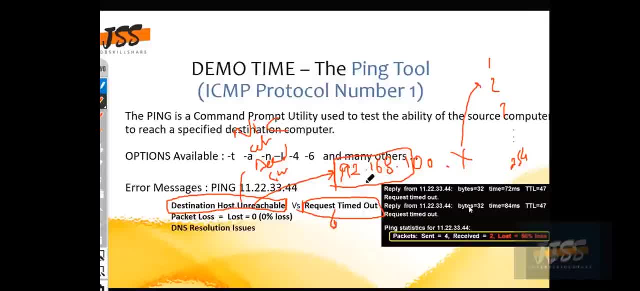 when you are not on the same subnet. you are not on the same subnet, you are not on the same subnet and this subnet does not exist in this and this subnet does not exist in this and this subnet does not exist in this domain. domain domain. these kind of errors you're gonna. 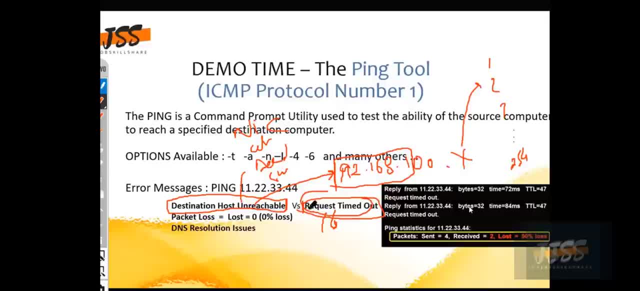 these kind of errors you're gonna these kind of errors you're gonna receive, receive, receive and we will discuss. you know, and we will discuss. you know and we will discuss. you know, you don't need to worry about this, we will. you don't need to worry about this, we will. 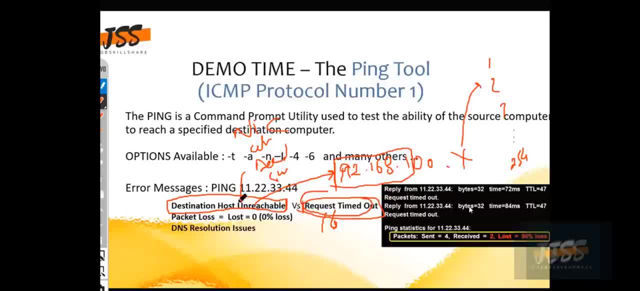 you don't need to worry about this. we will go a lot in detail. when we go a lot in detail, when we go a lot in detail, when we in a router and switches, we will be in a router and switches, we will be in a router and switches, we will be pinging. you will see. 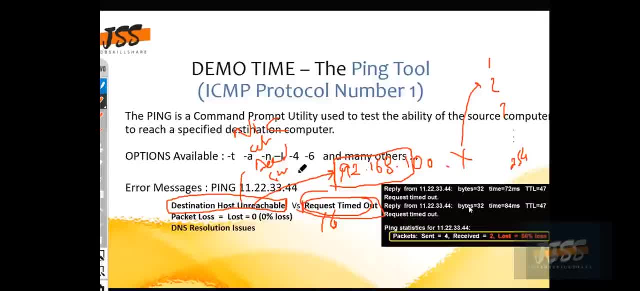 pinging, you will see pinging, you will see several kind of errors there and these several kind of errors there and these several kind of errors there, and these just i'm giving you, just i'm giving you, just i'm giving you, i just, uh, flag overview the difference. 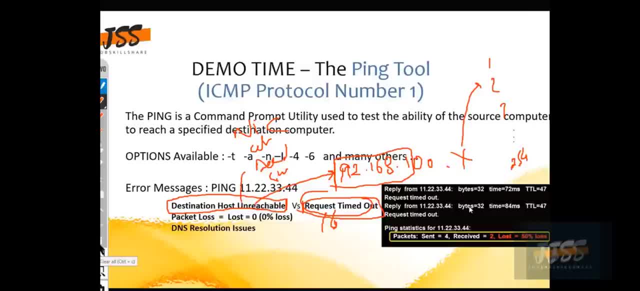 i just uh flag overview the difference. i just uh flag overview the difference between these two. then this packet loss, uh it. then this packet loss, uh it. then this packet loss, uh it gives the gives you the information. how gives the gives you the information. how gives the gives you the information. how many packets have been lost, like in this. 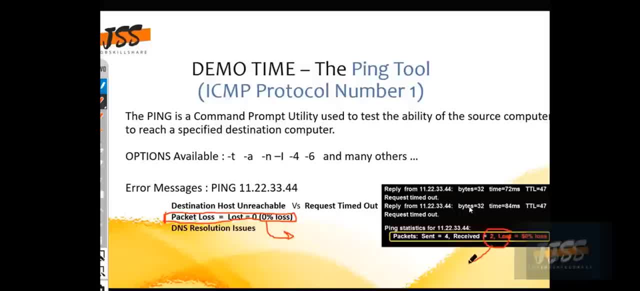 many packets have been lost, like in this many packets have been lost, like in this case, case, case. you can see two packets lost. you can see two packets lost. you can see two packets lost. it means there is kind of some issue in. it means there is kind of some issue in. 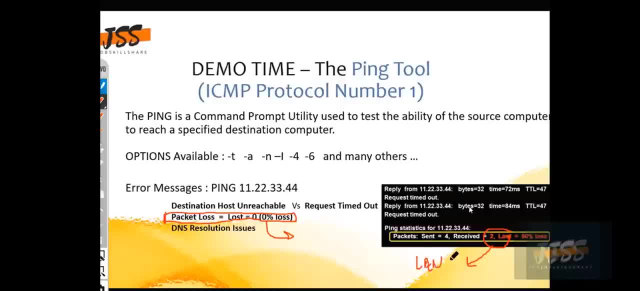 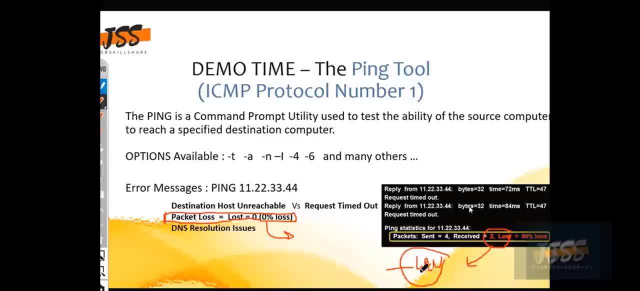 if you are pinging your device that is in the your same, the your same, the your same, lan environment, lan environment, lan environment, then i'm sure this is a problem with your, then i'm sure this is a problem with your, then i'm sure this is a problem with your cable. 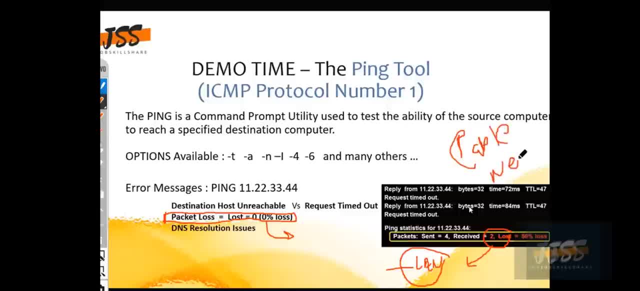 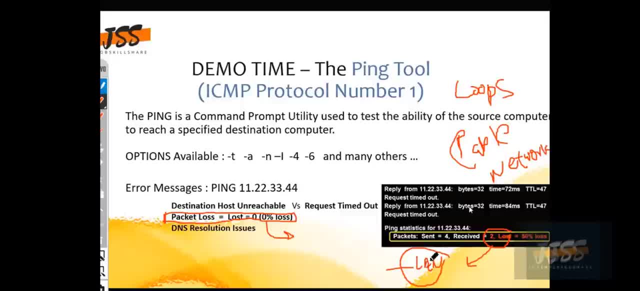 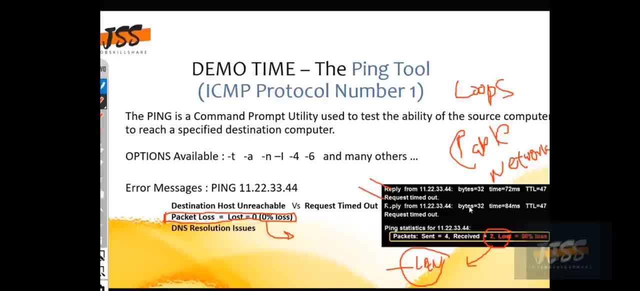 this kind of errors, like as i said, this kind of errors, like as i said earlier, reply is coming. then there is earlier reply is coming. then there is earlier. reply is coming. then there is request time out. request time out. request time out. then reply is coming, request time out it. 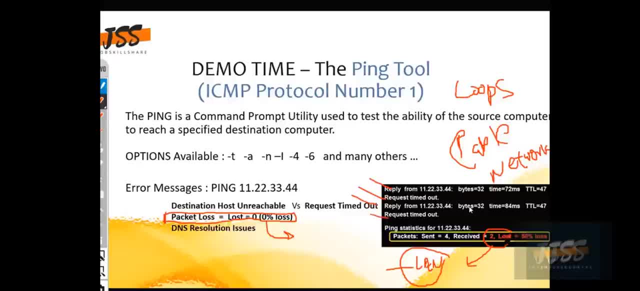 then reply is coming, request time out. it then reply is coming, request time out. it means you have some kind of serious means. you have some kind of serious means, you have some kind of serious internet connectivity is going on in your. internet connectivity is going on in your. 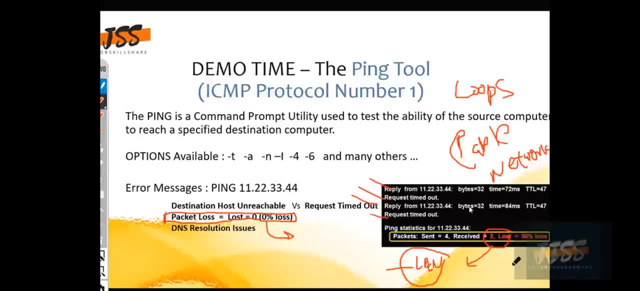 internet connectivity is going on in your uh uh uh, your uh working environment, your uh working environment, your uh working environment. the other tool we're going to use is the other tool we're going to use is: the other tool we're going to use is the trace. 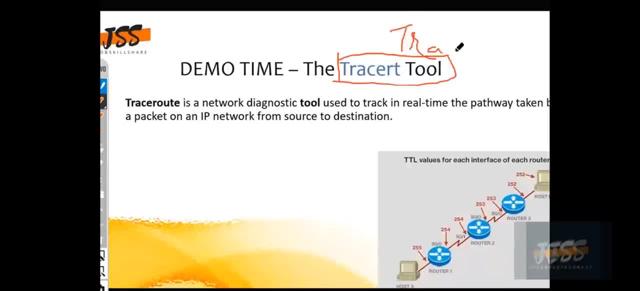 the trace, the trace tracer tool, also known as tracer tool, also known as tracer tool, also known as phase route tool, phase route tool, phase route tool and what it does and what it does and what it does: trace out is a network diagnostic tool. trace out is a network diagnostic tool. 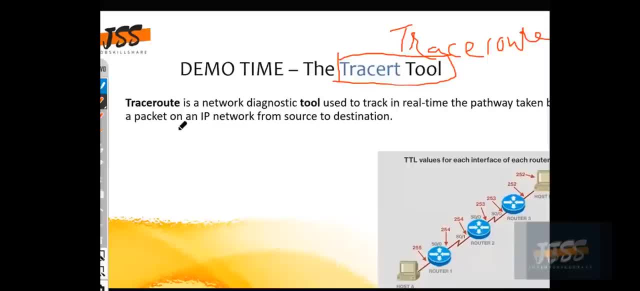 trace out is a network diagnostic tool used to track in a real time the pathway used to track in a real time, the pathway used to track in a real time, the pathway taken by the packet, taken by the packet taken by the packet on an ip network from source, all the way. 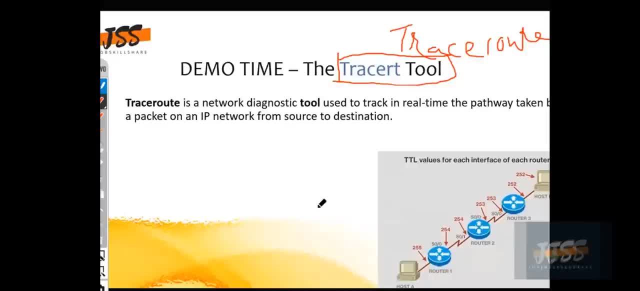 on an ip network from source all the way on an ip network from source, all the way to the destination, to the destination, to the destination. in a very plain english, what does it mean in a very plain english? what does it mean in a very plain english? what does it mean? we have host a here. 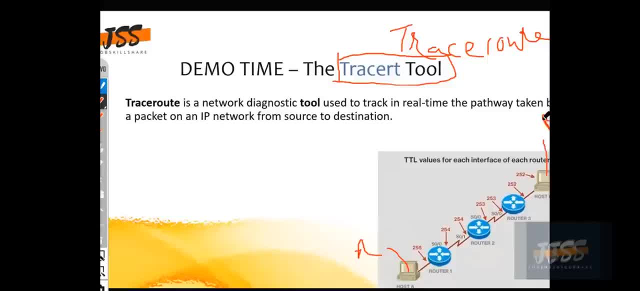 we have host a here, we have host a here and some host b is somewhere for and some host b is somewhere for and some host b is somewhere for location, location, location. we have multiple, we have multiple. we have multiple routers in between routers in between routers in between, and we will use this pressure tool. 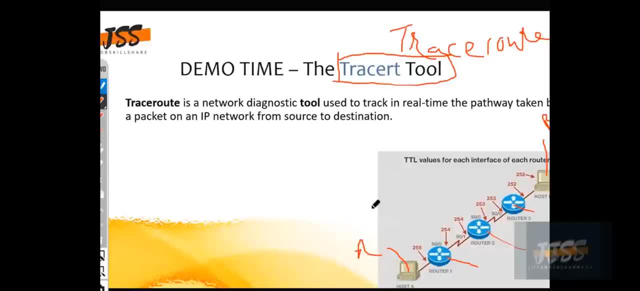 and we will use this pressure tool, and we will use this pressure tool to find out, to find out, to find out how far away this device is from us, how far away this device is from us, how far away this device is from us. so, in this case, 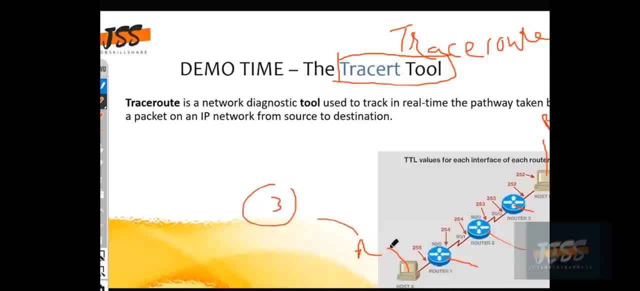 so in this case, so in this case, it's gonna give me reply three, it's gonna give me reply three, it's gonna give me reply three: one, one, one, two, two, two and three, and then it is gonna hit that. and three, and then it is gonna hit that. 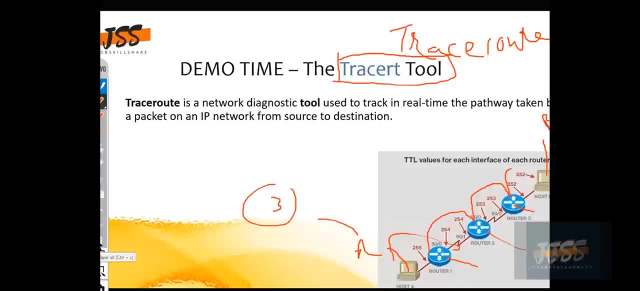 and three and then it is gonna hit that destination. so the tool is very simple, it is, but it, so the tool is very simple, it is, but it, so the tool is very simple, it is, but it is very useful, is very useful, is very useful. why, why? 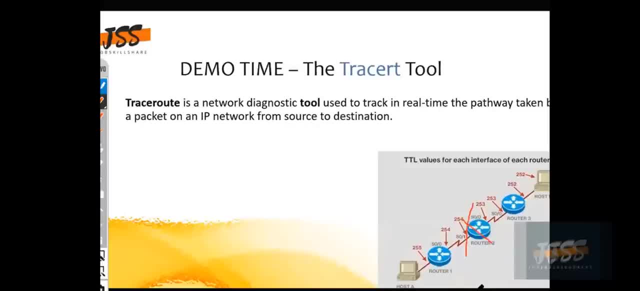 why. let's suppose, let's suppose, let's suppose your this router is down. first you will do ping. ping will tell that ping will tell that ping will tell that host is unreachable. host is unreachable, host is unreachable, then your second tool, then your second tool, then your second tool, which is pressure, is going to be very handy. 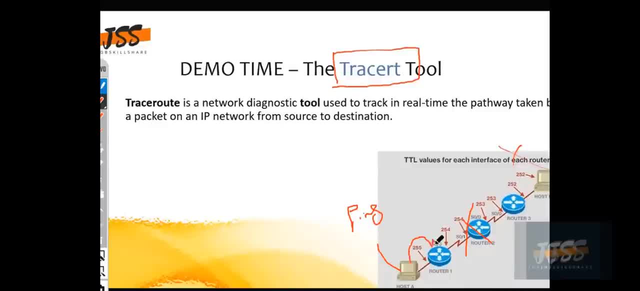 which is pressure, is going to be very handy, which is pressure is going to be very handy. when you will apply a tracer, it will. when you will apply a tracer, it will. when you will apply a tracer, it will hit this one, hit this one, hit this one. it will hit this interface because this: 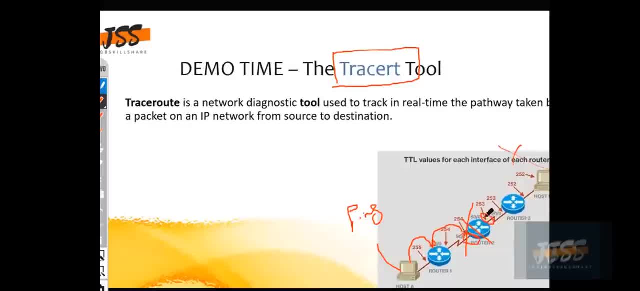 it will hit this interface because this. it will hit this interface because this is still working. only i am talking about is still working, only i am talking about is still working, only i am talking about: this interface is down, this interface is down, this interface is down. so immediately the reply will come from. 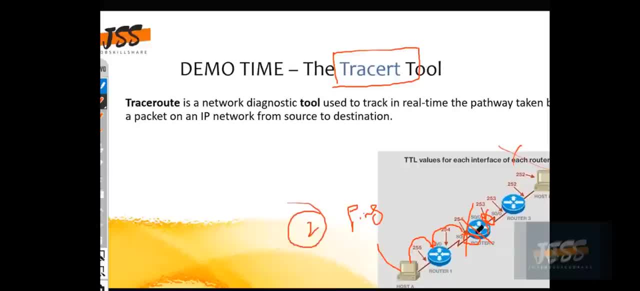 so immediately the reply will come from. so immediately the reply will come from: or will say the two, or will say the two, or will say the two. it means after reaching the second device. it means after reaching the second device. it means after reaching the second device. we cannot go beyond. 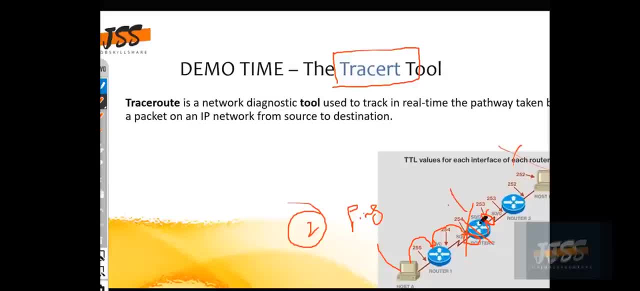 we cannot go beyond. we cannot go beyond. so it means it is a clear indication. so it means it is a clear indication. so it means it is a clear indication that we have somewhere the problem that we have somewhere. the problem that we have somewhere, the problem lies somewhere inside. 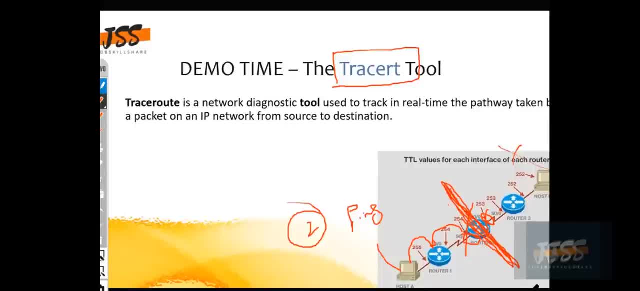 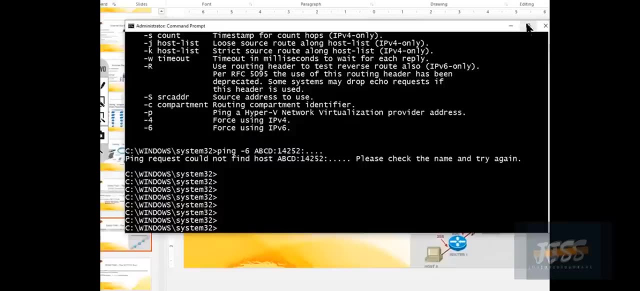 lies somewhere inside, lies somewhere inside in this router and in this boundary. so let's do the so, let's do the so, let's do the uh uh, uh, the demo, the demo, the demo for the present, for the present, for the present. so let's go to the again. command prompt. 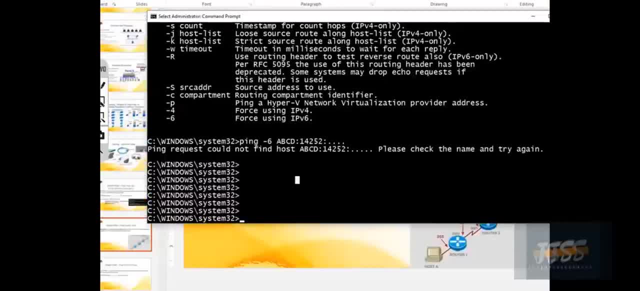 so let's go to the again command prompt. i hope, i hope it is visible. it is visible, it is visible, the command prompt. yeah, the command prompt. yeah, the command prompt. yeah, yep, okay, so you will type t-r-a-c-r-t. okay, so you will type t-r-a-c-r-t. 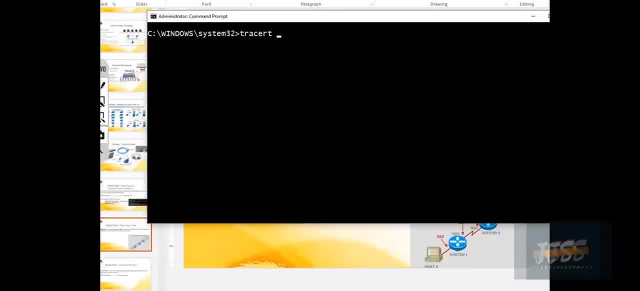 okay, so you will type t-r-a-c-r-t. tracer, tracer, tracer, and the desired and the desired, and the desired address. let's suppose, uh, we want to address. let's suppose, uh, we want to address. let's suppose, uh, we want to trace out, trace out. 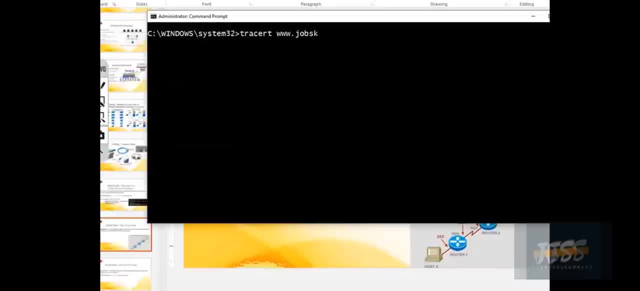 trace out how many, how far, how many, how far, how many, how far job skillshare server is from us. that's my basement. right there, there you go. that's my basement. right there, there you go. that's my basement. right there, there you go. but this is very simple. it's gonna take so. 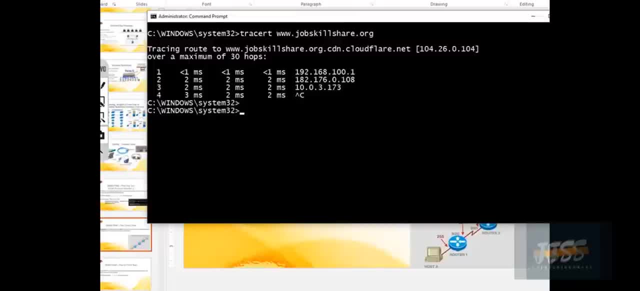 but this is very simple, it's gonna take so, but this is very simple, it's gonna take so long, so i will long, so i will long, so i will go some another option. so here you can go some another option. so here you can go some another option. so here you can see. 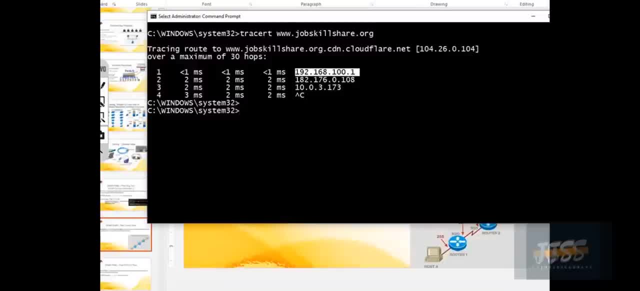 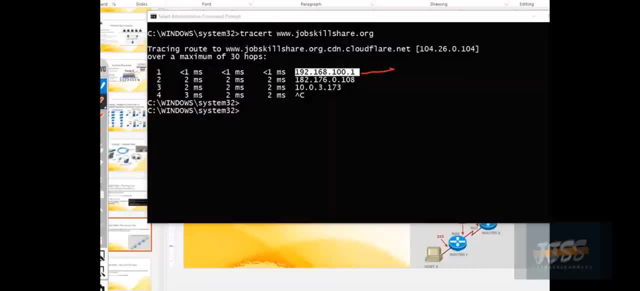 see, see, this is uh 19216 100.1, which is: this is uh 19216 100.1, which is: this is uh 19216 100.1, which is my gateway, gateway, gateway, yes, yes, yes, my gateway, my gateway, my gateway, or, in simple term, is my access point. 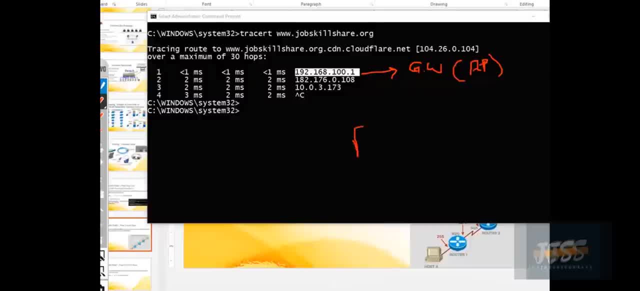 or, in simple term, is my access point? or, in simple term, is my access point: the router, the router, the router then this router, then this router, then this router is connected somehow with the isp, is connected somehow with the isp, is connected somehow with the isp. maybe the router? 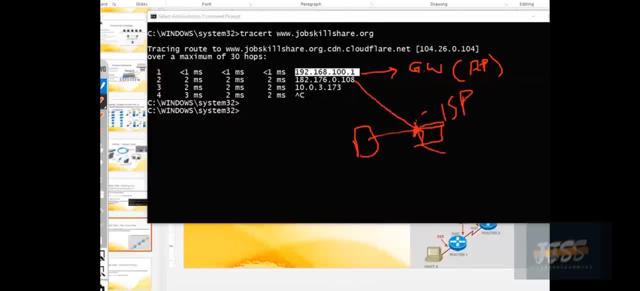 maybe the router, maybe the router, and this is going to the interface of and this is going to the interface of and this is going to the interface of this, this, this router, router, router. then this router is connected with some, then this router is connected with some, then this router is connected with some- another router. 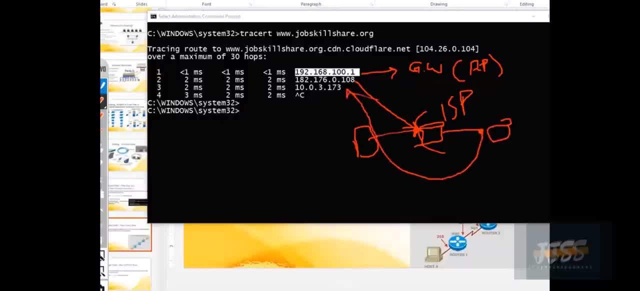 another router, another router on this interface, and this is going to on this interface and this is going to on this interface and this is going to be the ip address for that ip address for that ip address for that. so, so, so it went, it went, it went to. 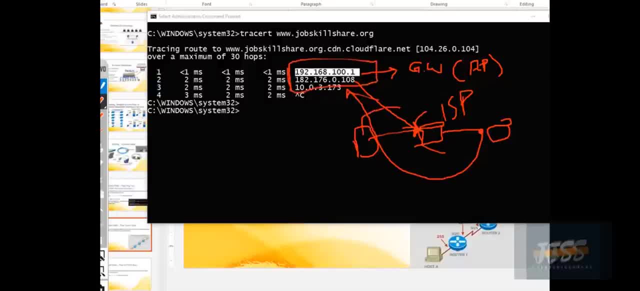 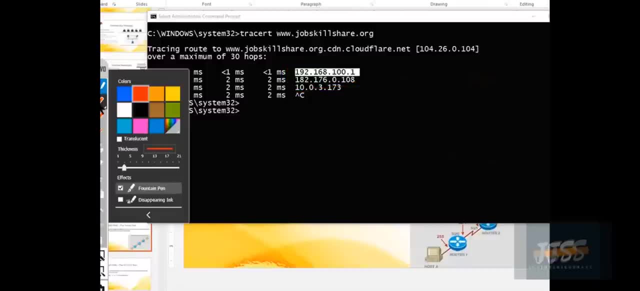 it went to how far three hops, how far three hops, how far three hops: one one, one, two and three. now in a real world example. you would now in a real world example. you would now in a real world example. you would use something like this and come around. 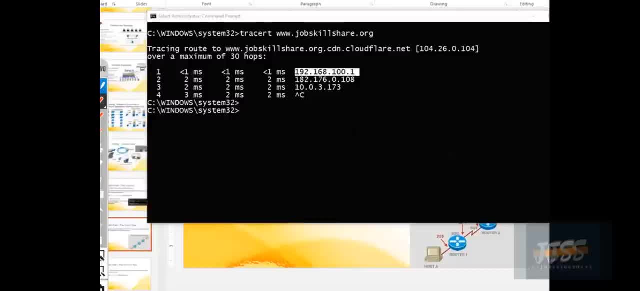 use something like this and come around. use something like this and come around. you can correct me if you have a big. you can correct me if you have a big. you can correct me if you have a big. building with four floors, four floors. building with four floors, four floors. 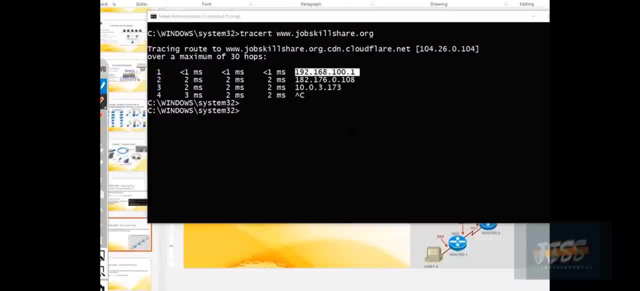 building with four floors. four floors each have its separate switches, each have its separate switches, each have its separate switches. and let's say on the bottom floor, and let's say on the bottom floor, and let's say on the bottom floor, something happened and machines are not. 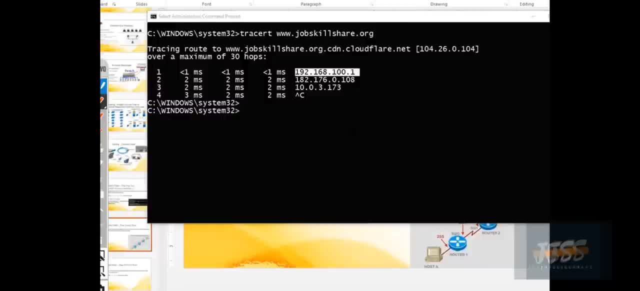 something happened and machines are not. something happened and machines are not able to go outside, and you would use able to go outside and you would use able to go outside and you would use some type of command like this, like some type of command like this, like some type of command like this, like tracer. 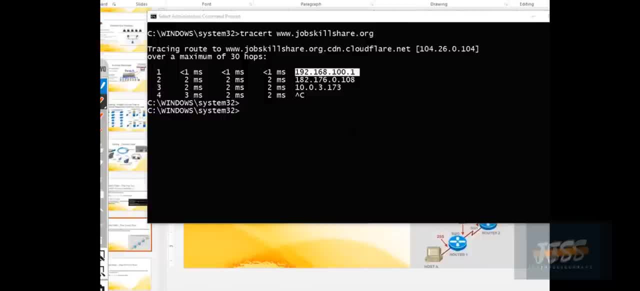 tracer, tracer, which then you can. you can find out which. which then you can. you can find out which, which then you can. you can find out which switch in that floor is then having an switch in that floor? is then having an switch in that floor is then having an issue right? 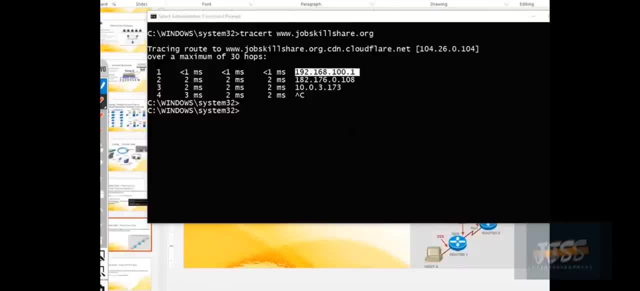 issue: right, issue right: uh, or a router, uh, or a router. uh, or a router, uh, i just want, yeah, yeah, uh. i just want, yeah, yeah, uh, i just want, yeah, yeah, you can continue, you can continue, you can continue, yeah. and another example that i can give: 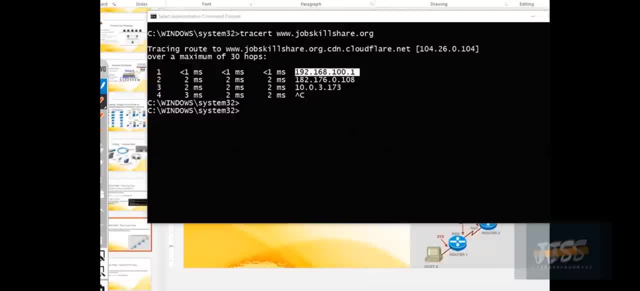 yeah, and another example that i can give: yeah, and another example that i can give you guys that sometimes companies are you guys, that sometimes companies are you guys, that sometimes companies are using a. you know two connections for using a. you know two connections for using a. you know two connections for companies because you don't want to rely. 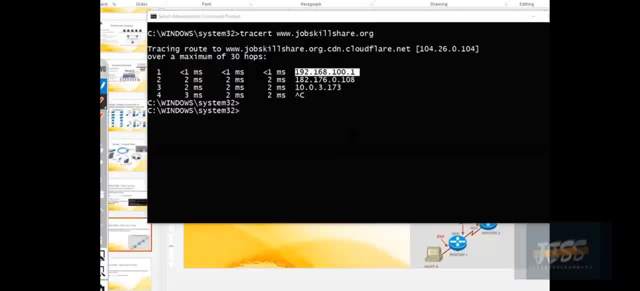 companies, because you don't want to rely companies, because you don't want to rely on one connection. so if one come one on one connection, so if one come one on one connection, so if one come, one goes down and let's say: goes down and let's say: 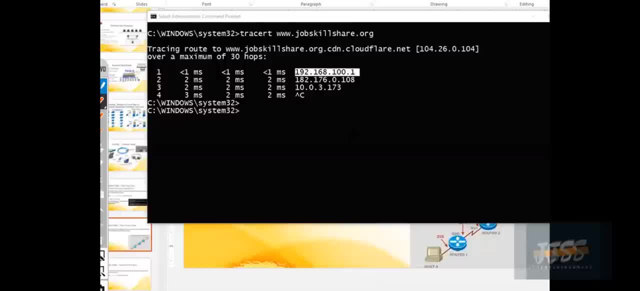 goes down and let's say one is a, one is a, one is a fast connection, another one is a backup fast connection. another one is a backup fast connection, another one is a backup in a slow connection, sometimes a lot of in a slow connection, sometimes a lot of. 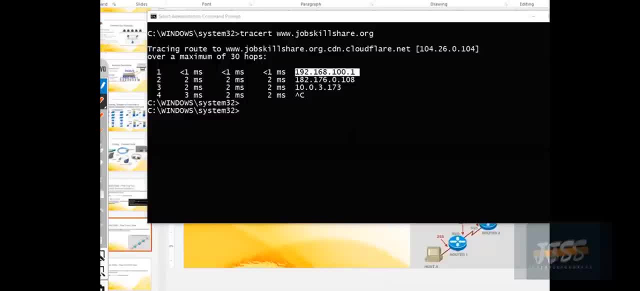 in a slow connection, sometimes a lot of people complain. oh people complain, oh people complain. oh, uh, we are, we can't use internet. uh, so, uh, we are, we can't use internet. uh, so we are, we can't use internet. uh, so slow. and this way you could use a tracer. 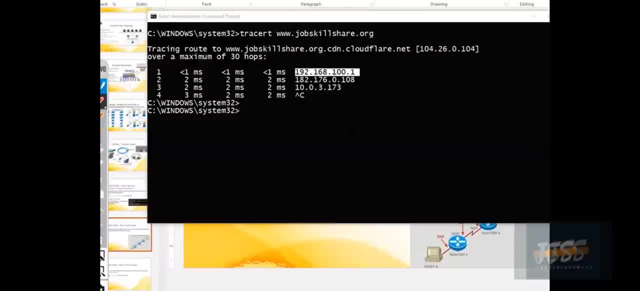 slow and this way you could use a tracer slow and this way you could use a tracer to find out if your connections are, to find out if your connections are, to find out if your connections are actually going to the slow router or the actually going to the slow router or the. 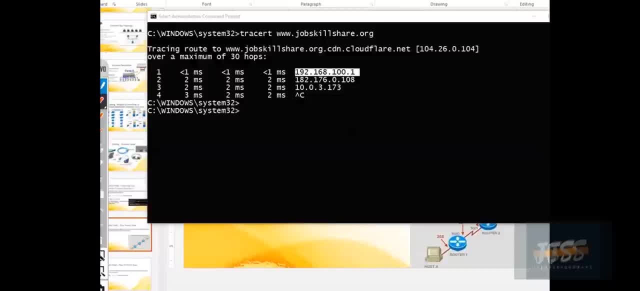 actually going to the slow router or the fast one? yeah, you could find that fast one. yeah, you could find that fast one. yeah, you could find that. because of these commands, just keep this. because of these commands, just keep this. because of these commands, just keep this in mind. there are different scenarios. 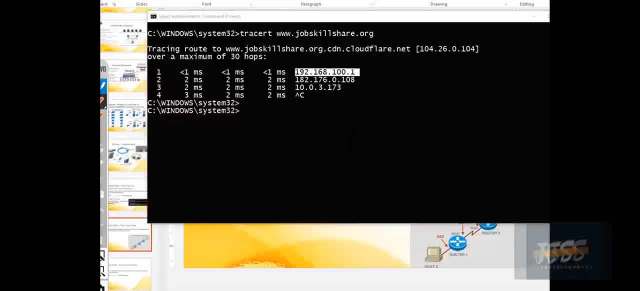 in mind. there are different scenarios in mind. there are different scenarios. you can use this command like that, okay. you can use this command like that, okay. you can use this command like that, okay. yeah, that is very great example. thank yeah, that is very great example. thank yeah, that is very great example. thank you, danish. 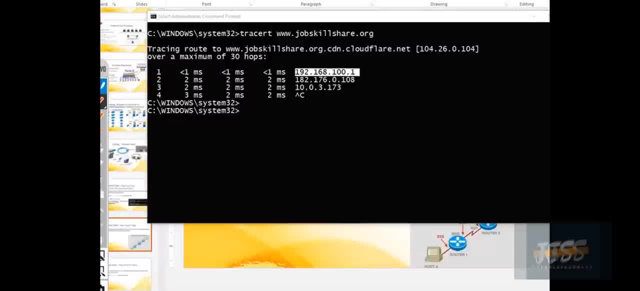 another thing i want to clarify here, uh, another thing i want to clarify here, uh, another thing i want to clarify here. uh, just tanish mentioned the switches. just tanish mentioned the switches. just tanish mentioned the switches. sometimes you know the switches, sometimes you know the switches. 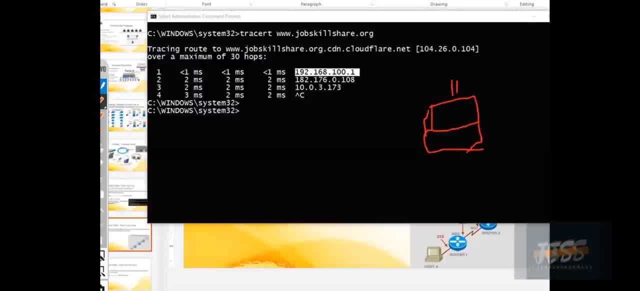 sometimes you know the switches, they are, they are, they are the dumb devices. they don't have ips, okay, okay, okay. so sometimes the tracer will not work, so sometimes the tracer will not work. so sometimes the tracer will not work for these switches, for these switches, for these switches, if we have, let's say we have- multiple. 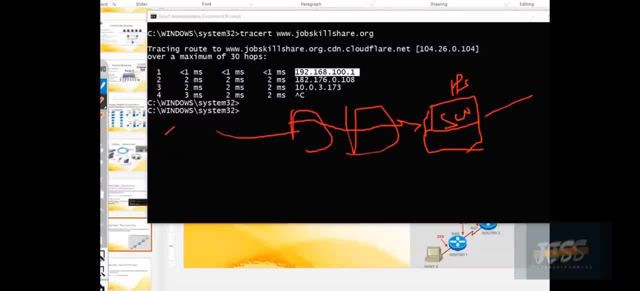 if we have, let's say we have multiple. if we have, let's say we have multiple switches connected like a daisy chain, switches connected like a daisy chain, switches connected like a daisy chain, fashion, fashion, fashion, and i will run tracer command from this and i will run tracer command from this. 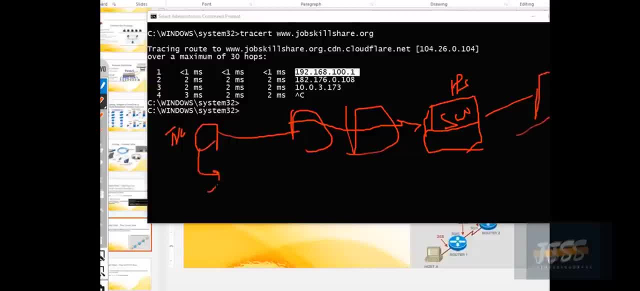 and i will run tracer command from this machine to this destination machine to this destination machine to this destination. it is gonna tell me you are one hop away. it is gonna tell me you are one hop away. it is gonna tell me you are one hop away because it will not consider these. because it will not consider these, because it will not consider these switches as switches, as switches as a routers, because they don't have any a routers, because they don't have any a routers, because they don't have any kind of ip connectivity, kind of ip connectivity, kind of ip connectivity, and it will not consider these like the. 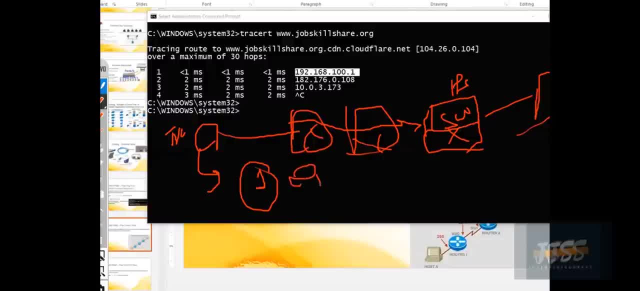 and it will not consider these like the and it will not consider these like the bumps in the wire. bumps in the wire, bumps in the wire. if we have the routers here, if we have the routers here, if we have the routers here, then, yes, this is three hops away. 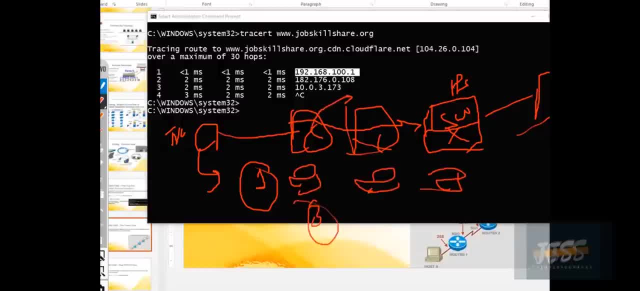 then yes, this is three hops away. then yes, this is three hops away, but but? but these days, switches are intelligent enough. these days, switches are intelligent enough. these days, switches are intelligent enough. you can have switch, you can have switch, you can have switch plus the router inside that device. it is. 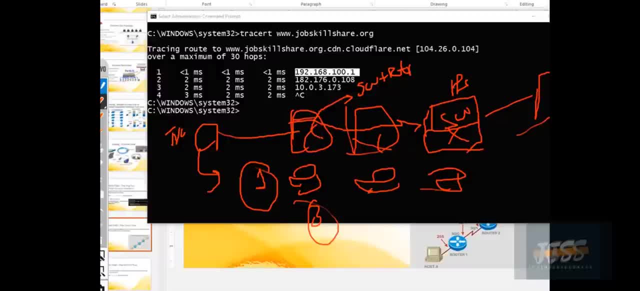 plus the router inside that device. it is plus the router inside that device. it is works as a switch as well as a router, works as a switch as well as a router, works as a switch as well as a router. then in that case, if we have these, 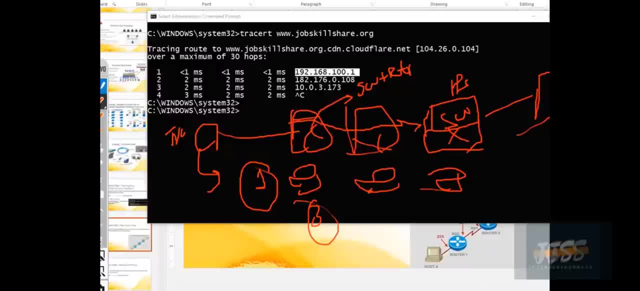 then in that case, if we have these, then in that case, if we have these things, then it will show the three hops things. then it will show the three hops things, then it will show the three hops. i hope you get it. i hope you get it. i hope you get it. yep, thank you, that was a good example. 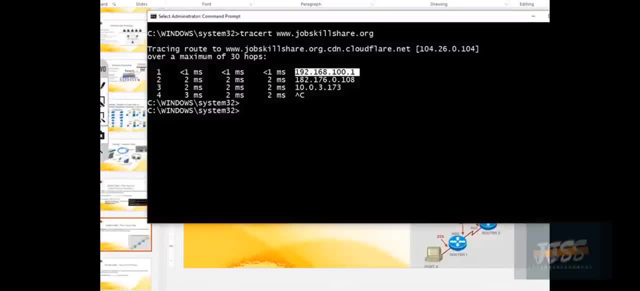 yep, thank you, that was a good example. yep, thank you, that was a good example. because, because, because some people may not know that, yeah you, some people may not know that, yeah you, some people may not know that, yeah, you can have it when you, when you, when people. 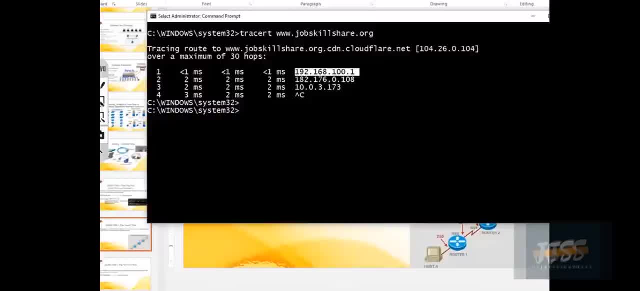 can have it when you, when you, when people can have it when you, when you, when people ask you about that, ask you about that, ask you about that? oh didn't, i hear that there are. oh, didn't i hear that there are. oh, didn't i hear that there are switches on layer 3? that's what he's. 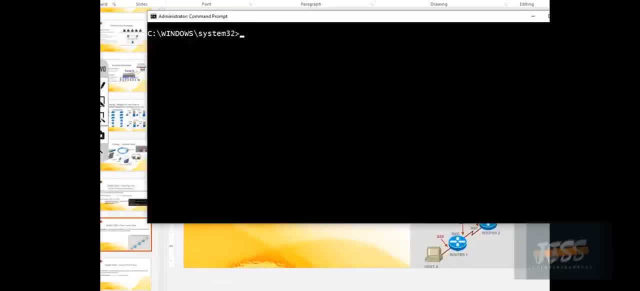 switches on layer 3. that's what he's. switches on layer 3. that's what he's talking about, that. talking about that. talking about that, anyone comes with that capabilities. it's, anyone comes with that capabilities. it's anyone comes with that capabilities. it's not that the whole switch is. 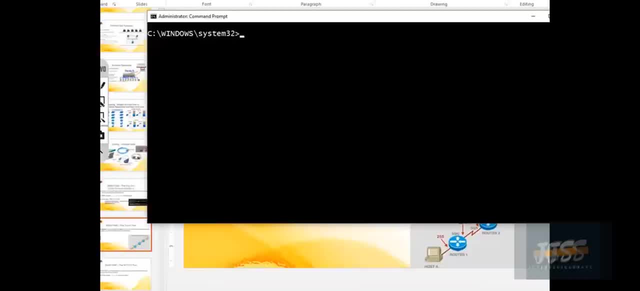 not that the whole switch is not that the whole switch is like a router, it's just the capability is like a router. it's just the capability is like a router. it's just the capability is being added to it being added to it being added to it. yes, right, okay, then we can go in detail. 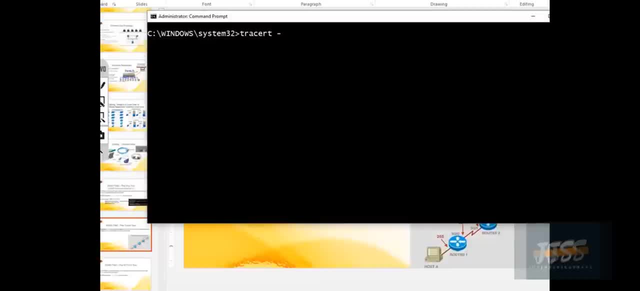 yes, right, okay, then we can go in detail. yes, right, okay, then we can go in detail about pressure, and the same method way about pressure and the same method way about pressure, and the same method way we did with the ping tracer minor minus, we did with the ping tracer minor minus. 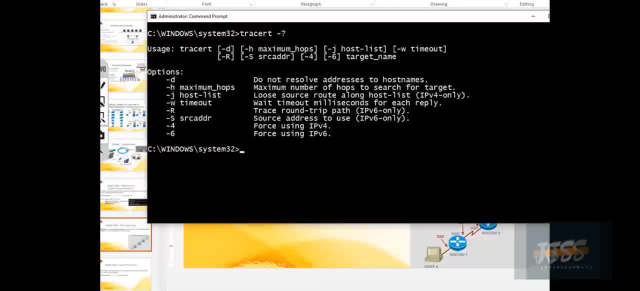 we did with the ping tracer minor minus and the question mark and you will see, and the question mark and you will see, and the question mark and you will see, there is not much going on in the, there is not much going on in the, there is not much going on in the tracer, as opposed to the pain, 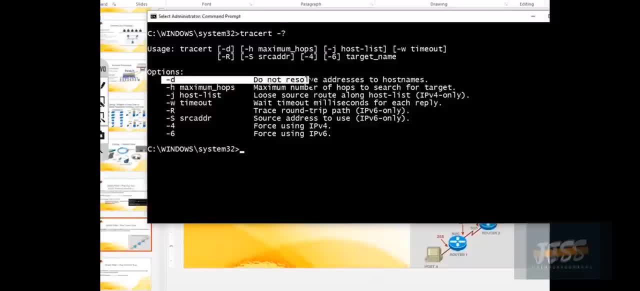 tracer as opposed to the pain, tracer as opposed to the pain. but this will go for the ipv6 only as. but. this will go for the ipv6 only as. but this will go for the ipv6 only as you can see. you can see, you can see, so uh. 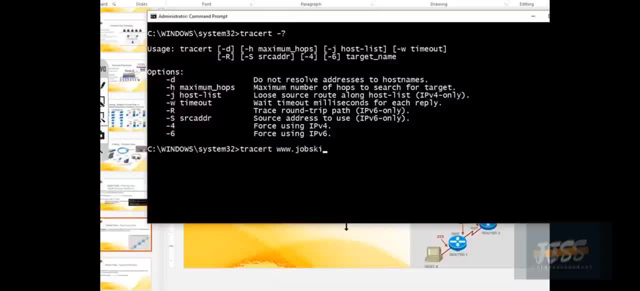 so, uh, so uh, i did tracer and i did, i did tracer and i did, i did tracer and i did wwwjobskillshareorg, wwwjobskillshareorg, wwwjobskillshareorg, and uh sorry and uh sorry and uh sorry, there's a typo in there. 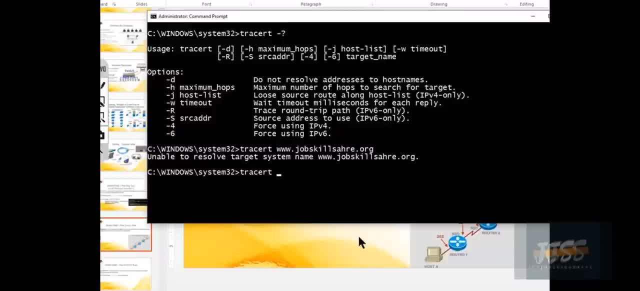 uh tracer, uh tracer, uh tracer, then, then, then, drop skill shareorg, drop skill shareorg, drop skill shareorg. yeah, as you can see, it is taking so long. yeah, as you can see, it is taking so long. yeah, as you can see it is taking so long here. why? 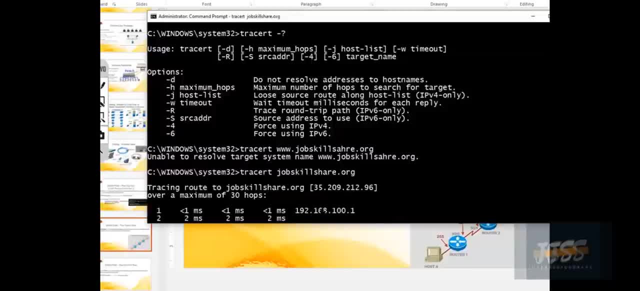 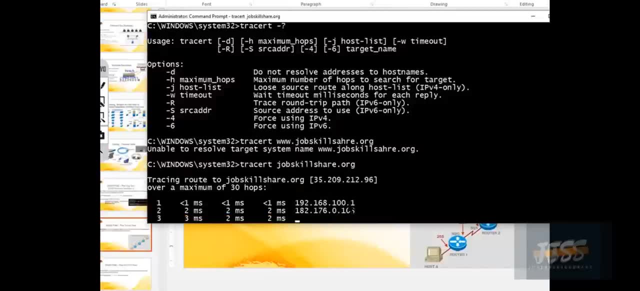 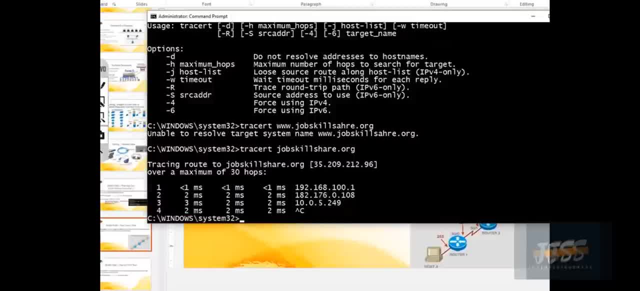 this name of this host machine. this name of this host machine, so every time it hit this device is so every time it hit this device is so every time it hit this device is trying to resolve on it this we don't do. trying to resolve on it this we don't do. 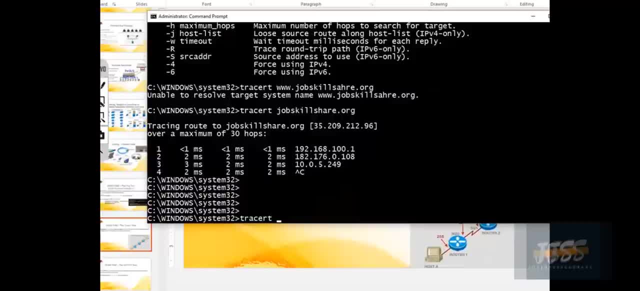 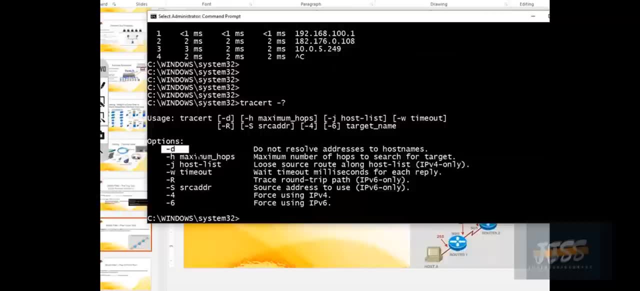 trying to resolve on it. this we don't, do not want, not want, not want. so what is the solution for that? you want to process preset, uh. you want to process preset, uh. you want to process preset, uh. very fast with the help of minus d. very fast, with the help of minus d. 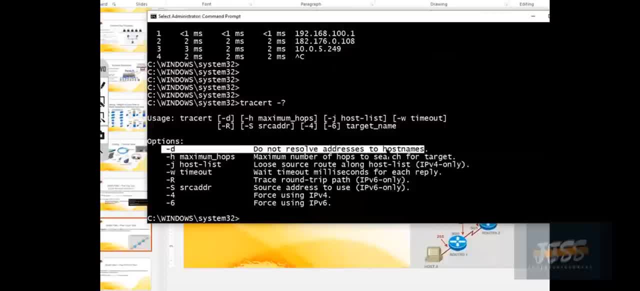 very fast with the help of minus d. and it is clearly mentioning here: do not. and it is clearly mentioning here: do not. and it is clearly mentioning here: do not resolve address to host, resolve, address to host, resolve, address to host. so the same thing we're gonna um. 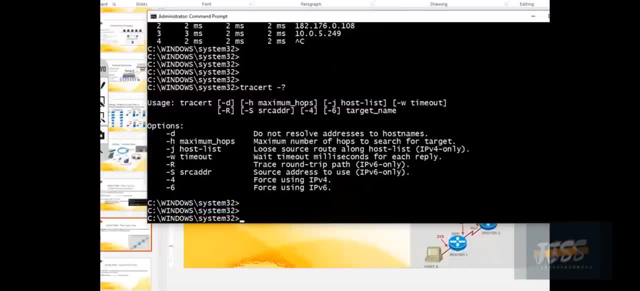 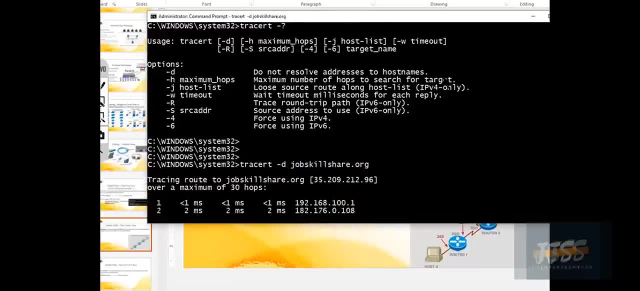 so the same thing, we're gonna um. so the same thing, we're gonna um. do with the help of minus d command and do with the help of minus d command. and do with the help of minus d command and you will see the difference. you can type minus d option here and now. 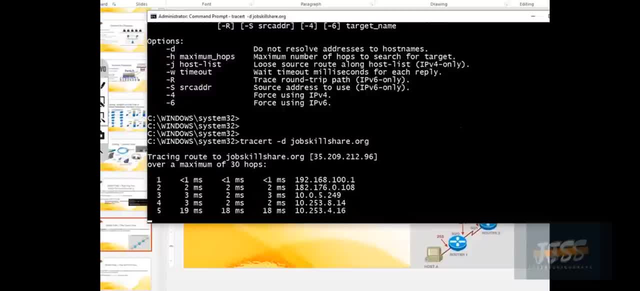 you can type minus d option here and now. you can type minus d option here and now. as you can see, this is much more quicker. as you can see, this is much more quicker. as you can see, this is much more quicker than before, than before, than before. now we can clearly see how far jobs 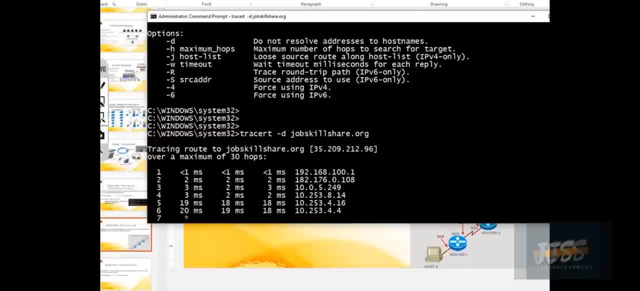 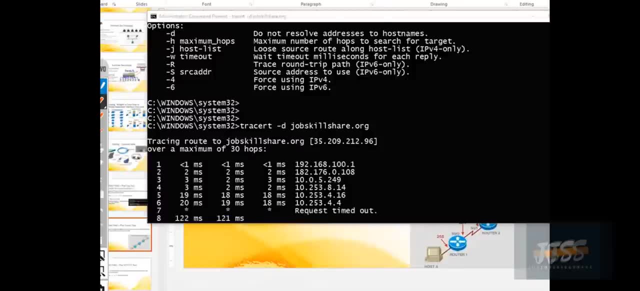 now we can clearly see how far jobs. now we can clearly see how far jobs gets here. or this promise- another thing very important here did you another thing very important here did you. another thing very important here. did you notice these sterics? notice these sterics. notice these sterics whenever you come across this character. 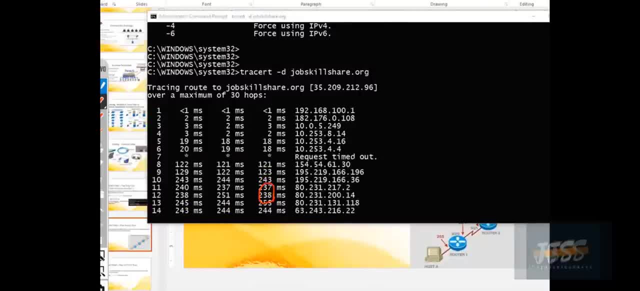 whenever you come across this character. whenever you come across this character, it doesn't mean that this device is not. it doesn't mean that this device is not. it doesn't mean that this device is not responding. this device is responding, but responding. this device is responding, but 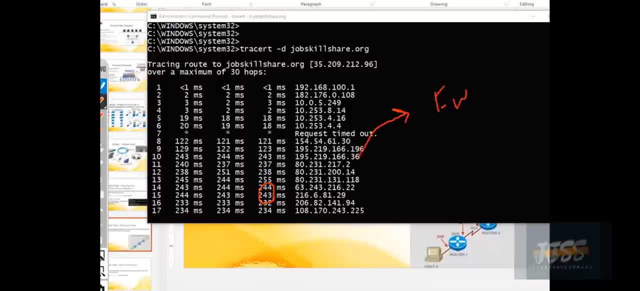 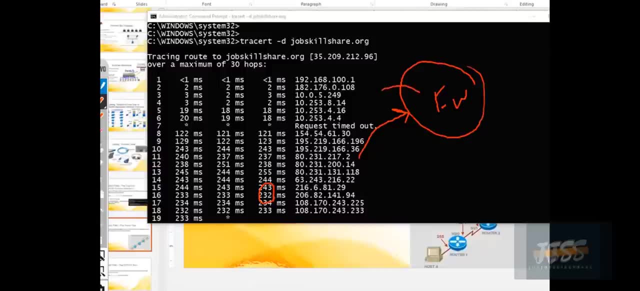 responding. this device is responding, but basically there is kind of firewall. basically there is kind of firewall. basically there is kind of firewall device device. device is installed, is installed, is installed. that is denying these icm ppings. that is denying these icm ppings. that is denying these icm ppings. uh, to hit this, uh. 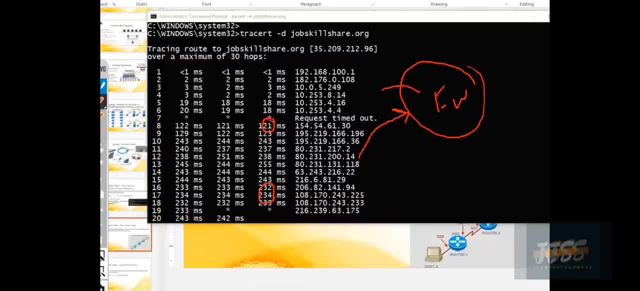 uh to hit this, uh, uh to hit this, uh, host machine, host machine, host machine. so this is for the security mechanism, so this is for the security mechanism, so this is for the security mechanism. so, since you know this, uh job skills here. so, since you know this, uh job skills here. 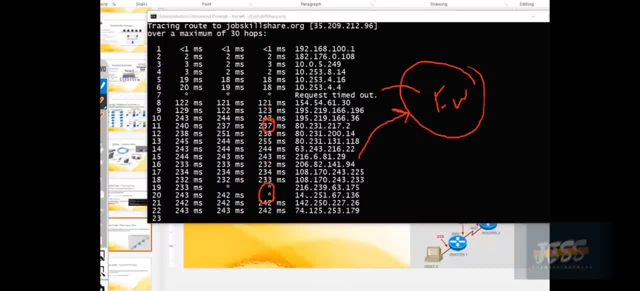 so, since you know this, uh, job skills here. i think this is located in somewhere in. i think this is located in somewhere in. i think this is located in somewhere in united states and it is far, far, far away, united states, and it is far, far, far away. 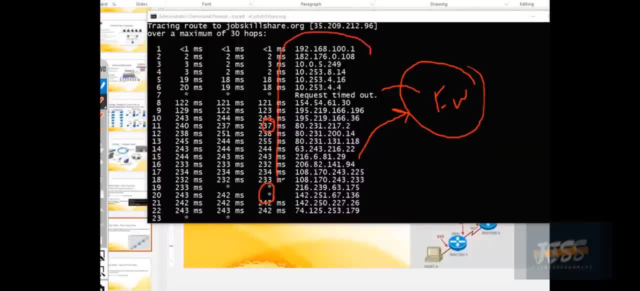 united states and it is far, far, far away from us in the pakistan, as you can see, from us in the pakistan, as you can see from us in the pakistan, as you can see, there is a lot, there is a lot, there is a lot of routers. basically, it is all routers. 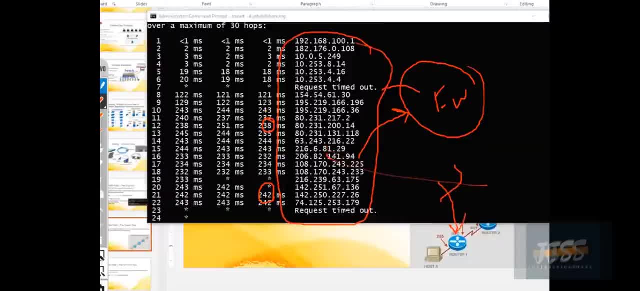 of routers. basically it is all routers of routers. basically it is all routers, these things, these things, these things. can we say that now it took some type of? can we say that now it took some type of? can we say that now it took some type of path or a best path? or is that a correct? 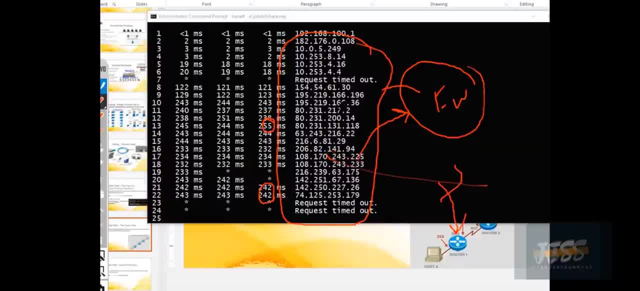 path or a best path? or is that a correct path or a best path? or is that a correct term to use, term to use term, to use exactly? you can use uh, for example: uh. you, exactly. you can use uh, for example. uh. you exactly. you can use uh, for example: uh, you can uh. 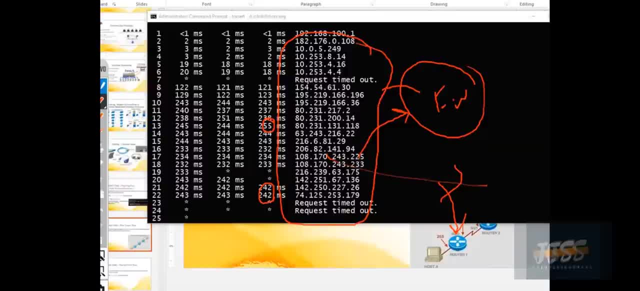 can uh, can uh. if job skip share has multiple servers. if job skip share has multiple servers, if job skip share has multiple servers, okay, then it is not going to use always. okay, then it is not going to use always. okay, then it is not going to use always the same path. maybe it will use some. 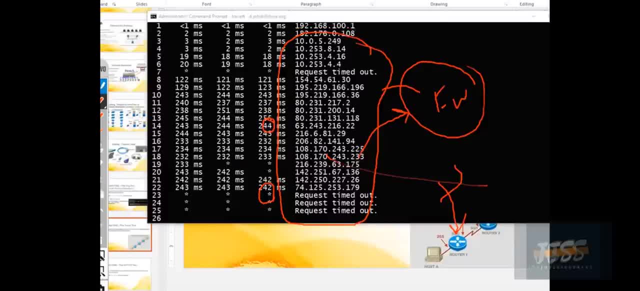 the same path. maybe it will use some the same path, maybe it will use some different path, different path, different path. it find it better than the other one. it find it better than the other one. it find it better than the other one. so from here you can also. 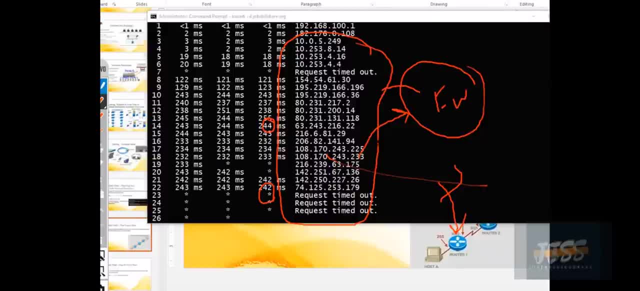 so from here you can also. so from here you can also see that sometimes you are hitting less. see that sometimes you are hitting less. see that sometimes you are hitting less routers, routers, routers than before than before, than before. okay, sorry, i'm eating, yes, okay, sorry, i'm eating, yes, okay. 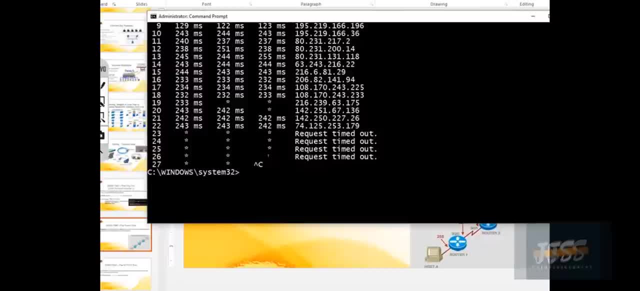 sorry, i'm eating. yes, okay, so i just uh, i press ctrl, so i just uh, i press ctrl, so i just uh, i press ctrl plus c, plus c, plus c, uh to disconnect this one, because it is uh to disconnect this one, because it is uh to disconnect this one because it is taking so long. 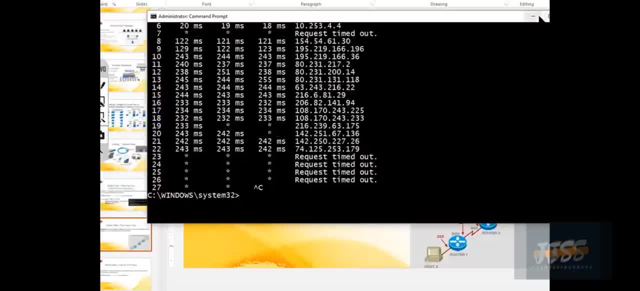 taking so long, taking so long. so this is preset command and, as i said, so, this is preset command and, as i said, so, this is preset command and, as i said, this is very helpful tool. this is very helpful tool. this is very helpful tool. uh, when you have multiple 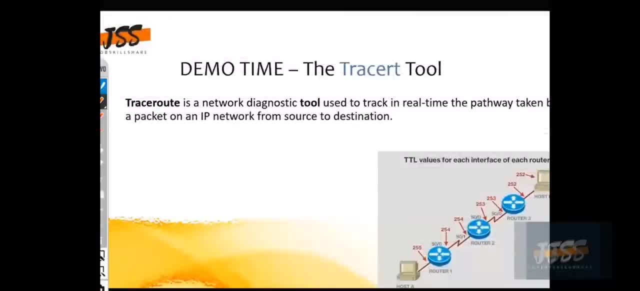 uh when you have multiple, uh, when you have multiple, when you have multiple devices in between, when you have multiple devices in between, when you have multiple devices in between, like routers, like routers, like routers, and we have no idea which device for. and we have no idea which device for. 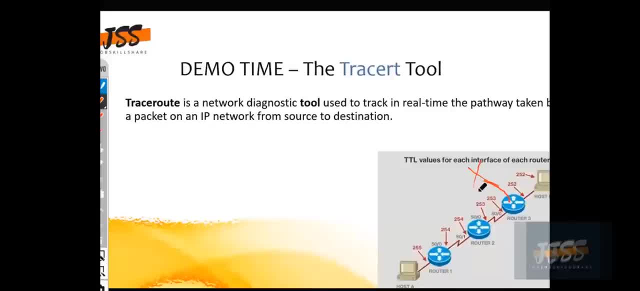 and we have no idea which device, for example. this one is example. this one is example. this one is: uh disconnected at shutdown, uh, disconnected at shutdown, uh, disconnected at shutdown. then we have reachability all the way, then we have reachability all the way, then we have reachability all the way up till this. 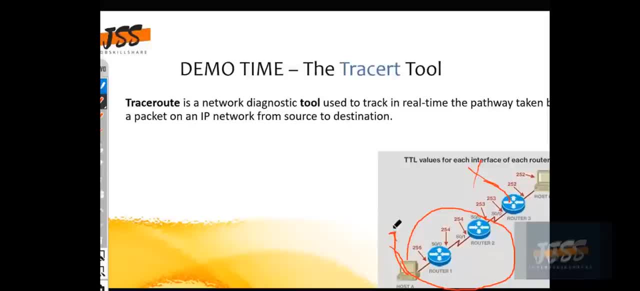 if, if i'm trying to pick from this, if, if i'm trying to pick from this, so this is how i'm going to. so this is how i'm going to. so this is how i'm going to: uh, imagine that, uh, uh, imagine that, uh, uh, imagine that, uh, we have the problem somewhere in this. 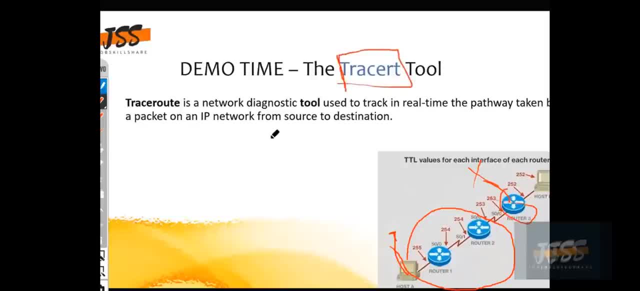 we have the problem somewhere in this. we have the problem somewhere in this folder, folder, folder. so that's is where pressure tool is being so that's is where pressure tool is being so that's is where pressure tool is being used and this is very helpful used and this is very helpful. 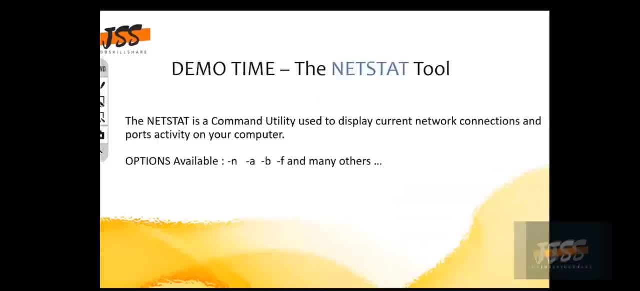 used and this is very helpful in your day-to-day uh working net stat. in your day-to-day uh working net stat. in your day-to-day uh working net stat: tool tool tool. uh, uh, uh. you can consider this is like the. you can consider this is like the. 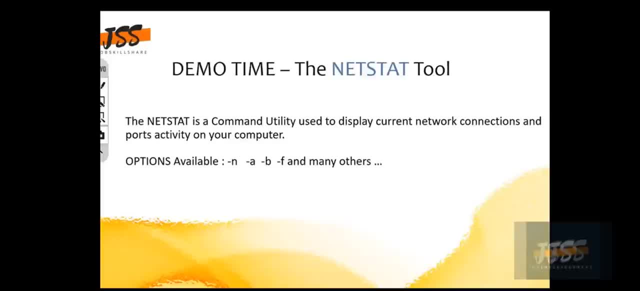 you can consider this is like the monitoring tool, monitoring tool, monitoring tool and basically what it is the next. that and basically what it is the next that and basically what it is the next that is a command utility utility used to. is a command utility utility used to. 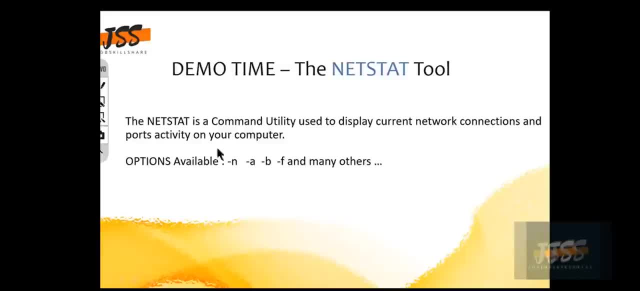 is a command utility utility used to display current network connections. and display current network connections. and display current network connections and the port activity on your computer. the port activity on your computer. the port activity on your computer. what does it mean? it means uh, whatever. what does it mean it means uh, whatever. 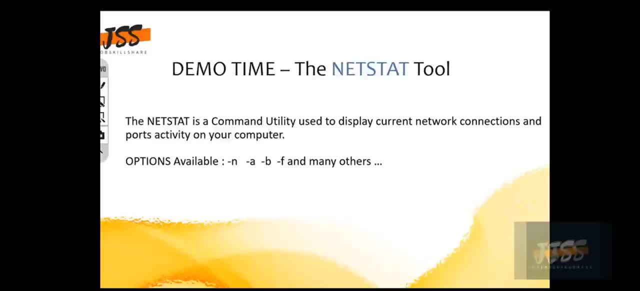 what does it mean? it means, uh, whatever the connectivity or the connections, is the connectivity or the connections, is the connectivity or the connections is going through from from my computer, going through from from my computer, going through from from my computer or coming to my computer? i can see. 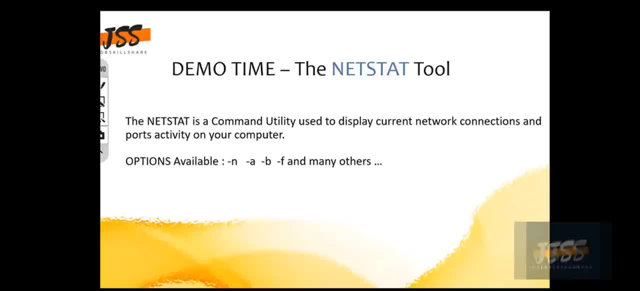 or coming to my computer, i can see. or coming to my computer, i can see what ports it is connected with, what ports it is connected with, what ports it is connected with: uh, whether i'm using chrome, uh, what? uh? whether i'm using chrome, uh, what? uh? whether i'm using chrome, uh, what other applications like we have. 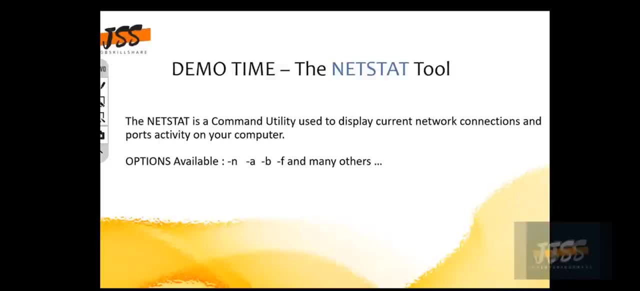 other applications. like we have other applications, like we have discord. we have skype. what kind of discord we have skype? what kind of discord we have skype? what kind of connections are connected on? my connections are connected on. my connections are connected on my computers. right now we can take a look. 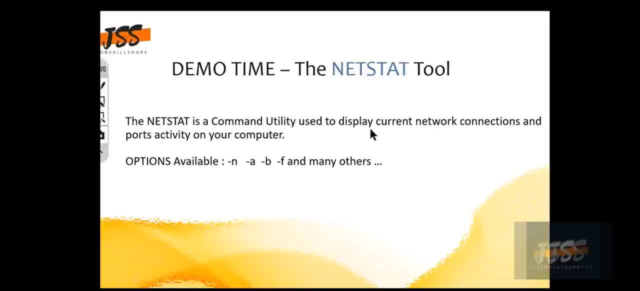 computers: right now we can take a look. computers, right now we can take a look from using next step 2.. from using next step 2.. from using next step 2.. so let's go into the. so let's go into the, so let's go into the demo. 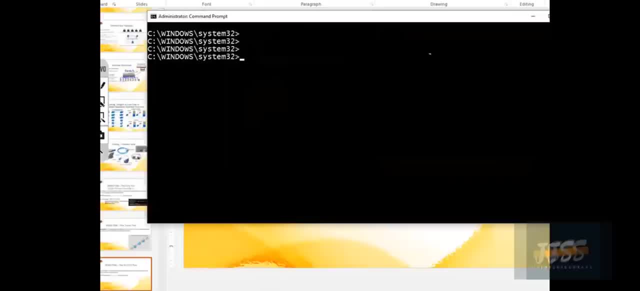 demo, demo. let's clear the screen. let's clear the screen. let's clear the screen. if i will do simply next step, if i will do simply next step, if i will do simply next step, without any option. as you can see, it is saying active. as you can see, it is saying active. 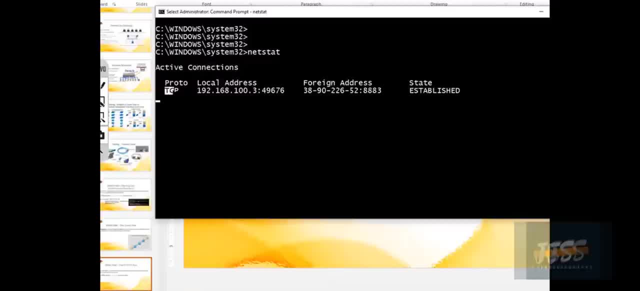 as you can see, it is saying active connections, connections, connections. what protocol my connection is using tcp? what protocol my connection is using tcp? what protocol my connection is using tcp? what is the local address of my system? what is the local address of my system? what is the local address of my system? 192.168.100.3. 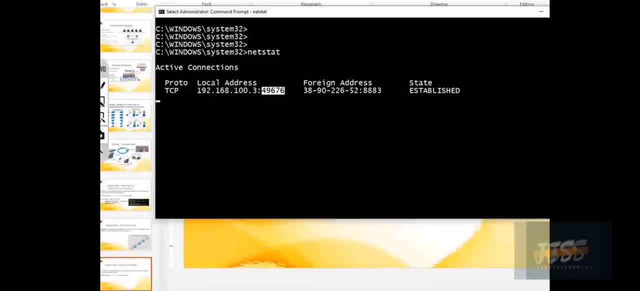 192.168.100.3, 192.168.100.3. and it is showing me the port address which, and it is showing me the port address which: and it is showing me the port address which is is is i told you, this is the random port. 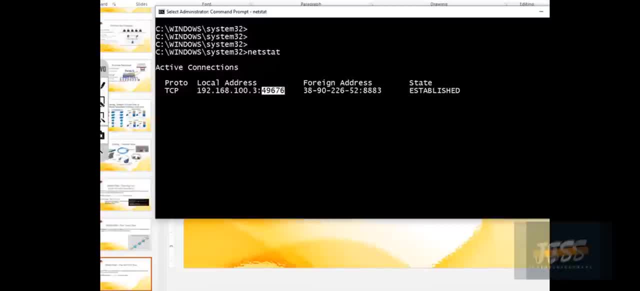 i told you this is the random port. i told you this is the random port and it is not well known port and it is not well known port and it is not well known port. it is the state is established. it is the state is established. it is the state is established, and is it? it is connected with the. 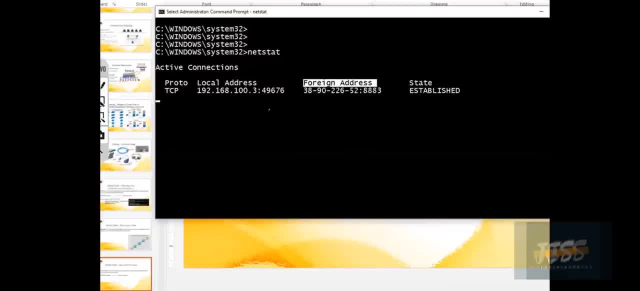 and is it it is connected with the and is it it is connected with the foreign address, which is which is foreign address, which is which is foreign address, which is which is located somewhere far, located somewhere, far, located somewhere far from my computer, from my computer, from my computer, and this is the ip which is going to be. 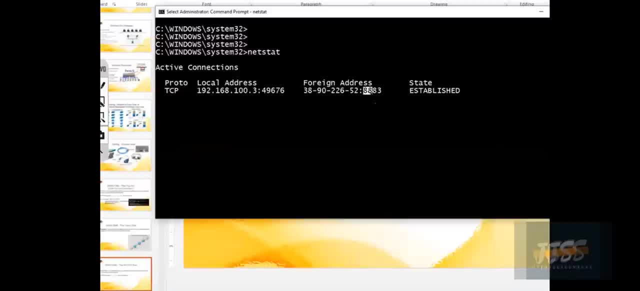 and this is the ip which is going to be and this is the ip which is going to be the public ip and this is connected with the public ip and this is connected with the public ip and this is connected with that 8883 um, that 8883 um. 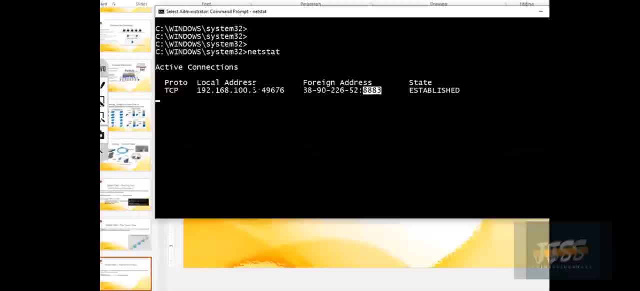 that 8883. um, maybe this is like the well-known port. maybe this is like the well-known port. maybe this is like the well-known port, but it is very slow again. the problem is, but it is very slow again. the problem is, but it is very slow again. the problem is it is trying to resolve the 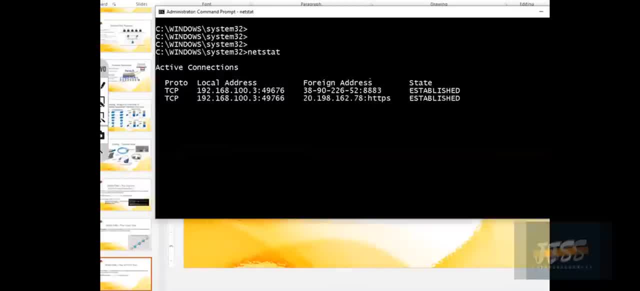 it is trying to resolve the. it is trying to resolve the host, or the dns information host, or the dns information host or the dns information. so what is the remedy? the same way, we can go next at the same way, we can go next at the same way. we can go next at minus question mark. 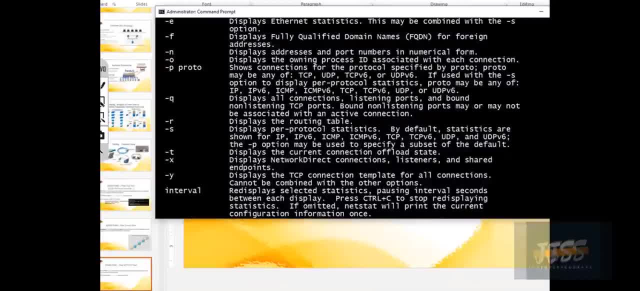 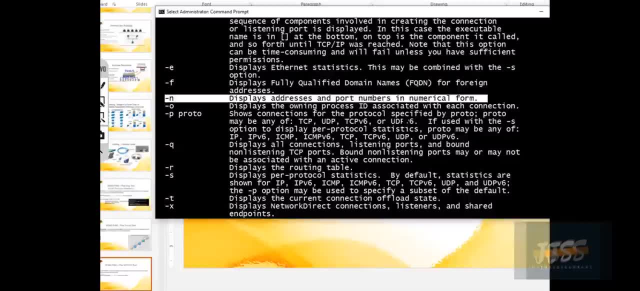 and then we can come here display the, and then we can come here display the. and then we can come here display the address: address: address: sorry, displays addresses and phone number. in displays addresses and phone number. in displays addresses and phone number in numerical form: numerical form: numerical form. let's try again with that minus n. 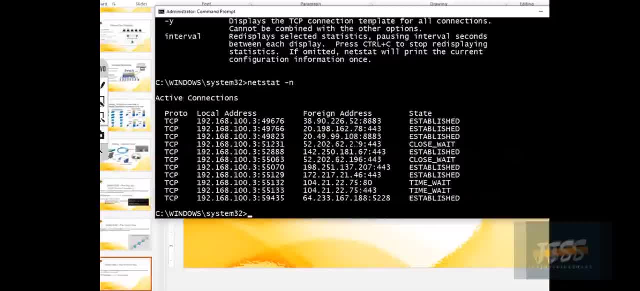 let's try again with that minus n. let's try again with that minus n and hit enter as you can see very quickly, and hit enter as you can see very quickly and hit enter as you can see very quickly: processed, processed, processed. which was? it was going to take time here. 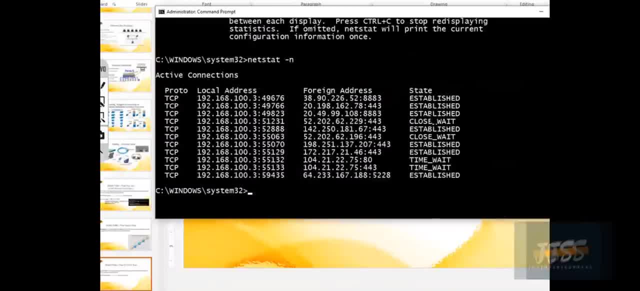 which was it was going to take time here, which was it was going to take time here. so we can see the same information, so we can see the same information, so we can see the same information. uh, uh, uh. that connection is established, we have. that connection is established, we have. 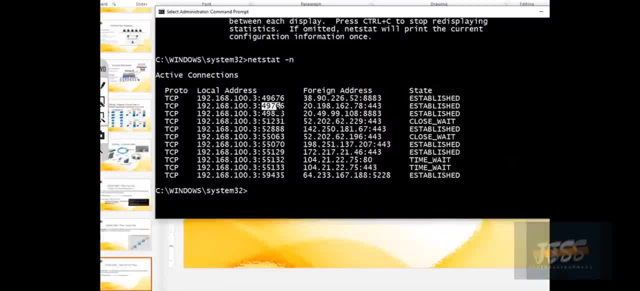 that connection is established. we have multiple local connections, multiple local connections, multiple local connections: uh, from the different ports going to the uh, from the different ports going to the uh, from the different ports going to the well-known ports like 443 is a well-known, well-known ports like 443 is a well-known. 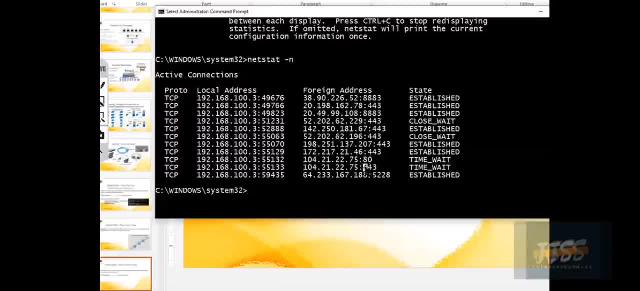 well-known ports like 443 is a well-known port, port. port. this is secure. non-secure. 443 is secure. this is secure. non-secure. 443 is secure. this is secure. non-secure 443 is secure and 80 is and 80 is. 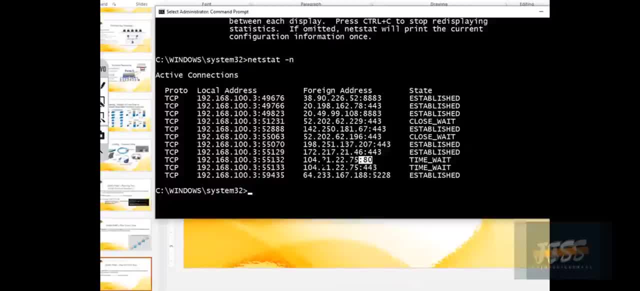 and 80 is non-secure, non-secure, non-secure. now i want to go, now, i want to go. now, i want to go one step further and i want to convert one step further, and i want to convert one step further and i want to convert these into the names. 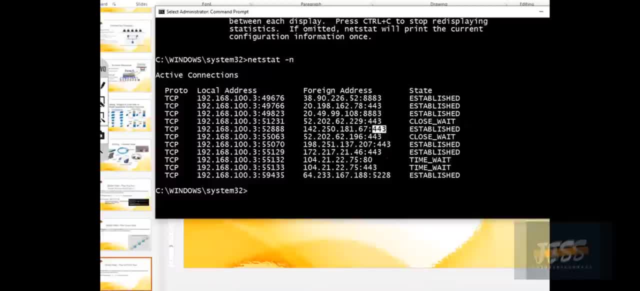 these into the names, these into the names i don't want, i don't know. for example, i'm, i don't want, i don't know. for example, i'm, i don't want, i don't know. for example, i'm very, uh, at the very basic level i have. 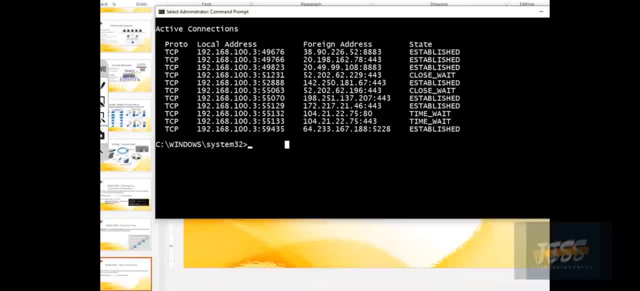 very uh at the very basic level. i have very uh at the very basic level. i have no idea what 443 statue, so further you. no idea what 443 statue, so further you. no idea what 443 statue, so further you. can dig deep and check. can dig deep and check. 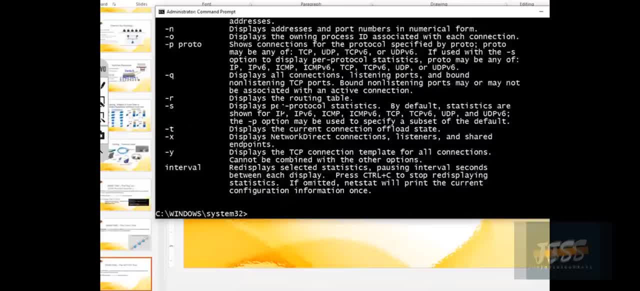 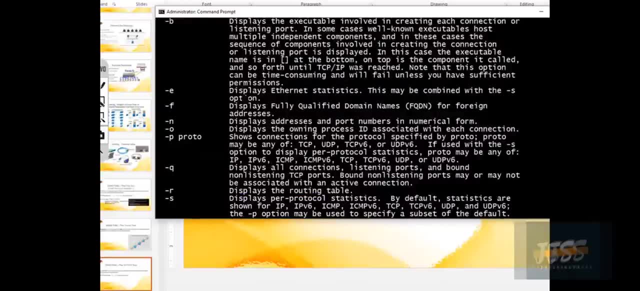 can dig deep and check that stat and type minus question to see that stat and type minus question. to see that stat and type minus question to see which options will enable that for us, which options will enable that for us, which options will enable that for us. uh. 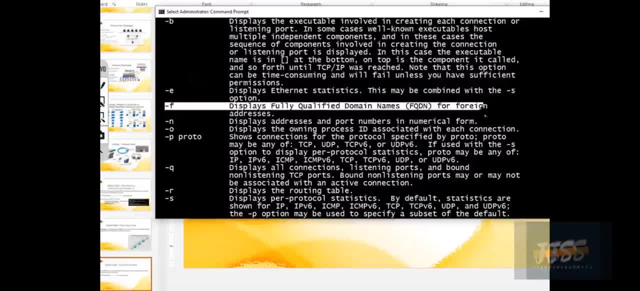 then we have fully qualified dna domain. then we have fully qualified dna domain, then we have fully qualified dna domain names as well. names as well, names as well. uh, let's try this minus b. uh, let's try this minus b. uh, let's try this minus b. displays the executable involved in. 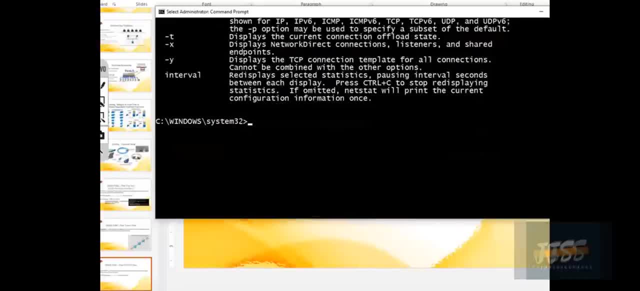 displays the executable involved in. displays the executable involved in creating, creating, creating, creating in creating. in each connection listening code. let's each connection listening code. let's each connection listening code. let's try this one, try this one, try this one minus b, and this minus b option basically is: 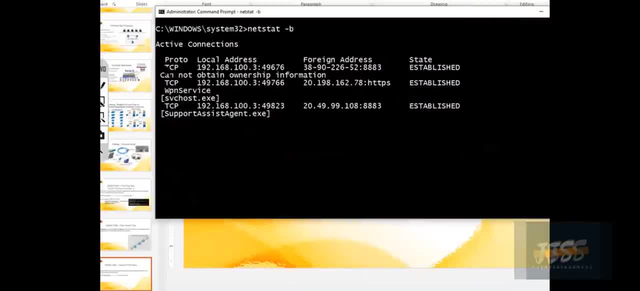 and this minus b option basically is. and this minus b option basically is: giving me information. not only uh what giving me information, not only uh what giving me information, not only uh what kind of protocol i'm using, but also what kind of protocol i'm using, but also what. 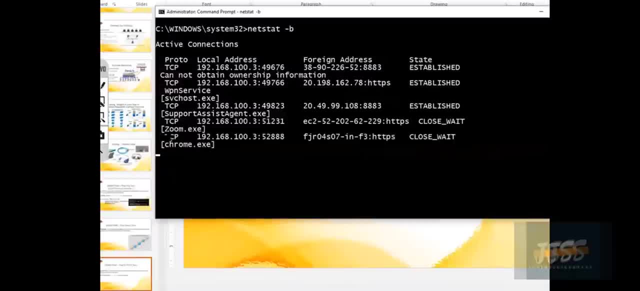 kind of protocol i'm using, but also what kind of application i'm using, kind of application i'm using, kind of application i'm using. so you can imagine how this could be. so you can imagine how this could be. so you can imagine how this could be. yeah, this could be a. 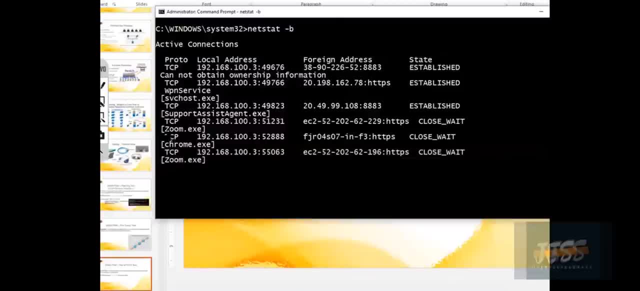 yeah, this could be a. yeah, this could be a great, great, great way to find out if somebody way to find out, if somebody way to find out, if somebody complaining about you know- hey, i complaining about you know, hey, i complaining about you know, hey, i, i'm having a lot of issues. my computer is. 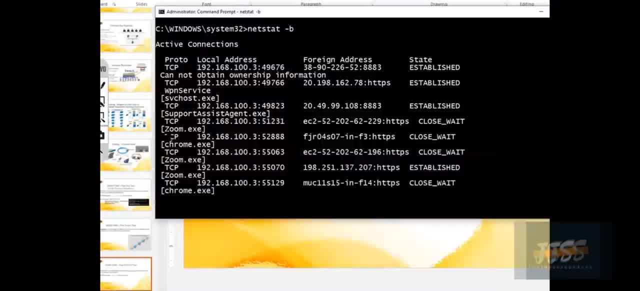 i'm having a lot of issues. my computer is. i'm having a lot of issues. my computer is very slow, very slow, very slow. or my computer is being like you know, or my computer is being like you know, or my computer is being like you know, doing weird stuff, but they can't see it. 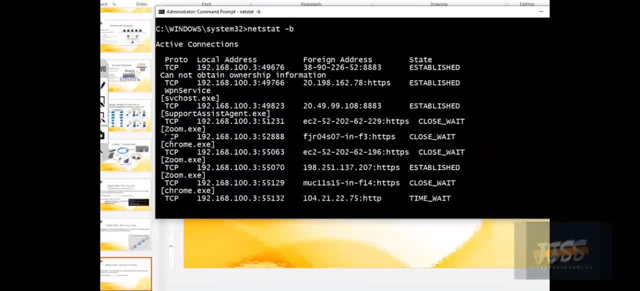 doing weird stuff, but they can't see it doing weird stuff, but they can't see it. right, right, right. this could be a great way to actually. this could be a great way to actually. this could be a great way to actually run this command and find out if there's. 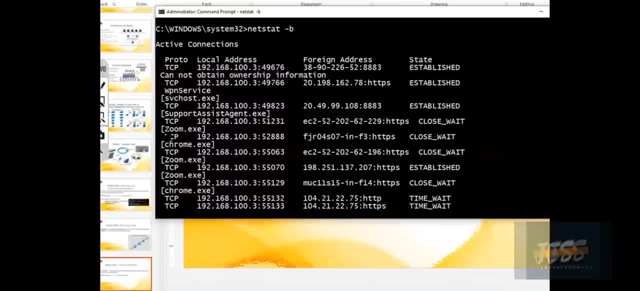 run this command and find out if there's. run this command and find out if there's a background application that's doing a, a background application that's doing a, a background application that's doing a lot of stuff, lot of stuff, lot of stuff, from the command line exactly, and 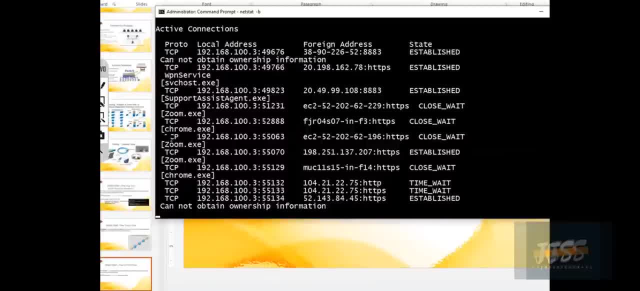 from the command line exactly, and from the command line exactly, and somebody raised this question as well. somebody raised this question as well. somebody raised this question as well earlier that, earlier that, earlier that um, if i disable, or one port out, so as. um, if i disable, or one port out, so as. 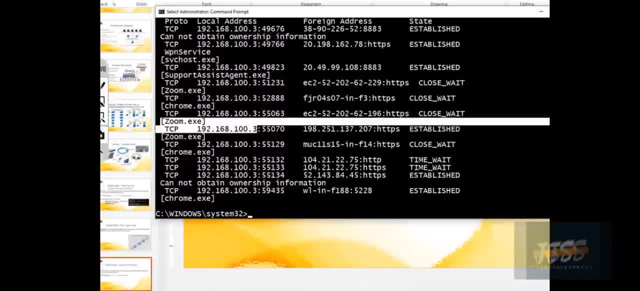 um, if i disable or one port out. so, as you can see clearly, here is zoom at the. you can see clearly, here is zoom at the. you can see clearly, here is zoom at the zoom, zoom, zoom. what kind of protocols, uh, the port number, what kind of protocols, uh, the port number. 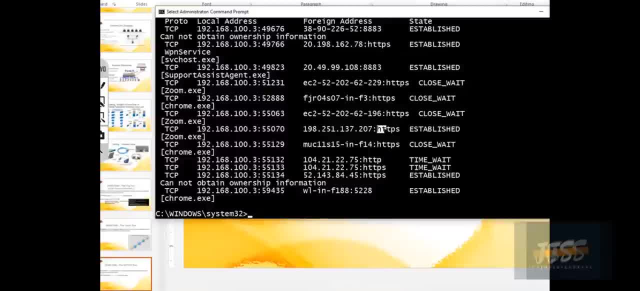 what kind of protocols? uh, the port number. it is running as a source. it is running as a source. it is running as a source and it is using the well-known port at. and it is using the well-known port at. and it is using the well-known port at ppps. 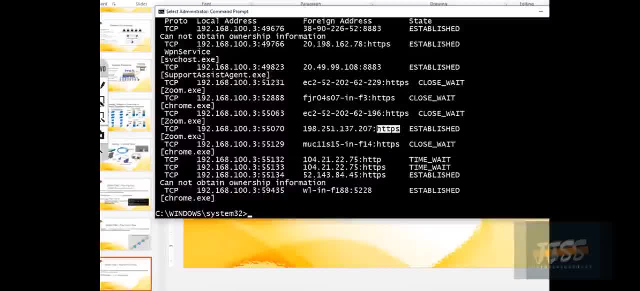 ppps, ppps. so it means zoom is using a very secure. so it means zoom is using a very secure. so it means zoom is using a very secure connection, connection connection. sorry if i'm getting ahead of myself, but sorry if i'm getting ahead of myself, but 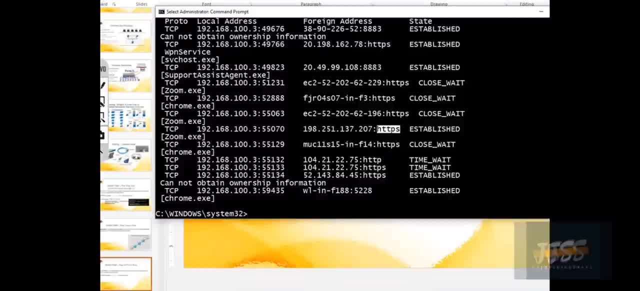 sorry if i'm getting ahead of myself, but what's the difference between? what's the difference between? what's the difference between: establishes but close, wait and time wait, but close, wait and time wait, but close, wait and time wait. okay. so establish is basically: this is okay. so establish is basically this is. 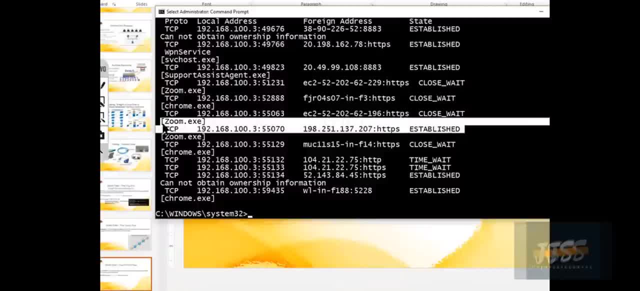 okay, so establish is basically: this is i'm connected with, i'm connected with, i'm connected with: okay, this connection is currently okay. this connection is currently okay. this connection is currently established. established. established, and these are previous connection which, and these are previous connection which and these are previous connection which is waiting to close. 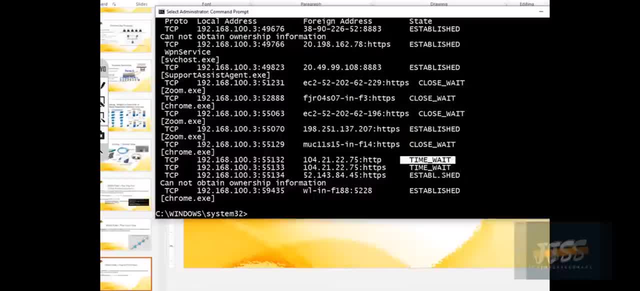 and similarly, time wait is it has. and similarly, time wait is it has. and similarly, time wait is it has already expired, already expired, already expired. like it's wait, like it's wait, like it's wait. i don't like when you say establish. i don't like when you say establish. 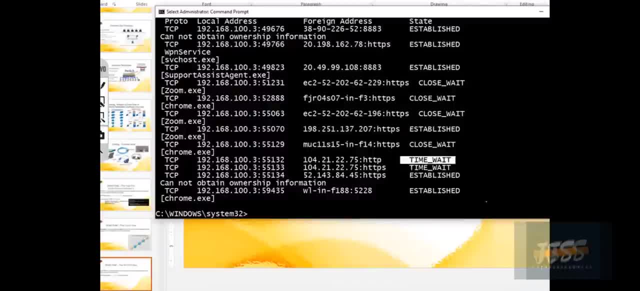 i don't like when you say: establish you're actively in that session paper, you're actively in that session paper, you're actively in that session paper, yes, so no, no, i get that one, i just i. yes so no, no, i get that one, i just i. 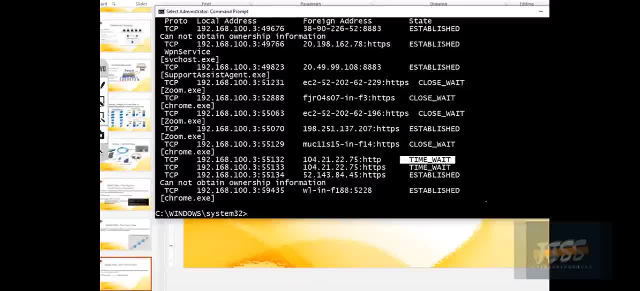 yes, so no, no, i get that one. i just i don't get time. wait, don't get time. wait, don't get time. wait like it's. like, it's like it's expired, expired, expired. yes, it is expired. yes, it is expired. yes, it is expired. this is like you can say: consider it. 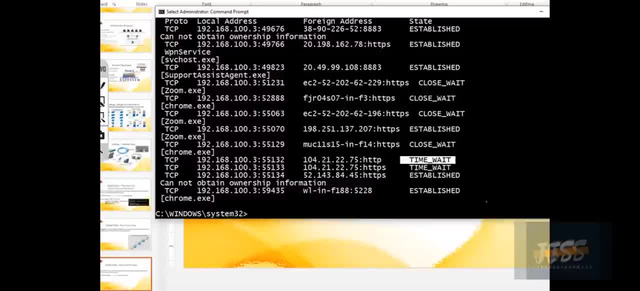 this is like you can say, consider it. this is like you can say: consider it like the session that like the session. that like the session that along over it happened now. it is waiting along over it happened now. it is waiting along over it happened now. it is waiting to time out. 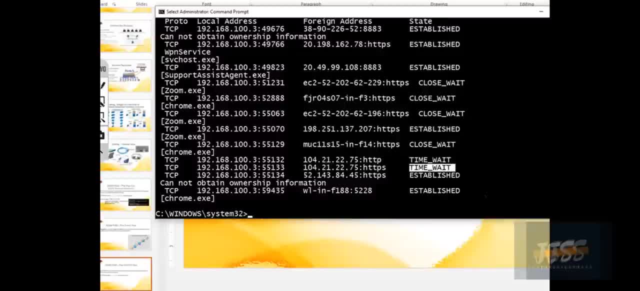 to time out, to time out. in short, yeah, so your computer, your computer is. yeah, so your computer, your computer is. yeah, so your computer, your computer, is going to keep going to keep going to keep some kind of some kind of some kind of- you know- connection to close down it. 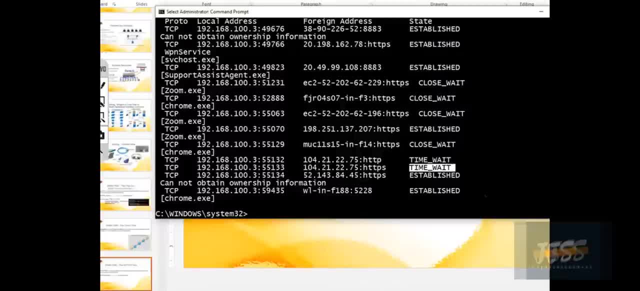 you know connection to close down it. you know connection to close down it won't just immediately close everything, won't just immediately close everything won't just immediately close everything. do you remember we, we talked about the? do you remember we, we talked about the? do you remember we, we talked about the sessions? 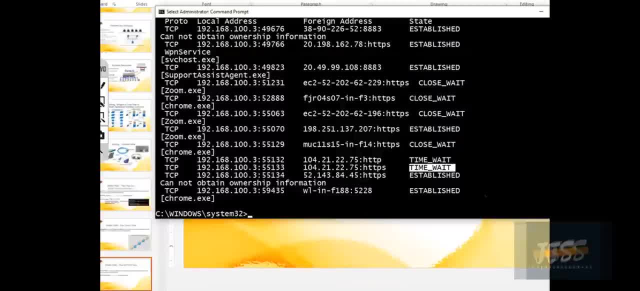 sessions, sessions. yeah, like it's good the session goes. yeah, like it's good the session goes. yeah, like it's good, the session goes on. yes on, yes on. yes, there are several sessions going on and there are several sessions going on, and there are several sessions going on and some of them are waiting to time out. 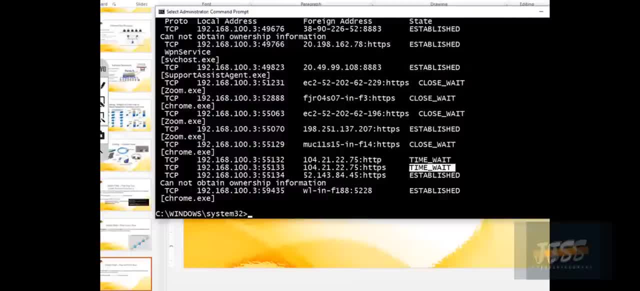 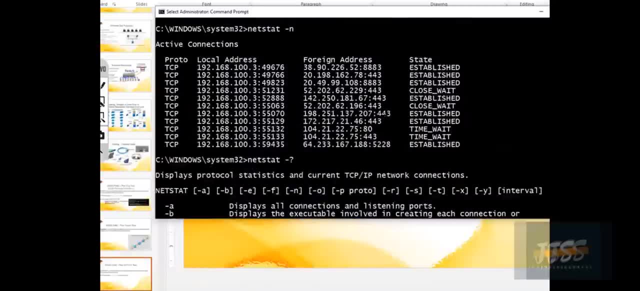 some of them are waiting to time out. some of them are waiting to time out okay, okay, okay, okay. and, as i said, and as i said, and as i said before, it was giving me information about before it was giving me information about before, it was giving me information about just the port numbers. 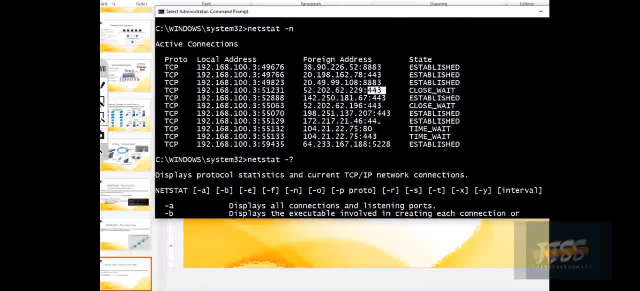 just the port numbers. just the port numbers. uh, if, uh, if, uh, if. i'm a newbie, i have no idea what these. i'm a newbie. i have no idea what these. i'm a newbie, i have no idea what these ports are. i can enable this switch. 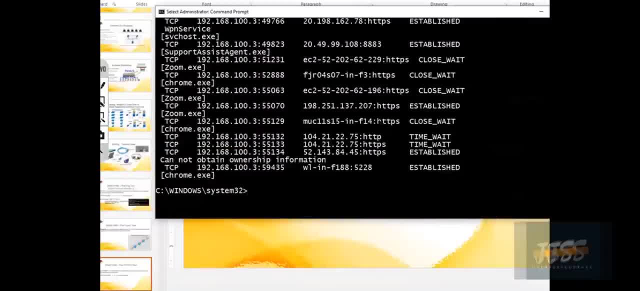 ports are i can enable this. switch ports are i can enable this: switch: minus b, minus b, minus b, uh, which is basically going to turn those uh, which is basically going to turn those uh, which is basically going to turn those into into, into the name xptps. 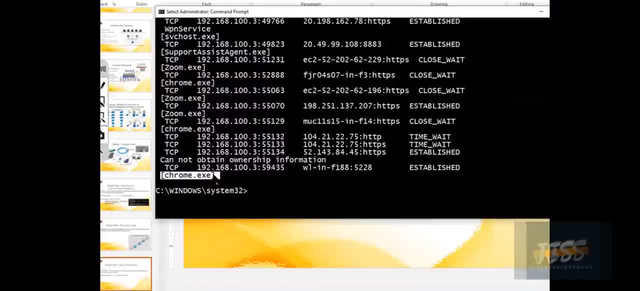 along. this is also going to give me along. this is also going to give me along. this is also going to give me information, information, information on what is going to be my new favorite, on what is going to be my new favorite, on what is going to be my new favorite. that's great. 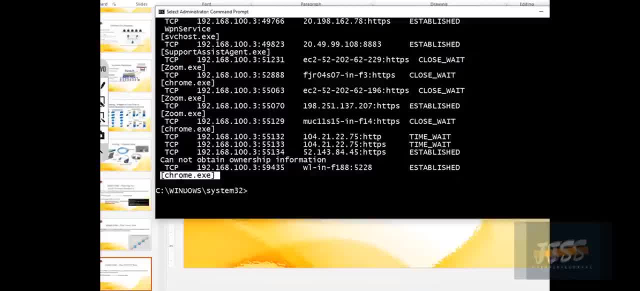 that's great. that's great. and also this is going to also tell me and also this is going to also tell me and also this is going to also tell me: um, um, um, okay, uh, what kind of application is okay? uh, what kind of application is okay? uh, what kind of application is connected? 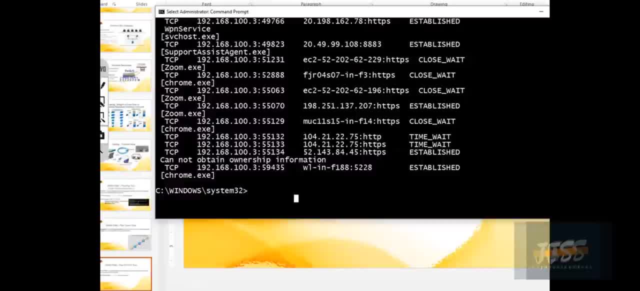 connected. connected. sorry, can you mute yourself? there's a lot, sorry, can you mute yourself? there's a lot, sorry, can you mute yourself? there's a lot of noise coming of noise, coming of noise coming, i think. i think, i think, okay, okay, okay, let's start over to. 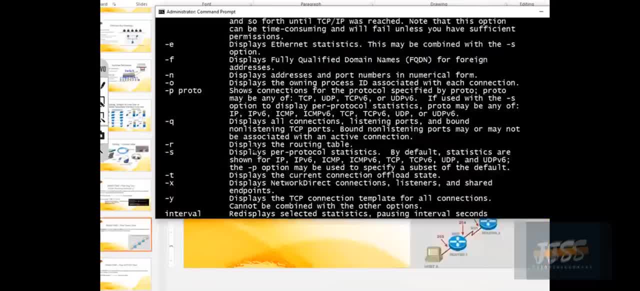 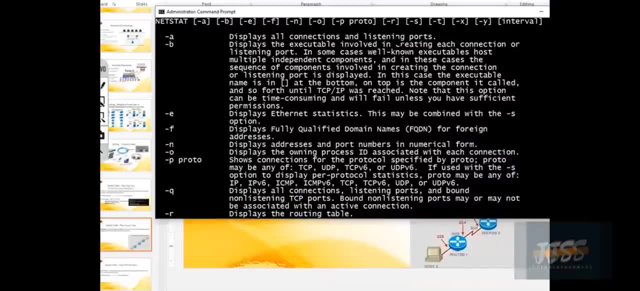 let's start over to. let's start over to another switch. if you can find something, then minus is going to display all, then minus is going to display all, then minus is going to display all connections and listening ports, even that connections and listening ports, even that connections and listening ports, even that is not being used. 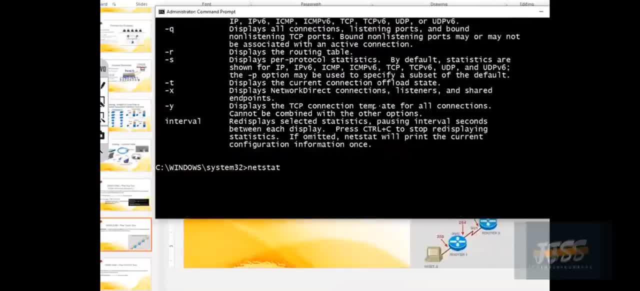 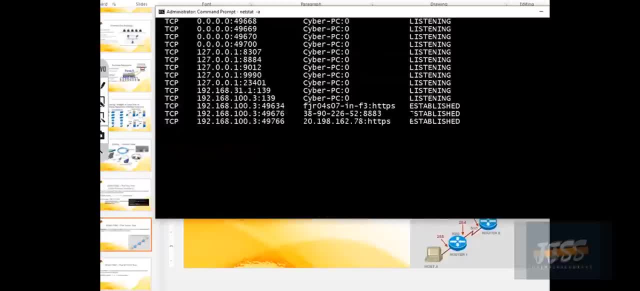 is not being used, is not being used. so, let's do, let's add, so, let's do, let's add, so, let's do, let's add, with the help of minus a, with the help of minus a, with the help of minus a, so, so, so, as you can see, this is established. these: 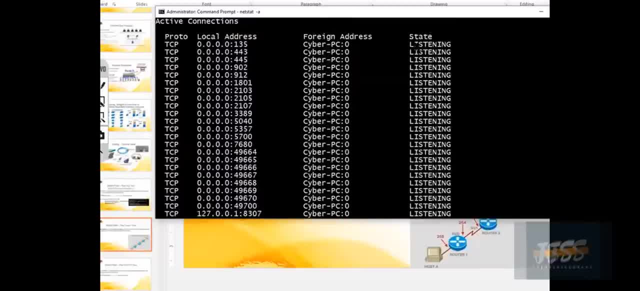 as you can see, this is established. these, as you can see, this is established. these connections have been established. connections have been established. connections have been established. but just take a look. these are the but just take a look. these are the but. just take a look. these are the listening ports means my computer. 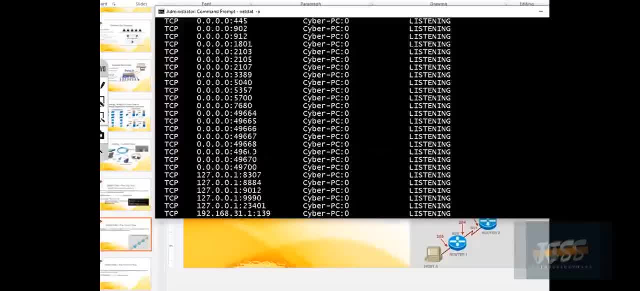 listening ports means my computer listening ports means my computer is ready to listen on these ports, these is ready to listen on these ports, these is ready to listen on these ports, these all. but this is not a good security practice. but this is not a good security practice. 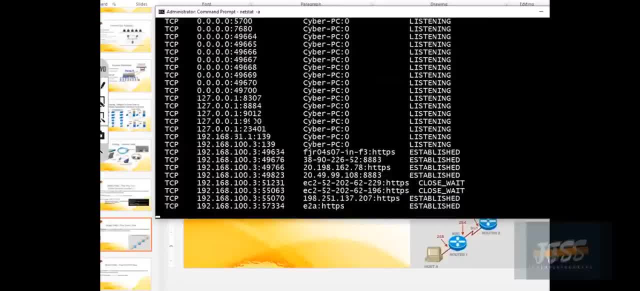 but this is not a good security practice. by the way, we need to close these. by the way, we need to close these. by the way, we need to close these ports if these are open. so, basically, it ports if these are open. so, basically, it ports if these are open. so, basically, it is telling me that these um multiple. 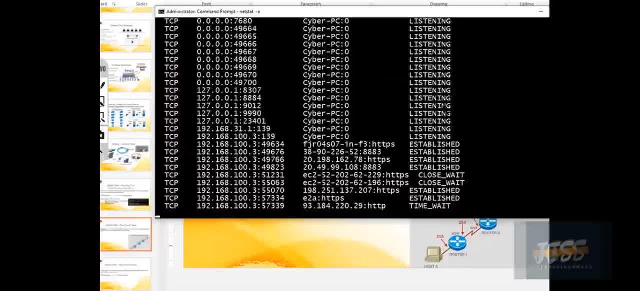 is telling me that these um multiple is telling me that these um multiple ports are open and if you want, i can ports are open and if you want, i can ports are open and if you want, i can connect and i'm listening on these four. connect and i'm listening on these four. 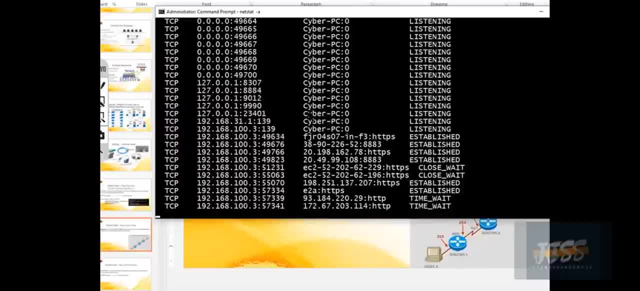 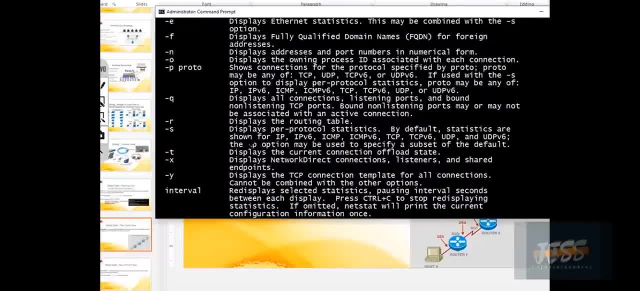 connect and i'm listening on these four actively, actively, actively. okay, then what else do we have something then? what else do we have something then? what else do we have something we can use? uh, we can use, uh, we can use, uh, but just avoid. some ports are. 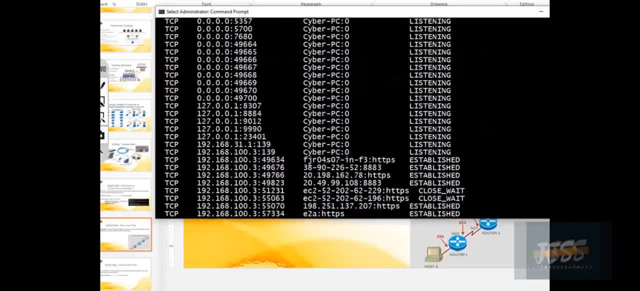 but just avoid. some ports are, but just avoid. some ports are listening, listening, listening, uh, they're open for normal, like uh, they're open for normal, like uh, they're open for normal, like connection connections: connections for your computer to work, for your computer to work, for your computer to work with other computers, and you know your. 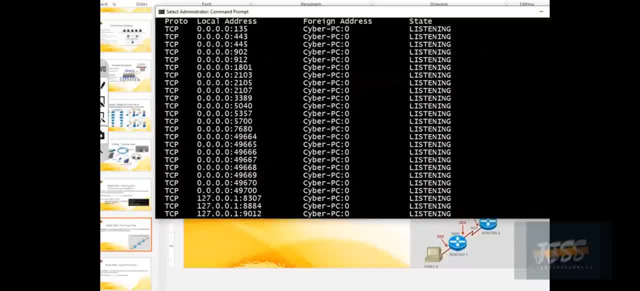 with other computers and you know your with other computers and you know your own local adapter. have when you see own local adapter. have when you see own local adapter. have when you see 127.0.01. that's a loop address, right? so 127.0.01, that's a loop address, right so? 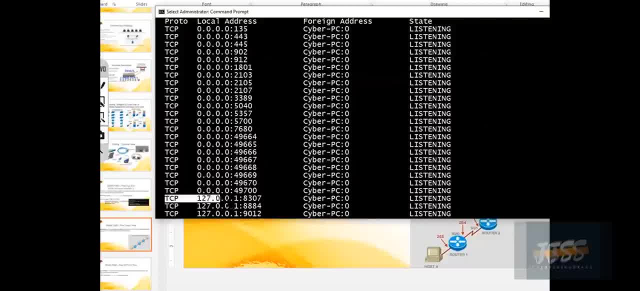 127.0.01. that's a loop address, right. so you, you don't, you, you don't, you, you don't. that's not like your open address and that's not like your open address. and that's not like your open address and maybe using just your own adapter to 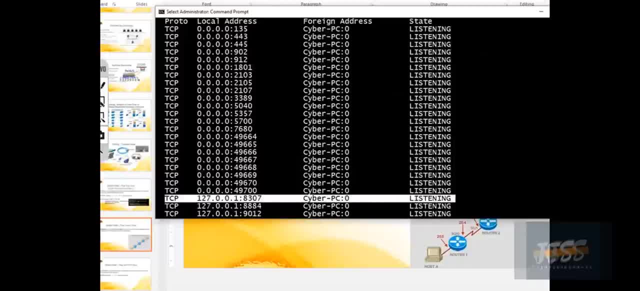 maybe using just your own adapter, to maybe using just your own adapter to listen to things that is happening. listen to things that is happening. listen to things that is happening inside your computer, inside your computer, inside your computer. so, yeah, make sure you guys don't go and start. 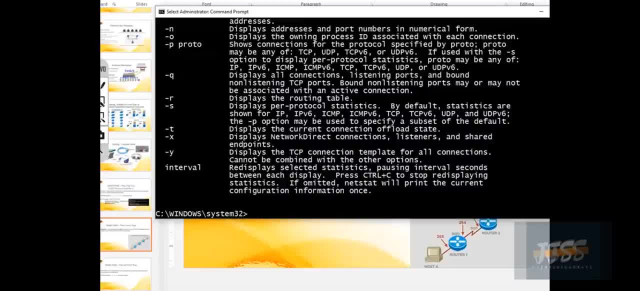 make sure you guys don't go and start, make sure you guys don't go and start blocking everything you know. blocking everything you know, blocking everything you know. something will not work, then yes. something will not work, then yes. something will not work, then yes. this is just for the verification. you 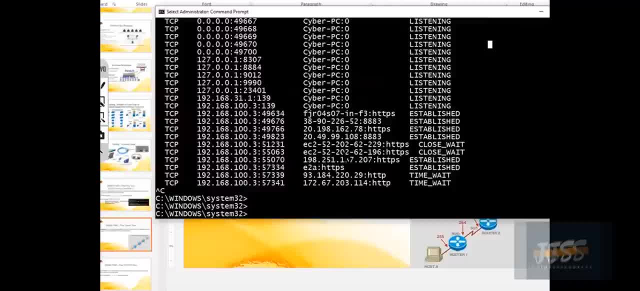 this is just for the verification. you, this is just for the verification. you know we can check what is happening and know we can check what is happening and know we can check what is happening and what is going on in our network. some rogue pc may be connected, so you. 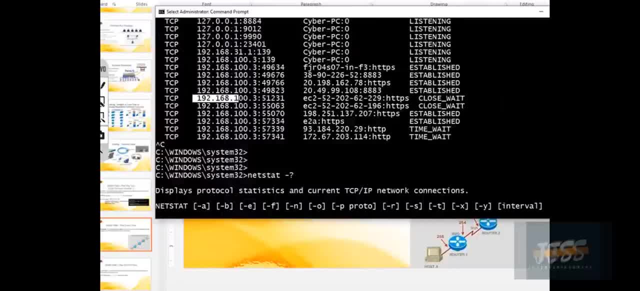 some rogue pc may be connected, so you some rogue pc may be connected so you can identify directly just by taking a, can identify directly just by taking a, can identify directly just by taking a look of the ip- ip and then you can ping. look of the ip- ip and then you can ping. 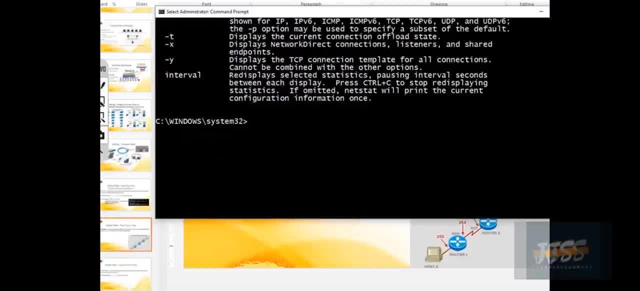 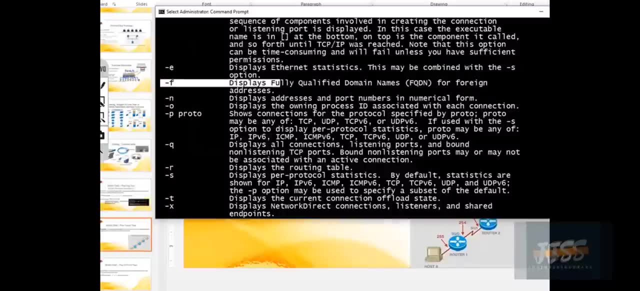 look of the ip, ip and then you can ping and you can resolve that ip to identify and you can resolve that ip to identify and you can resolve that ip to identify what host. basically, that is okay. other than that, okay. other than that, okay, other than that, we have this. um, we don't use this. 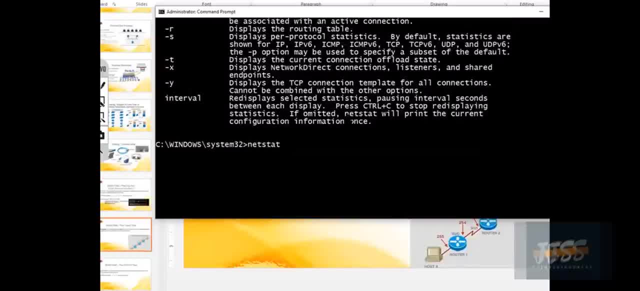 we have this um. we don't use this. we have this um we don't use this software. but let's try this one net software. but let's try this one net software, but let's try this one net: stat minus f. stat minus f. stat minus f. uh, basically, it is going to resolve the 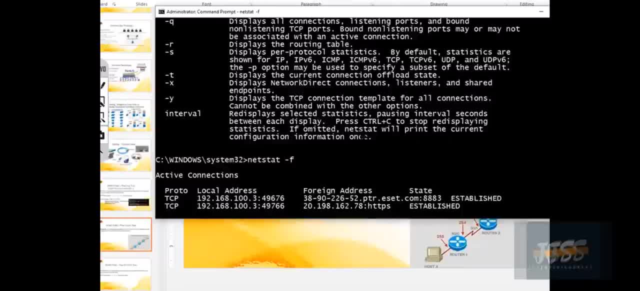 uh, basically, it is going to resolve the. uh, basically, it is going to resolve the fully qualified, fully qualified, fully qualified domain name. just like in case of job domain name, just like in case of job domain name, just like in case of job skill, we have wwwjobsshareorg. 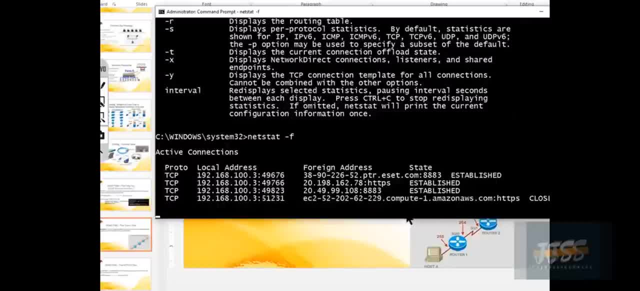 skill. we have wwwjobsshareorg skill, we have wwwjobsshareorg, so this is called fqdn. so this is called fqdn, so this is called fqdn. so, as you can see here, uh, maybe somewhere. so, as you can see here, uh, maybe somewhere. so, as you can see here, uh, maybe somewhere, i'm connected to amazon. 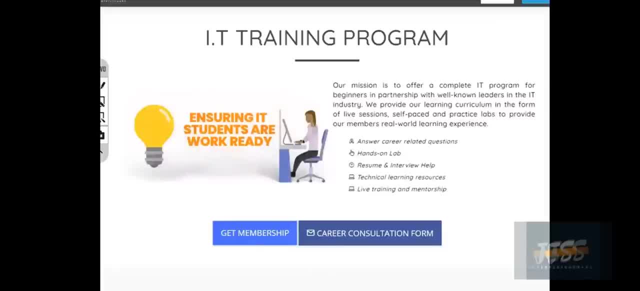 i'm connected to amazon. i'm connected to amazon, or i think this uh, or i think this uh, or i think this uh. job skillshare basically hosted on job skillshare, basically hosted on job skillshare, basically hosted on amazon. so, as you can see, it is giving. 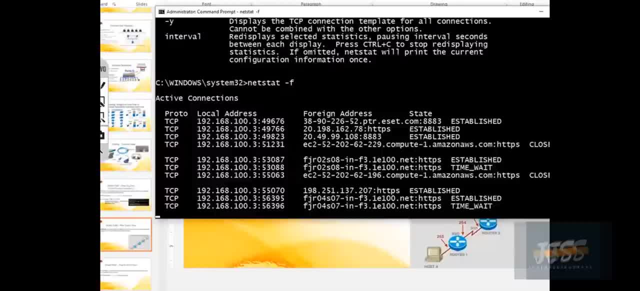 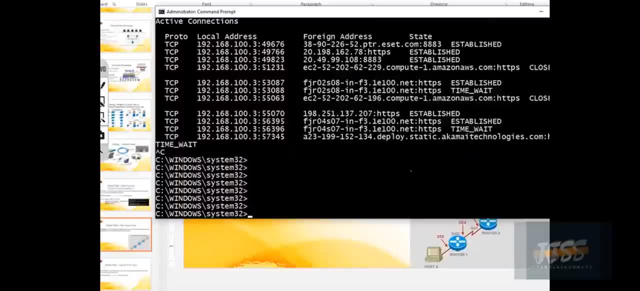 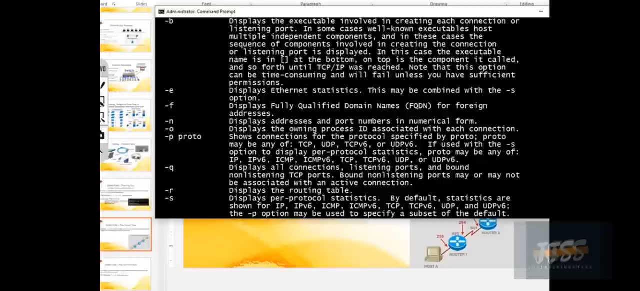 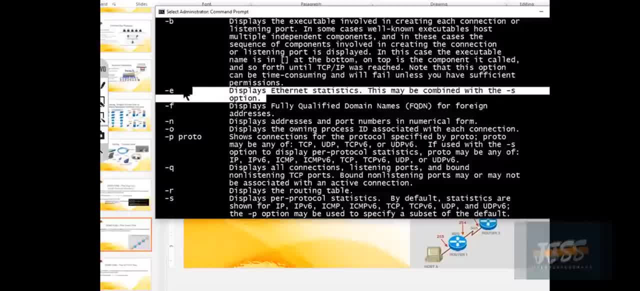 uh, yeah, this minus e displays the. uh yeah, this minus e displays the ethernet statistics. ethernet statistics. ethernet statistics: uh, if we want to see how many data. uh, if we want to see how many data. uh, if we want to see how many data or the bytes have been received or sent. 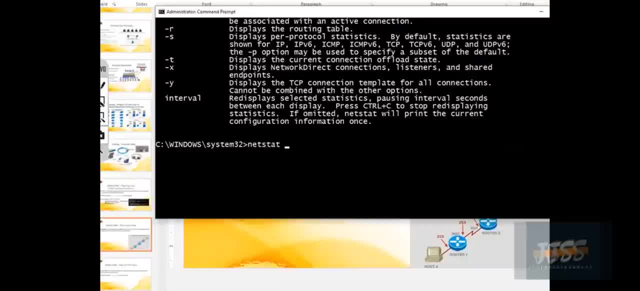 or the bytes have been received or sent. or the bytes have been received or sent. we can just check from here as well. very, we can just check from here as well. very, we can just check from here as well, very quickly, quickly, quickly, just by putting minus e option. 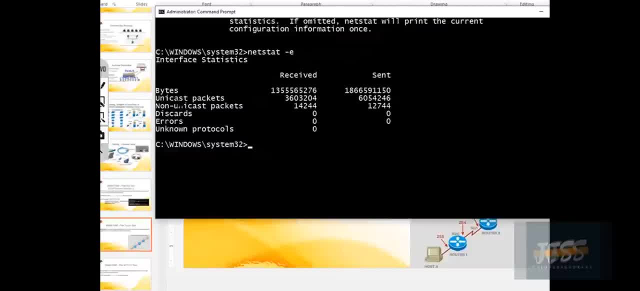 just by putting minus e option, just by putting minus e option, and this is also very good information, and this is also very good information, and this is also very good information, like how many unicast packets are being like, how many unicast packets are being like, how many unicast packets are being sent. 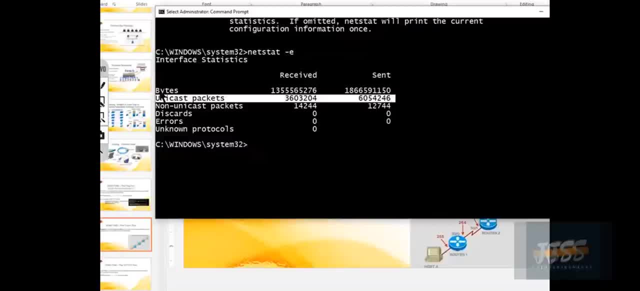 sent, sent. uh from your lan interface card. how many uh from your lan interface card? how many uh from your lan interface card? how many bytes are sent, received and sent? bytes are sent, received and sent. bytes are sent, received and sent. how many non-unicast spectators and how? 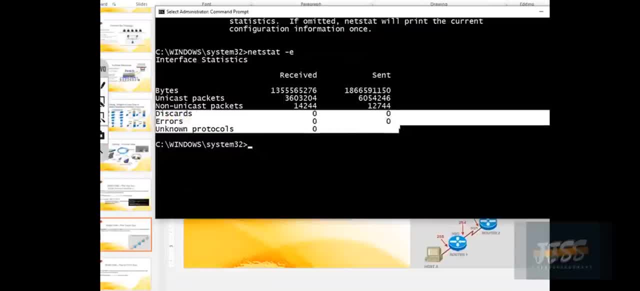 how many non-unicast spectators and how how many non-unicast spectators and how many have been discarded. many have been discarded, many have been discarded. or how many are in the error state, or how many are in the error state, or how many are in the error state. so this is also. 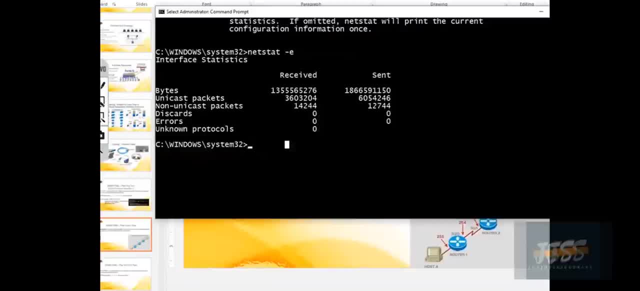 so this is also. so this is also- could be a very helpful piece of, could be a very helpful piece of, could be a very helpful piece of information. so i think this is enough for the next. so i think this is enough for the next. so i think this is enough for the next set. 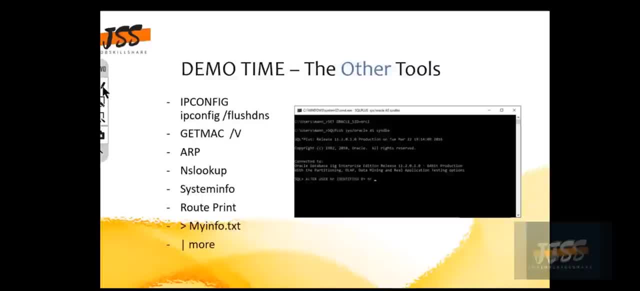 set set. we have some other, we have some other. we have some other tools, like our ip config uh. sometime we have some dns issue with uh. sometime we have some dns issue with uh. sometime we have some dns issue with the help of ip config slash, the help of ip config slash. 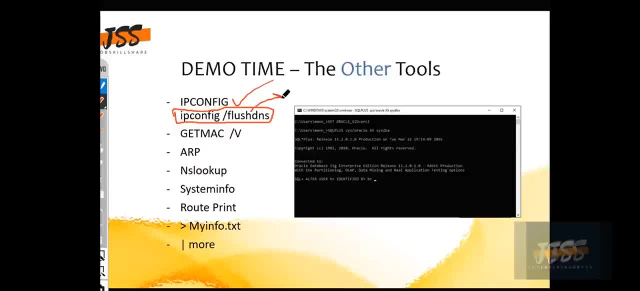 the help of ip config: slash, slash dns, slash dns, slash dns. you are going to flush your dns. you are going to flush your dns. you are going to flush your dns. information, information, information. and you know i'm going to discuss this, and you know i'm going to discuss this. 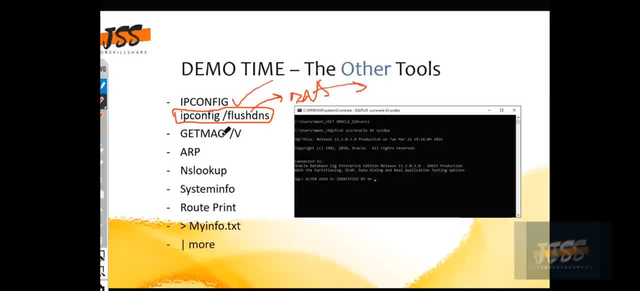 and you know i'm going to discuss this thing a lot in your d2 module thing, a lot in your d2 module thing, a lot in your d2 module. then every computer has some kind of mac. then every computer has some kind of mac. then every computer has some kind of mac addresses or even. 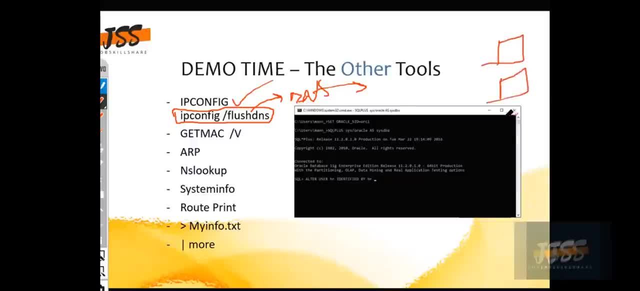 addresses or even addresses or even every network interface card that is attached on your computer, has that is attached on your computer, has that is attached on your computer has different mac address, it has different mac address if one has it has different mac address if one has. it has different mac address if one has different, even your virtual machine. 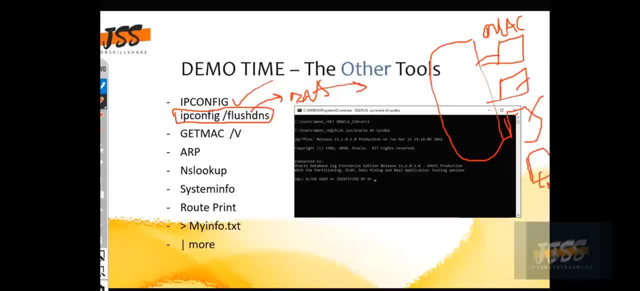 different even your virtual machine, different even your virtual machine. has some kind of uh virtual electrical, has some kind of uh virtual electrical, has some kind of uh virtual electrical interface card which is having different interface card, which is having different interface card, which is having different mac address. 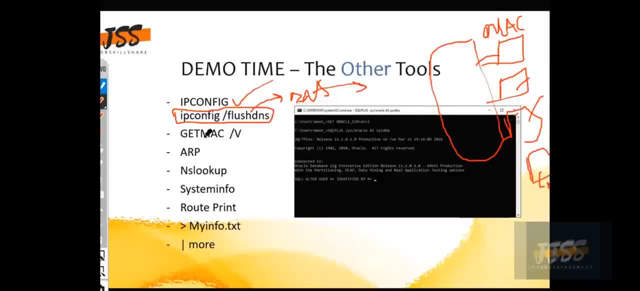 mac address, mac address and these all will be a unique so to, and these all will be a unique so to, and these all will be a unique so to just to identify, to get those you very just to identify, to get those you very just to identify, to get those you very quickly, you can go through this. 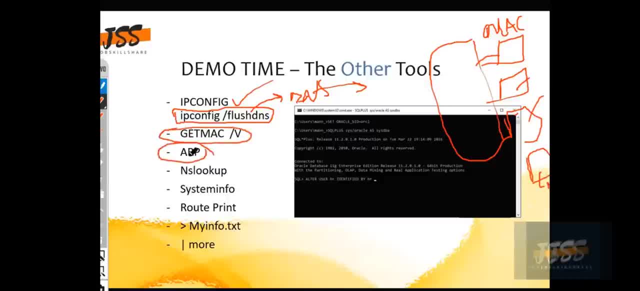 quickly, you can go through this quickly, you can go through this command, command, command, and then we have our, and then we have our and then we have our. uh are basically will show, uh are basically will show, uh are basically will show how many computers, how many computers. 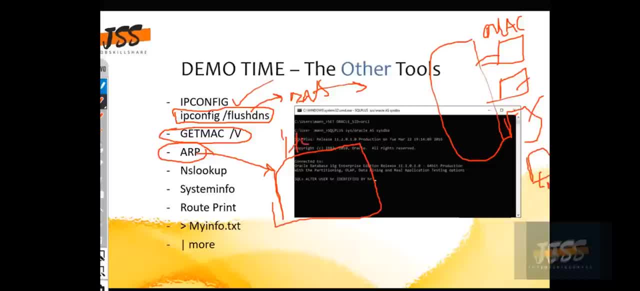 how many computers, um, um, um, your, your host machine, your, your host machine, your, your host machine has learned by the way, has learned by the way, has learned by the way how many mac addresses it has learned how many mac addresses it has learned how many mac addresses it has learned. maybe you're in your land environment, we 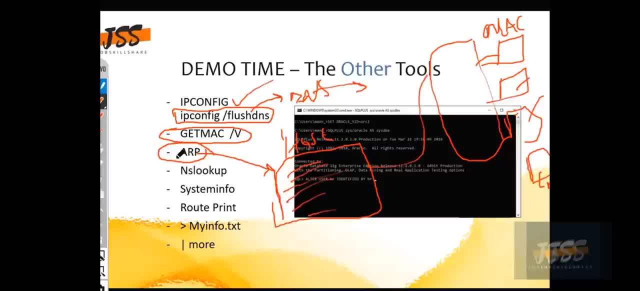 maybe you're in your land environment, we, maybe you're in your land environment, we, you know in the art, you know in the art, you know in the art, arc is a arc is a arc, is a complete chapter as its own. so we're going, complete chapter as its own. so we're going. 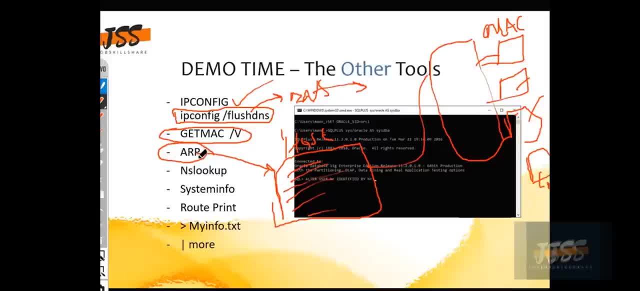 complete chapter as its own. so we're going to discuss art a lot in detail and to discuss art a lot in detail and to discuss art a lot in detail and the cc and a switching section- the cc and a switching section- the cc and a switching section- is totally dependent on art. 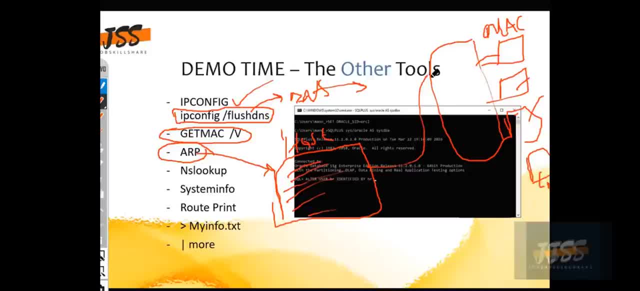 is totally dependent on art, is totally dependent on art. so what i was showing is we have the. so what i was showing is we have the. so what i was showing is: we have the land, environment we have, let's suppose land environment we have. let's suppose 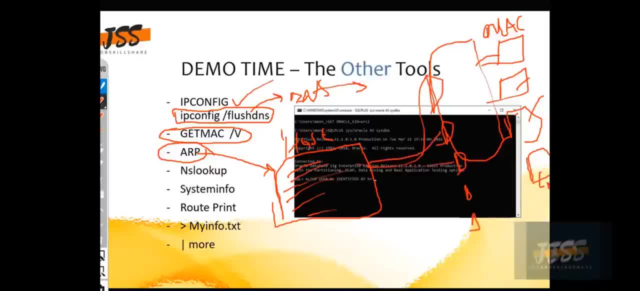 land, environment. we have, let's suppose, 100 computers connected in the same, 100 computers connected in the same, 100 computers connected in the same environment, environment, environment with the same subnet, with the same subnet, with the same subnet. this just both of the computer, this just both of the computer. 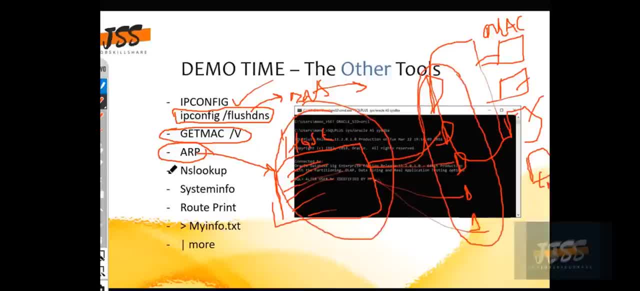 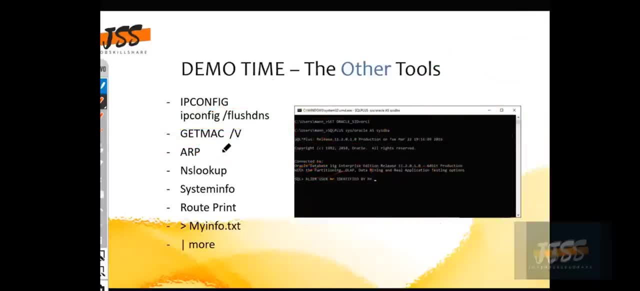 this, just both of the computer will have the information about these, will have the information about these, will have the information about these all post machines. in using the help of all post machines, in using the help of all post machines, in using the help of our protocol, then we have ns lookup. we have one. 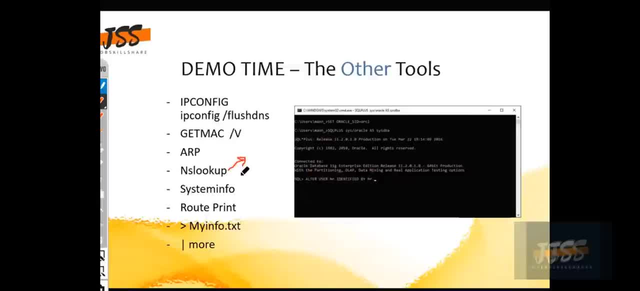 then we have ns lookup. we have one, then we have ns lookup. we have one dedicated section, dedicated section, dedicated section: uh talking about ns lookup. we will go a uh talking about ns lookup. we will go a uh talking about ns lookup. we will go a lot in detail. 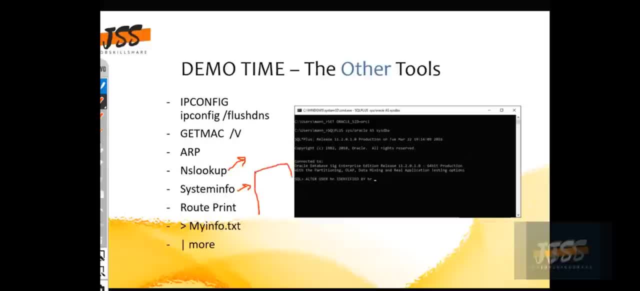 lot in detail, lot in detail. system info is going to give you the system info, is going to give you the system info, is going to give you the information about your computer, and i will, i will demonstrate this one as, and i will, i will demonstrate this one as. 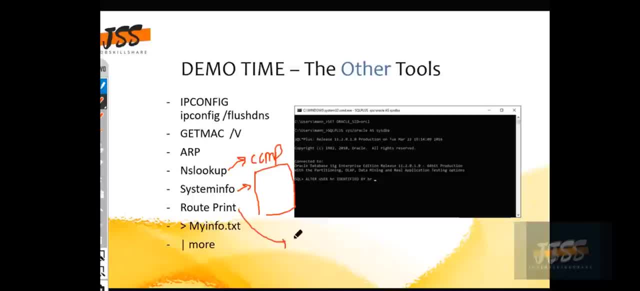 and i will. i will demonstrate this one as well. well, well, route print is just like if you are route. print is just like if you are route. print is just like if you are familiar, familiar, familiar in a routing environment. we have command in a routing environment. we have command. 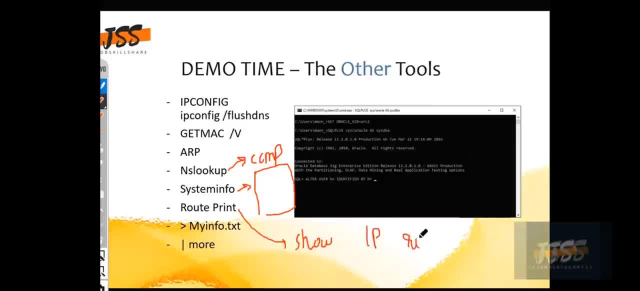 in a routing environment. we have command through ip route which is going to give me information? how, which is going to give me information? how, which is going to give me information? how many best paths do i have many best paths? do i have many best paths? do i have? so in command prompt you can have. 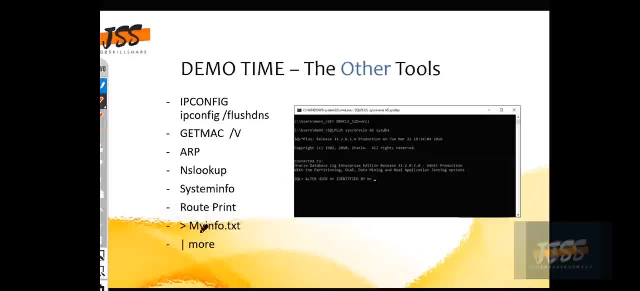 so in command prompt you can have. so in command prompt you can have route print my uh, this greater the sign if we use in, the greater the sign, if we use in the greater the sign if we use in the command prompt, command prompt, command prompt, this command prompt. this is also very handy and useful command. 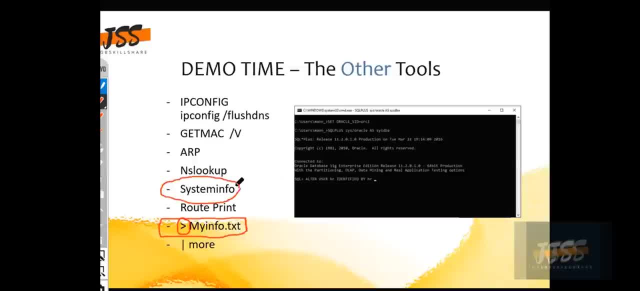 is also very handy and useful command is also very handy and useful command. for example, if this is the system, for example, if this is the system, for example, if this is the system, information, information, information. uh, that is very verbose information. uh, that is very verbose information. uh, that is very verbose information, and we want to save this information in. 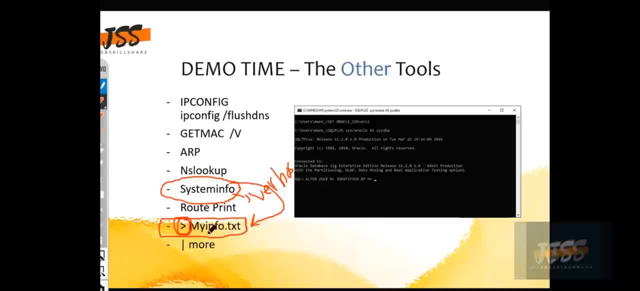 and we want to save this information in. and we want to save this information in my text, my text, my text, so you can use greater than sign and you, so you can use greater than sign and you, so you can use greater than sign and you can save in. 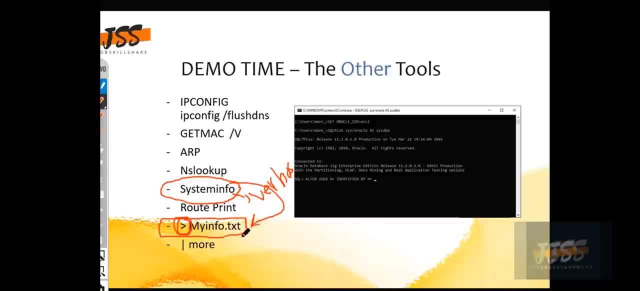 can save in, can save in somewhere in your computer to send to somewhere in your computer, to send to somewhere in your computer to send to some your friend or some your boss or some your friend or some your boss or some your friend or some your boss or colleague, in format of the notepad. 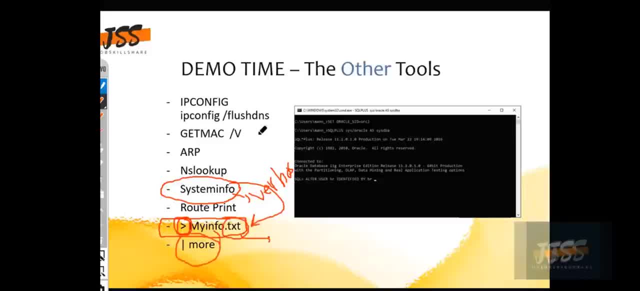 colleague in format of the notepad, colleague in format of the notepad. then we have five more, then we have five more, then we have five more, uh, uh, uh. so i will give you a demo, then you will. so i will give you a demo, then you will. 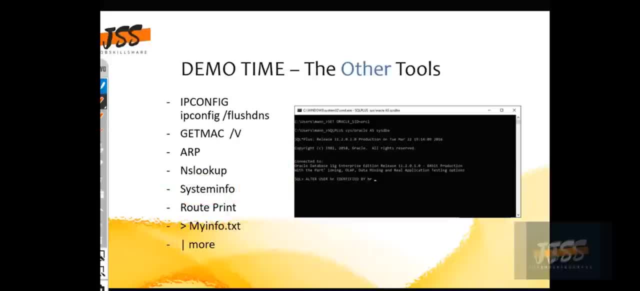 so i will give you a demo. then you will have a better idea about this, have a better idea about this, have a better idea about this. so let's very quickly, so, let's very quickly, so, let's very quickly. i'm going to give a demo about these. 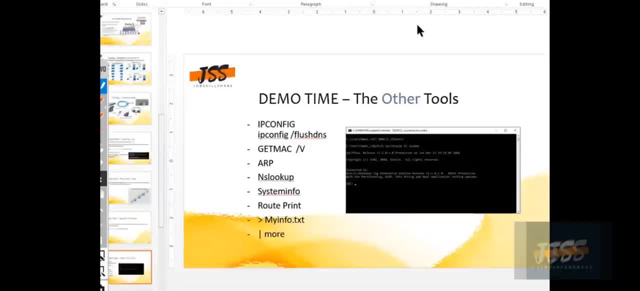 i'm going to give a demo about these. i'm going to give a demo about these: are each command, but i'm not going to go. are each command, but i'm not going to go. are each command, but i'm not going to go a lot in detail. 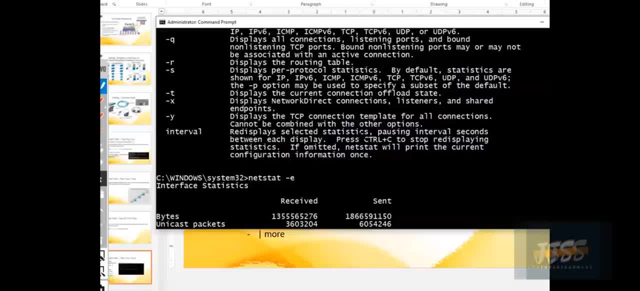 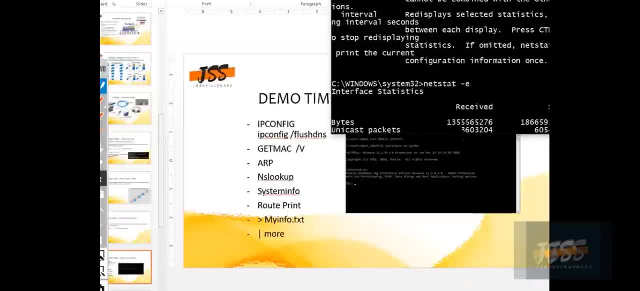 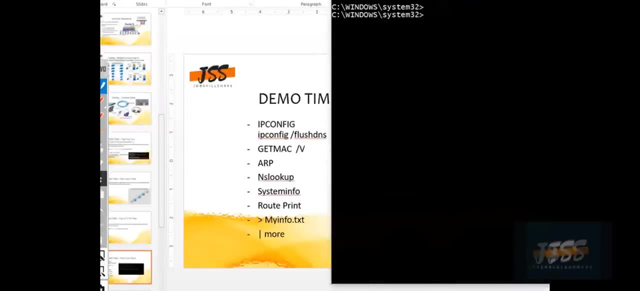 a lot in detail. a lot in detail because we have already covered so many, because we have already covered so many, because we have already covered so many concepts. so you will be confused. i will clear the screen. i will clear the screen. i will clear the screen. so ipconfig, very basic command. 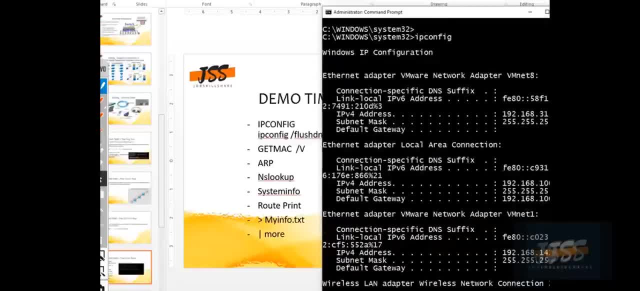 so ipconfig very basic command. so ipconfig very basic command, and and and you will use a lot, you will use a lot, you will use a lot. it will give you the information. it will give you the information. it will give you the information about what network interface cards you 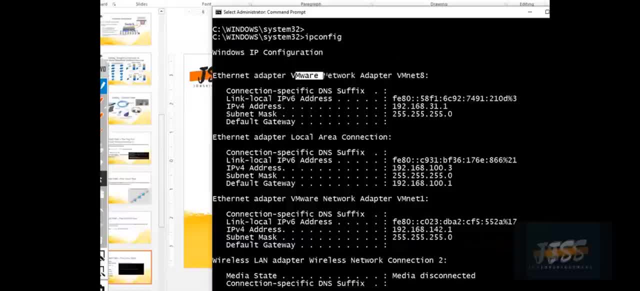 about what network interface cards you, about what network interface cards you have have, have like ethernet adapter. i have on a vmware like ethernet adapter. i have on a vmware like ethernet adapter. i have on a vmware which is virtual environment, which is virtual environment, which is virtual environment. uh, this is also a virtual environment. 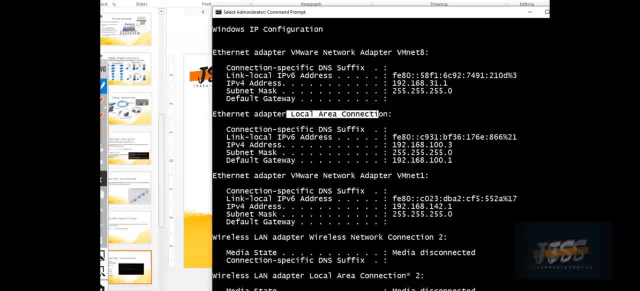 uh, this is also a virtual environment. uh, this is also a virtual environment and this is my physical local and this is my physical local and this is my physical local: network interface cards, network interface cards, network interface cards. then we have a wireless and then these. then we have a wireless and then these. 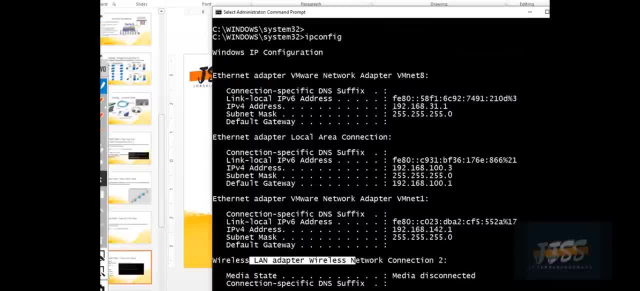 then we have a wireless and then these are uh, are, uh, are, uh, uh. can say the: what are the ip addressing? can say the what are the ip addressing? can say the: what are the ip addressing? i am using on my, i am using on my, i am using on my relevant uh network interface card, like on: 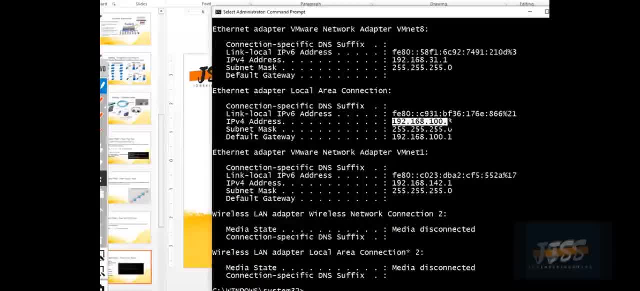 relevant uh network interface card. like on relevant uh network interface card. like on my land, i'm using this kind of ip 192.1. my land. i'm using this kind of ip 192.1. my land. i'm using this kind of ip 192.1 for my wireless land. 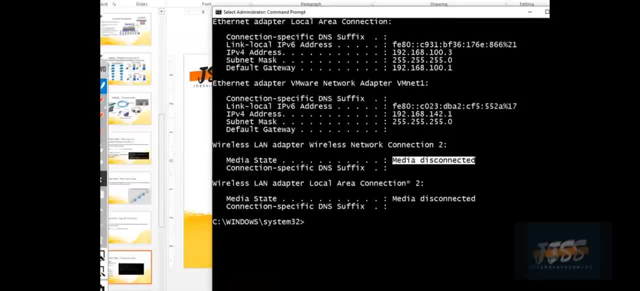 for my wireless land, for my wireless land which is not connected, which is not connected, which is not connected because media has been disconnected, because media has been disconnected, because media has been disconnected. for ethernet adapter vmware i'm using. for ethernet adapter vmware i'm using. 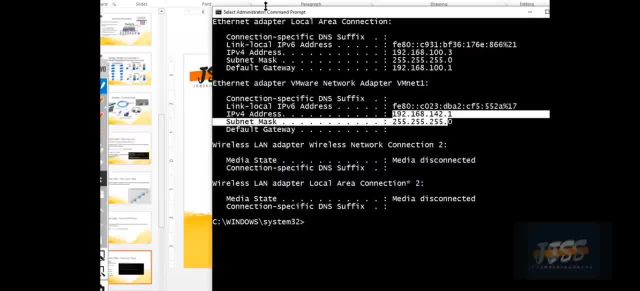 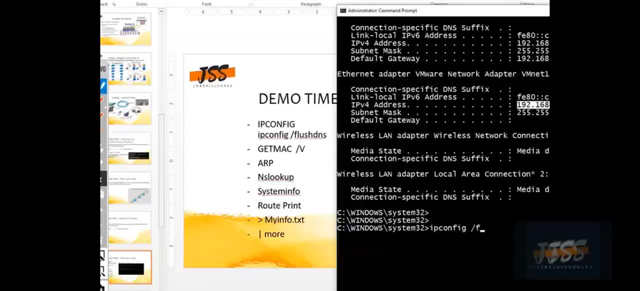 for ethernet adapter vmware. i'm using these kind of addressing, these kind of addressing, these kind of addressing, so very quickly you can go over and so very quickly you can go over and so very quickly you can go over and check the ip connectivity. then you have ip config slash flush dns. 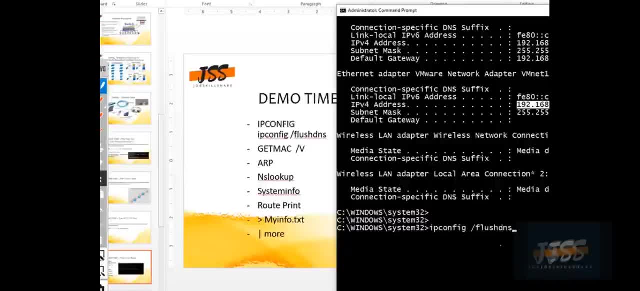 then you have ip config- slash flush dns, then you have ip config- slash flush dns. so, basically, if i will hit enter, it is so. basically, if i will hit enter, it is so, basically, if i will hit enter, it is going to going to going to erase all dns information that. 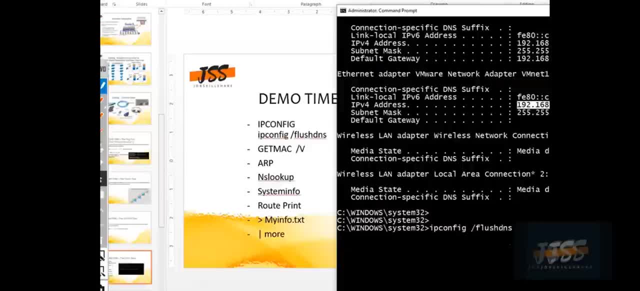 erase all dns information that erase all dns information that resides in my, resides in my, resides in my uh uh uh post machine, which i do not want because i post machine which i do not want, because i post machine which i do not want because i want to keep dns information. 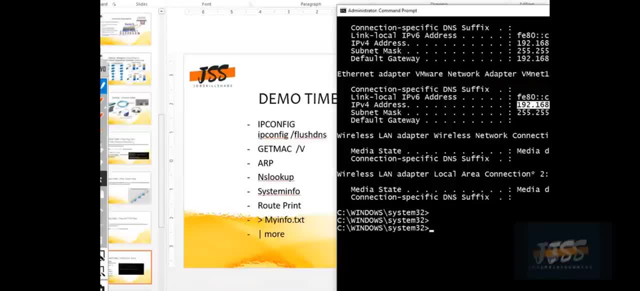 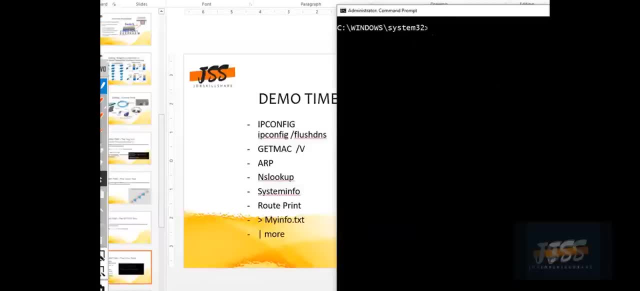 want to keep dns information. want to keep dns information and for the dns: uh, we have a dedicated and for the dns- uh, we have a dedicated and for the dns- uh, we have a dedicated section in week section in week section in week, two modules again, then the we have get math, if i will. 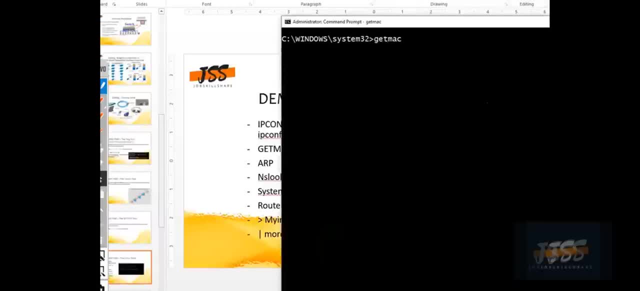 then the we have get math. if i will, then the we have get math. if i will simply press, simply press, simply press. or type get mac and hit enter, or type get mac and hit enter, or type get mac and hit enter, it is very quickly going to give me. 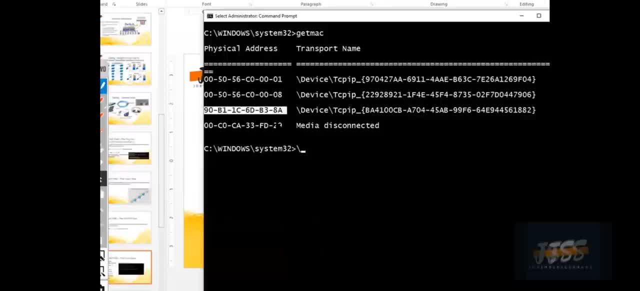 it is very quickly going to give me. it is very quickly going to give me information about the mac addresses, information about the mac addresses, information about the mac addresses, but the problem is it is not giving me. but the problem is it is not giving me. but the problem is it is not giving me what this? 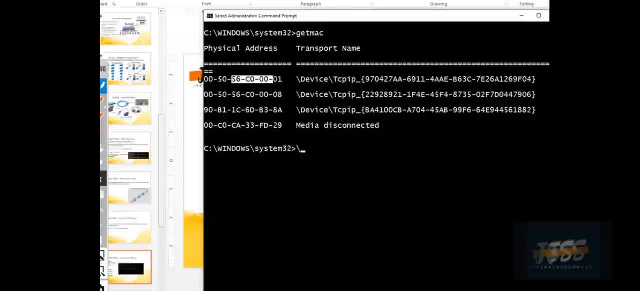 what this, what this physical address is connected with, which physical address is connected with, which physical address is connected with which interface, interface interface, or which, or which or which nick card, nick card, nick card, network interface card, network interface card, network interface card. to get that, to get that. 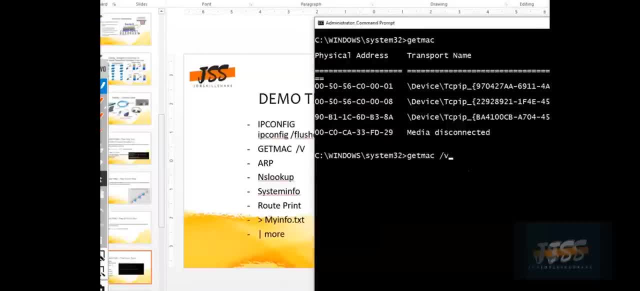 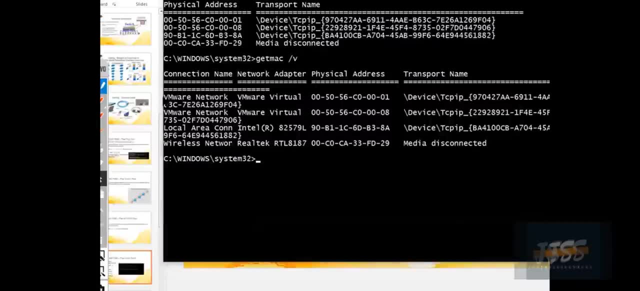 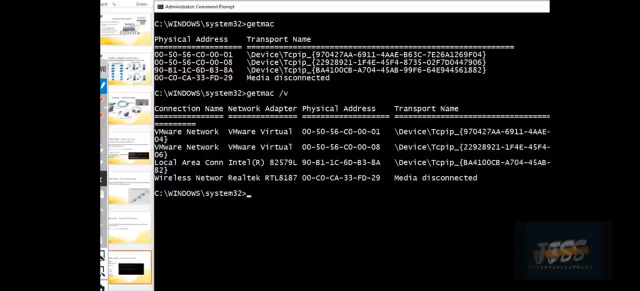 to get that. you type get mac, you type get mac. you type get mac and type slash b, hit enter. if i will just expand this one here you can see, here you can see. here you can see my vm virtual is using this physical. my vm virtual is using this physical. 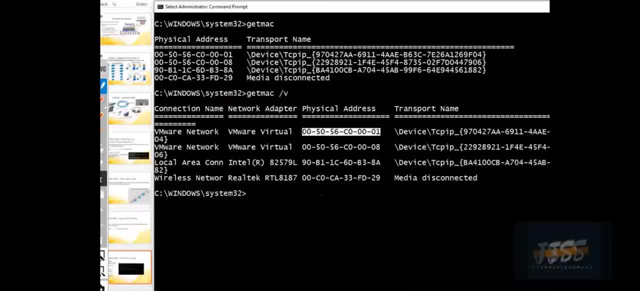 my vm virtual is using this physical interface card: interface card. interface card. uh physical address or the mac address. uh physical address or the mac address: uh physical address or the mac address. my local area connection or lan card is my local area connection or lan card. is my local area connection or lan card is using this. 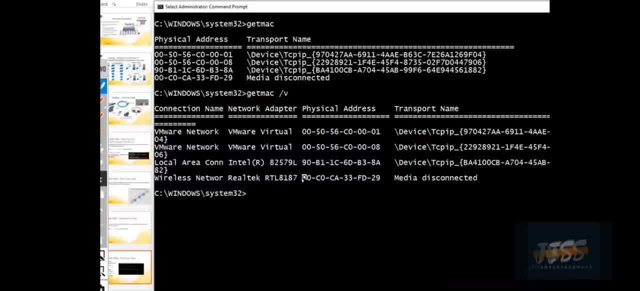 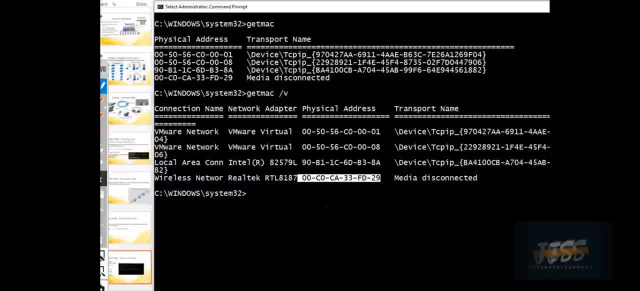 so see how quickly. so see how quickly. uh, you just get the knowledge about the, get the knowledge about the, get the knowledge about the mac addresses of your mac addresses of your mac addresses of your network interface cards, network interface cards, network interface cards. so this is also some kind of very handy. 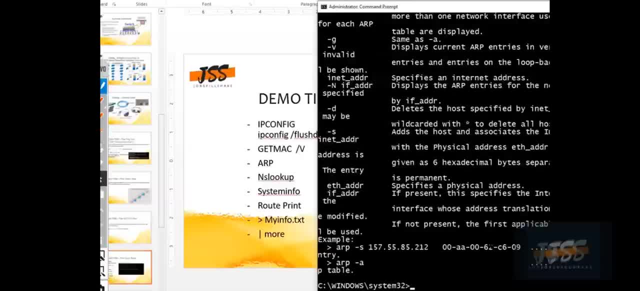 so this is also some kind of very handy. so this is also some kind of very handy command, command, command. then we have our, then we have our, then we have our. it comes with uh, it comes with uh, it comes with uh. a lot of uh, a lot of uh. 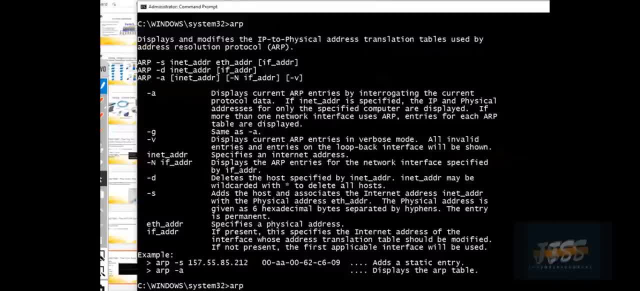 a lot of uh options. let's uh do with r options. let's uh do with r options. let's uh do with r minus a, minus a, minus a, and it is going to give me the, and it is going to give me the and it is going to give me the information. 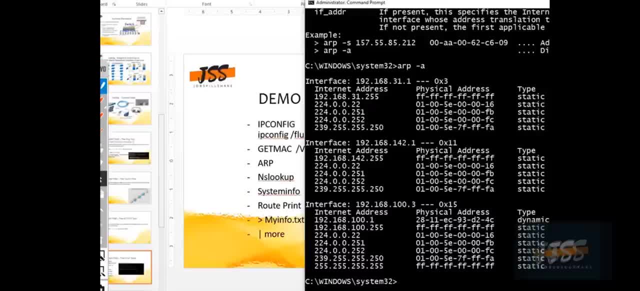 information, information. uh, what other host machine my? uh, what other host machine my? uh, what other host machine my computer has learned so far? computer has learned so far. computer has learned so far. so in this case, for example, if i give, so in this case, for example, if i give. 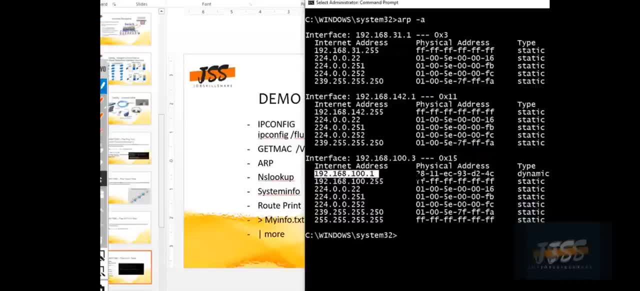 so in this case, for example, if i give you information, this is my gateway, you information, this is my gateway, you information, this is my gateway and this is a physical and this is a physical and this is a physical address that is correlated to my address, that is correlated to my. 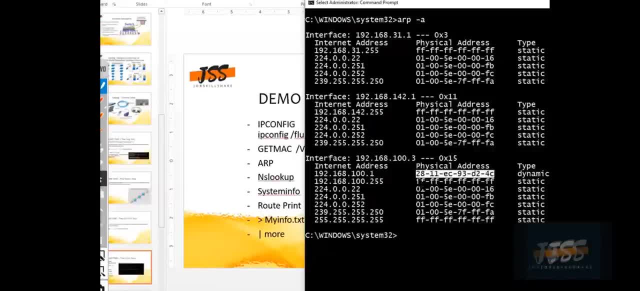 address that is correlated to my access point- access point, access point. so, instead of resolving this mac address, so instead of resolving this mac address, so, instead of resolving this mac address, it will send a r and it will receive our. it will send a r and it will receive our. 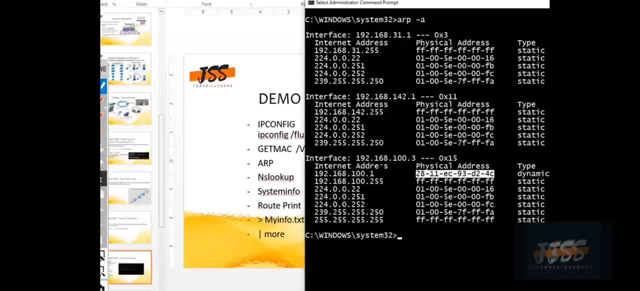 it will send a r and it will receive our reply, and then i will get this magnet reply, and then i will get this magnet reply, and then i will get this magnet. it already keeps this information saved. it already keeps this information saved. it already keeps this information saved in its arc table. 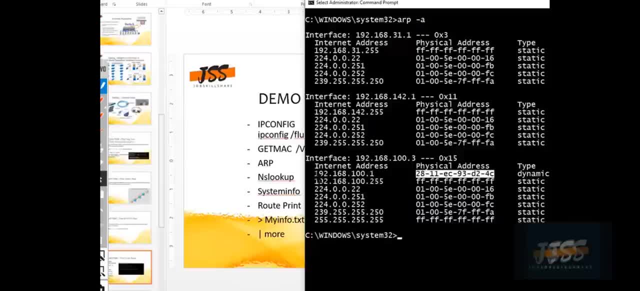 in its arc table. in its arc table. why? why? why, when i want to reach my access point, when i want to reach my access point, when i want to reach my access point, it will go directly to mac address and it will go directly to mac address and. 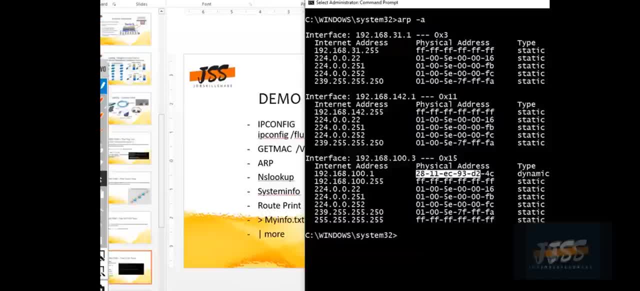 it will go directly to mac address and just go directly to the access point. just go directly to the access point. just go directly to the access point instead going through some another, instead going through some another, instead going through some another address. as i said, ns lookup. as i said, ns lookup. 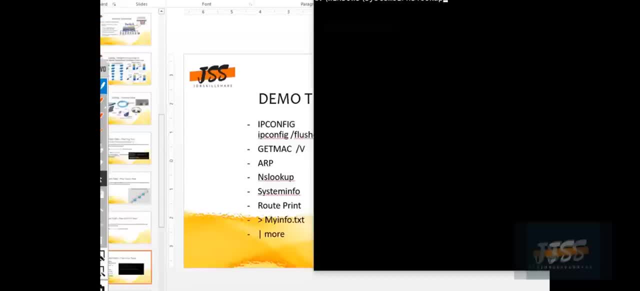 as i said, ns lookup, we have, we have. we have one dedicated section for ns lookup, one dedicated section for ns lookup, one dedicated section for ns lookup. but just but, just but just give you information, what it does if you give you information, what it does if you. 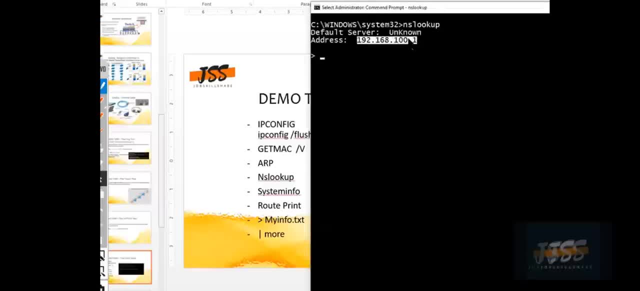 give you information what it does. if you hit ns lookup, it is going to give me hit ns lookup. it is going to give me hit ns lookup. it is going to give me information. what my gateway address is. information what my gateway address is. information what my gateway address is connected. 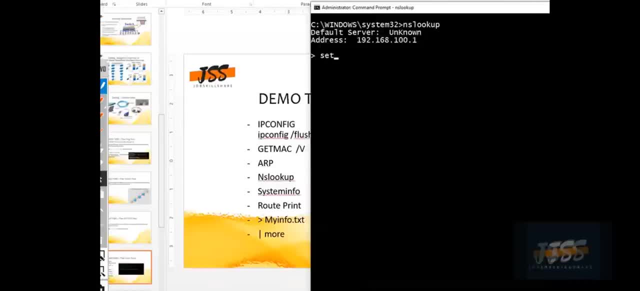 connected, connected. and if i want to go a lot in detail, and if i want to go a lot in detail, and if i want to go a lot in detail, i can go like set type uh, i want to know. i can go like set type uh, i want to know. 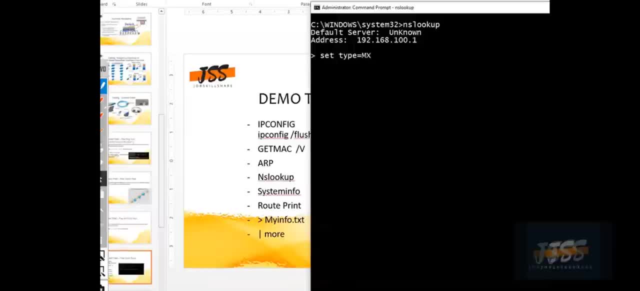 i can go like set type. uh, i want to know information about the information, about the information about the mail exchange server, mail exchange server, mail exchange server, about some. uh, let's go about some. uh, let's go about some. uh, let's go uh like wwwjobskill. 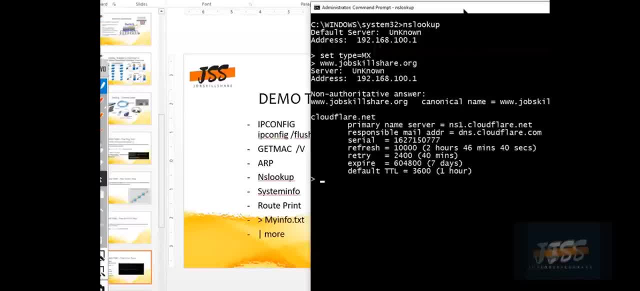 uh like wwwjobskill. uh like wwwjobskill. shareorg. if i hand, if i hit, enter it shareorg. if i hand, if i hit, enter it shareorg. if i hand, if i hit enter, it will show me my mail server basically. will show me my mail server basically. 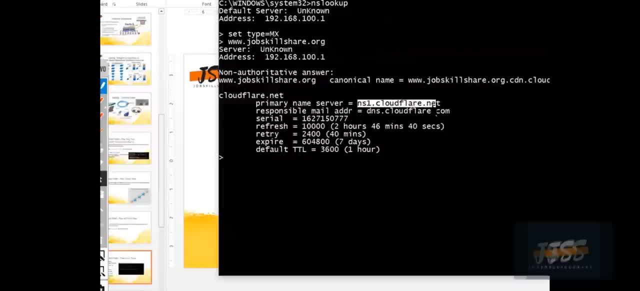 will show me my mail server. basically, uh, uh, uh, have have have this, uh, this, uh, this, uh. name of the server is ns1.cloudnet. name of the server is ns1.cloudnet. name of the server is ns1.cloudnet. so this is going to give me the information. 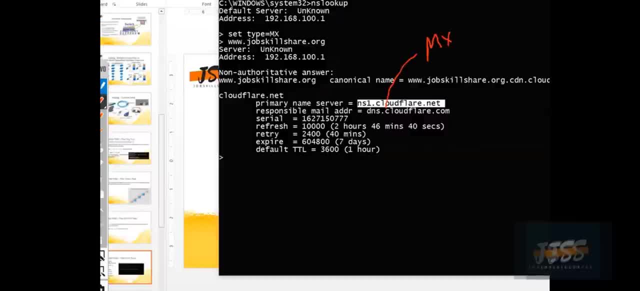 so this is going to give me the information. so this is going to give me the information about my, about my, about my mail exchange server. so not to worry, mail exchange server. so not to worry. mail exchange server, so not to worry about if you are not getting this at. 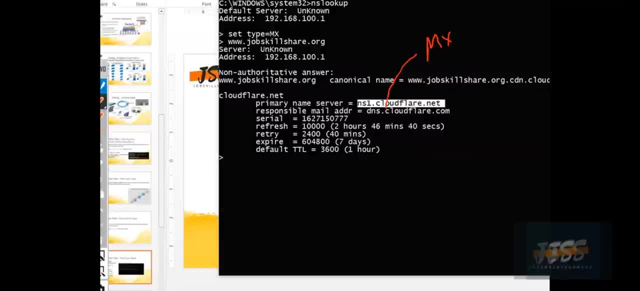 about if you are not getting this at about, if you are not getting this at this time, because this time, because this time, because my intention is just to my intention, is just to my intention, is just to make sure you have this command in your. make sure you have this command in your. 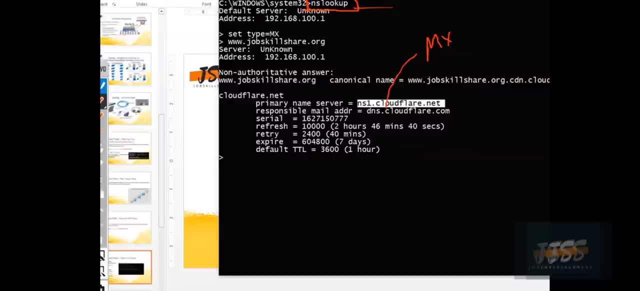 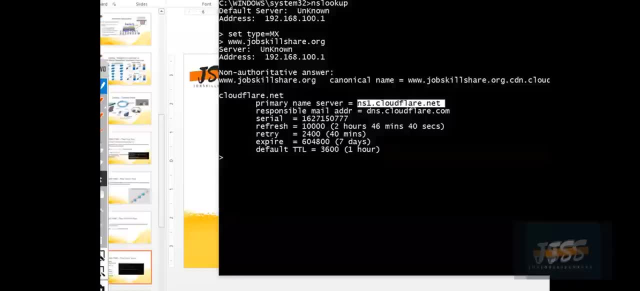 make sure you have this command in your tool bank, tool bank, tool bank- and this is we gonna discuss a lot in, and this is we gonna discuss a lot in, and this is we gonna discuss a lot in detail in subsequent videos. if you want to exit, just type exit and. 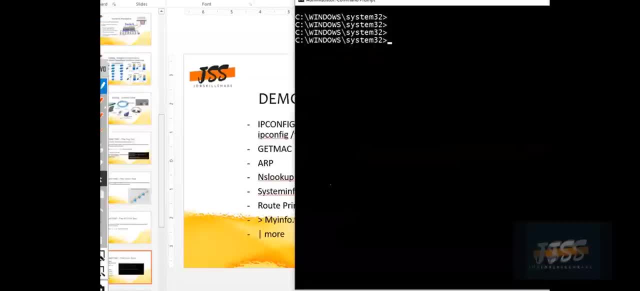 if you want to exit, just type exit. and if you want to exit, just type exit and you will be in the. you will be in the. you will be in the command prompt again. command prompt again. command prompt again. then the other tool: we have system info, which is: 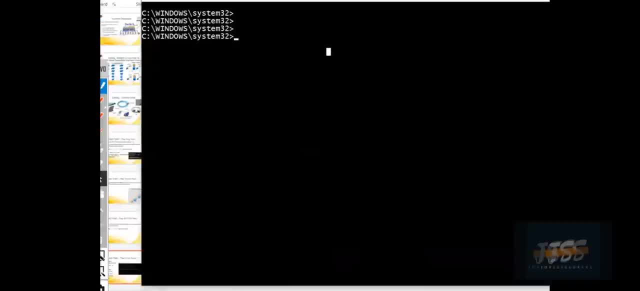 other tool. we have system info, which is other tool. we have system info which is going to give me, going to give me, going to give me the purpose information about my computer, the purpose information about my computer, the purpose information about my computer, just type, system and info. 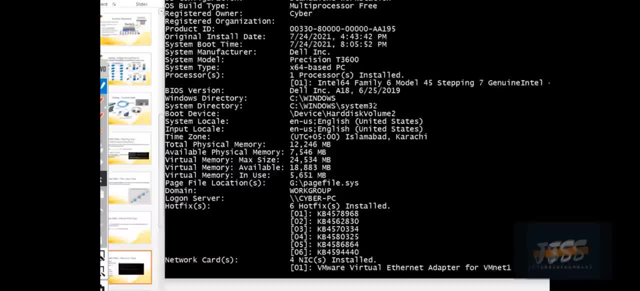 just type system and info. just type system and info as you can see how quickly it is going. as you can see how quickly it is going, as you can see how quickly it is going to give me, to give me, to give me a nitty-gritty detail about what my 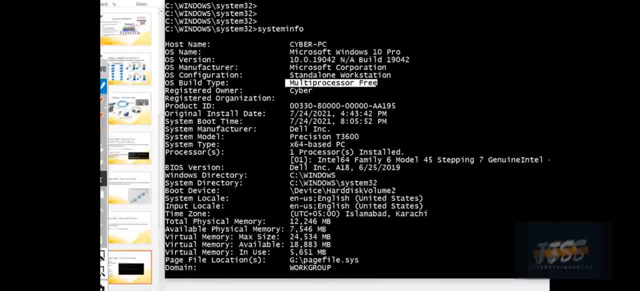 a nitty-gritty detail about what my a nitty-gritty detail about what my computer is. computer is computer is. what is the processor type? multi-processor? what is the processor type multi-processor? what is the processor type multi-processor? i'm using microsoft corporation. 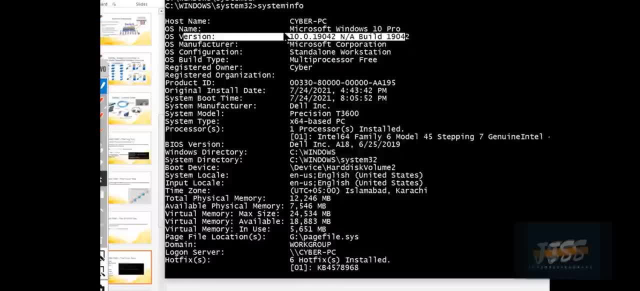 i'm using microsoft corporation. i'm using microsoft corporation. the operating system version and the. the operating system version and the. the operating system version and the build, build, build. what kind of operating system name is? what kind of operating system name is? what kind of operating system name is windows 10 pro? 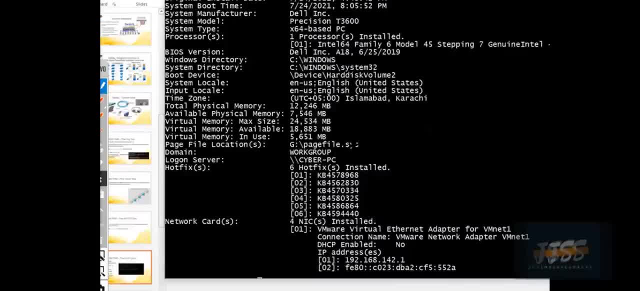 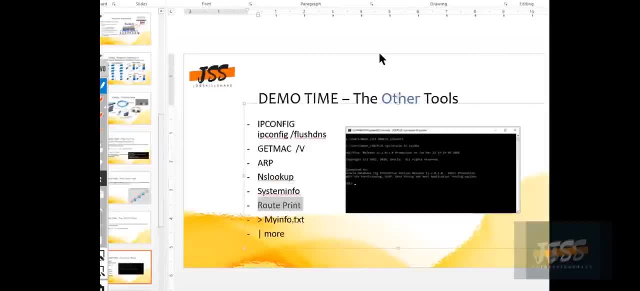 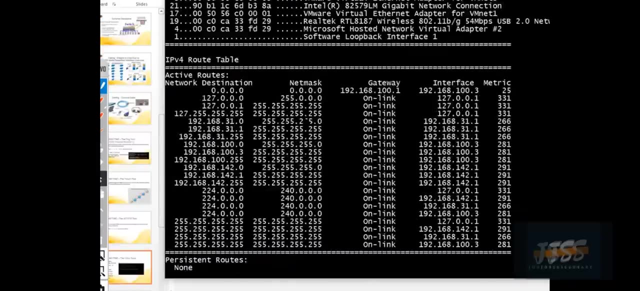 windows 10 pro. windows 10 pro and there is a ton and ton of information. then we have route print. if you do route, then we have route print. if you do route, then we have route print, if you do route print. so this is just like um ip routing table. 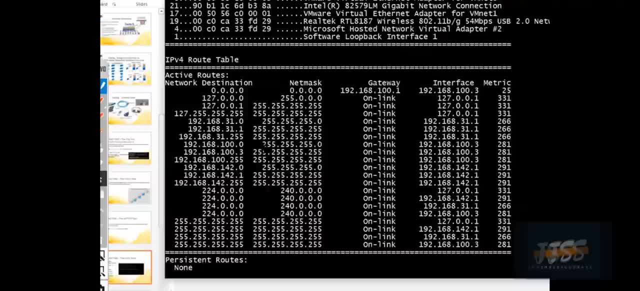 so this is just like um ip routing table. so this is just like um ip routing table. it is having information about the. it is having information about the. it is having information about the multiple gateway, for example. multiple gateway, for example, multiple gateway, for example, and which is the best one i am going to 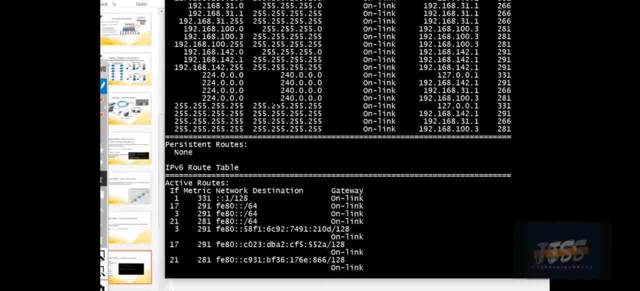 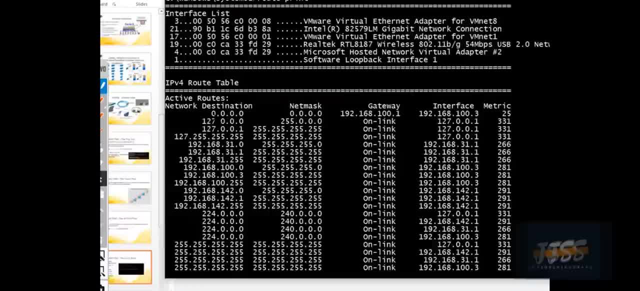 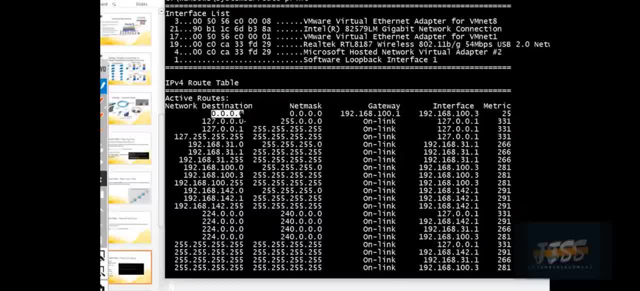 network destination is 0.0.0.0. it is nothing but your default gateway. it is nothing but your default gateway. it is nothing but your default gateway. just you know, i don't want to discuss a. just you know, i don't want to discuss a. 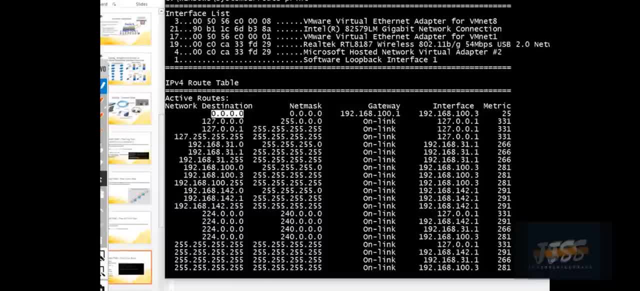 just, you know, i don't want to discuss a lot this one. what is the point? uh, lot this one? what is the point uh, lot this one? what is the point? uh, i default, i default, i default. route, because you will be confused. route, because you will be confused. 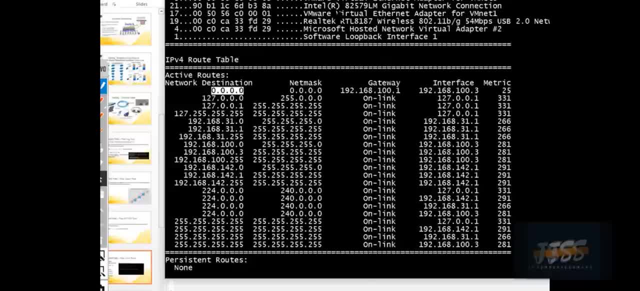 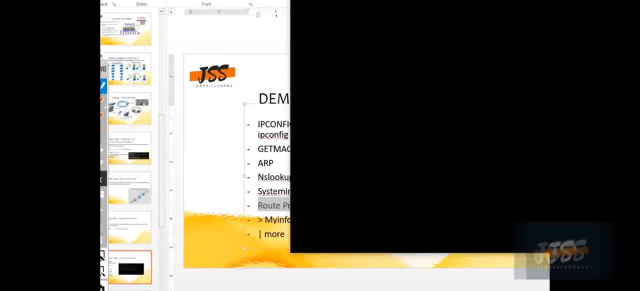 route, because you will be confused. so keep it, so keep it, so keep it. for the routing uh, for the routing uh, for the routing uh topics. then i, as i said, for example, then i, as i said, for example, then i, as i said, for example, we have 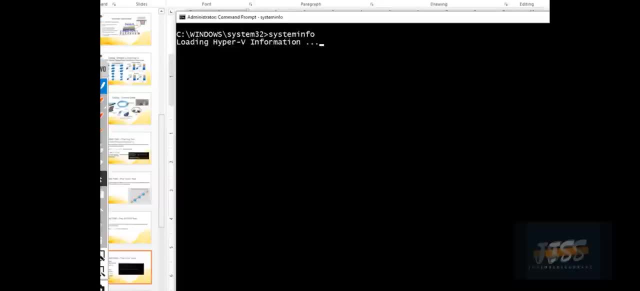 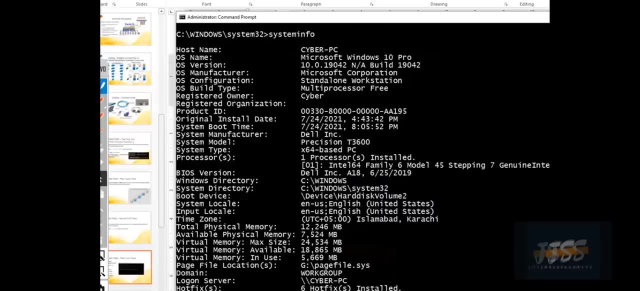 we have, we have system info. this all information i want to send. using this all information i want to send, using this all information i want to send using email address, email address. email address. of course i want to save this information. of course i want to save this information. 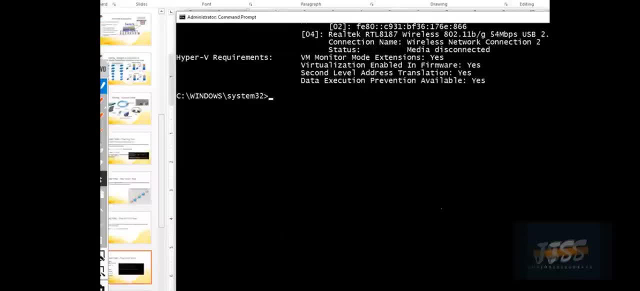 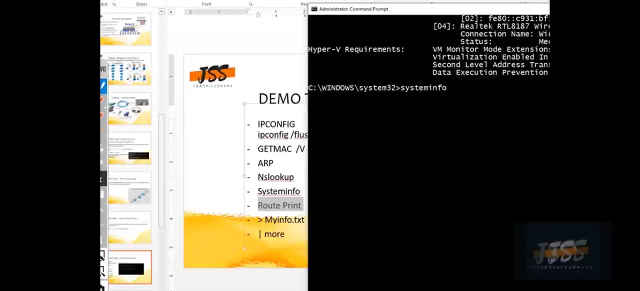 of course i want to save this information somewhere, somewhere, somewhere, so so so for that we can use, for that we can use, for that we can use the greater than the greater than the greater than command, command, command, and you can type: we will use the command system info then. 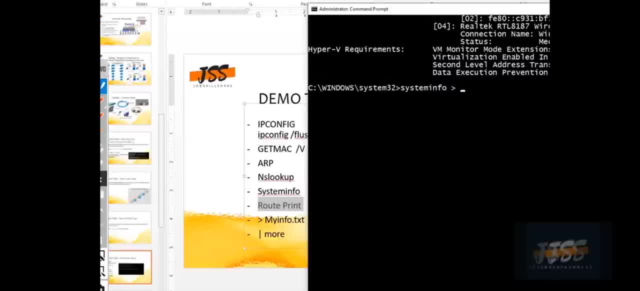 we will use the command system info. then we will use the command system info. then, greater than sign. greater than sign. greater than sign. and where we want to save this file with, and where we want to save this file with, and where we want to save this file with the. what name? let's put the name of: 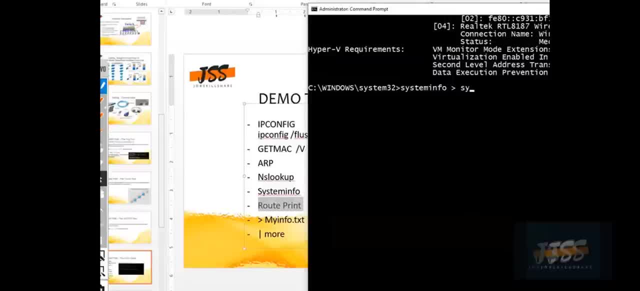 the. what name? let's put the name of the. what name? let's put the name of file is, file is, file is uh, uh, uh, system, system, system, info dot text, info dot text, info dot text. and i will hit enter. and if i take a look of direct, 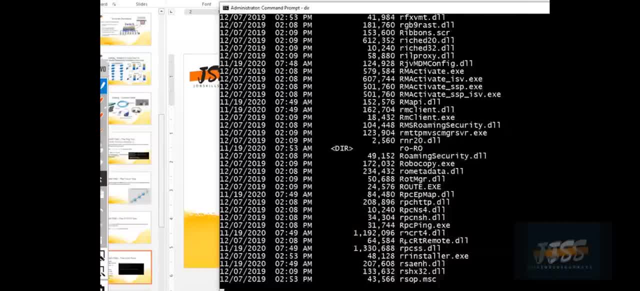 and if i take a look of direct, and if i take a look of direct, uh, uh, uh, there's so much going on, there's so much going on, there's so much going on. but, by the way, if you will go into c, but, by the way, if you will go into c, 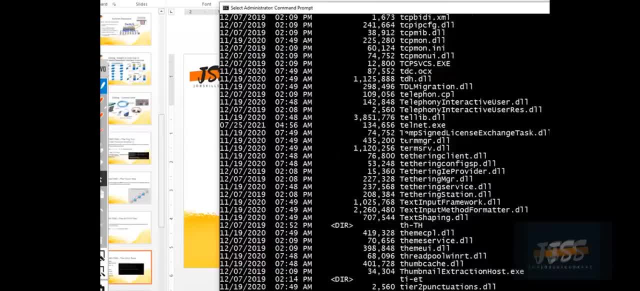 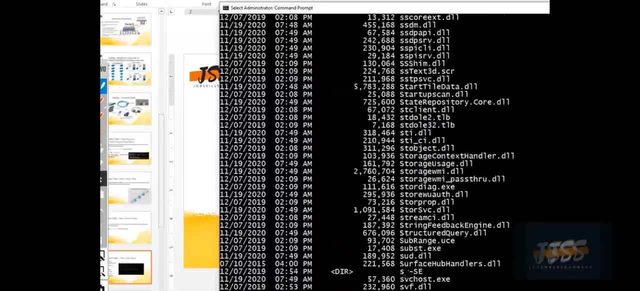 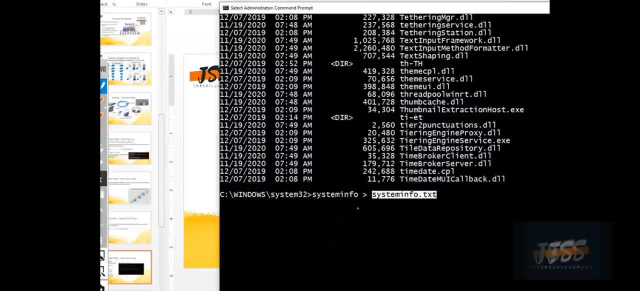 but, by the way, if you will go into c- windows system 32, windows system 32, windows system 32, you will find- sorry, you will find this file system, info dot. you will find this file system, info dot. you will find this file system info dot t actually, which will be having the. 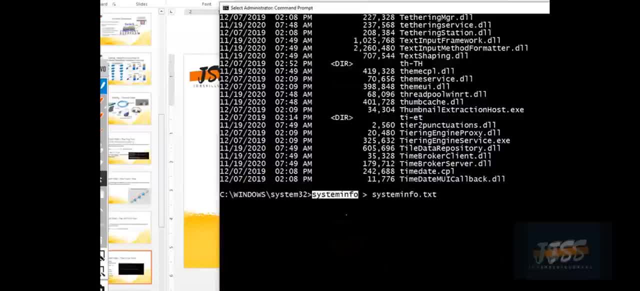 t actually, which will be having the t actually, which will be having the information about your information, about your information, about your system information. so this is how, system information. so this is how, system information. so this is how, how, how, how very quickly you can say whatever the. 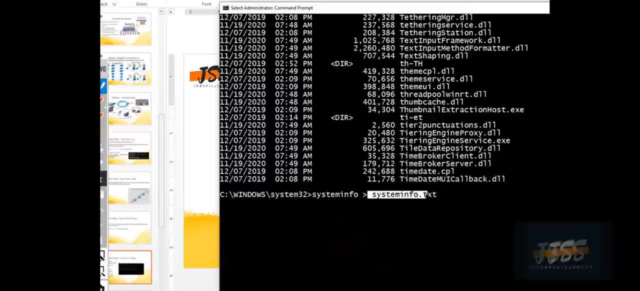 very quickly you can say whatever the very quickly you can say whatever the command you are going to give and it command you are going to give and it command you are going to give, and it will be saved in. this will be saved in. this will be saved in this: uh text notepad. 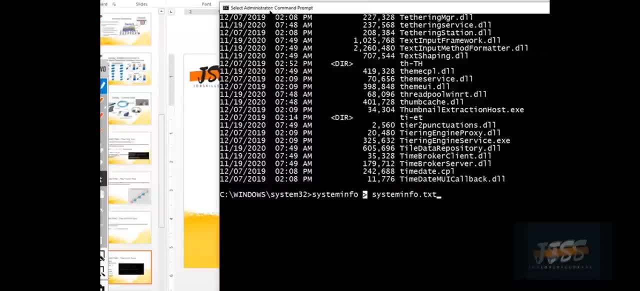 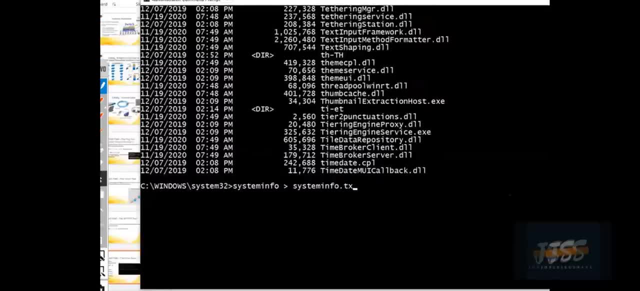 uh text notepad, uh text notepad. with the help of greater than sign. so with the help of greater than sign. so with the help of greater than sign. so this is the syntax. then the last command is slash more, then the last command is slash more, then the last command is slash more. and this is also very helpful and handy. 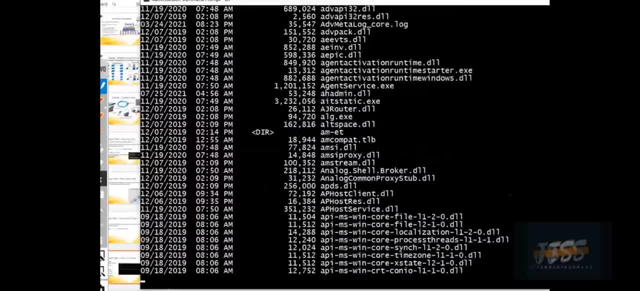 and this is also very helpful and handy. and this is also very helpful and handy, like in this case, if i type directory, like in this case, if i type directory, like in this case, if i type directory and you can see there's so many things, and you can see there's so many things. 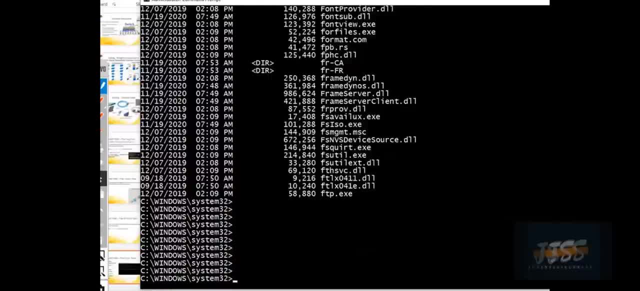 and you can see there's so many things, as so many pages, as so many pages, as so many pages. uh, it is going through, but i do not want. uh, it is going through, but i do not want. uh, it is going through, but i do not want this behavior. i want page by page. so what? 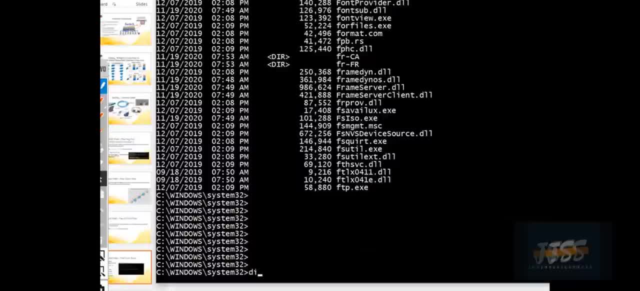 this behavior. i want page by page. so what? this behavior? i want page by page. so what you can do, you can do, you can do, you can type, you can type, you can type directory, directory, directory, then five command and more, then five command and more, then five command and more. now you will hit enter, you will see it. 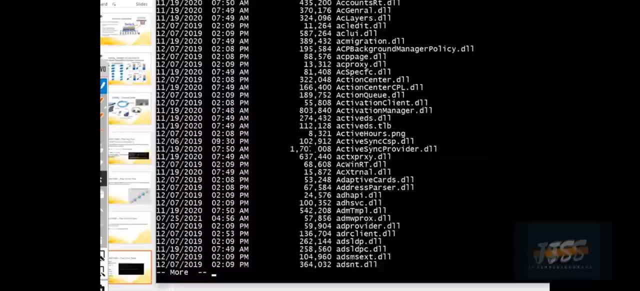 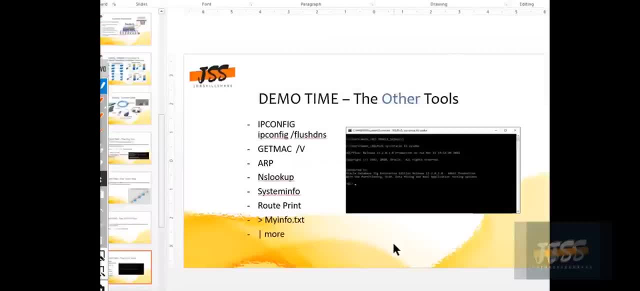 now you will hit enter, you will see it. now you will hit enter, you will see it is gonna go page by page. is gonna go page by page. is gonna go page by page. okay, so our demo time, so our demo time, so our demo time, uh, ends here. 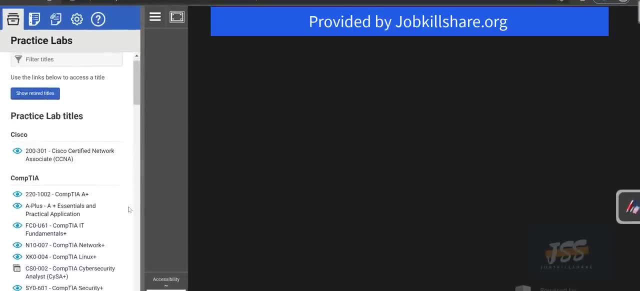 uh ends here. uh ends here the next part of this training. we will the next part of this training, we will, the next part of this training, we will use, use, use different command line videos from our different command line videos, from our different command line videos from our practice lab. 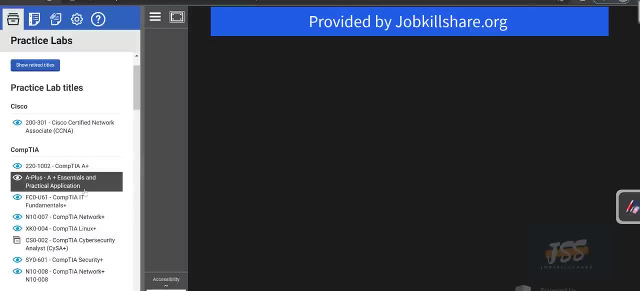 practice lab. practice lab that we use in our system. so if you want that we use in our system. so if you want that we use in our system. so if you want to do a practical practice, just like to do a practical practice, just like to do a practical practice, just like instructor. 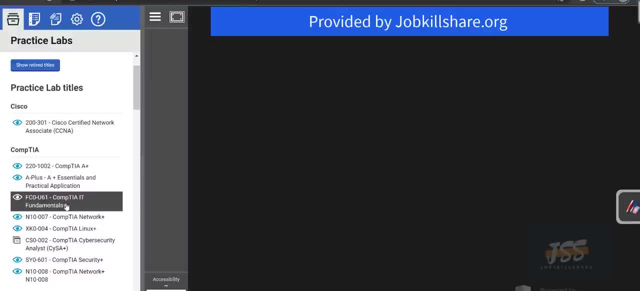 instructor, instructor. you may want to get a membership on. you may want to get a membership on. you may want to get a membership on jobskillshareorg- jobskillshareorg, jobskillshareorg- especially premium membership. because you especially premium membership, because you especially premium membership. because you will see that we will be jumping around. 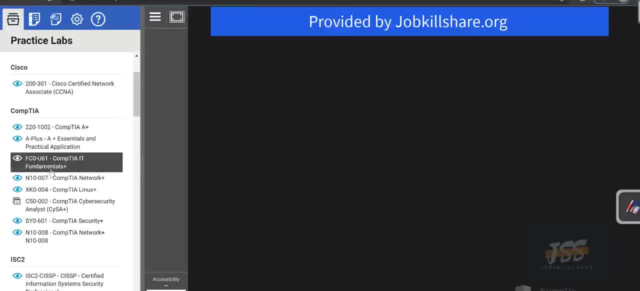 will see that we will be jumping around, will see that we will be jumping around in different courses because we in different courses, because we in different courses, because we have these type of modules inside courses, have these type of modules inside courses, have these type of modules inside courses, for example. 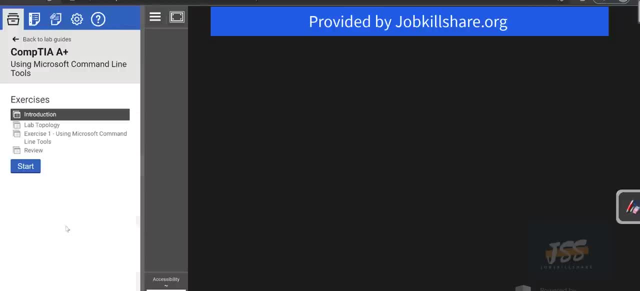 for example, for example, in comtia. there's a full command line in comtia. there's a full command line in comtia. there's a full command line. set right here that you will be working. set right here that you will be working. set right here that you will be working on hands-on. so we are going to add some. 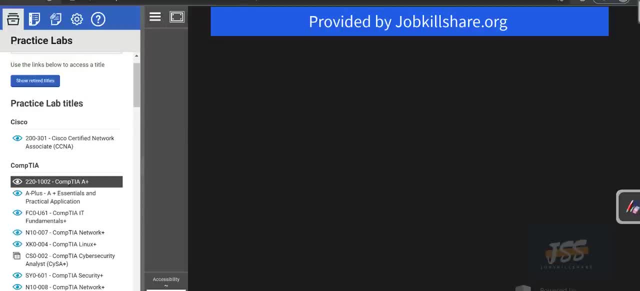 on hands-on, so we are going to add some on hands-on. so we are going to add some of the videos from different modules over of the videos from different modules, over of the videos from different modules over here, here, here, to enhance this video for your learning. 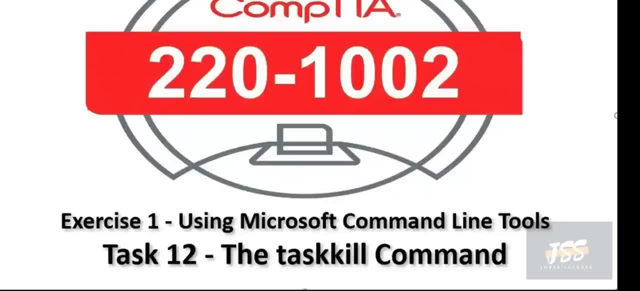 to enhance this video for your learning, to enhance this video for your learning. thank you, the task kill command. thank you, the task kill command. thank you, the task kill command, and here in this video, we're going to, and here in this video, we're going to, and here in this video we're going to show you this command. so, 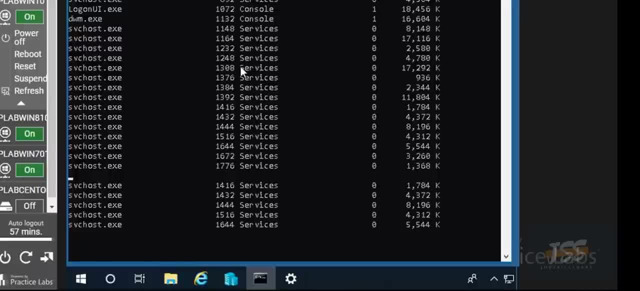 show you this command. so show you this command. so if the screen is not clear, so first run. if the screen is not clear, so first run. if the screen is not clear, so first run the cls and this the cls and this the cls and this. then we're going to run the task kill. 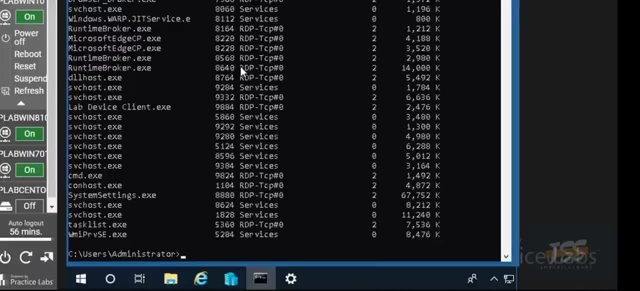 then we're going to run the task kill, then we're going to run the task kill. task list command. so task list command, so task list command. so for killing any tasks, you must know, for killing any tasks, you must know. for killing any tasks, you must know the task and the list of that. 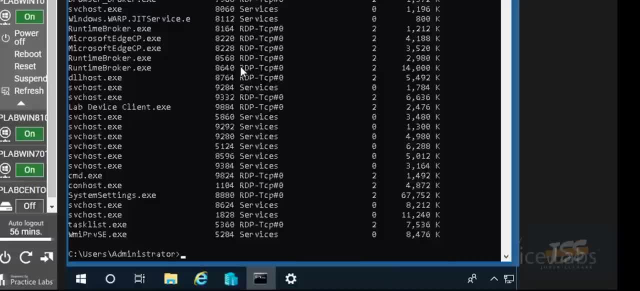 the task and the list of that, the task and the list of that, all the tasks from which you want to, all the tasks from which you want, to, all the tasks from which you want to select, select, select. any of the tasks to kill, so before that, any of the tasks to kill, so before that. 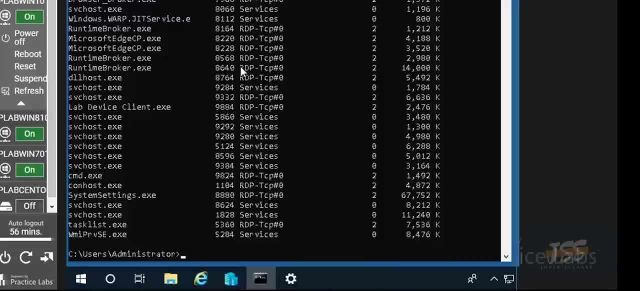 any of the tasks to kill. so, before that you run the task list command, and here you run the task list command, and here you run the task list command, and here you will find, you will find, you will find there are a lot more tasks that are. there are a lot more tasks that are. 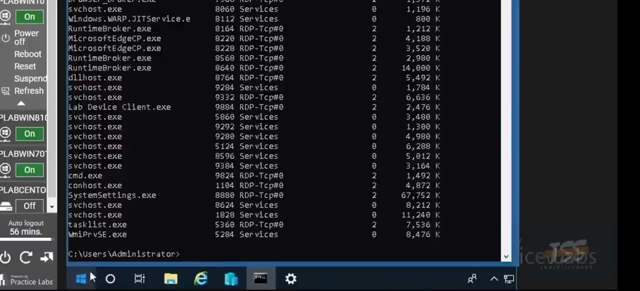 there are a lot more tasks that are running because definitely when you're running, because definitely when you're running, because definitely when you're using operating system or any operating using operating system or any operating using operating system or any operating system, system, system, there are a few more services running. 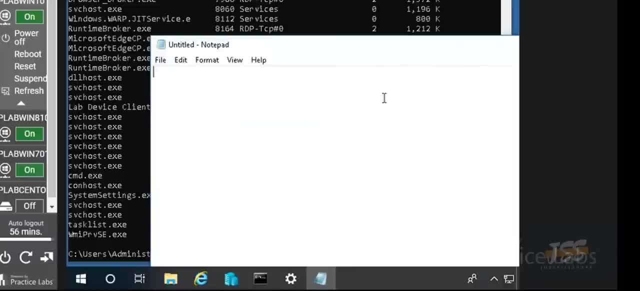 there are a few more services running. there are a few more services running on the background. that is allowing you on the background, that is allowing you on the background, that is allowing you, letting you to use the resources and letting you to use the resources and letting you to use the resources and doing your own daily operations. so here, 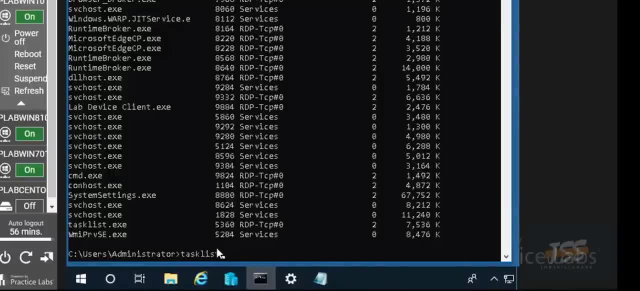 doing your own daily operations. so here doing your own daily operations. so here we cannot easily see all the tasks here. we cannot easily see all the tasks here. we cannot easily see all the tasks here, so we're going to type the task. so we're going to type the task. 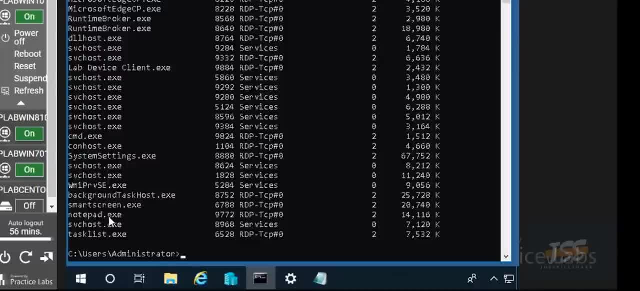 so we're going to type the task list and we're going to list and we're going to list and we're going to just type the notepad here to show: just type the notepad here to show: just type the notepad here to show that how the task is being added. so as 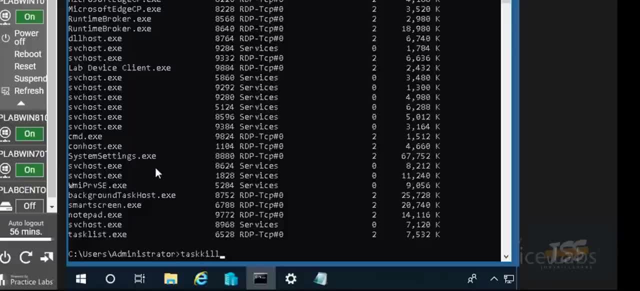 that how the task is being added. so as that how the task is being added. so as we open the notepad. you can see the. we open the notepad. you can see the. we open the notepad. you can see. the notepad is now came under the task list. 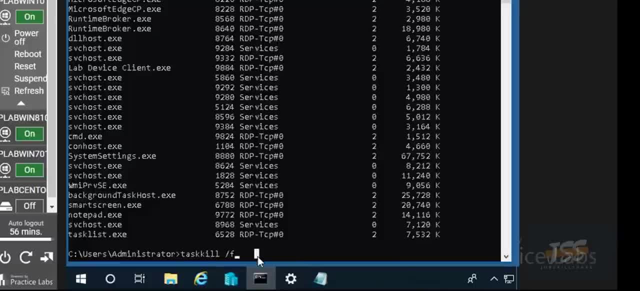 notepad is now came under the task list. notepad is now came under the task list. now we're going to type the task kill. now we're going to type the task kill. now we're going to type the task kill because we're going to, because we're going to. 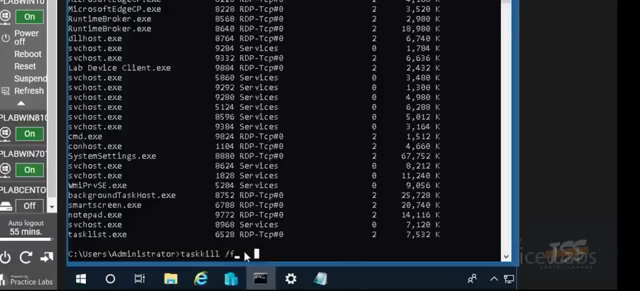 because we're going to shut down. we're going to kill the task shut down. we're going to kill the task shut down. we're going to kill the task that is running. that is running. that is running in the notepad form. so for that we're. 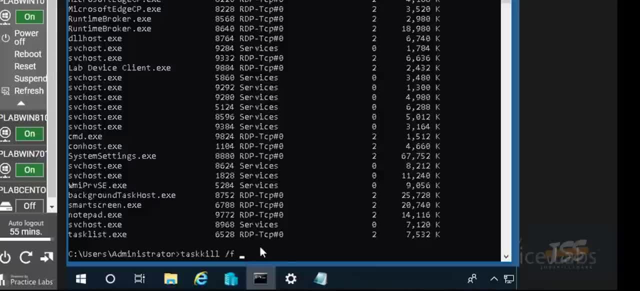 in the notepad form. so for that we're in the notepad form. so for that we're going to type test kill space full slash. going to type test kill space, full slash. going to type test kill space, full slash, f. f means forcefully, because we don't. 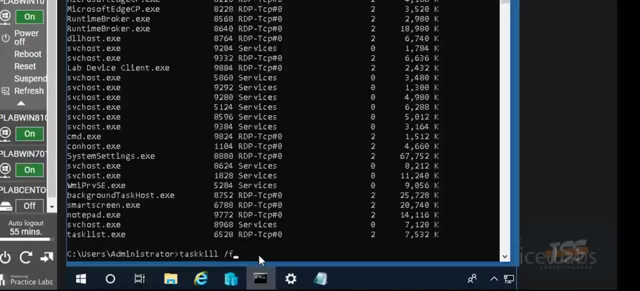 f. f means forcefully, because we don't f. f means forcefully because we don't need little laps in between to kill the need. little laps in between to kill the need. little laps in between to kill the test. that's why test, that's why test, that's why we are adding this argument. 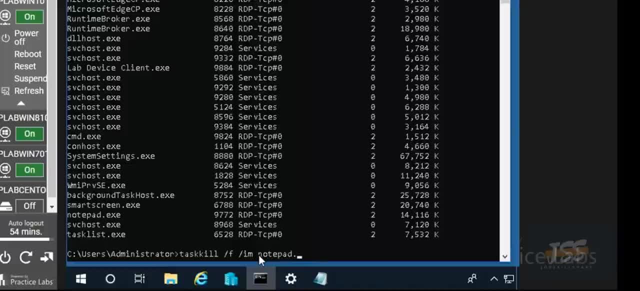 we are adding this argument. we are adding this argument and space forward slash im and space forward slash im and space forward slash im. notepad dot xc. notepad dot xc. notepad dot xc. so it will do what it will. so it will do what it will. 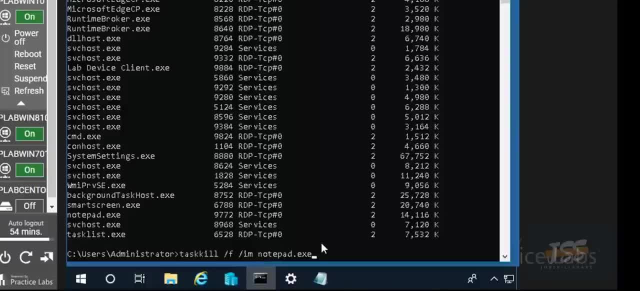 so it will do what it will: kill this task and kill this task and kill this task and close this application and whatever it close this application and whatever it close this application and whatever it is. sometimes there are application in is, sometimes there are application in is. sometimes there are application in the test, sometimes there are services. 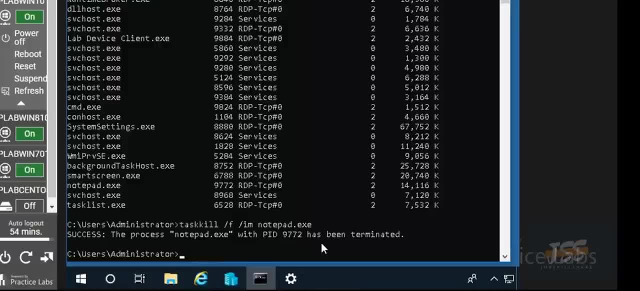 the test, sometimes there are services, the test, sometimes there are services, so it will, so it will, so it will terminate. and yes, here you can see the terminate. and yes, here you can see the terminate. and yes, here you can see the message that tells, message that tells. 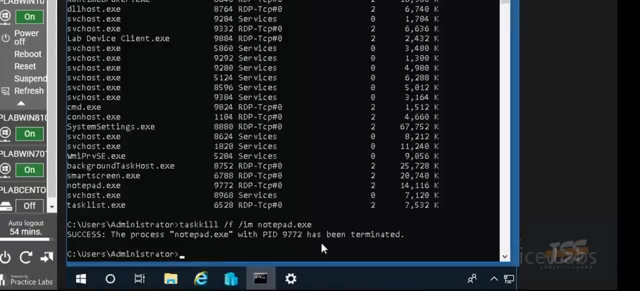 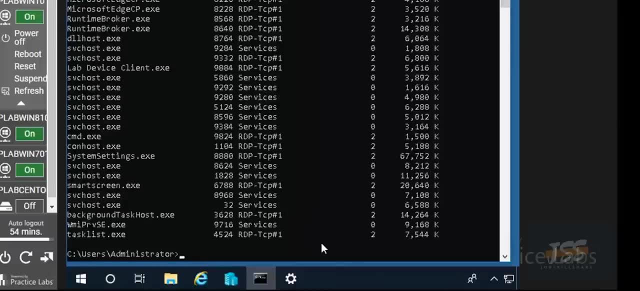 message that tells that this process with that pid has been, that this process with that pid has been that this process with that pid has been terminated, terminated, terminated now, after that, if you again now after that, if you again now after that, if you again run the task list command, you see here: 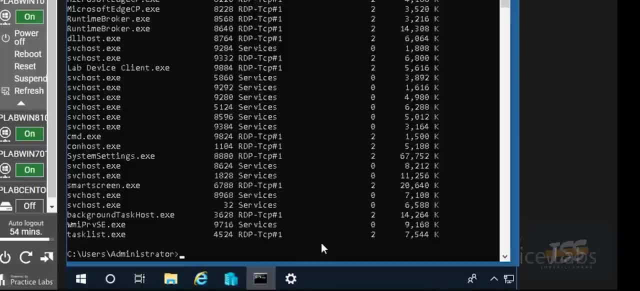 run the task list command you see here. run the task list command. you see here, there's no notepad file, there's no notepad. there's no notepad file. there's no notepad. there's no notepad file, there's no notepad task here. and also you can. 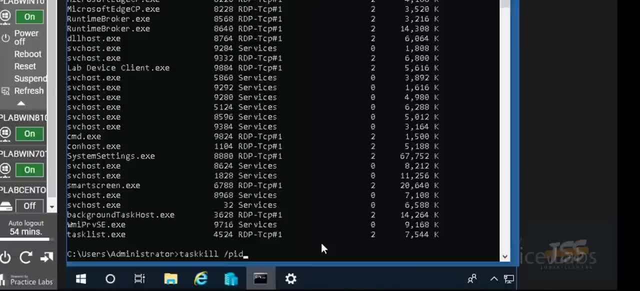 task here and also you can task here and also you can kill the test by kill the test by. kill the test by typing the pid: the process id of that typing the pid, the process id of that typing the pid, the process id of that specific task. specific task. 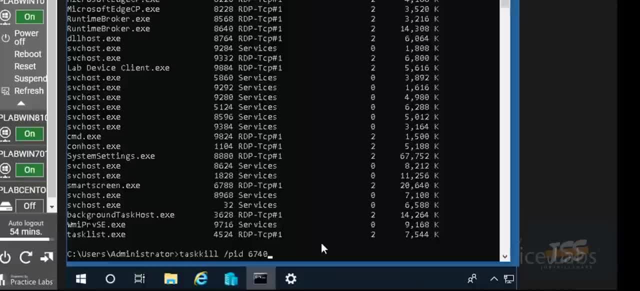 specific task. so you can type 6740 any specific task. so you can type 6740 any specific task. so you can type 6740 any specific task for the testing. you can kill by typing for the testing. you can kill by typing for the testing. you can kill by typing the id. and here this is the cmt: the same. 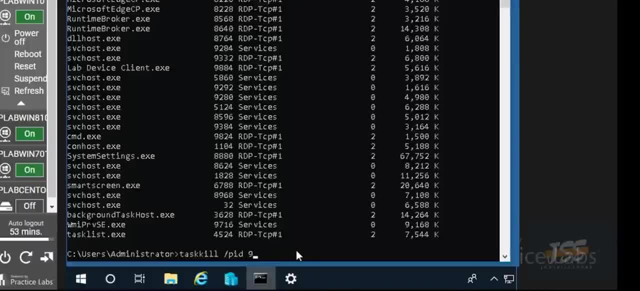 the id, and here this is the cmt: the same the id, and here this is the cmt: the same cmd which we are using. so if you type cmd, which we are using, so if you type cmd, which we are using, so if you type that, it will. 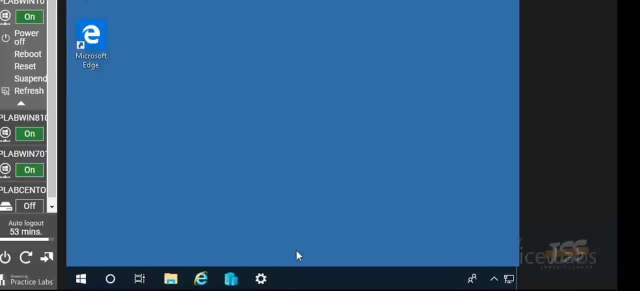 that it will, that it will close the cmd. and there you go: the cmd, close the cmd. and there you go: the cmd, close the cmd. and there you go. the cmd is closed, is closed, is closed. and that's how we can check how it kills and that's how we can check how it kills. 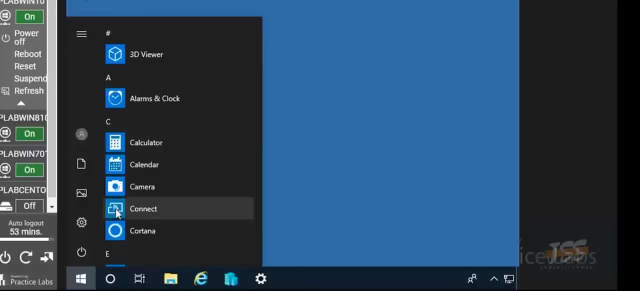 and that's how we can check how it kills the task, the task, the task, by using the pid, the process ids, by using the pid, the process ids, by using the pid, the process ids. so let us open the command prompt again. so let us open the command prompt again. 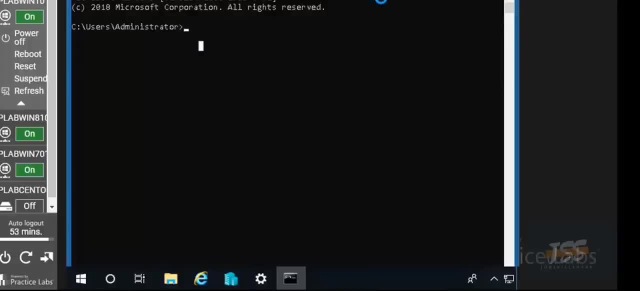 so let us open the command prompt again to further, to further, to further explore this task: kill command. explore this task, kill command. explore this task: kill command. other arguments that you can add with other arguments that you can add, with other arguments that you can add with the task kill command. 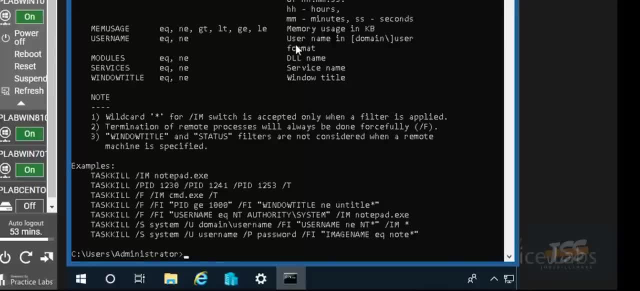 the task kill command. the task kill command. so simply type task kill space forward. so simply type task kill space forward. so simply type task kill space forward. slash question mark. slash question mark. slash question mark and it will show you other arguments. and it will show you other arguments. 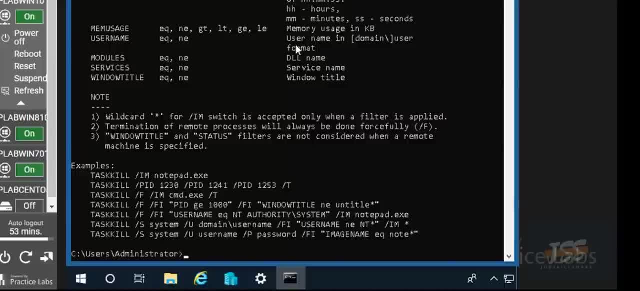 and it will show you other arguments and additions that you can and additions that you can and additions that you can apply with this test skill command: apply with this test skill command. apply with this test skill command. exercise 1: test 13: the gp update. exercise 1- test 13: the gp update. 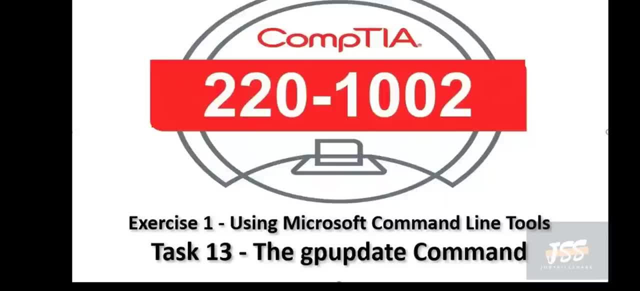 exercise 1, test 13: the gp update command command. command, and here in this test video we're going, and here in this test video we're going, and here in this test video we're going to show you how this gp update command, to show you how this gp update command. 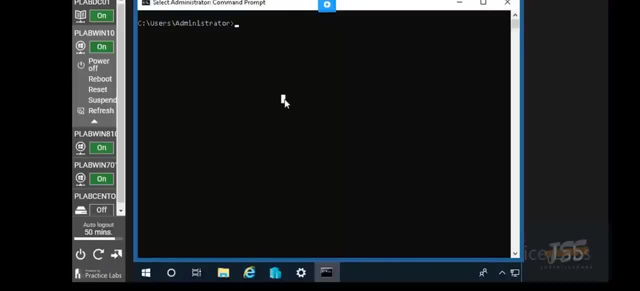 to show you how this gp update command works, works, works. so here, as you can see, we have the. so here, as you can see, we have the. so here, as you can see, we have the command prompt, command prompt, command prompt. on the screen, it's visible, and here. 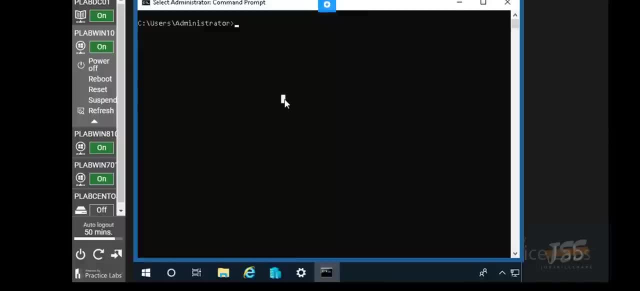 on the screen it's visible, and here on the screen it's visible. and here, if we type the gp update, if we type the gp update, if we type the gp update without any parameter, so without any parameter, so without any parameter, so you'll find that it will update. 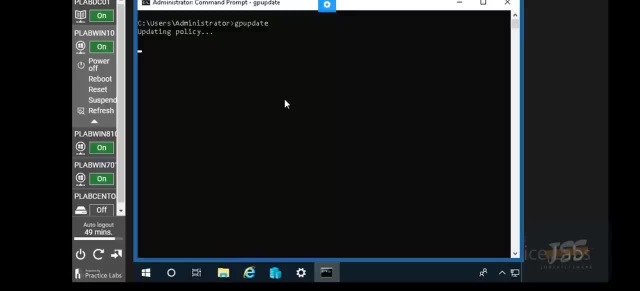 you'll find that it will update. you'll find that it will update. we'll clear the cache from this clan. we'll clear the cache from this clan. we'll clear the cache from this clan machine to the active directory machine, to the active directory machine, to the active directory domain controller machine, and it will. 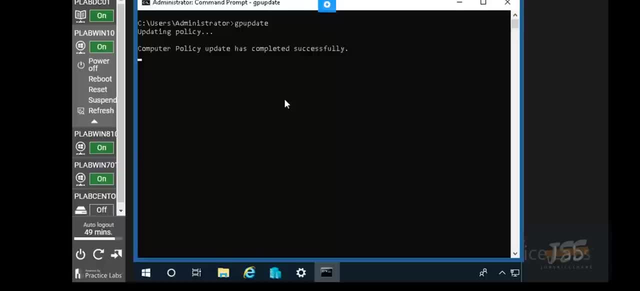 domain controller machine and it will. domain controller machine and it will just sync your machine's policies local. just sync your machine's policies, local, just sync your machine's policies, local policies, policies, policies with the group policies, so you will get. with the group policies, so you will get. 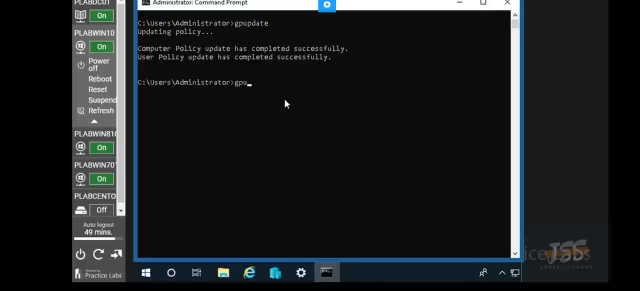 with the group policies, so you will get this message, this message, this message once the command is executed, that it is once the command is executed, that it is once the command is executed that it is done successfully, done successfully, done successfully. then if you add a parameter forward, 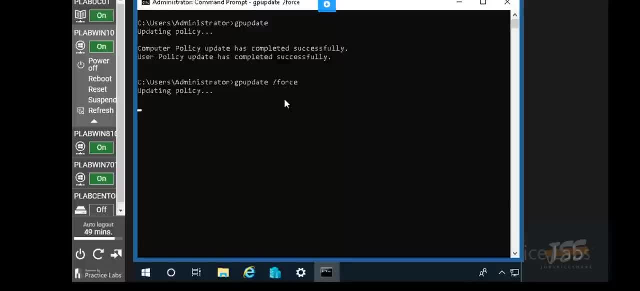 then if you add a parameter forward, then if you add a parameter forward, slash force, slash force, slash force. so it will do all the work with the. so it will do all the work with the. so it will do all the work with the force, with force, with. 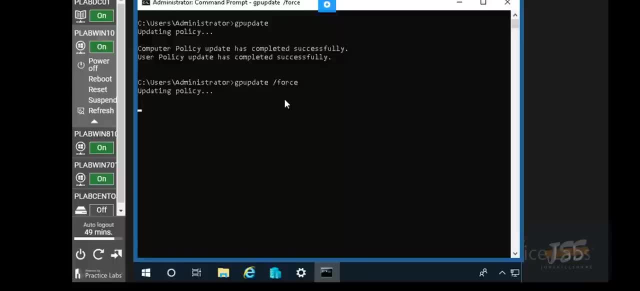 force with, within no matter of time, in quickly, quick, within no matter of time, in quickly, quick, within no matter of time, in quickly, quick, way, way, way. so if you want to do things in a quick, so if you want to do things in a quick, so if you want to do things in a quick way, in an instant, 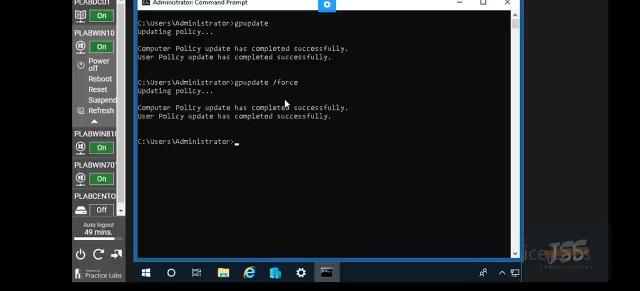 way, in an instant way, in an instant, so you can add this forward slash force. so you can add this forward slash force. so you can add this forward slash force argument with this command, and then argument with this command, and then argument with this command and then execute. 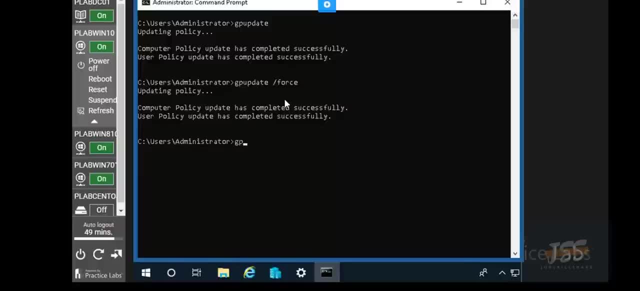 execute. execute, let's say. if you want to run the gp, let's say. if you want to run the gp, let's say: if you want to run the gp update by default user and the computer update by default user and the computer update by default user and the computer policies are applied. 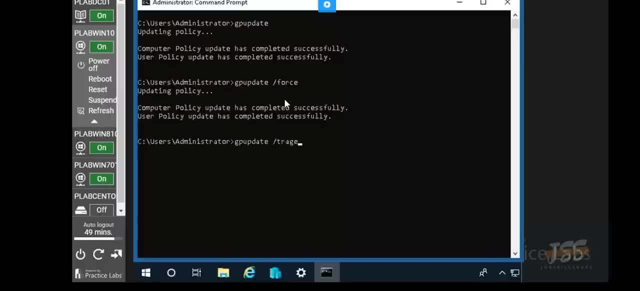 policies are applied. policies are applied so you can choose to apply either user, so you can choose to apply either user, so you can choose to apply either user or computer so you can add another, or computer so you can add another, or computer so you can add another argument. this forward slash target: 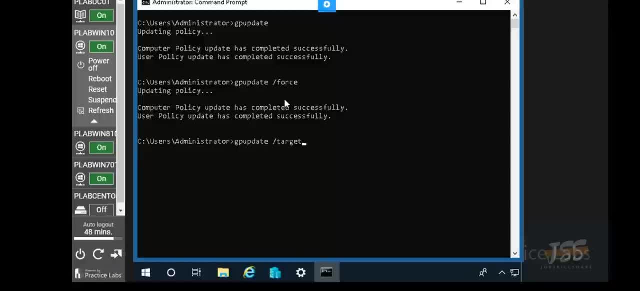 argument, this forward slash target argument, this forward slash target: colon: user, colon user, colon user. so because the policies are of two types, so because the policies are of two types, so because the policies are of two types, the computer base or the user base- so the computer base or the user base, so 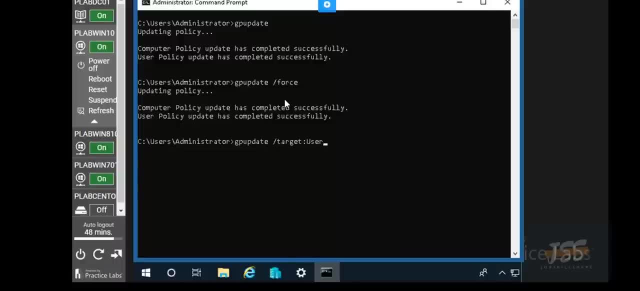 the computer base or the user base. so here here, here you're typing that we want new policies. you're typing that we want new policies. you're typing that we want new policies on the user level. so all the policies on the user level. so all the policies. 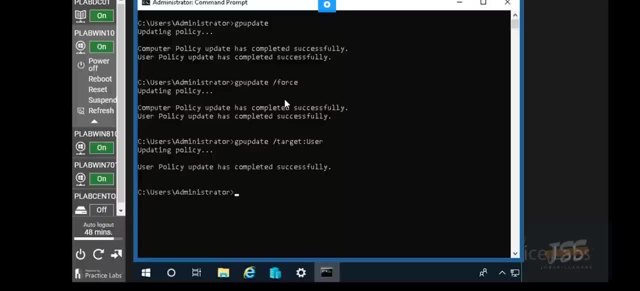 on the user level. so all the policies that were configured and altered on the that were configured and altered on the that were configured and altered on the user base are now the default number of user base, are now the default number of user base, are now the default number of seconds to wait for the policy. 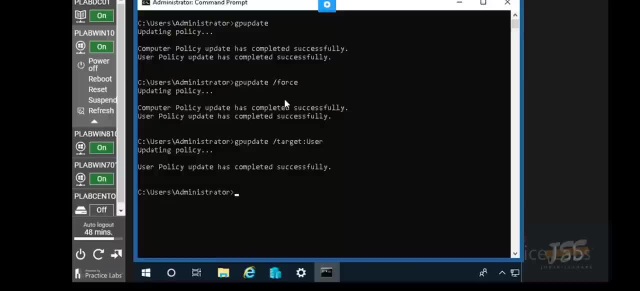 seconds to wait for the policy. seconds to wait for the policy processing is 600 seconds, so you can. processing is 600 seconds, so you can. processing is 600 seconds, so you can remove this wait time and add another. remove this wait time and add another. remove this wait time and add another argument with the numbers and reduce. 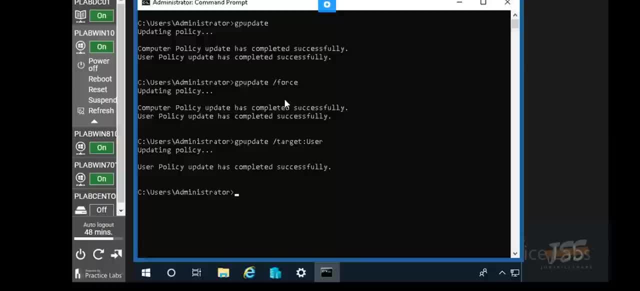 argument with the numbers and reduce argument with the numbers and reduce this wait time for the gp update, this wait time for the gp update, this wait time for the gp update. so it would be simple. you can type. so it would be simple. you can type. so it would be simple, you can type: gp update space. 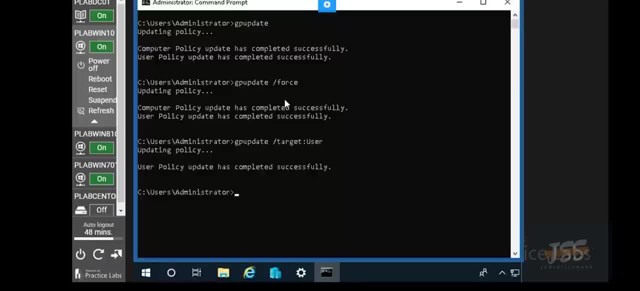 gp update space. gp update space. forward slash wait. and then you can forward slash wait, and then you can forward slash wait, and then you can type the number, the time, the seconds. type the number, the time, the seconds. type the number, the time, the seconds on which you want to reduce this. 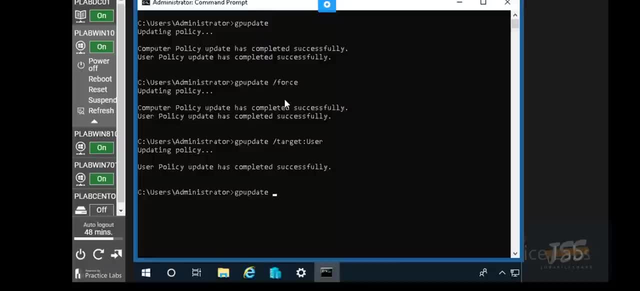 on which you want to reduce this, on which you want to reduce this implementation of the policies, implementation of the policies, implementation of the policies. so, in that way, in the, in this way you so, in that way, in the. in this way you so, in that way, in the. in this way, you can type gp: update space. 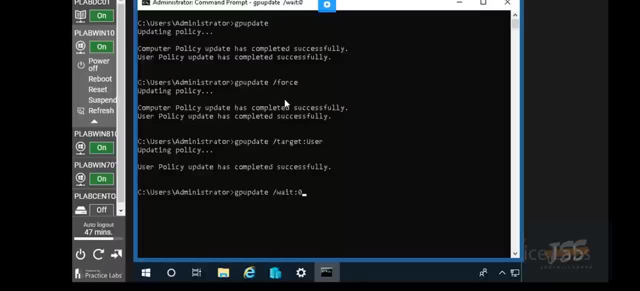 can type gp: update space. can type gp: update space: forward slash, wait, forward slash, wait forward, slash, wait, column zero. so we are reducing this column zero. so we are reducing this column zero. so we are reducing this 600 seconds to zero, 600 seconds to zero, 600 seconds to zero. so it will, it won't take. 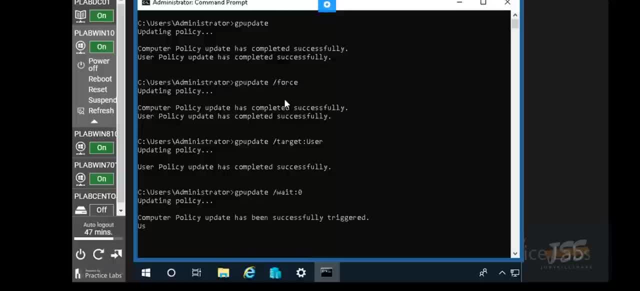 so it will. it won't take so it will. it won't take this much, this much, this much seconds and time to apply policy. seconds and time to apply policy. seconds and time to apply policy. now, let's clear the screen. and if you, now let's clear the screen. and if you. 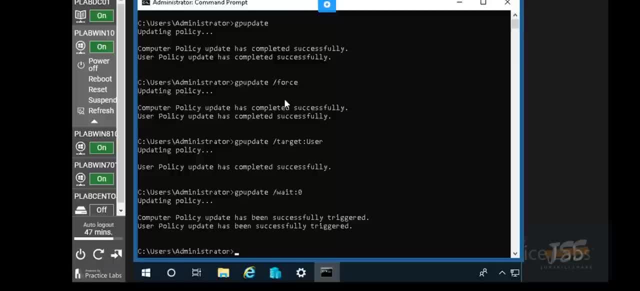 now let's clear the screen and if you want to further, want to further, want to further explore this gp update, explore this gp update, explore this gp update argument. so you could do the same argument, so you could do the same argument, so you could do the same thing. 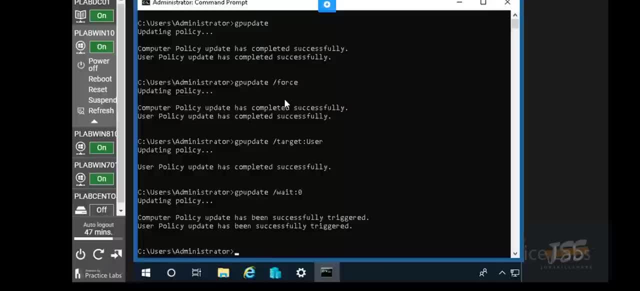 thing thing. as you did with the previous commands, as you did with the previous commands, as you did with the previous commands: like space, follow slash cushion mark. like space, follow slash cushion mark. like space, follow slash cushion mark. so it will show you other arguments. so it will show you other arguments. 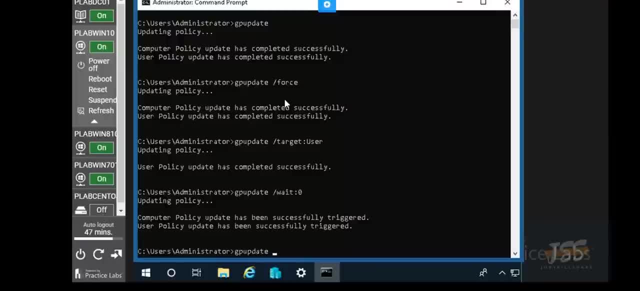 so it will show you other arguments and additions that you can add the and additions that you can add the. and additions that you can add the keywords that you can add with the keywords that you can add, with the keywords that you can add with the command and. 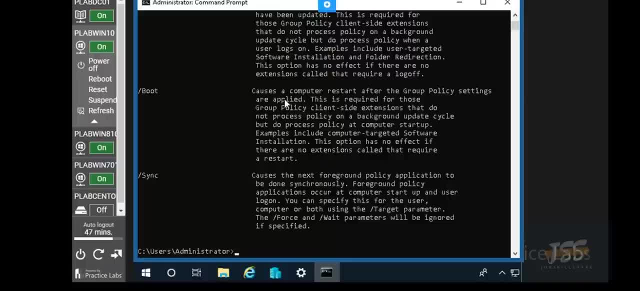 command and command and explore different features and explore different features. and explore different features and get benefit in different ways by using get benefit in different ways by using get benefit in different ways by using this command, the gp result command, and this command, the gp result command, and. 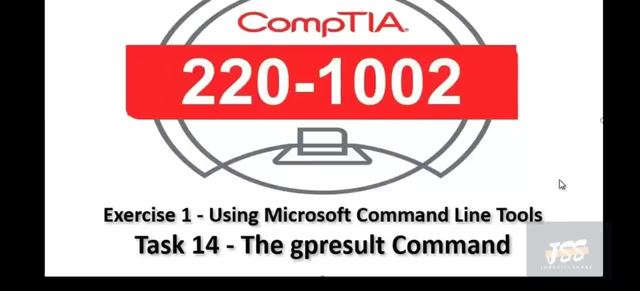 this command, the gp result command, and this is another command that helps you. this is another command that helps you. this is another command that helps you in the group policy section, in the group policy section, in the group policy section and here for the set of policies which 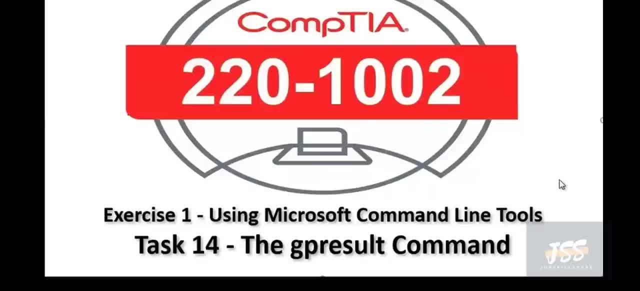 and here for the set of policies which, and here for the set of policies which get applied. these policies are about get applied. these policies are about get applied. these policies are about how to how to how to the application programs, resource based, the operating system, behave for the. 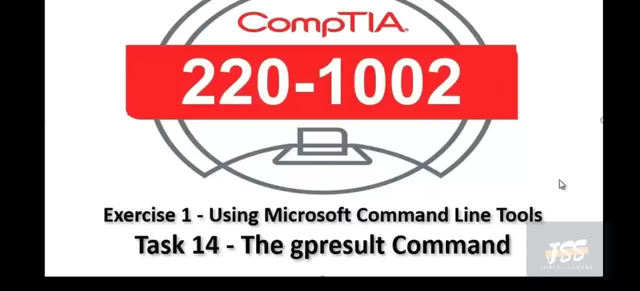 the operating system behave for the, the operating system behave for the particular user or a computer, particular user or a computer, particular user or a computer. so these policies can overlap in nature, so these policies can overlap in nature. so these policies can overlap in nature and this gp result command. 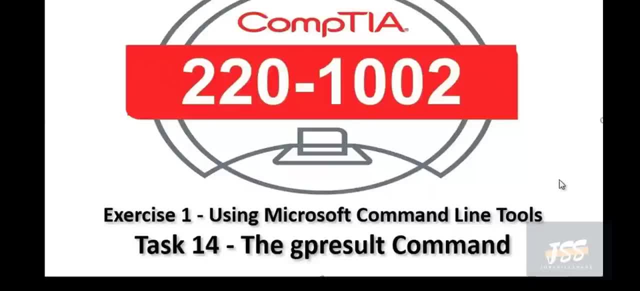 and this gp result command. and this gp result command generates the resulting set of the, generates the resulting set of the. generates the resulting set of the applicable policies. applicable policies. applicable policies: after considering the overlapping, after considering the overlapping, after considering the overlapping. so here in this video you're going to 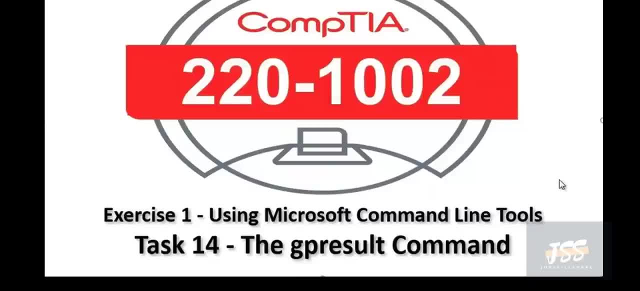 so here in this video you're going to so here in this video you're going to learn how to use, learn how to use, learn how to use this gp result command and to use the gp- this gp result command- and to use the gp- this gp result command- and to use the gp result command to. 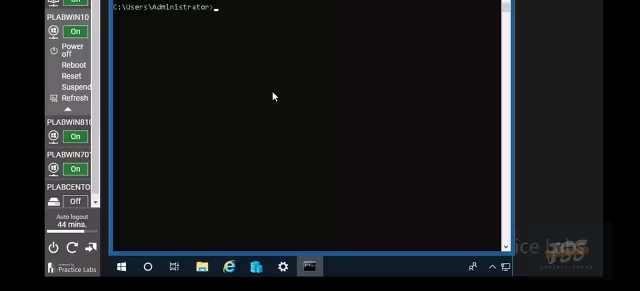 result: command to result. command to: to see, to see, to see the functions you, the functions you, the functions. you will need to follow these steps, that we will need to follow these steps, that we will need to follow these steps that we are going to show you are going to show you. 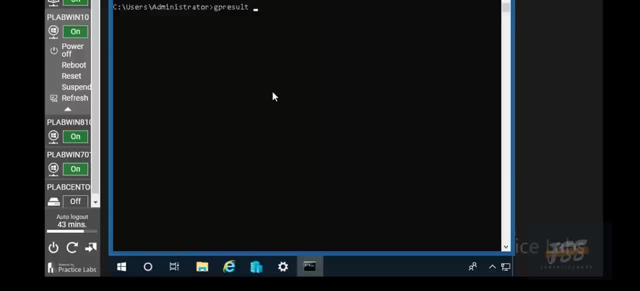 are going to show you. so if you type gp result- space forward. so if you type gp result- space forward. so if you type gp result- space forward, slash r, slash r, slash r, so it will display the rsop summary data. so it will display the rsop summary data. 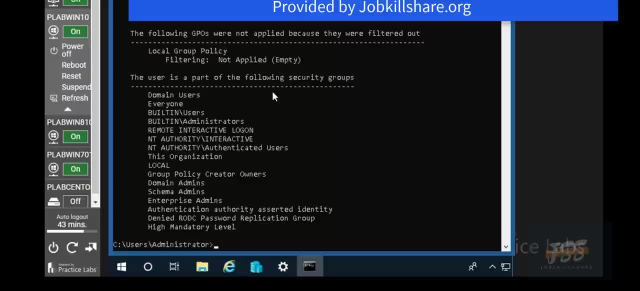 so it will display the rsop summary data of the policies and the user of the policies and the user of the policies and the user and the security groups. so, and the security groups. so, and the security groups. so you can maximize the command prompt. you can maximize the command prompt. 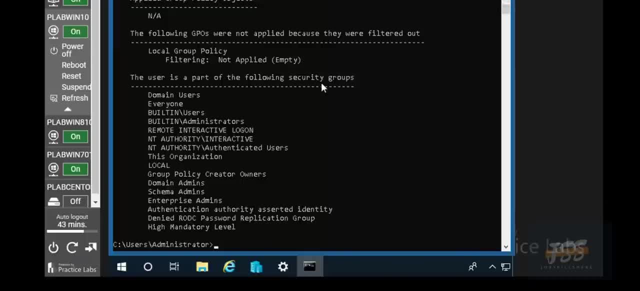 you can maximize the command prompt window, window window, if you further want to see each, and if you further want to see each, and if you further want to see each and everything, everything, everything, and once you realize, once you find out, and once you realize, once you find out, 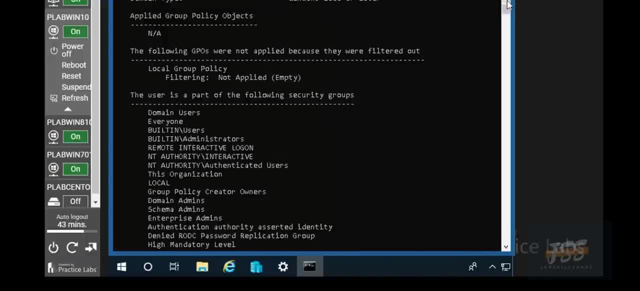 and once you realize, once you find out all the stuff and the policies, that are all the stuff and the policies, that are all the stuff and the policies that are applied and working right now, applied and working right now, applied and working right now. so, so, so there's, you will find there's a lot of. 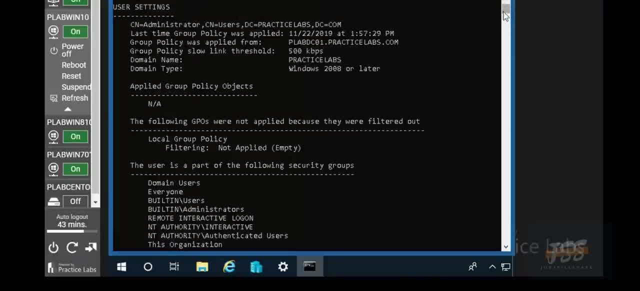 there's, you will find there's a lot of there's, you will find there's a lot of stuff and a lot of things, stuff and a lot of things, stuff and a lot of things. a lot of policies applied on the user. a lot of policies applied on the user. 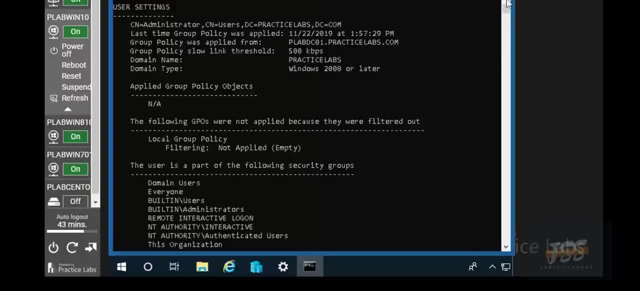 a lot of policies applied on the user level, on the computer level level, on the computer level level, on the computer level. so you can easily, so you can easily, so you can easily find out the difference, find out the difference, find out the difference and once you get this output from the 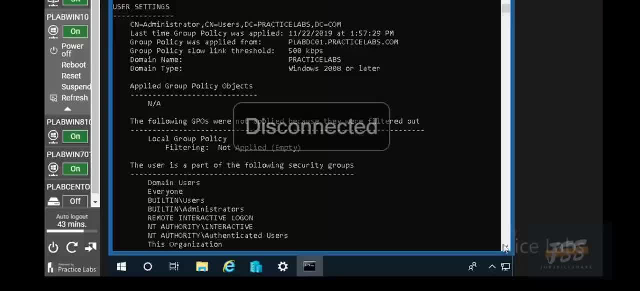 and once you get this output from the and once you get this output from the gp result command- gp result command- gp result command- you can also display all the information. you can also display all the information. you can also display all the information about the group policy, about the group policy. 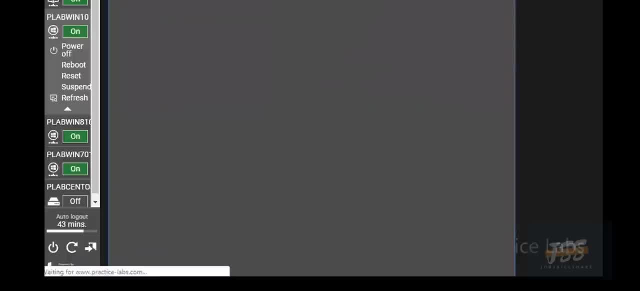 about the group policy and this work by, and this work by, and this work by adding another argument with this gp, adding another argument with this gp, adding another argument with this gp: result, command, result, command, result, command. now, here, the machine is disconnected. and now here, the machine is disconnected and 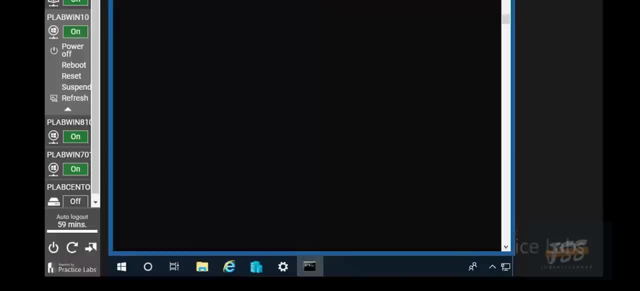 now, here, the machine is disconnected and once when it happens, click to the once when it happens, click to the once when it happens, click to the reconnect button, reconnect button, reconnect button, and it will reconnect the machine as it and it will reconnect the machine as it and it will reconnect the machine as it were connected. 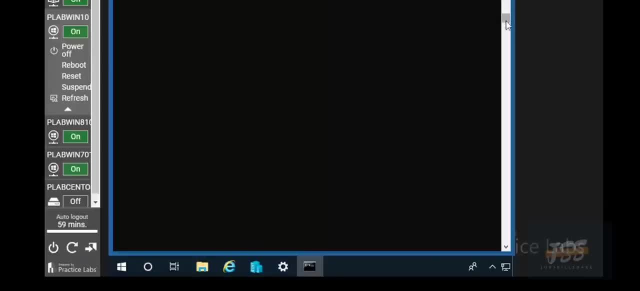 were connected, were connected on the same moment, on the same point, on the same moment, on the same point, on the same moment, on the same point. so let me scroll up and reach to that. so let me scroll up and reach to that. so let me scroll up and reach to that point where we left. 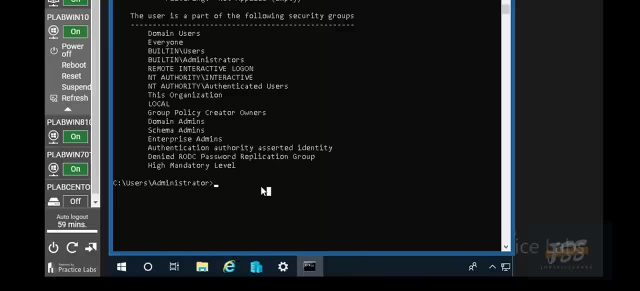 point where we left. point where we left, and here i'm gonna run another gp, and here i'm gonna run another gp, and here i'm gonna run another gp. result command with another argument. result command with another argument. result command with another argument. and that would be false like z. 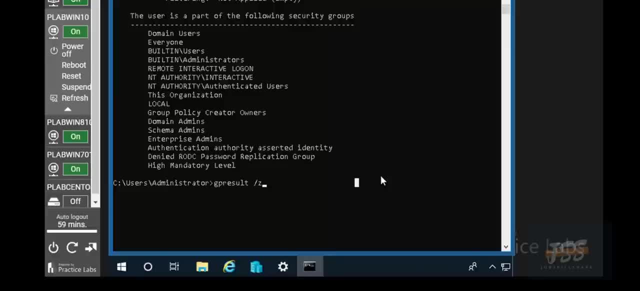 and that would be false like z, and that would be false like z. so it gonna do what it will display. so it gonna do what it will display. so it gonna do what it will display: all the information about the group. all the information about the group, all the information about the group policy. 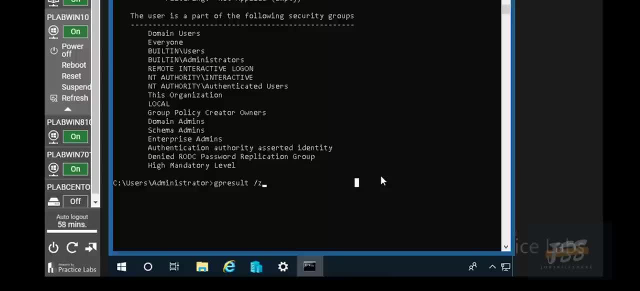 policy policy. and let's press enter to execute, and let's press enter to execute, and let's press enter to execute. and here you can see the output of this. and here you can see the output of this. and here you can see the output of this command. 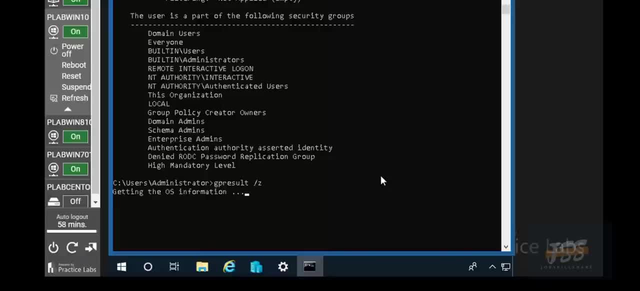 command. command spans through multiple pages, so you need spans through multiple pages. so you need spans through multiple pages, so you need to scroll and read the information. to scroll and read the information. to scroll and read the information and you can also find out the details and you can also find out the details. 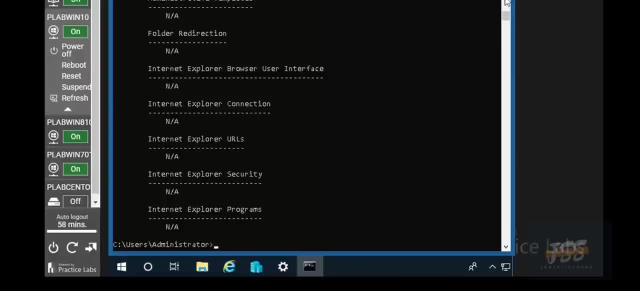 and you can also find out the details from the screenshots, from the screenshots, from the screenshots. so this is the output and it tells you. so this is the output and it tells you. so this is the output, and it tells you that each specific policy, that is, that each specific policy, that is. 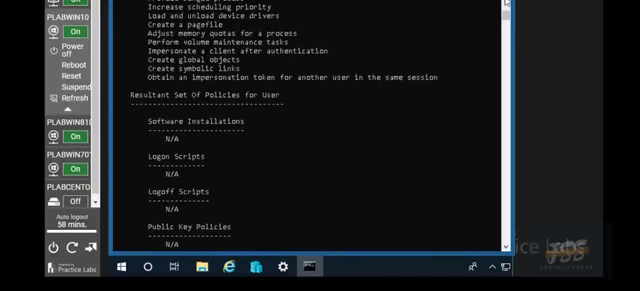 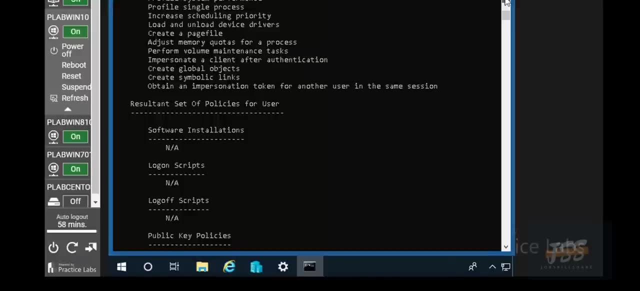 that each specific policy that is applied on each object applied on each object, applied on each object in your environment, in your group policy, in your environment, in your group policy, in your environment, in your group policy. so, once after getting this, so once after getting this, so once after getting this detail about the group policy, and 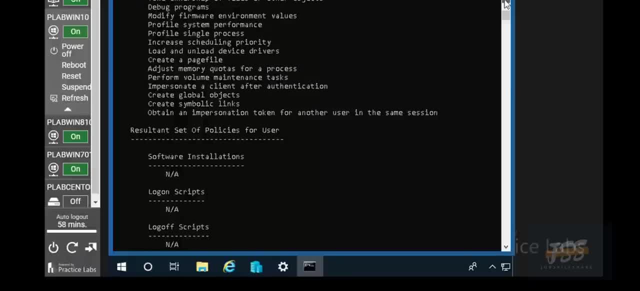 detail about the group policy and detail about the group policy and actually this is allowing you, actually this is allowing you, actually this is allowing you. let's say, for example, if you applied. let's say, for example, if you applied. let's say, for example, if you applied some policies on the machine and the 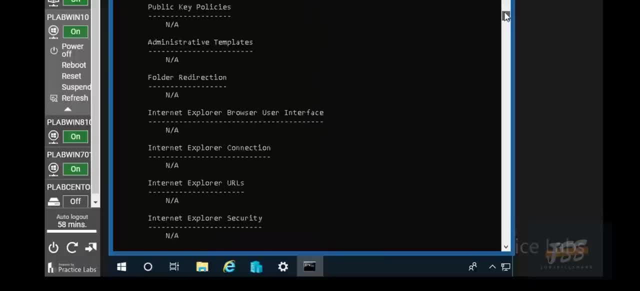 some policies on the machine and the some policies on the machine and the machine didn't get that policy. it is not machine didn't get that policy. it is not machine didn't get that policy. it is not implemented at the moment. implemented at the moment. implemented at the moment. so you can run this gp result forward. 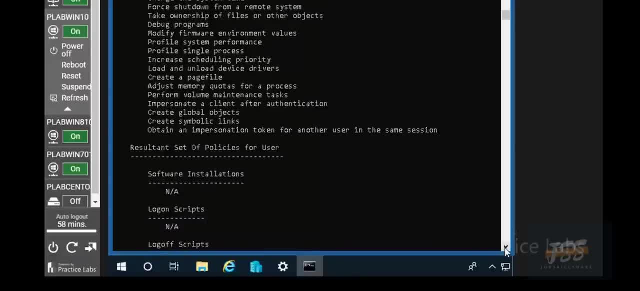 so you can run this gp result forward. so you can run this gp result forward: slash, slash, slash z command and it will show you which z command. and it will show you which z command and it will show you which policy policy policy is being altered and configured for. 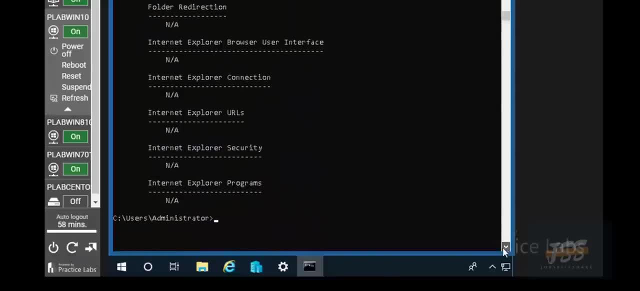 is being altered and configured for, is being altered and configured for which object? which object, which object? so there are a lot of benefits, and so there are a lot of benefits. and so there are a lot of benefits and a lot of different. you could say a lot of different. you could say: 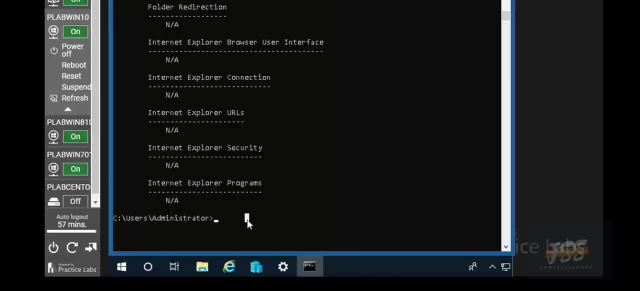 a lot of different. you could say: tools you're getting by learning these tools. you're getting by learning these tools. you're getting by learning these commands, commands, commands, issues in active directory. issues in active directory, issues in active directory. now once getting this much. now once getting this much. 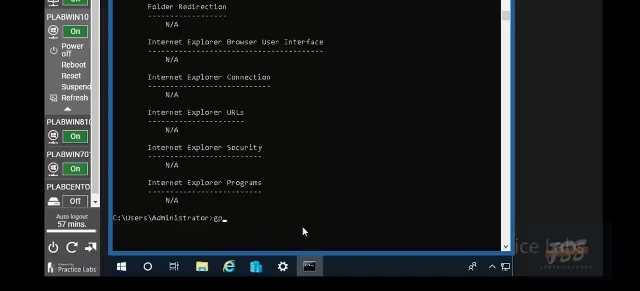 now, once getting this much lengthy, lengthy, lengthy output, output output. you can clear the screen or you can run. you can clear the screen or you can run. you can clear the screen or you can run. another command, another command. another command that shows the details of remote. that shows the details of remote. 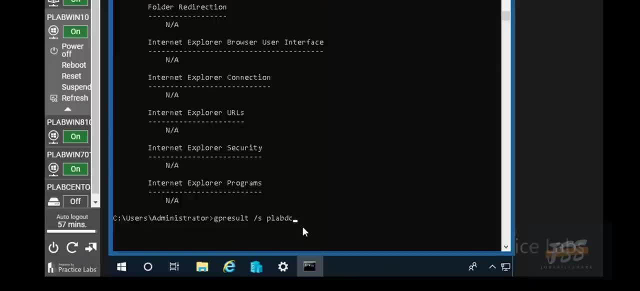 that shows the details of remote computer computer computer. it display the policy details of remote. it display the policy details of remote. it display the policy details of remote computer. so you can type computer. so you can type computer. so you can type gp reserve s space, gp reserve s space. 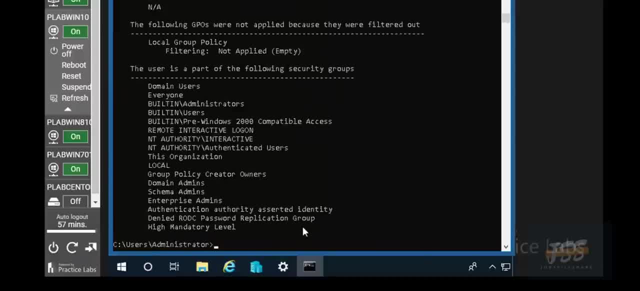 gp reserve s space, that specific remote machine, and then that specific remote machine, and then that specific remote machine, and then forward slash r, forward slash r, forward slash r. so it will provide you the detail of, so it will provide you the detail of so it will provide you the detail of that remote computer, the policies that 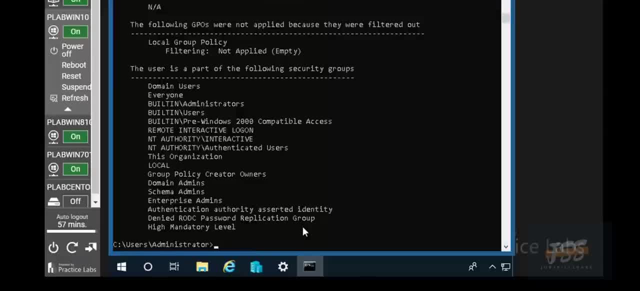 that remote computer. the policies that that remote computer, the policies that are implemented on that specific machine, are implemented on that specific machine, are implemented on that specific machine. so you can explore, you can find out the. so you can explore, you can find out the. so you can explore, you can find out the policies of another machine, of another. 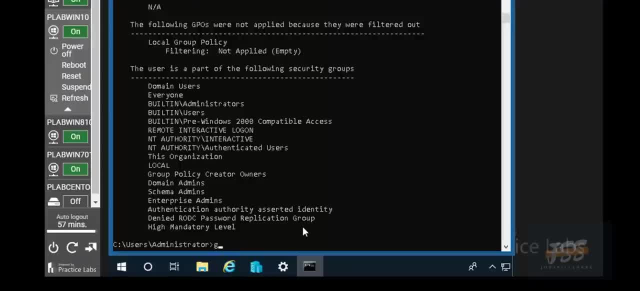 policies of another machine, of another policies of another machine, of another remote computer, within your domain, within remote computer, within your domain, within remote computer, within your domain, within your network. by running this command, the your network. by running this command, the your network. by running this command, the net use command and this command is used. 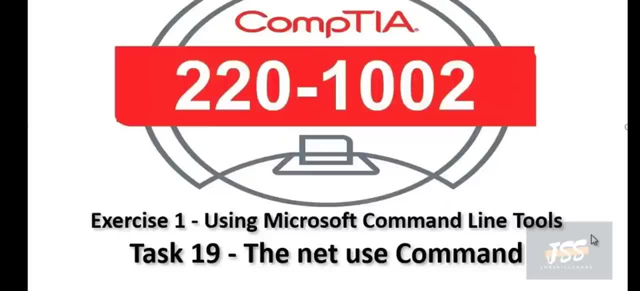 net use command and this command is used. net use command. and this command is used to connect your computer system to the, to connect your computer system to the. to connect your computer system to the shared folder or drive on the network. so shared folder or drive on the network, so. 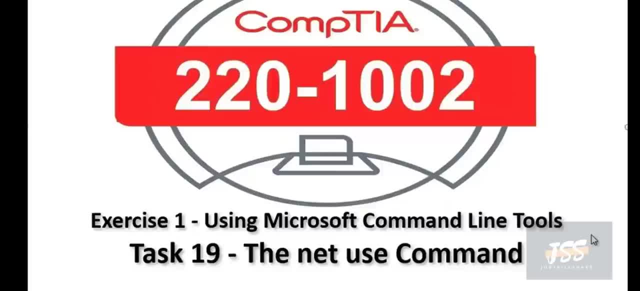 shared folder or drive on the network. so, by using this command, it's possible to. by using this command, it's possible to. by using this command, it's possible to have the direct access to such have, the direct access to such have, the direct access to such shared directories, and treating it as it. 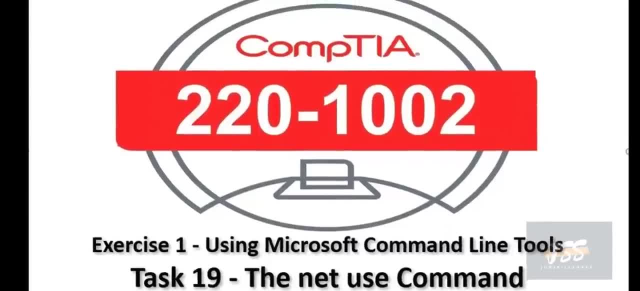 shared directories and treating it as it shared directories. and treating it as it as if it is a local directory or drive, as if it is a local directory or drive as if it is a local directory or drive. so there are different variations with. so there are different variations with. 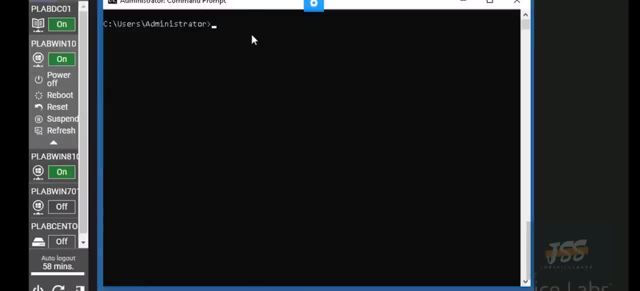 so there are different variations with this command which we're going to show, this command which we're going to show, this command which we're going to show you later in this video, you later in this video, you later in this video. so basically, in a simple way, you can. 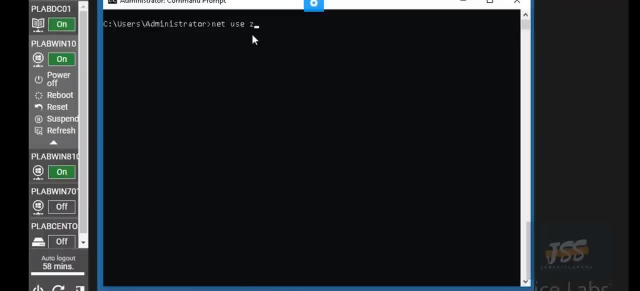 so, basically, in a simple way, you can. so, basically, in a simple way, you can type net use command to view the type net use command, to view the type net use command, to view the existing network connection, existing network connection, existing network connection. so you type net use space z colon. 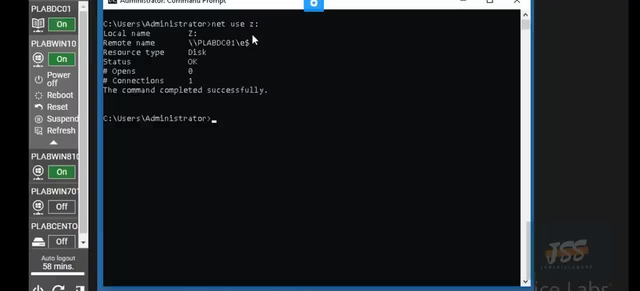 so you type net use space z colon. so you type net use space z colon, so you will start seeing. so you will start seeing. so you will start seeing the shared drive. and there you go the, the shared drive. and there you go the, the shared drive. and there you go, the command successfully. 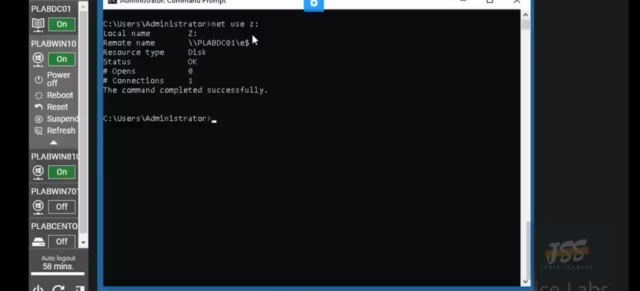 command successfully, command successfully executed and you have currently executed, and you have currently executed and you have currently this detail within this, this detail within this, this detail within this network drive command, network drive command, network drive command: now we can also map a network share, or now we can also map a network share, or 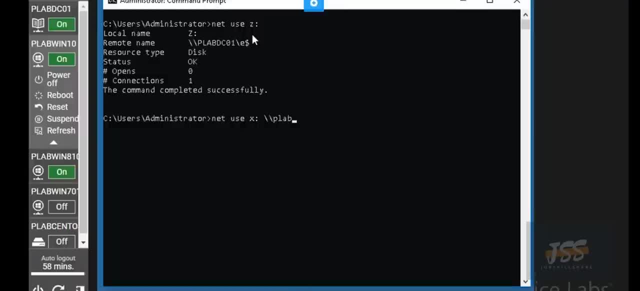 now we can also map a network share or drive or specific drive letter on your drive or specific drive letter on your drive or specific drive letter on your system so you can use nets net space used system. so you can use nets net space used system. so you can use nets net space used space. x colon double backslash p live. 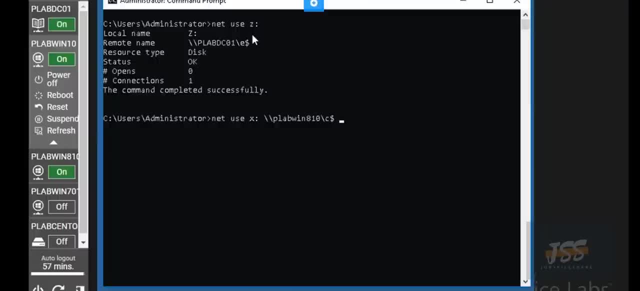 space x- colon. double backslash: p live. space x, colon. double backslash p live. eight one c dollar c is the c location. eight one c dollar c is the c location. eight one c dollar c is the c location. false is persistent. false is persistent. false is persistent. colon: yes, so when you type this, 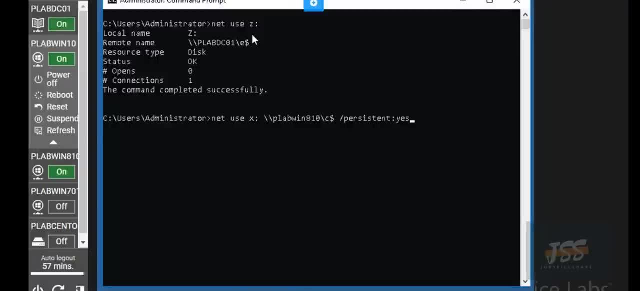 colon yes. so when you type this colon yes. so when you type this value, so the value yes means value. so the value yes means value. so the value yes means that the mapping will be available when that the mapping will be available, when that the mapping will be available when you log on to the system next time. and 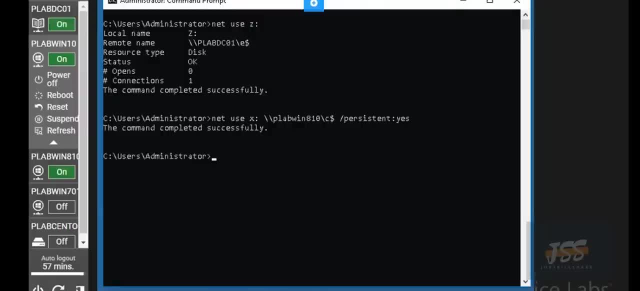 you log on to the system next time, and you log on to the system next time. and when you go with no, that means the. when you go with no. that means the. when you go with no. that means the mapping is limited to this session only. mapping is limited to this session only. 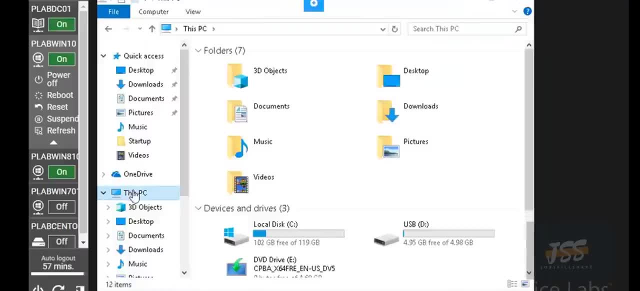 mapping is limited to this session, only if you minimize the command prompt and if you minimize the command prompt and if you minimize the command prompt and want to see go to the file explorer, so want to see go to the file explorer, so want to see go to the file explorer, so you're going to find this x drive. 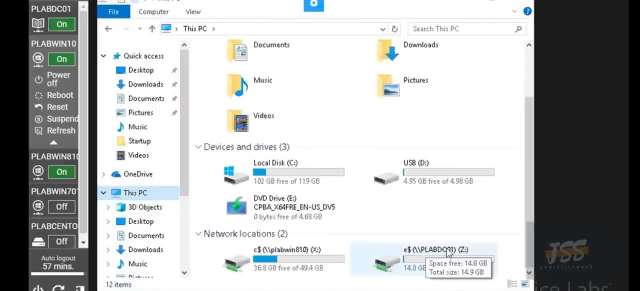 you're going to find this x drive. you're going to find this x drive here, here, here, on your system, on your machine, on your system, on your machine, on your system, on your machine. and you go with yes, so it will be. and you go with yes, so it will be. 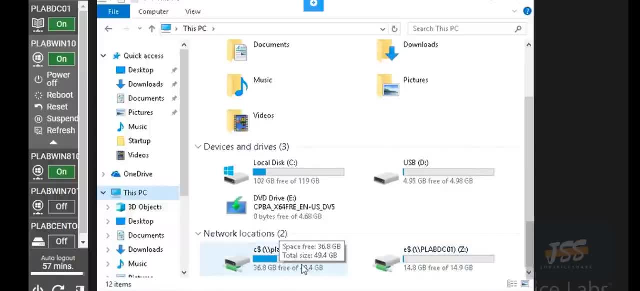 and you go with: yes, so it will be available when you re-log to your system, available when you re-log to your system, available when you re-log to your system again, again, again, now, if you want to delete this network, now, if you want to delete this network. 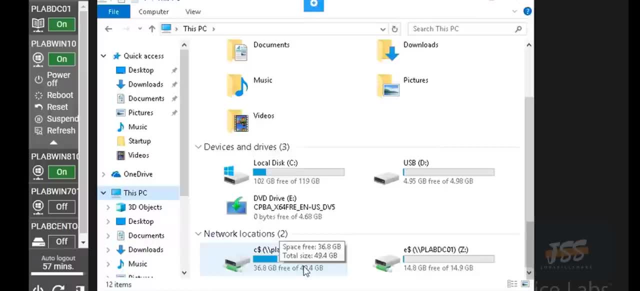 now, if you want to delete this network, drive, drive, drive. because if you don't need that drive, because if you don't need that drive, because if you don't need that drive, and the time and want to delete that, and the time and want to delete that. 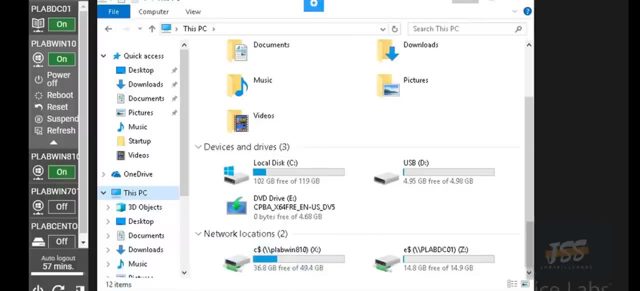 and the time and want to delete that specific drive, specific drive, specific drive. so for that you have. so for that you have. so for that you have basic and simple argument of this net. basic and simple argument of this net. basic and simple argument of this net use command. 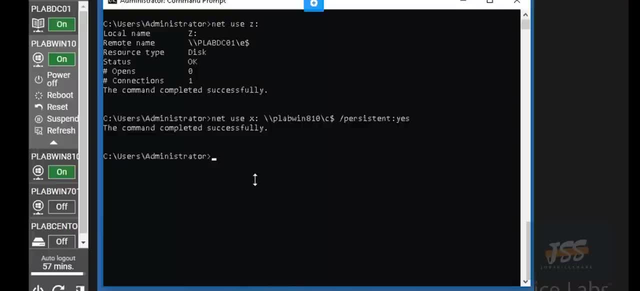 use command. use command that you can add with it, that you can add with it, that you can add with it, and run and run and run, and here you need to specify the letter and here you need to specify the letter, and here you need to specify the letter first. so 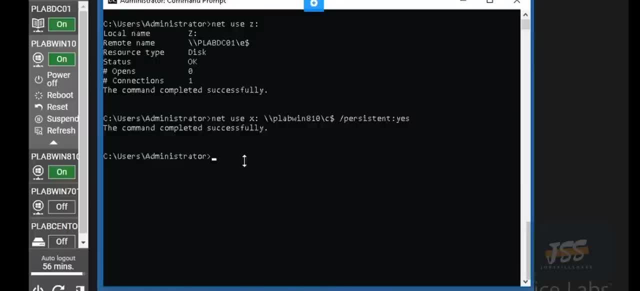 first. so, first, so you can type net dash, use, you can type net dash use, you can type net dash use, dash, dash, dash. that specific letter, that specific letter, that specific letter which you need to find out from the file, which you need to find out from the file. 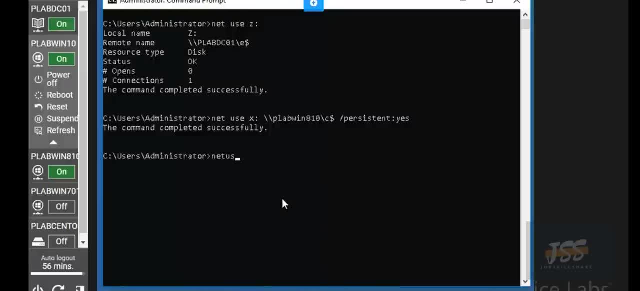 which you need to find out from the file: explorer, explorer, explorer. so it's up to you if you remember so. so it's up to you if you remember so. so it's up to you if you remember. so don't need to open the fire. don't need to open the fire. 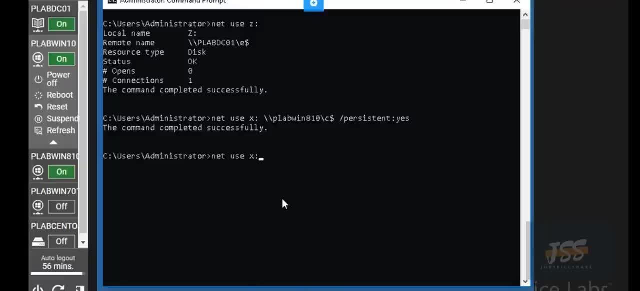 don't need to open the fire. file explorer type: net space. use space. file explorer type: net space: use space. file explorer type: net space. use space x- column space x- column space x- column space- false slash and delete false slash and delete false slash and delete. so this argument will help you to delete. 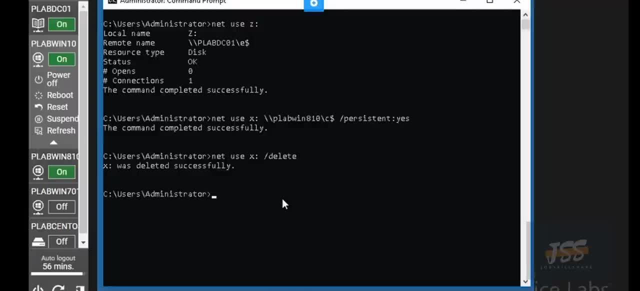 so this argument will help you to delete. so this argument will help you to delete your specific, your specific, your specific network drive that you just mapped, but now network drive that you just mapped, but now network drive that you just mapped, but now do you want to delete that one? 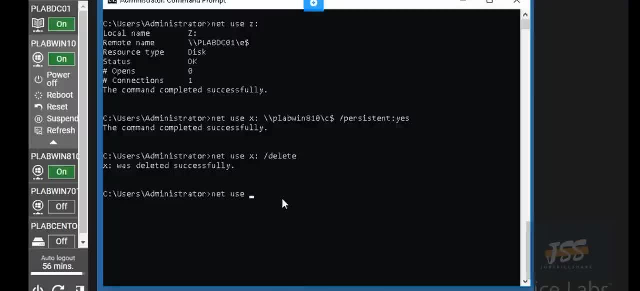 do you want to delete that one? do you want to delete that one? and, and and you will. if you want to find out that, you will. if you want to find out that you will. if you want to find out that thing, thing, thing, so you can go. 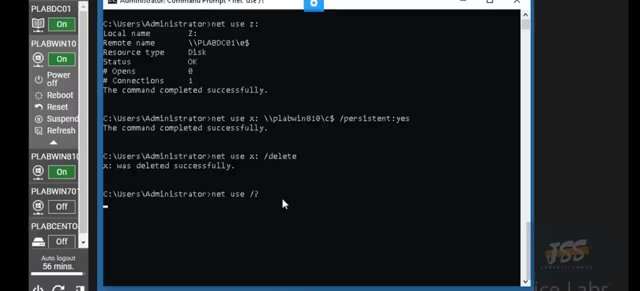 so you can go. so you can go to the file explorer and want to explore to the file explorer and want to explore to the file explorer and want to explore other arguments of this net use. so other arguments of this net use. so other arguments of this net use. so simply type net space, use space. 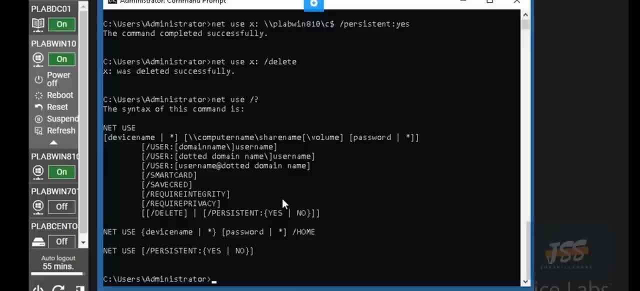 simply type net space, use space. simply type net space, use space. false slash question mark. so it will false slash question mark. so it will false slash question mark. so it will show you, show you, show you that there are arguments in the keywords, that there are arguments in the keywords. 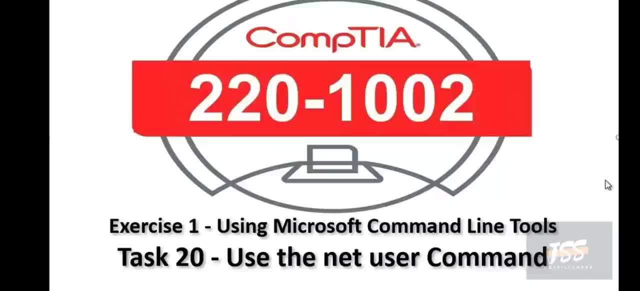 that there are arguments in the keywords that you can use along with the net use. that you can use along with the net use, that you can use along with the net use. use the net user command, use the net user command, use the net user command and this command allows you to perform. 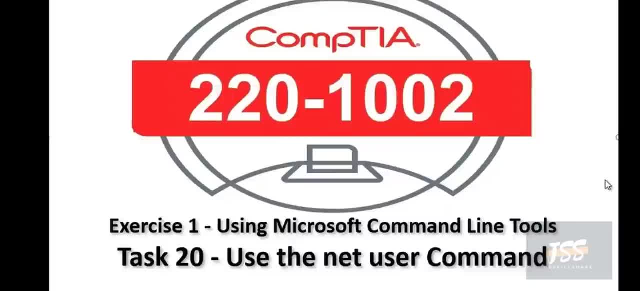 and this command allows you to perform. and this command allows you to perform user account related task. user account related task, user account related task on the computer. so this command allows on the computer. so this command allows you to create new user. you can modify you to create new user, you can modify. 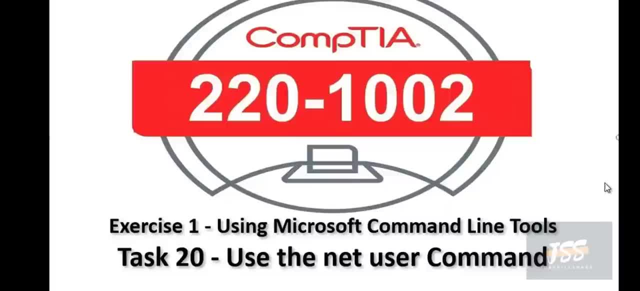 you to create new user, you can modify the user account related parameters and the user account related parameters and the user account related parameters. and this account has various parameters to this account, has various parameters to this account, has various parameters to it, so each one of them perform a 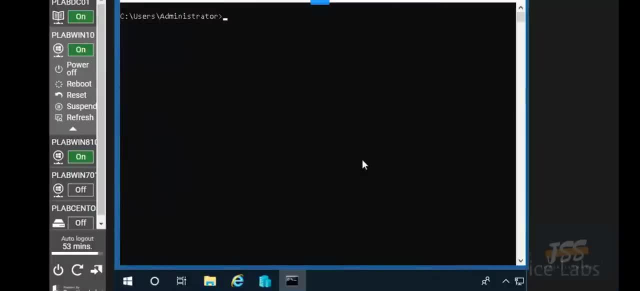 it, so each one of them perform a it, so each one of them perform a specific task, specific task, specific task. so using this command, you can manage. so, using this command, you can manage. so, using this command, you can manage local and both domain based user account, local and both domain based user account. 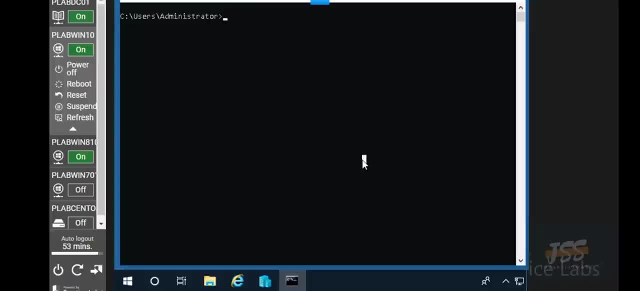 local and both domain based user account. so let's open the cmd. so let's open the cmd. so let's open the cmd in type, in type in type: net space, net space, net space, user, user, user. so so right now we're going to use it on. 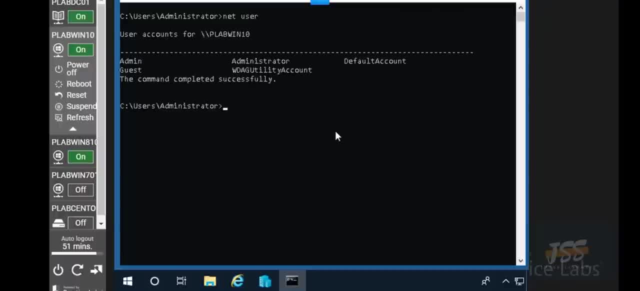 so right now we're going to use it on. so right now we're going to use it on the local, the local, the local system and type net space user, and there system and type net space user, and there system and type net space user. and there you go. 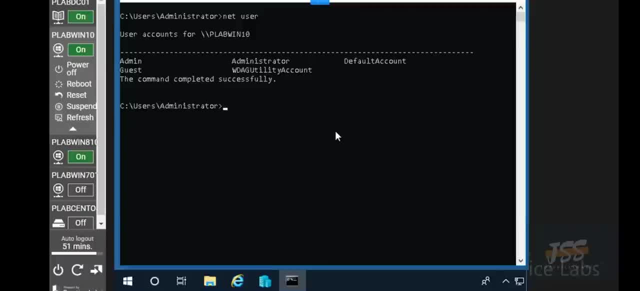 you go. you go show the list of all local users. you show the list of all local users. you show the list of all local users you have in this machine, have in this machine, have in this machine. so for getting the list, you just need to. so, for getting the list, you just need to. 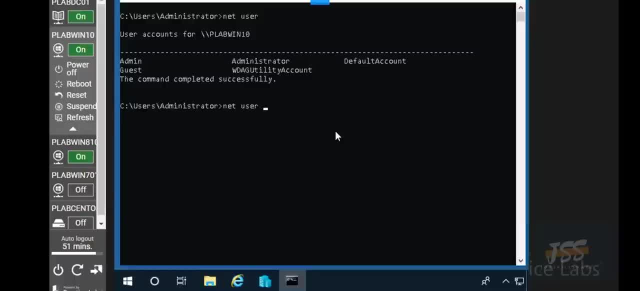 so for getting the list, you just need to type let space user, it will show you. type let space user, it will show you. type let space user, it will show you. then if you want to view the information, then if you want to view the information, then if you want to view the information about specific users, you can type net. 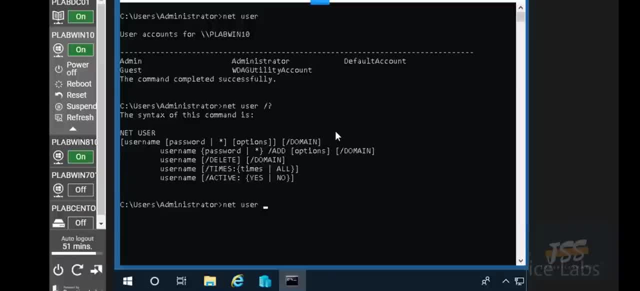 about specific users. you can type net about specific users. you can type net. and if you want to know the arguments, so, and if you want to know the arguments, so, and if you want to know the arguments, so run full slash question mark and right. run full slash question mark and right. 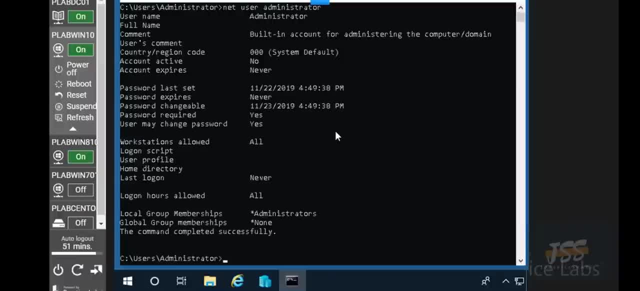 run full slash question mark and right now i want to see the specific user. so i now i want to see the specific user. so i now i want to see the specific user. so i type net space user administrator and type net space user administrator and type net space user administrator and now it's showing me. 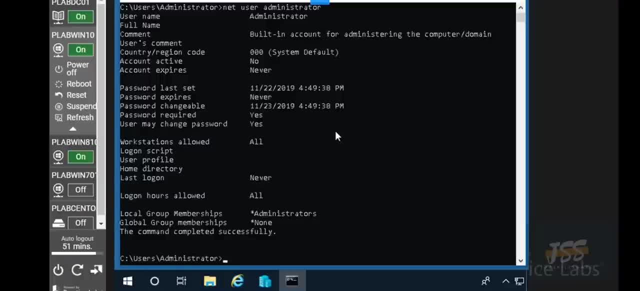 now it's showing me. now it's showing me what the information about the specific, what the information about the specific, what the information about the specific user: user: user, the administrator and all the permissions. the administrator and all the permissions. the administrator and all the permissions, password, things and account expiry. 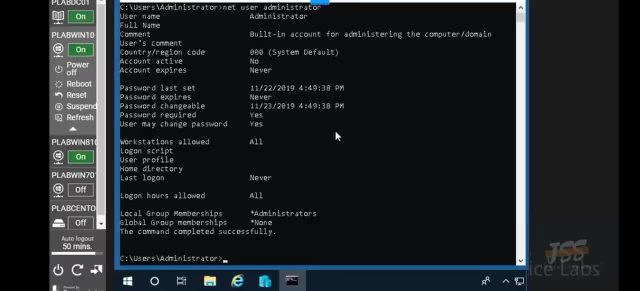 password things and account expiry, password things and account expiry and other workstation allowed and last and other workstation allowed and last and other workstation allowed and last hour logon allowed. hour logon allowed. hour logon allowed. and local group membership- global group and local group membership- global group. 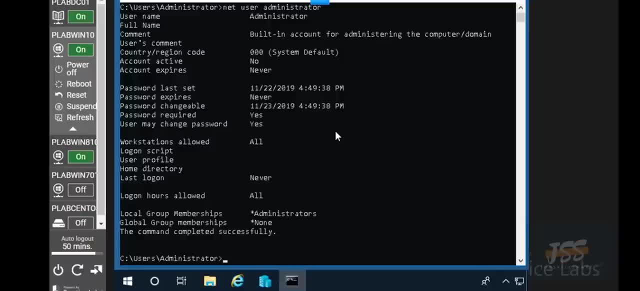 and local group membership, global group membership, membership, membership- all the basic information about the user. all the basic information about the user, all the basic information about the user. it is showing here, it is showing here, it is showing here: after executing that command, after executing that command, after executing that command, then 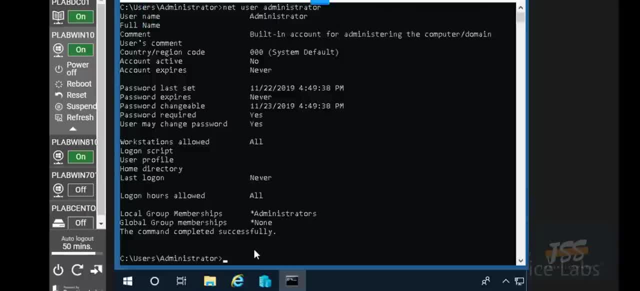 then then we can simply find out other things. we can simply find out other things. we can simply find out other things and we can manage, and we can manage and we can manage account credentials. so, if you want to account credentials, so if you want to account credentials, so if you want to create new account by using the net user, 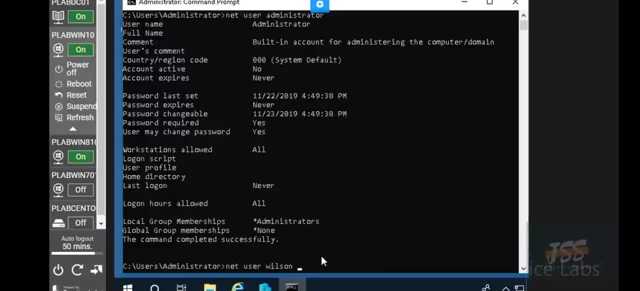 create new account by using the net user. create new account by using the net user so we can type net user space any name. so we can type net user space any name. so we can type net user space any name, like we're using wilson, like we're using wilson. 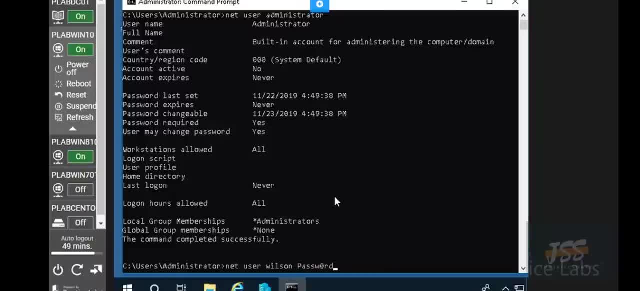 like we're using wilson, and then just directly type this exact. and then just directly type this exact and then just directly type this exact password that you want to set password that you want to set password that you want to set. then space false slash. add false slash. 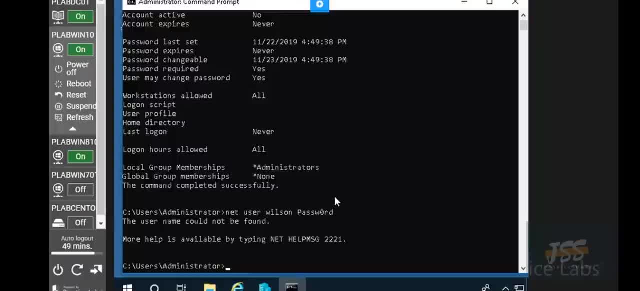 then space false slash, add false slash. then space false slash, add false slash. time, time, time, and then, and then, and then colon, all, colon, all, colon, all. so it will, so it will, so it will, directly, directly, directly, in an instant, create the account and when. in an instant, create the account and when. 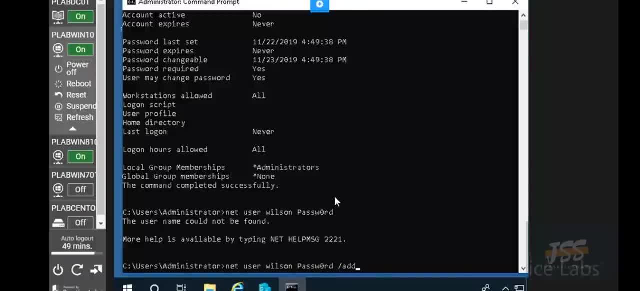 in an instant create the account and when you add false slash add parameter it, you add false slash add parameter it. you add false slash add parameter, it adds the user account and the user is adds the user account and the user is adds the user account and the user is configured to log on all days of the. 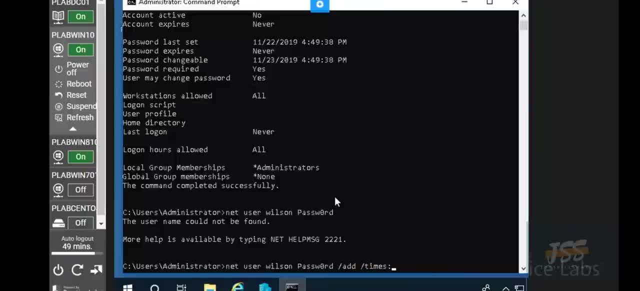 configured to log on all days of the configured to log on all days of the week, week, week, so, on the above, we miss the remaining. so, on the above, we miss the remaining. so, on the above, we miss the remaining arguments of this command. that's why arguments of this command. that's why 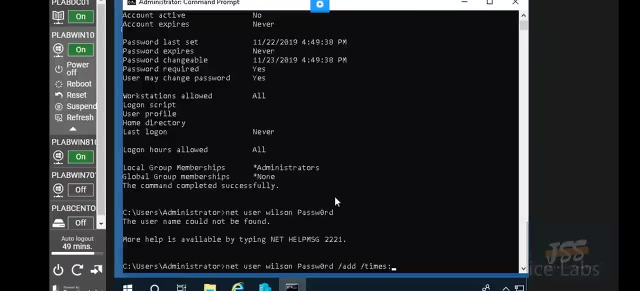 arguments of this command. that's why we see we saw this error, we see we saw this error, we see we saw this error. now we're going to use, now we're going to use, now we're going to use these false slash add and then false: these false slash add and then false. 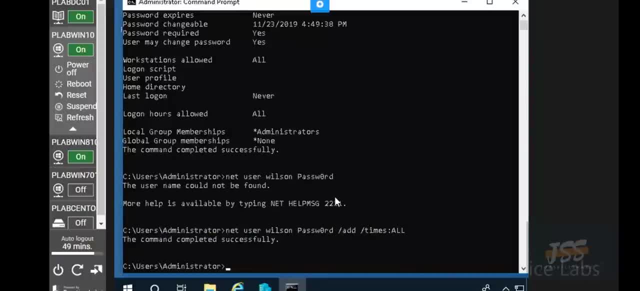 these false slash add, and then false slash, these false slash add, and then false times colon. all so, now it is the proper times colon. all so, now it is the proper times colon. all so, now it is the proper way to execute the command. in order to way to execute the command, in order to 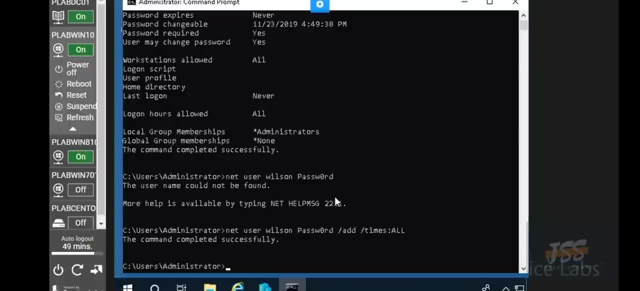 way to execute the command in order to create the new user. create the new user, create the new user and the command is successfully executed. and the command is successfully executed and the command is successfully executed as you can see the message. as you can see the message. as you can see the message. now you can recall the net user command. 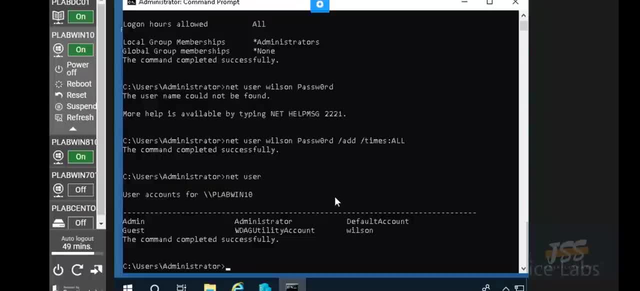 now you can recall the net user command. now you can recall the net user command and just see, and just see and just see the list of user. and there you go, you the list of user. and there you go, you the list of user. and there you go, you have the wilson in the list. 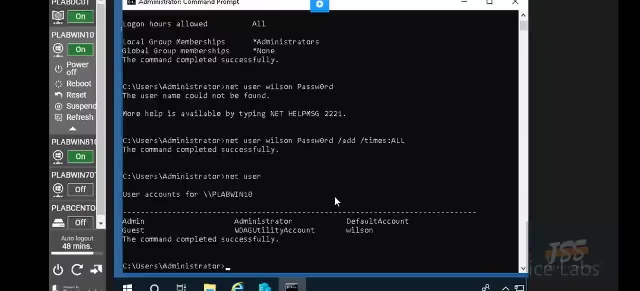 have the wilson in the list. have the wilson in the list, just add it after you create it, just add it after you create it, just add it after you create it. and if you want to delete any user, so, and if you want to delete any user, so. 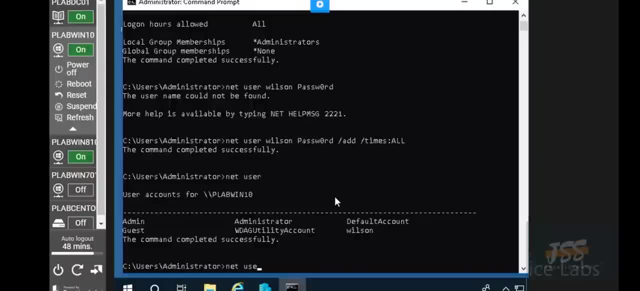 and if you want to delete any user, so simply type net space- here space that. simply type net space- here space that simply type net space- here space that specific user. then space false slash specific user. then space false slash specific user. then space false slash and delete and delete. 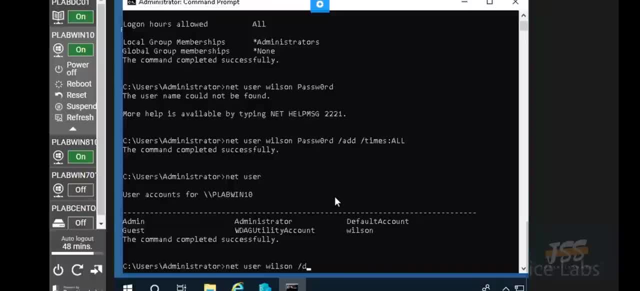 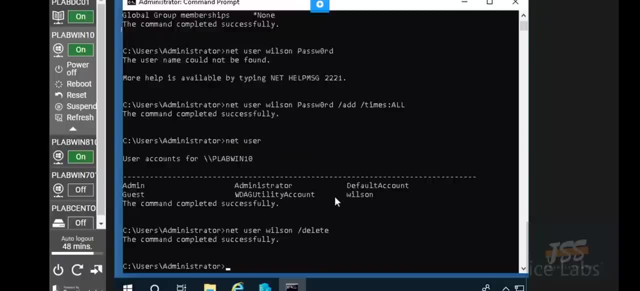 and delete. so it will delete the newly created user. so it will delete the newly created user. so it will delete the newly created user. or, or. or. you can delete any previous user you have. you can delete any previous user you have. you can delete any previous user you have on the local machine. 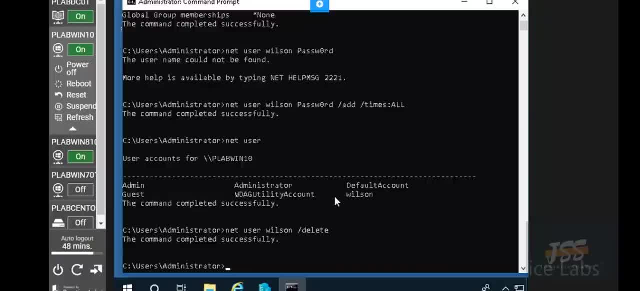 on the local machine. on the local machine. then again recall, then again recall, then again recall. basic net user command. i will show you basic net user command. i will show you that user that you just deleted, that user that you just deleted, that user that you just deleted. so 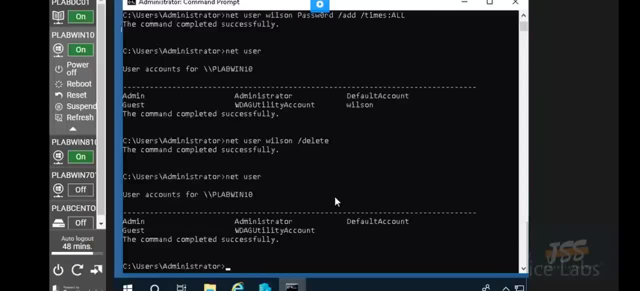 so. so verification is a good thing. verification is a good thing. verification is a good thing. you need to. you always have to verify, you need to. you always have to verify, you need to. you always have to verify after, after, after doing things. so there you go, there's no. 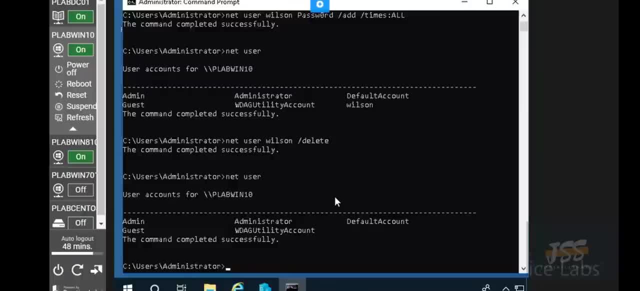 doing things. so there you go. there's no doing things, so there you go. there's no entry of the wilson here, entry of the wilson here, entry of the wilson here. and we already showed you how to explore, and we already showed you how to explore. 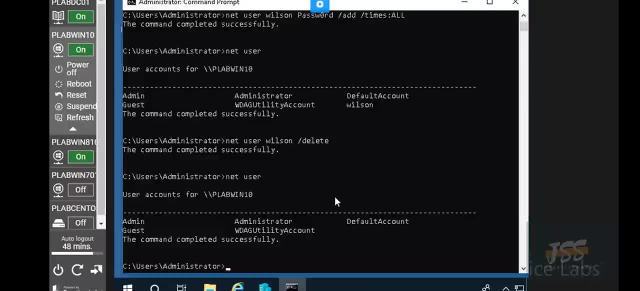 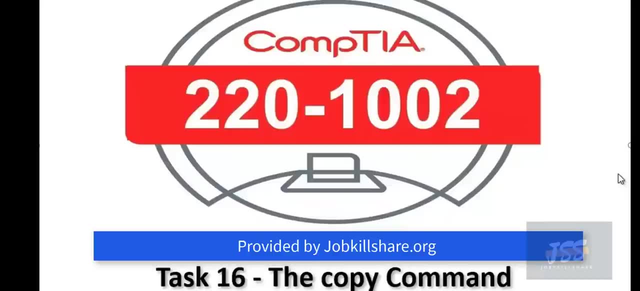 and we already showed you how to explore its other arguments and keywords, its other arguments and keywords, its other arguments and keywords that you could use with the command, to that you could use with the command to do different things, the command, and here in this video we're going to show you different functions. 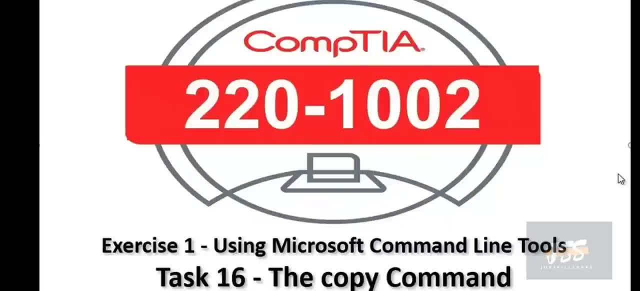 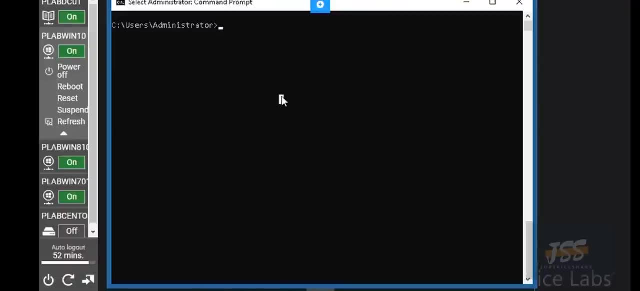 of this copy command and how it is useful to copy any file, any text file or any file, because you are familiar with the GUI environment, how to copy things and it's so easy peasy to just right click on any file and copy things. so first let's open the command. 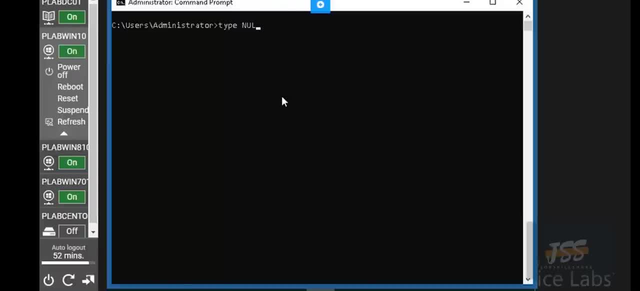 prompt with the administrator privilege and type space, null space, dot, not dot. the gradient, then symbol, then abc text file. that would be any file you have in dot text. so this command does what it's an easy to create a text file using a notepad, but it it's a bit. 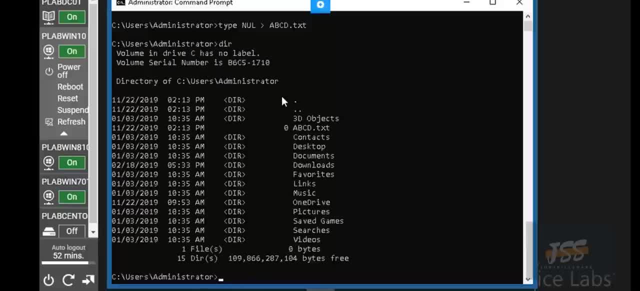 tricky, because what you're doing in a command prompt and if you then run the dir, so you will see the file. now, after creating the file, you can simply just locate the file in the directory and then type, copy space, that specific name and the location where you want to copy that file. so it would be. 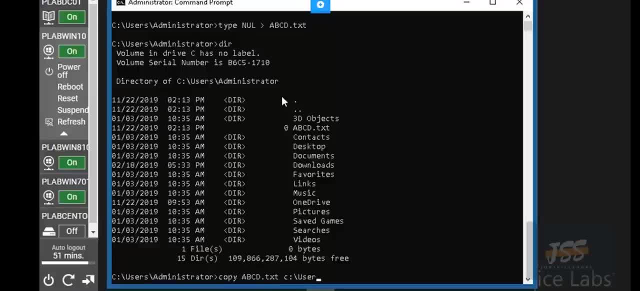 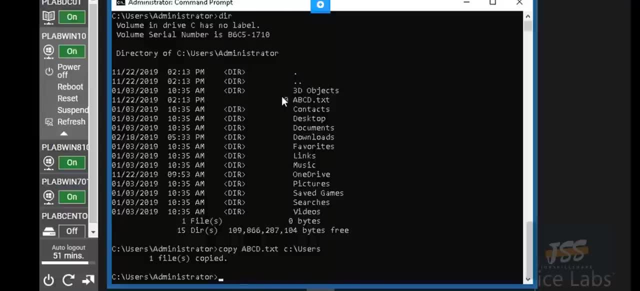 like c colon users, and it would be whatever it, whatever you like, whatever you, wherever you want to copy that file and it will be copied. and if you add this forward, slash y extension. so when you have a copy to a file, to destination, the same file exists, but you will be prompt with 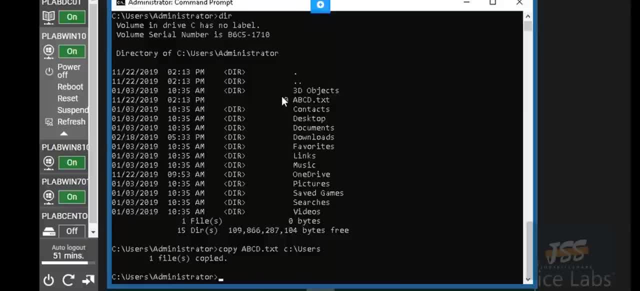 the warning and if the file exists in the same directory, so you can still override without getting the warning. so if you want to override the file on the same specific location, so you need to add this forward slash y parameter. so this is suppressing the prompt for confirmation to 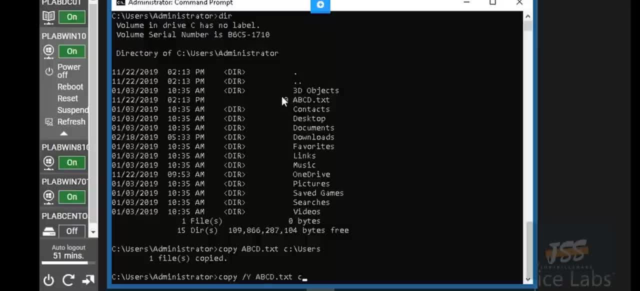 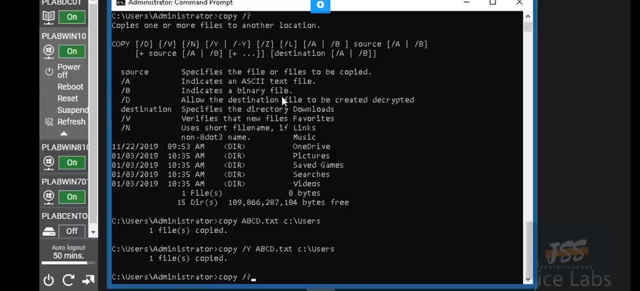 override a file on that same location. so here we're going, we're going to copy the same file on that same location and here we are already adding forward slash y. so it didn't ask for the confirmation for overriding, now we're going to. if you want to verify and explore other arguments, 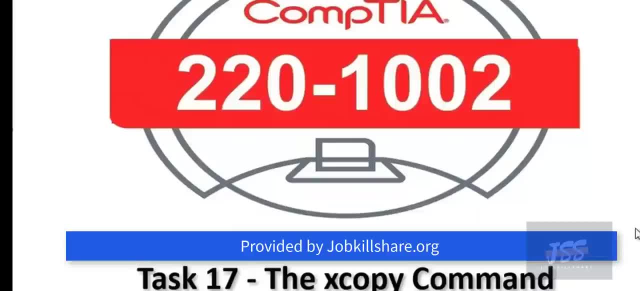 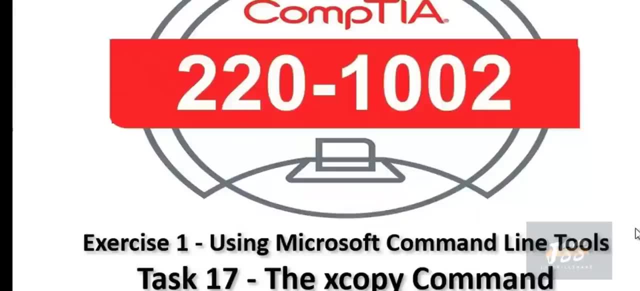 so just type false question mark in the x copy command. and this command is useful to copy the file, as well as the directories, from the source location to any specified location. and while copying this directory, this command also copies the subdirectory of that directory and as well, if it's present. so to performing to experience this command. 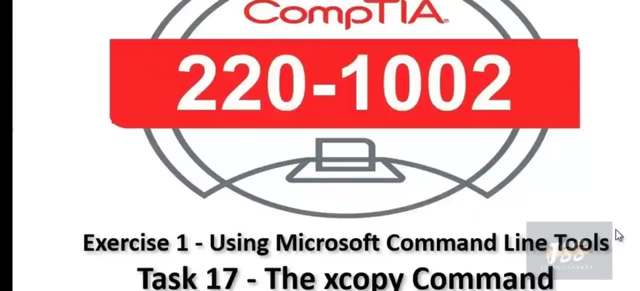 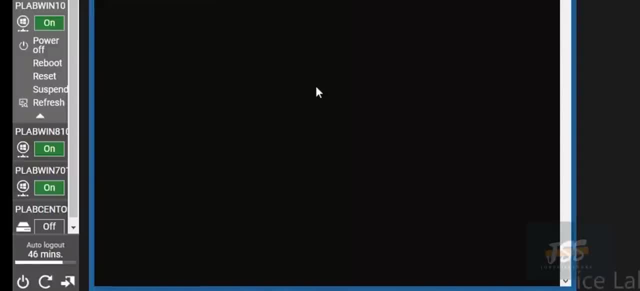 on the cmd, first, let's move. let's move to the practice labs resources, practice labs portal. in here on the command prompt, we're going to type x, copy space, forward, slash, y and here start dot text space c, colon, backslash user. this would be the location and here 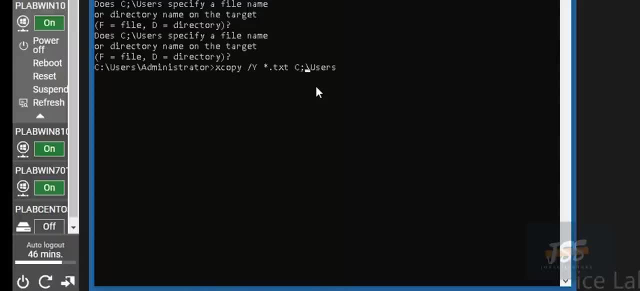 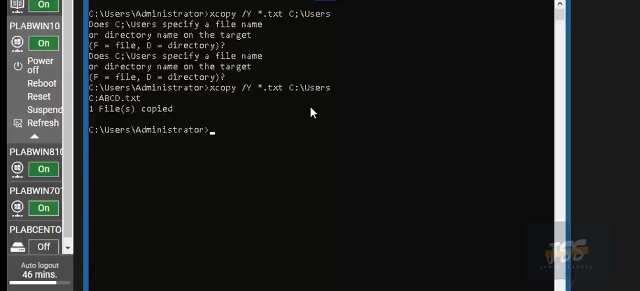 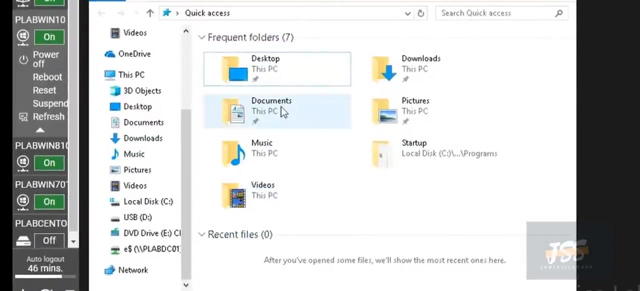 it will copy the directory as well as the subdirectory and it shows that it has these directories. and now you can see: the one file is copied, abctxt, along with these directories. so in this way, this command, it simply allows you and enables you to download the file along with its directory. now we're going to now copy these folders that 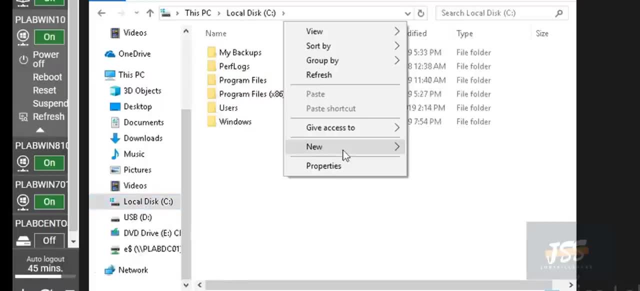 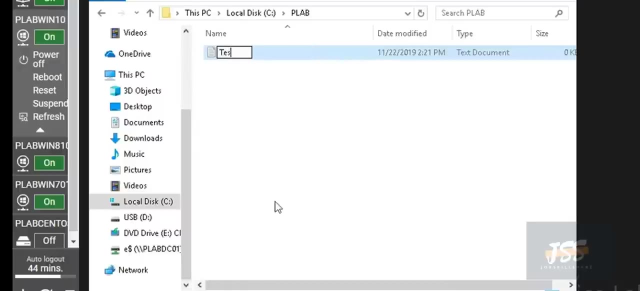 have multiple directories within. so if you go to the c and create the new folder, let's say plaps, and now if we create another folder in that folder, so we create the test file here within this folder subdirectory. it would be so we're creating another file, text, test.2, here for this command. now. 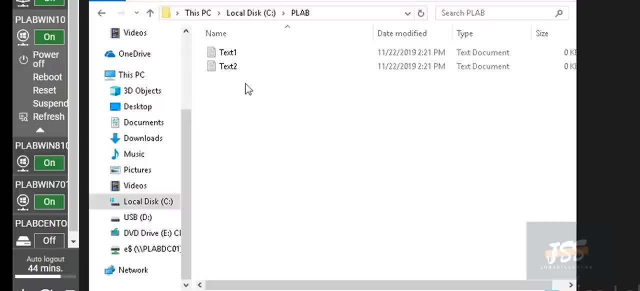 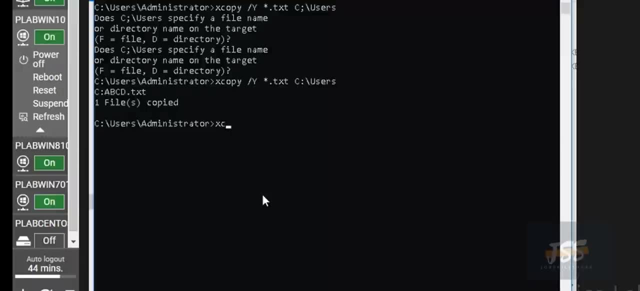 you can see, we have two files within this plap folder and then we're going to copy this plap directory to another location. so we did the same. we type x, copy space c, backslash plap, and there we're going to provide the destination location and then put forward slash e. 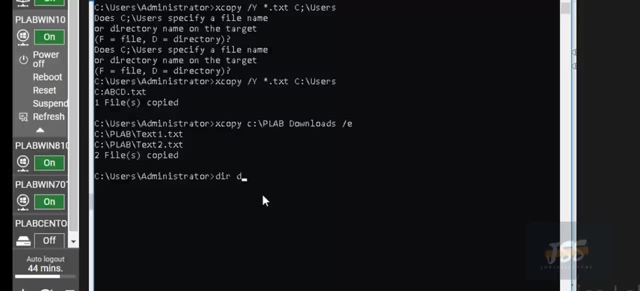 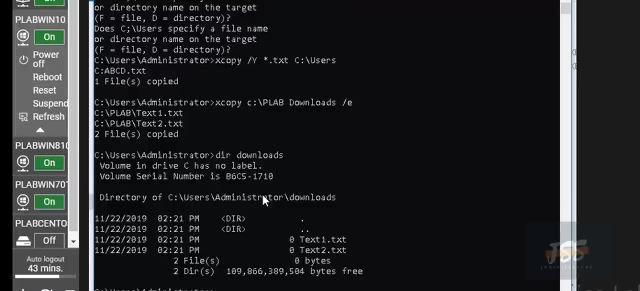 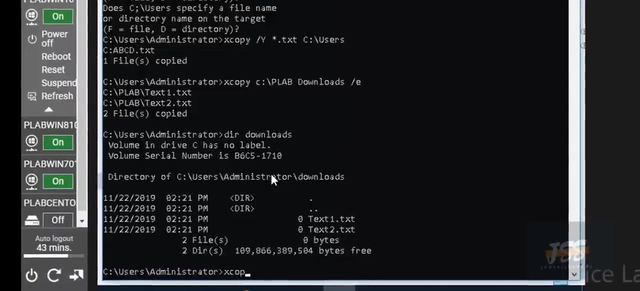 so you can see the both files are copied, along with the directories: dir space, download to see the download directory. so there you go, you found both files here. so in this way you directly copied the internal files of that folder to that specific location, right? so in the same way you can. you wanna, if you want to explore this command, start forward slash. 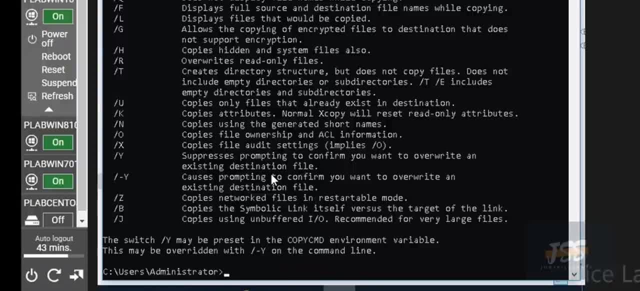 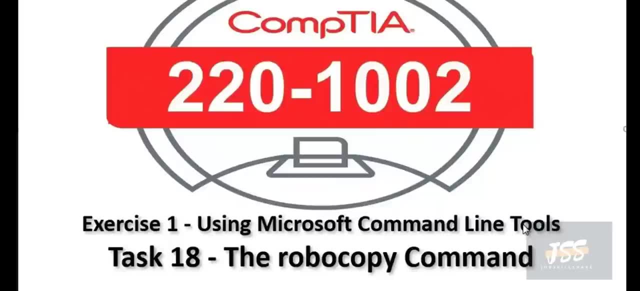 question mark and you will see and you will find out different arguments that you can add. and here in this command we're going to show you the robocopy command and it copies the file data and all the necessary parameters have to be passed in the command itself. so the source: 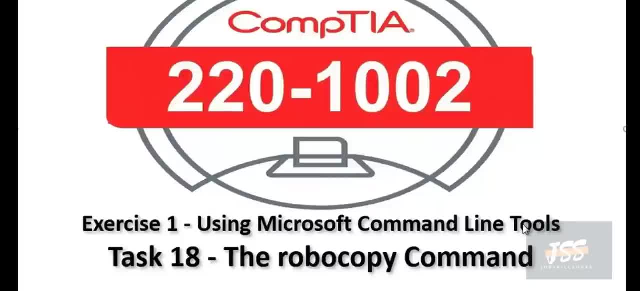 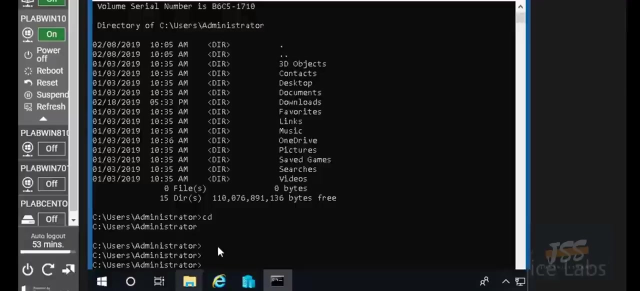 directory, destination directory and file and whose content are to get copied. like details are specified, so the robocopy command will keep the original file and create what a replica of the same at the specified location. so in this test, we're going to show you how to use the robocopy command in environment in the command prompt. so let's start. 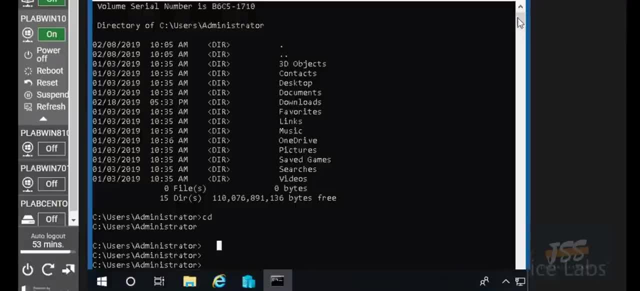 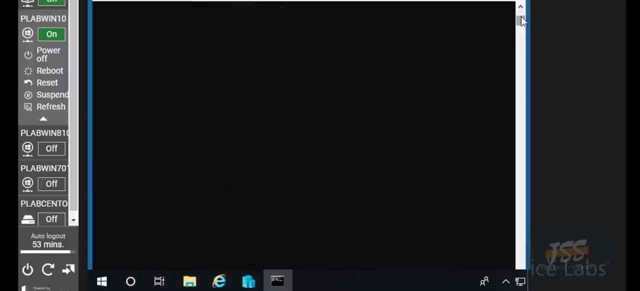 with the CMD and here, as you can see, in the previous command we already created directories with the xcopy command video. the last one now here. let's scroll up and type robocopy for the xcopy command, and here you can see that the xcopy command is already created, so you can. 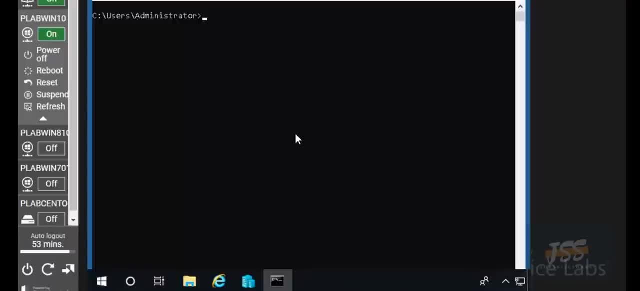 go back to the xcopy command, and here you can see that the xcopy command is already created, so you can first clear the screen and then we're going to type the robocopy. space downloads, space c, column backslash users. so this users would be the specified location. 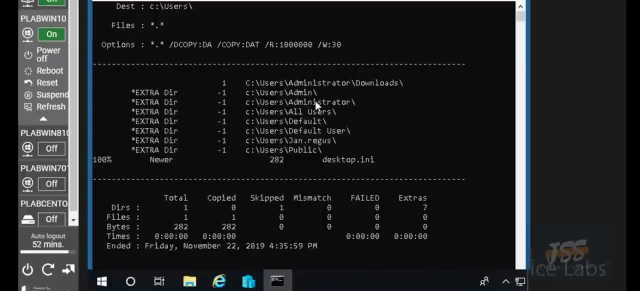 and now it shows this data, this detail, and it shows what? that it created the replica of the original file and it copy all the content in the source directory, the destination directory. in the file the content is just copied, so the details are specified, and it kept the original file and create a replica of the same at 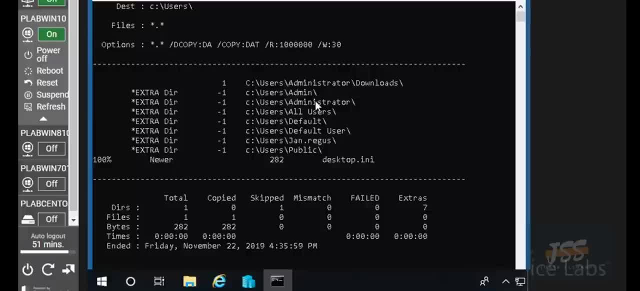 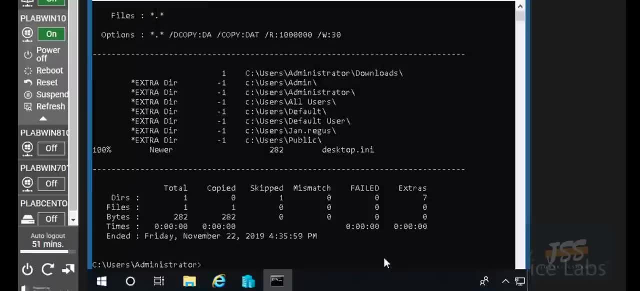 the specified location. so this is the benefit of this Robocopy command and there are few other and various parameters of this command we have and if you want to see, if you want to know about those parameters, you simply do what type Robocopy space forward, slash, question mark and then execute so it. 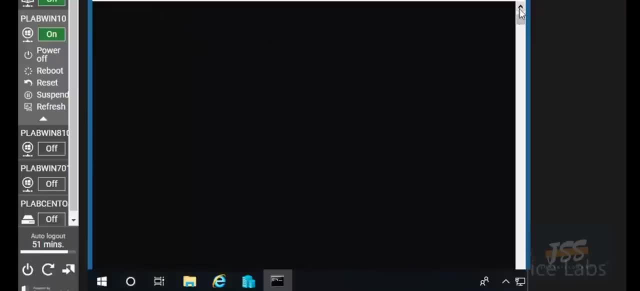 will show you the other rest of other arguments that you could use. you could use the other arguments that you could use and then execute. so it will show you the other rest of other arguments that you could use with that command to do different things and use in different environment. 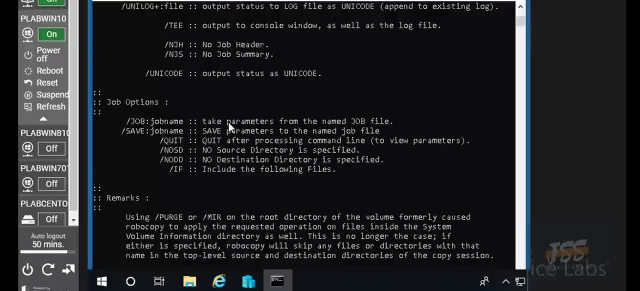 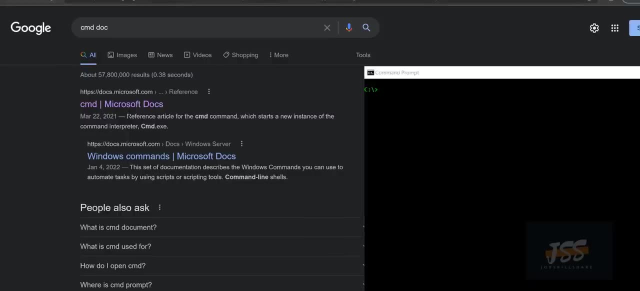 in different scenarios. so it will show you the rest of other arguments here on the screen. so that's it for this video. stay with us and thanks for watching now. this is great knowledge so far. after this, of course, there's- this is not an ending skill, so you can go to google, type CMD doc and you will see this Microsoft link click. 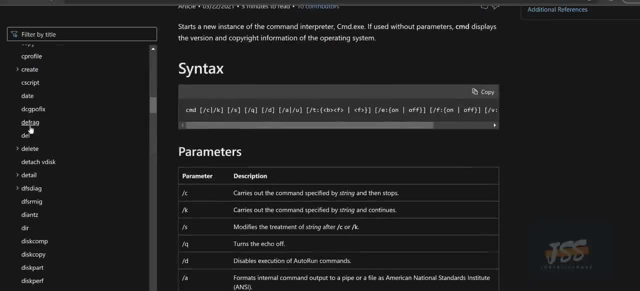 on it and then you can use so many other commands there is available inside for you to practice so you can create some batch files after this. if you feel like you're really good at using these commands now, then go and find some more commands that can help you with your job or your future skills, but try to get 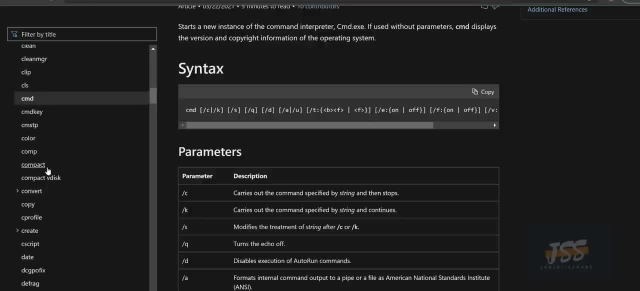 into scripting. then you get into scripting. you'll be able to use two commands together. maybe you want to copy one command and then do something with it. delete it later on. so create some batch files. these are the scripting you can do on cmd. so create something like that where you can actually achieve more. 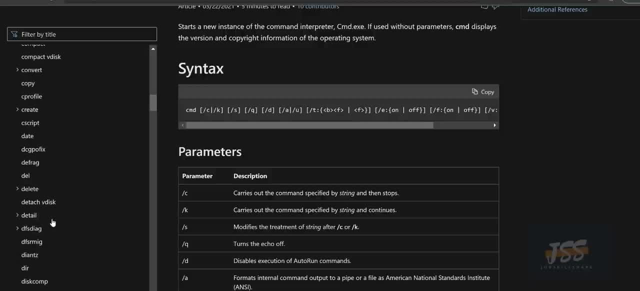 out of it and that's where your mind will start to accept advanced learning, and the more you get into this stuff, the later on you're going to do a lot of advanced stuff in devops. or maybe you want to become a sysadmin where you have to work with a lot of partial, and that's where things can go. 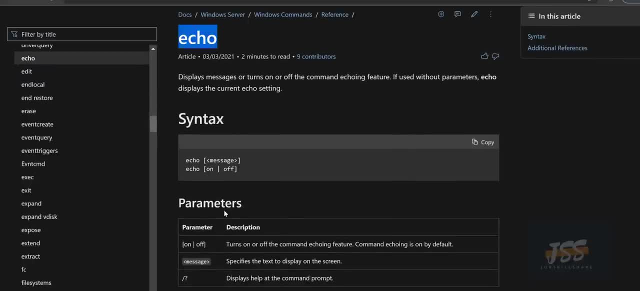 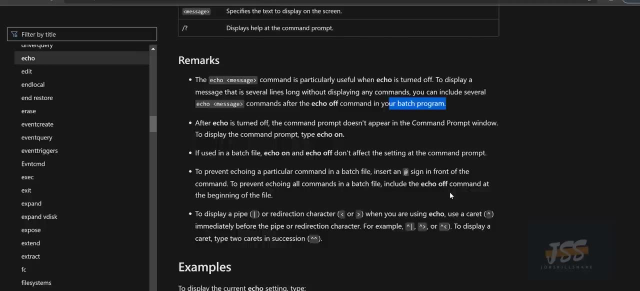 into that. so maybe you can start with the echo command where you can start doing that- batch files and everything. as you can see here, there is some information about it so you can use it- there's examples out here- and have you know a go with this, because this is a 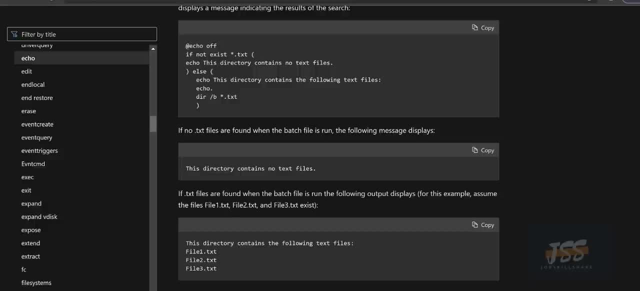 you know, a go with this, because this is a go with this, because this is a go with this, because this is really going to help you. thank you so much for watching this. don't forget to subscribe to our youtube channel to see more videos like this.